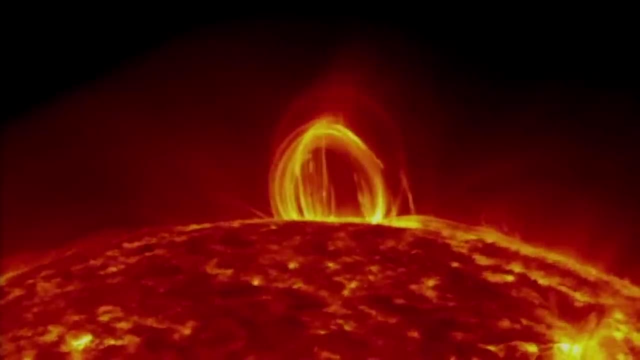 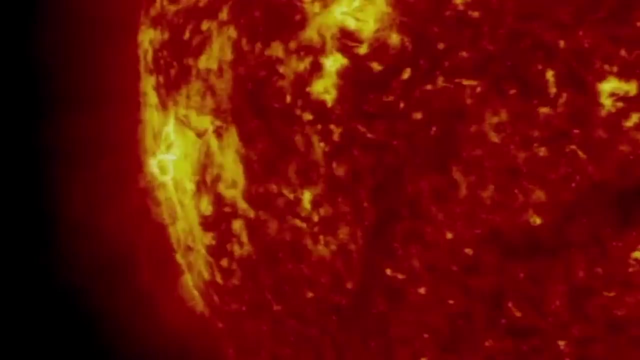 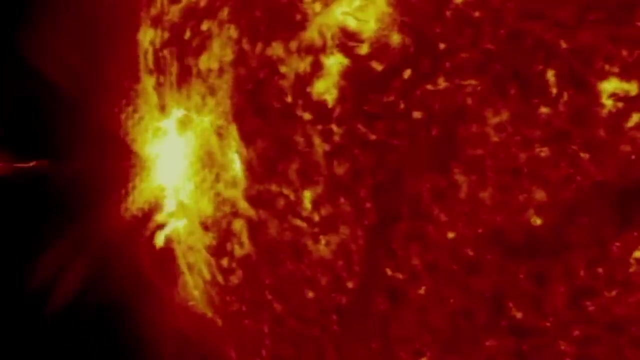 But in a sense what the theme is. It's going to be about power in the universe. what are the most powerful objects in the universe that we can see? and often it's involving magnetism. sometimes it's gravity. most often gravity and magnetism that is driving what I'm going to talk about. 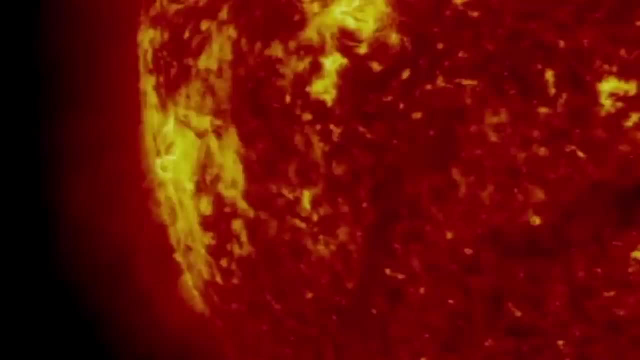 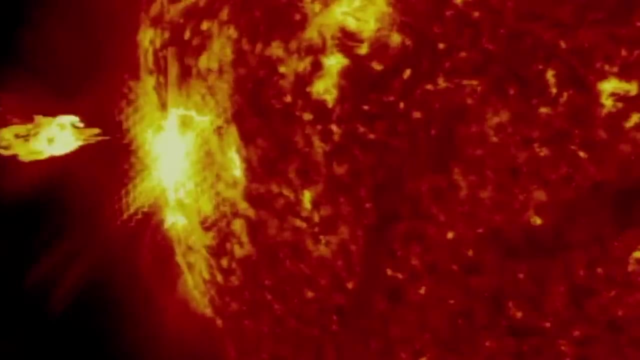 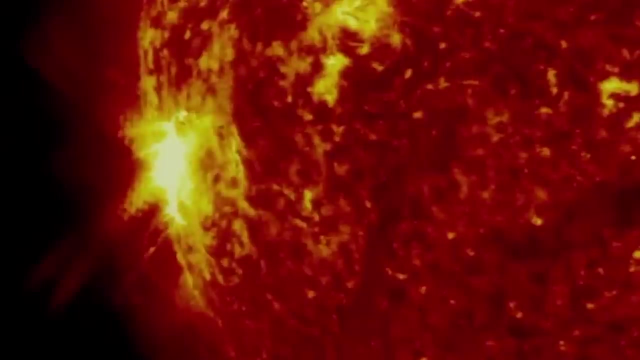 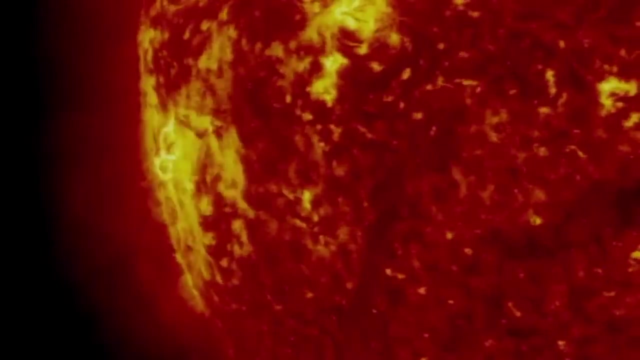 So I'll move ahead talking now. looking at these eruptions from the sun connected with solar flares. The sun is actually a very inactive star compared to many stars out there. It's a dwarf star, and things about our solar system are not very eruptive like this. 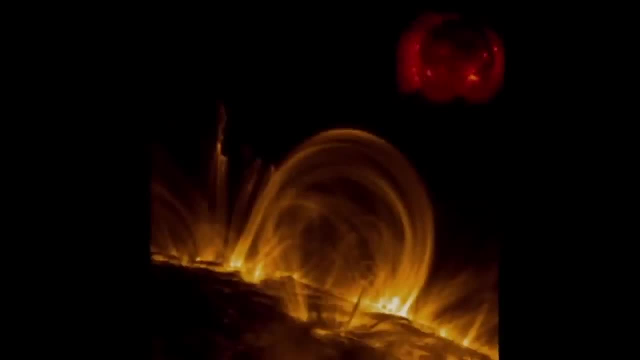 thankfully for us, I think. But what we've got on the sun? the sun, as you know, has not got a solid surface, but it's a gas ball and it's rotating, not this fast, in this little X-ray image up here. 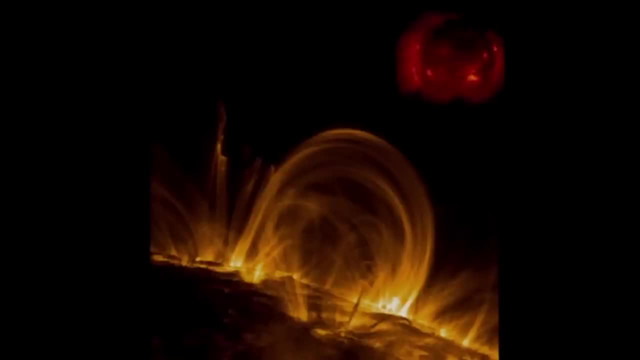 It rotates at 26 days at the equator and at 30 days at the poles. This means it's differentially rotating, And if you differentially rotate a magnetized plasma, it's like winding up a basket full of rubber bands. 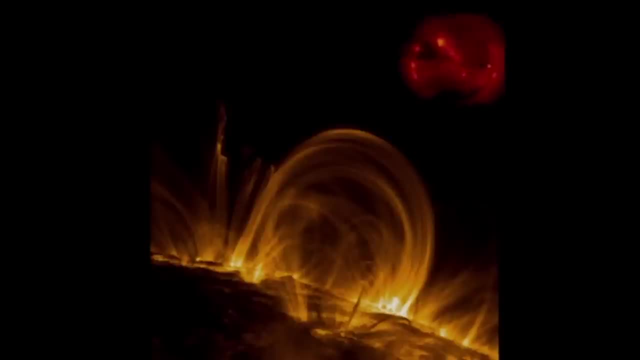 Eventually they start springing out, and here are the rubber bands, the magnetic field lines springing out from the surface of the sun in this picture down here, taken in the ultraviolet. But sometimes there are really enormous eruptions on the sun, so-called solar flares. 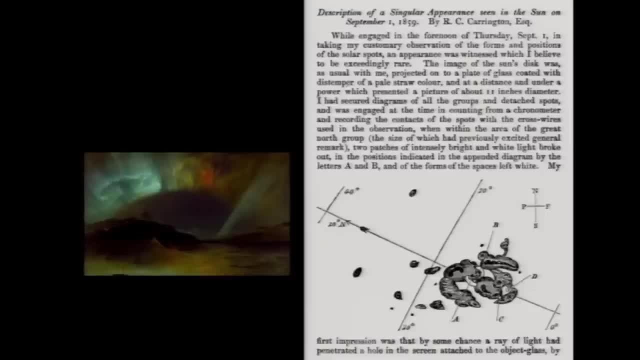 and perhaps the brightest solar flare seen in historical times was recorded by RC Ritchie Ritchie Carrington Esquire, while engaged in the forenoon. how many of us talk about the forenoon of Thursday September the 1st? 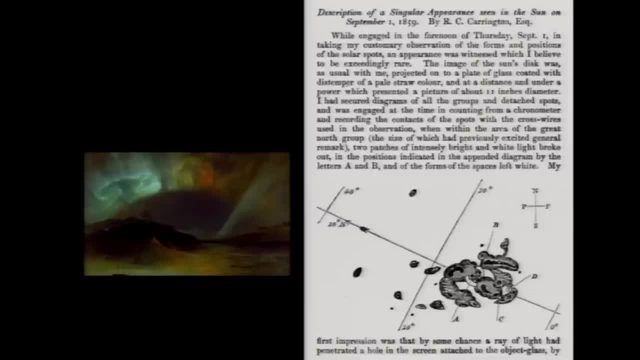 in taking my customary observation of the forms and positions of the solar spots, an appearance was witnessed which I believe to be exceedingly rare, And that is in this drawing here. it's these white bits just here and what we refer to as a white light flare. 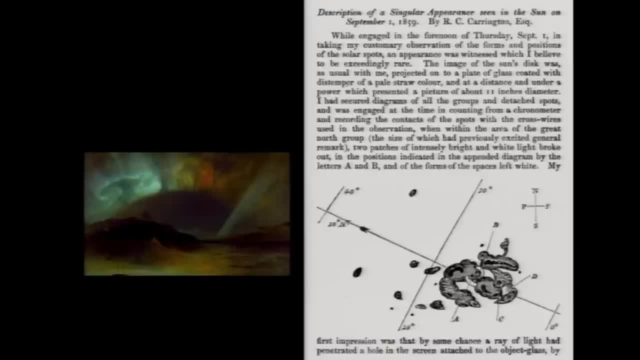 Now, white light flares on the sun are very rare. He's the only one to have seen one and it was verified by somebody else, so it's a genuine observation, But it coincided with the observation of the aurora. This is a painting of observation of the aurora as far south as the Caribbean. 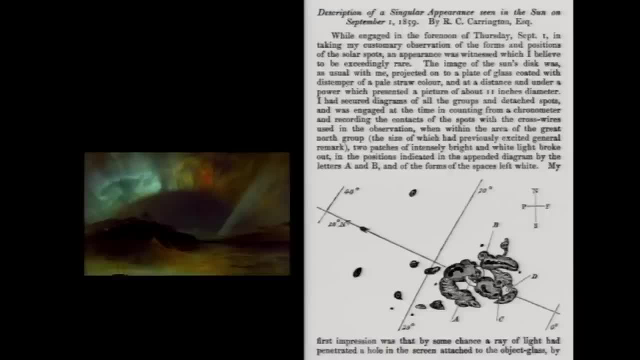 Also, back in those days they had telegraphs connecting cities that ran along railway lines and things. They were long wires And people, People were getting sparks off them and things were being set on fire by them. This is because there was an enormous eruption from the sun at the same time. 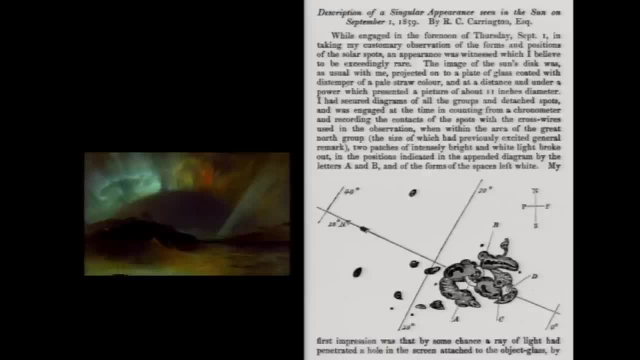 or plasma coming out directly towards the Earth, and that plasma striking the Earth a few days later, giving rise to all these phenomena. Essentially, what you've got is the Earth's magnetic field is encased in this solar wind all the time, but there's a big eruption passing through it. 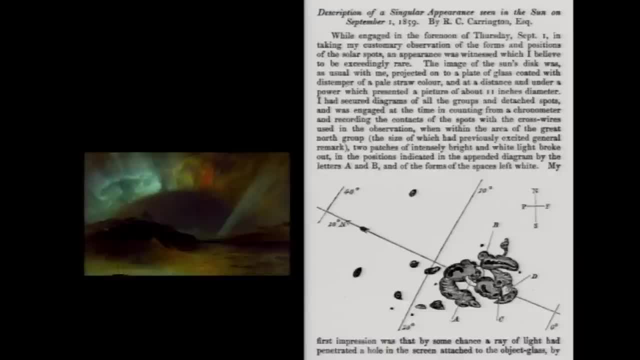 It squeezes the Earth's magnetic field and everybody knows from Faraday's law that if you move a magnetic field you generate an electric field, and those electric fields lead to all of this phenomena, and also the sparks And were one, to happen today. 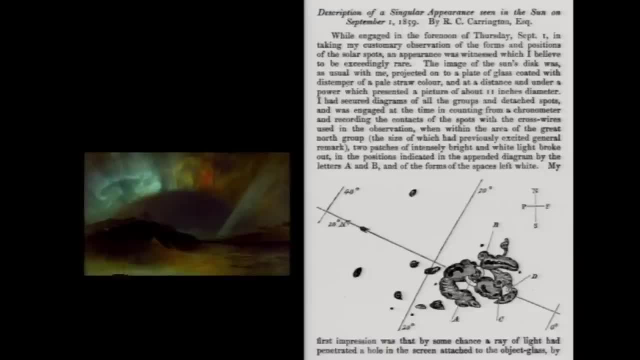 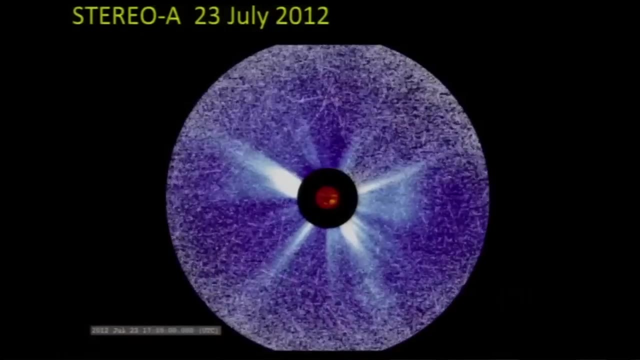 it could easily wipe out many of our transmission systems and wipe out our satellites, particularly the GPS satellites. The next time one happens- and they're not predictive, we can't predict when they occur- the next time one happens, I don't want to be landing in an aeroplane. 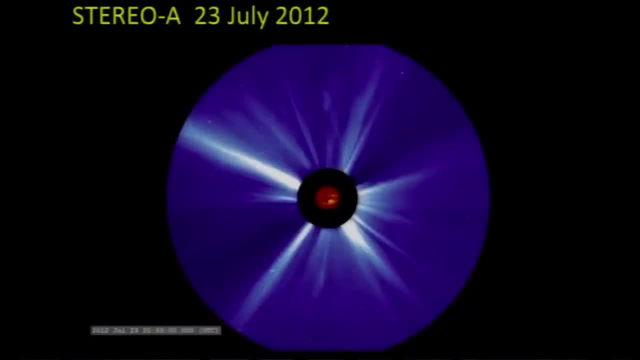 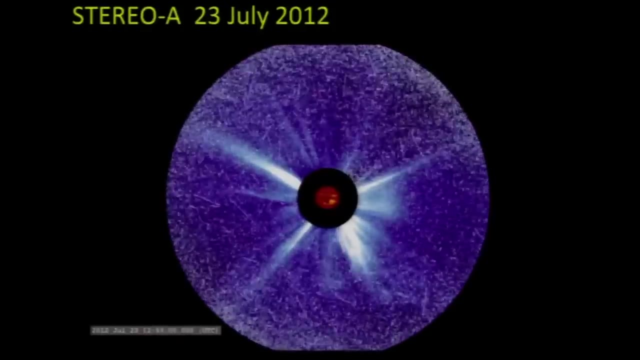 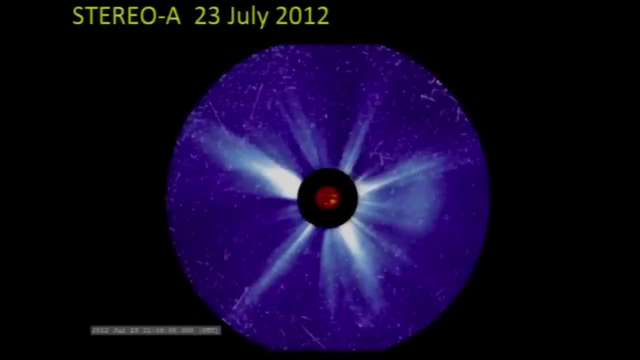 Now it was thought that these were extremely rare and haven't happened recently, but actually we have got two satellites monitoring the sun: one ahead of us in our orbit, one behind us in our orbit by about 60 degrees, and they're called Stereo A and Stereo B. 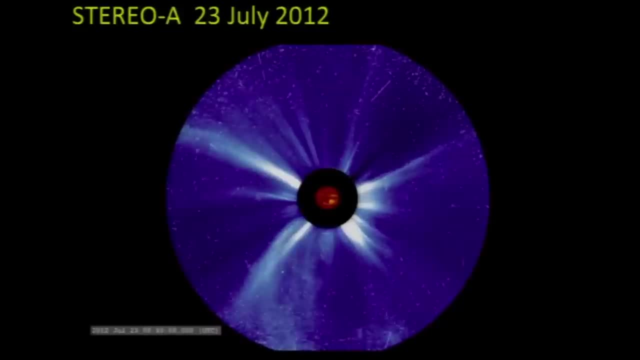 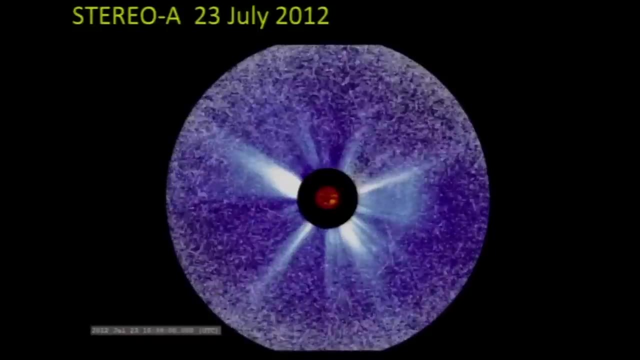 You're now seeing the whole of July, the 23rd 2012.. That's the sun in the center. It's just an image pasted on. This is a disk blotting out the image of the sun and you can see in this speeded-up movie. 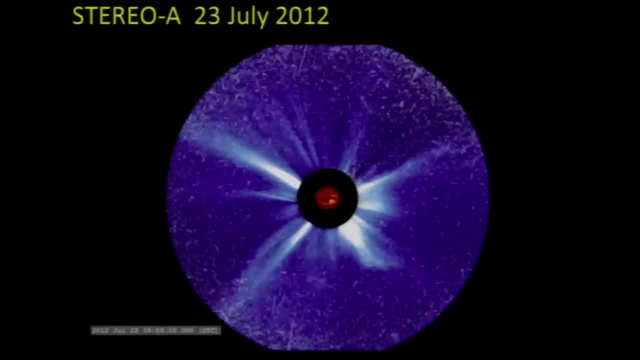 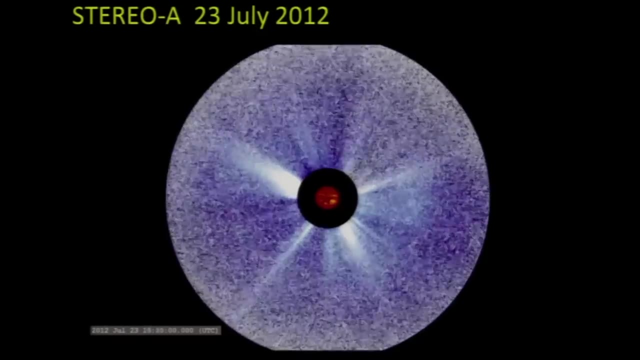 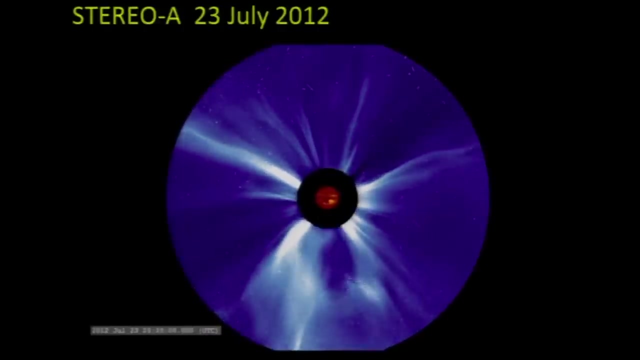 you can see that something is erupted from the sun. Here it goes, this vast coronal mass ejection it's called. But notice how this image suddenly gets terrible. It's full of It's full of spots. That's because there's a vast cloud of very energetic particles coming out as well. 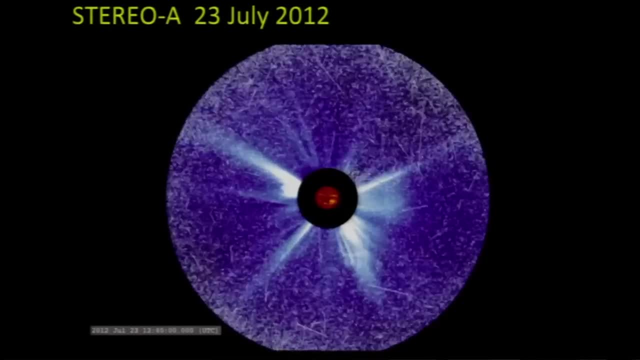 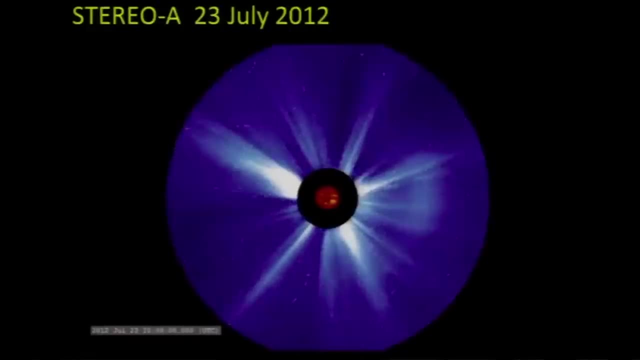 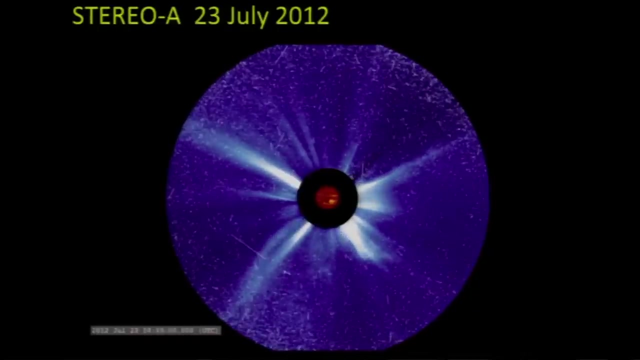 and those energetic particles which come out only slightly slower than the speed of light are then bombarding that satellite with this intense- It's very intensely- irradiated. That's what causes a lot of damage to satellites. It's what we don't want. 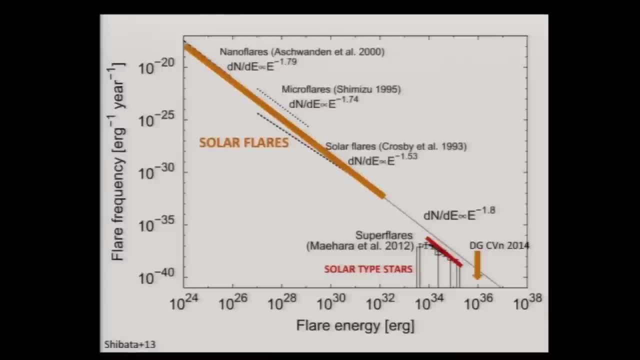 So this was 23rd of July 2012,. had it happened just a week earlier, it would have happened directly at us, So 2012 would be known to all of you. This date would have been known to all of you had it happened. 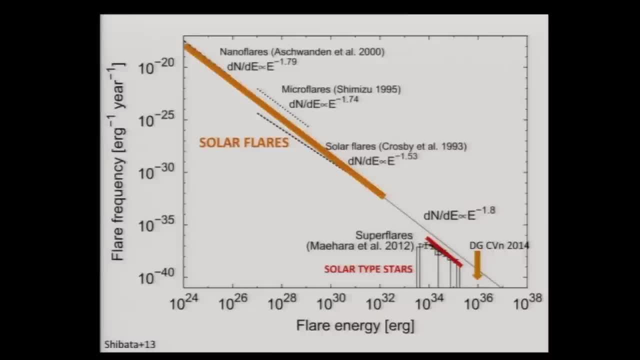 Well, or let's say, it would be 16th of July 2012,. would be known to all of you if the alignment had been different? So are solar flares the biggest things that happen on the sun. Well, this is just a technical plot. 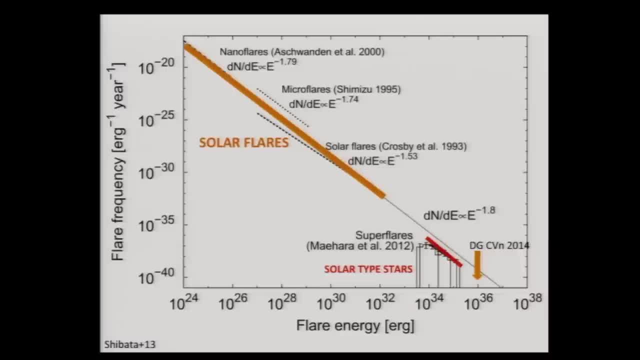 but this is the frequency at which flares occur versus their energy. And don't worry about the units, But what we've got, each of these ticks is a factor of 10.. So you know, this is 10 to the 24,, 10 to the 26.. 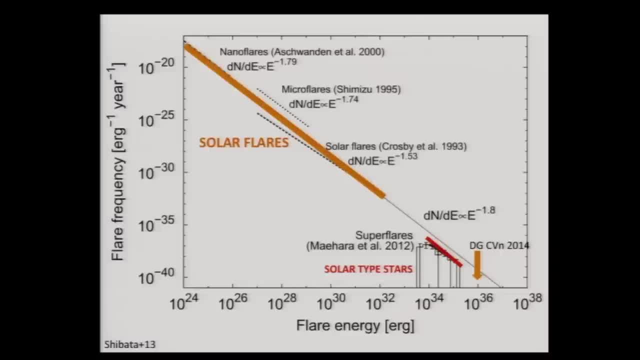 That's a factor of 100. That's a factor of 100. That's a factor of 100.. In order to plot anything- and I'm going to show you only a few plots, but I'm going to talk- I'm going to talk about big numbers. 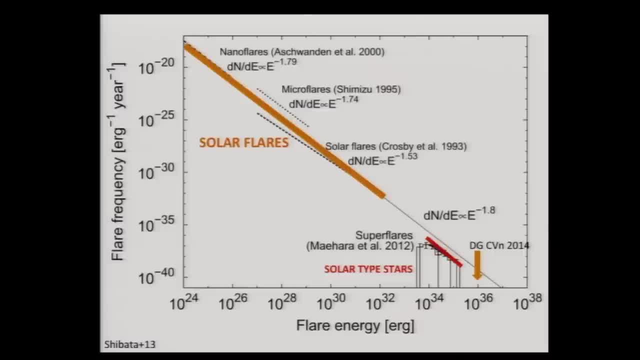 And the only way I can talk about big numbers in astronomy- because they are astronomically huge- is to talk about them in powers of 10.. So when I say 10 to the 20, that means a 1 followed by 20 noughts. 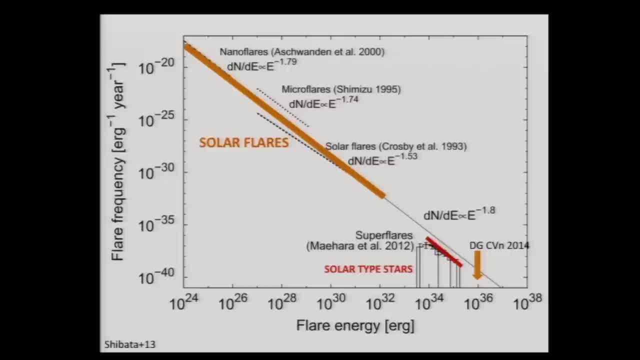 10 to the 40 is a 1, followed by 40 noughts. 10 to the 52 watts: we're going to get there. 10 to the 52 watts is a 1, followed by 52 zeros watts. 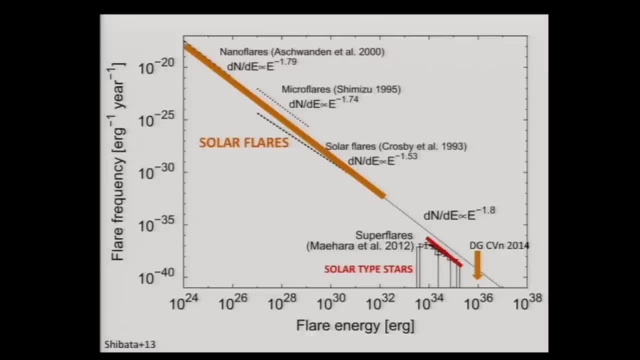 Well, here we're talking about 10 to the 32 ergs. This is the total energy in a flare. And you see, people have looked at the rate at which flares occur there. Do they also occur up here? Well, you can. 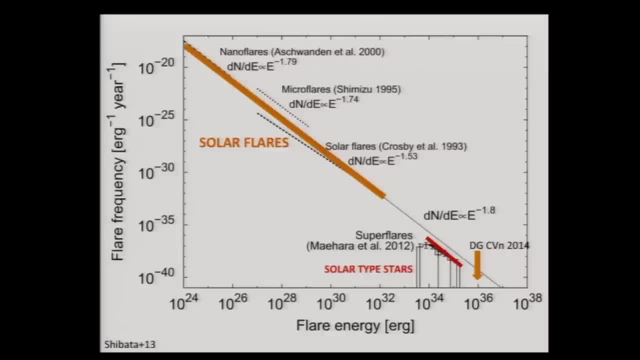 If you work it out, these flares up here, were they to occur, would occur once every 1,000 years or so. So we have to look at the sum for 1,000 years to see one of these super flares. 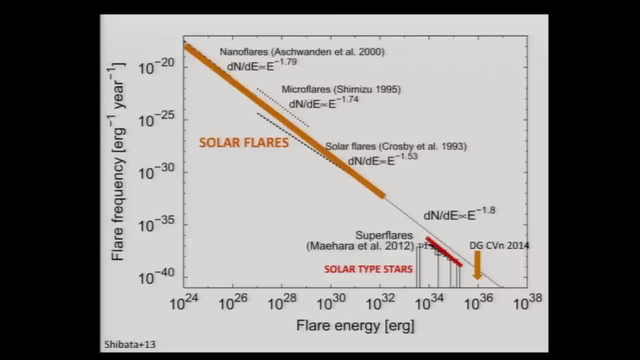 But another way to do it is to actually look at 1,000 stars like the Sun for a year, And that's what's been done with the Kepler satellite just staring at 1,000 solar-type stars, and they do see these flares, and it continues up there. 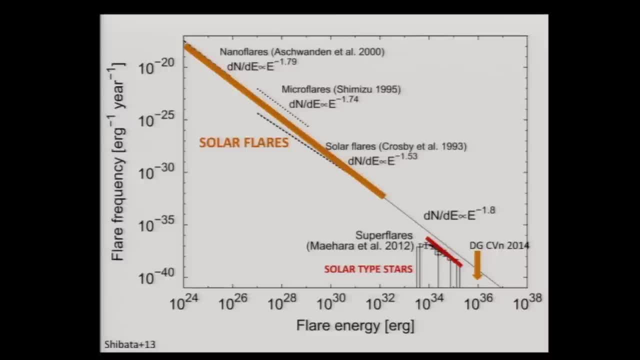 So we don't quite know where this ends and there's probably some physical limitation, but they can be extremely energetic. And this is just a dwarf star, unlike the Sun, It's smaller than the Sun: a small red dwarf star. Actually, it's smaller than the Sun: a small red dwarf star. 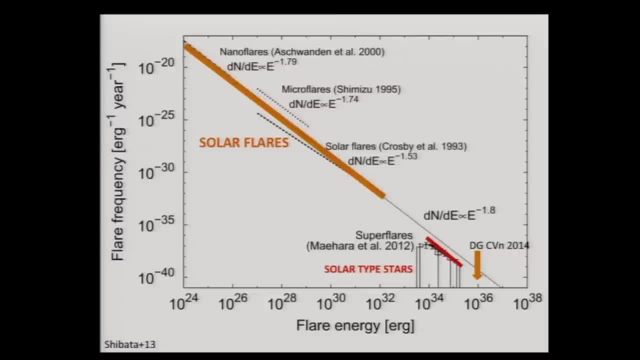 And you have a flare that big in 2014.. Now, I'm going to go on now with I'm doing the preliminaries. before we get into all the exciting details of all the powerful events in the Universe, I want to talk you through a little bit about what I 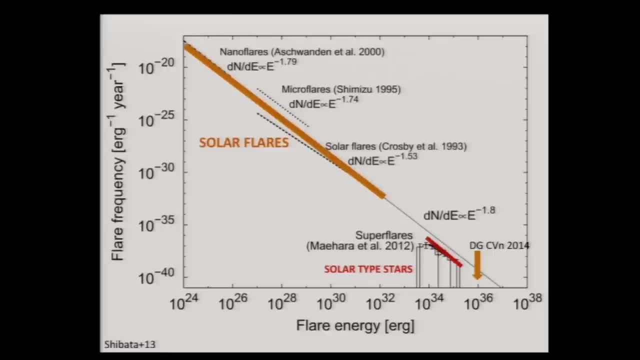 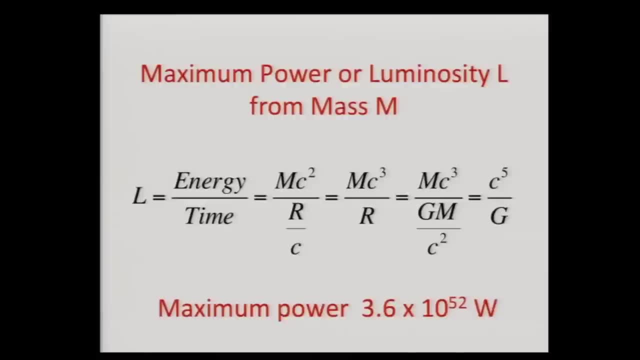 whathow big power can be? How muchhow large can you think about the maximum power? And I'm going to send you all out of the room because I'm going to give you an equation which everybody says one shouldn't do. 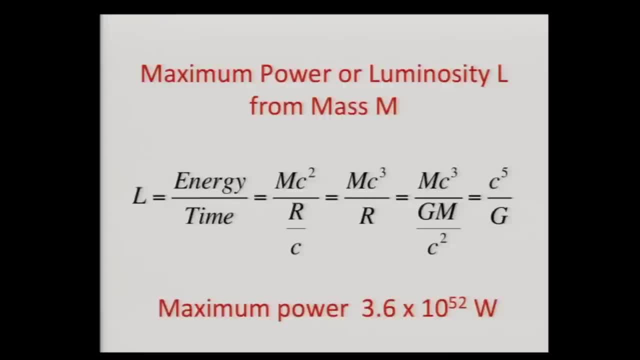 But this is a very simple equation. It's just what is the maximum power that you can get from an object of mass m, And so it's very simple. but if you've not seen it, it's very cute. at least in terms, I think it's cute. 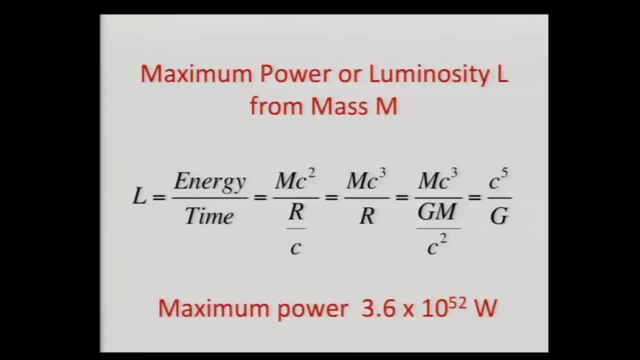 But this is the power of luminosity. It's defined as energy divided by time. You all know about light bulbs- 100-watt light bulbs or 15-watt light bulbs that you use, So that'sthat's a unit of power. 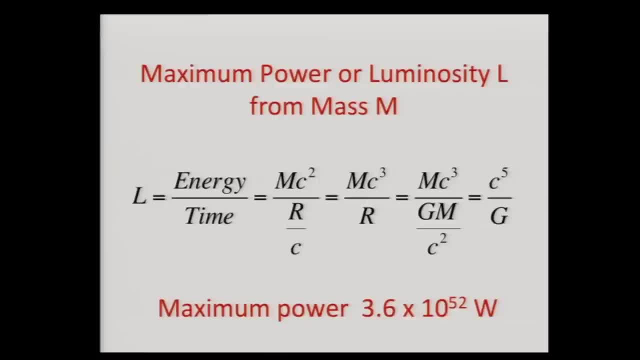 So it's energy divided by time. What's the maximum energy you can get from mass m? Einstein gave us the answer: It's mc squared, And I'm sure everybody in this room knows E equals mc squared. So there's energy equals mc squared. 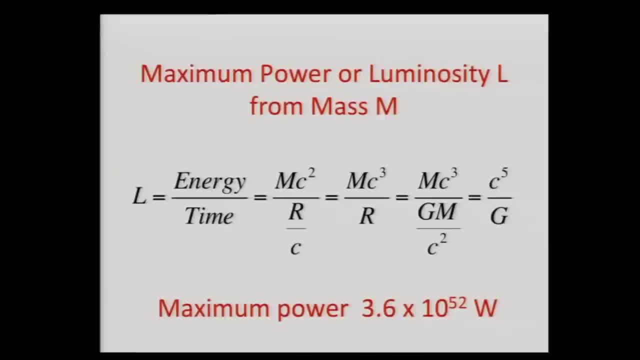 What's the shortest time that you can get it out on. It's what we call the light crossing time. It's how long light takes to cross the object, because the fastest you can remove the energy is at the speed of light And, of course, if you want to get a pulse from it, 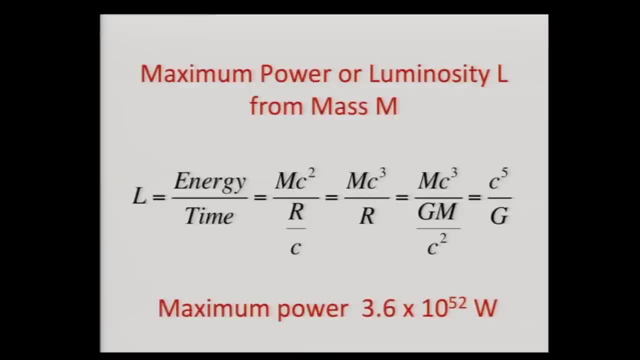 you've got to have the light from the back side and you've got to see the light from the front side and there's a time difference between the two. So that's r over c. Rearrange that We get mc cubed over r. 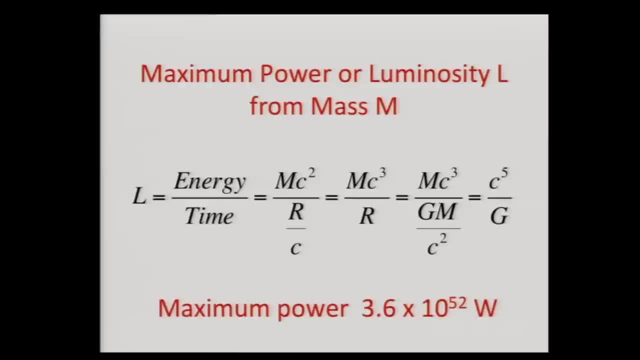 And then what's the smallest radius? it can be. What's the smallest radius a mass can be? It's a black hole. What's the side of a black hole? It's gm over c squared if it's spinning. Okay, So I now rearrange it. 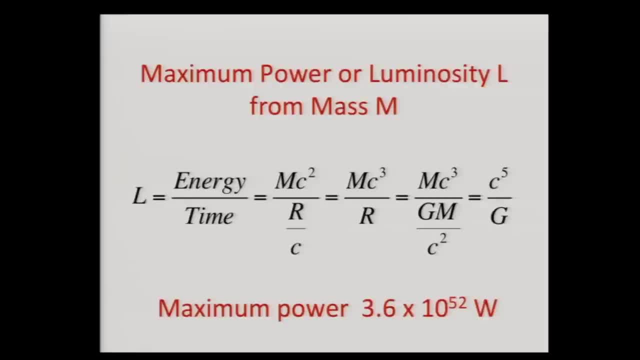 and the m cancels and I get c to the fifth over g, And that's the maximum power that you can generate from an object. c to the fifth. c is the speed of light, which is a very large number. g is the gravitational constant. 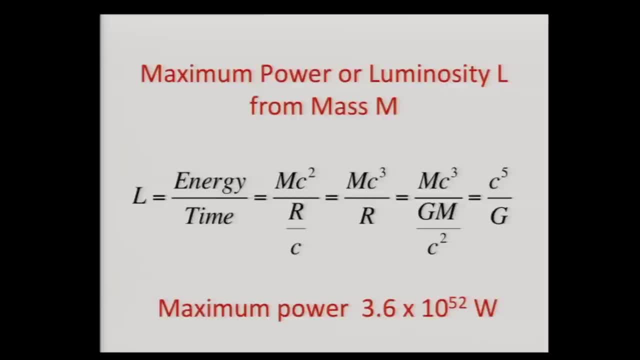 Gravity is not a very strong force. It's a small number, A very large number divided by a small number, It turns out to be 3.6 times 10 to the 52 watts. Okay, That sounds utterly ridiculous, Utterly, utterly ridiculous. But it's not completely ridiculous. It turns out to be. the maximum power is 10 to the 26 times the luminosity of the sun. Okay, Now it turns out that in our galaxy there's 100 billion stars and there's about 100 billion galaxies in the universe. 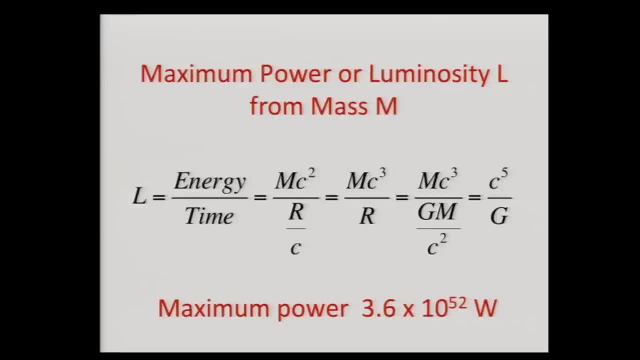 So if I take the power of all the stars in the universe and then add them all together, that's going to be 100 billion times 100 billion. That's 10 to the 22. So this maximum power is 10,000 times bigger. 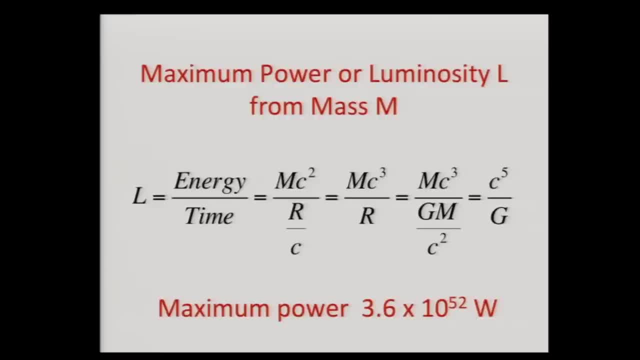 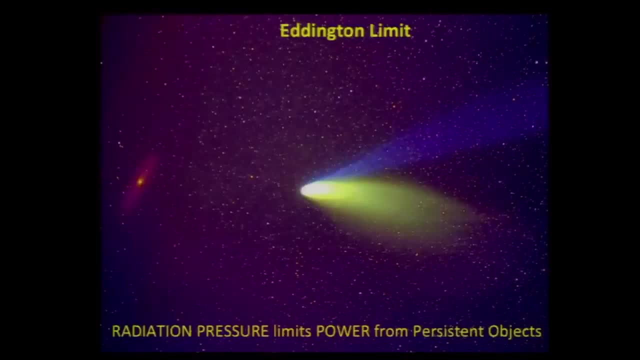 than all the luminosity of all the stars and all the galaxies in the universe, But this is my maximum. Another limitation on power in the universe comes from what we call the Eddington limit. 100 years ago, one of the most prominent astronomers 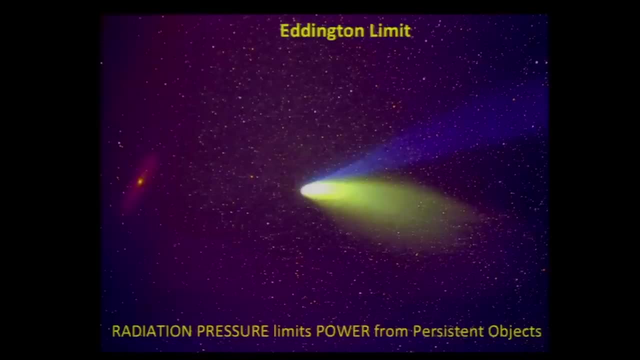 in the last century was Professor Arthur Eddington, a plumian professor here in the University of Cambridge. This is named after Eddington. He pointed out there's a limitation to how powerful something can be, because power because radiation, and if you've got something radiating, 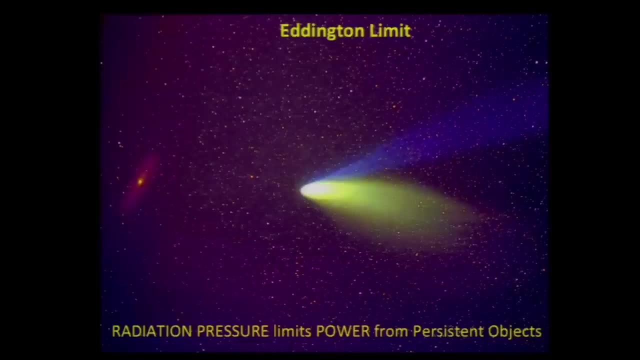 radiation exerts a pressure. We've all seen pictures of this. This is Comet Hale-Bopp that the older members of the audience will remember from about 20 years ago. This is its tail, or tails. This is the so-called iron tail. 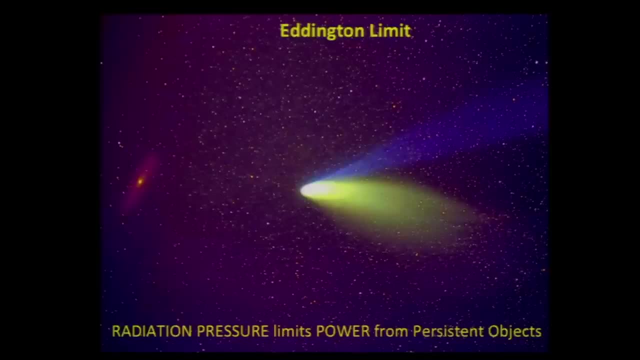 which I'm not interested in. This is the dust tail. Basically, the sun is way over on the left here. The radiation from the sun is blowing the tail away from the comet. This is very visible, visibly demonstrating that radiation pressure can push things. 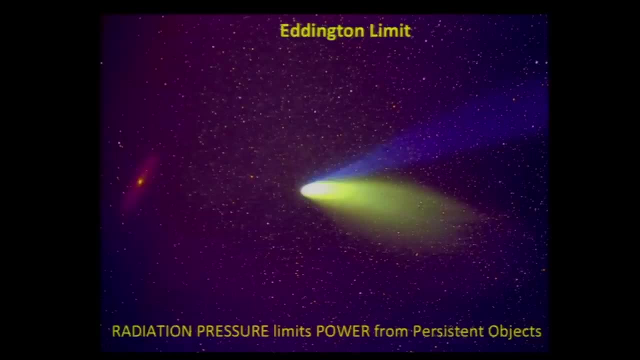 Once you can get, there's a limit to how powerful something can be in terms of radiation. when the radiation is so powerful, it blows the thing to pieces. If radiation outwards is equal to the gravitational pull inwards or is greater than the gravitational pull inwards, 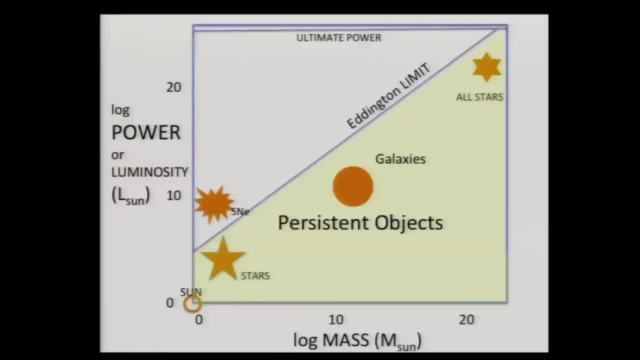 then obviously the object will blow itself to pieces. That's called the Eddington limit. when you're there- And this is a plot showing power up there versus mass of objects in the universe, And I'm again using this logarithmic unit, so zero means one, it's 10 to the nought. 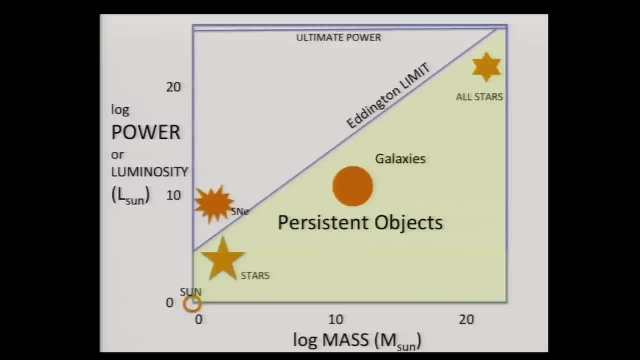 That's 10 billion and so on. The sun's down this bottom part, This is the Eddington limit. There's the ultimate or maximum power. It turns out. stars are down here, galaxies up here and all stars in the universe up there. 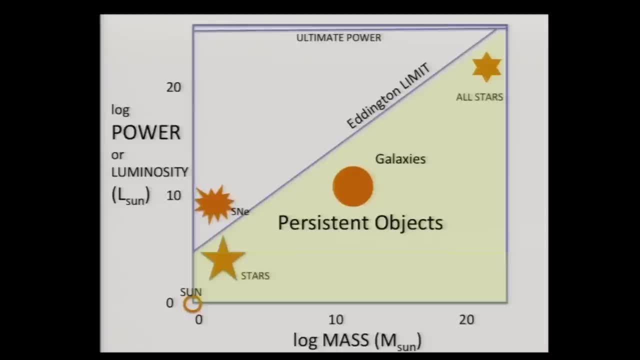 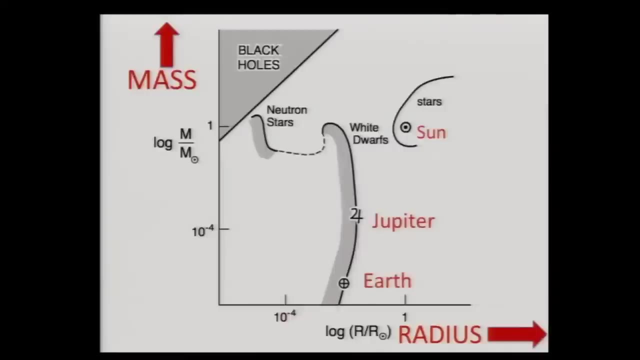 Now we're going to start thinking about exploding stars. So, in order to talk about exploding stars, I want you to think about what stars are and what's going on in stars, And I'm going to do this in terms of this mass-radius plot. 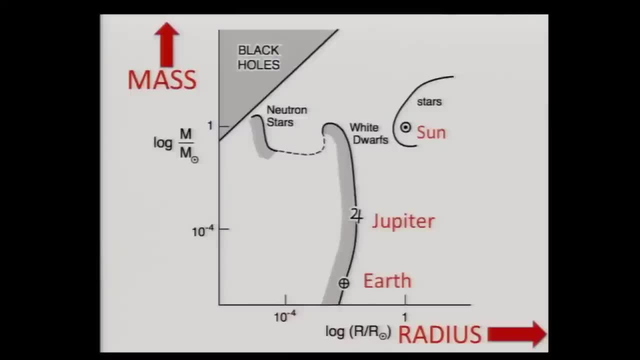 Don't get too worried about it. but this is mass and radius, And astronomers like plotting everything in the universe all on one plot, And so we've got logarithmic units again, okay, And stars are over here, with the sun there on one of these units. 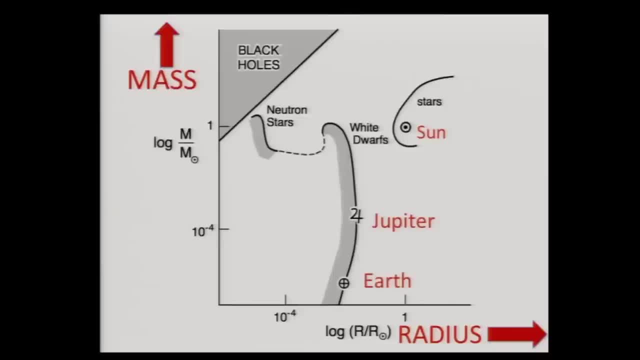 And these are black holes, These are planets, And when you get up here, this sort of turns around and goes down to these objects called white dwarfs. Incidentally, white dwarfs were first understood by the master's grandfather, Ray Fowler. 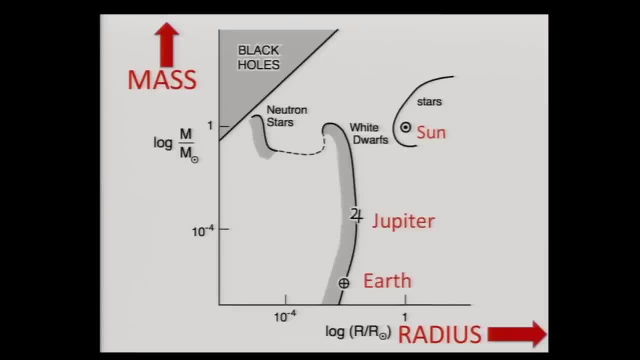 This turning point here is known as the Chandrasekhar mass. There's a maximum mass to a white dwarf and it's up here. Down here there's another point at which things you can have stable objects. This defines where stable objects occur. 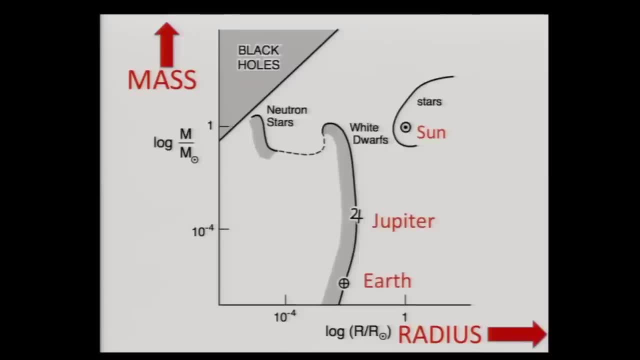 White dwarfs, planets, that's Jupiter, that's the Earth, and neutron stars are over here just before you get to black holes. There's nothing that is made that what we would see as a solid object above in this part of the diagram. 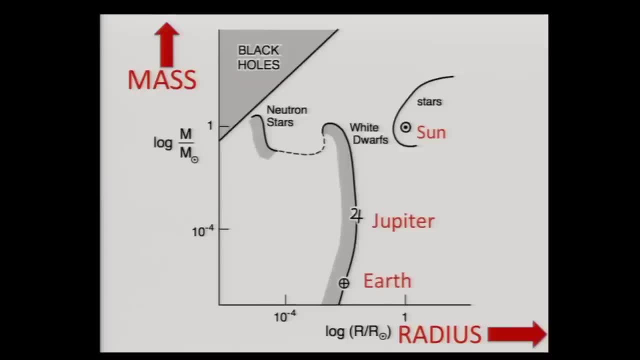 above the white dwarfs and neutron stars. You then have the black holes, which are objects which I'll get to later, where they've collapsed in on themselves. Stars are over here and they're held out over there because they have nuclear reactions in their cores. 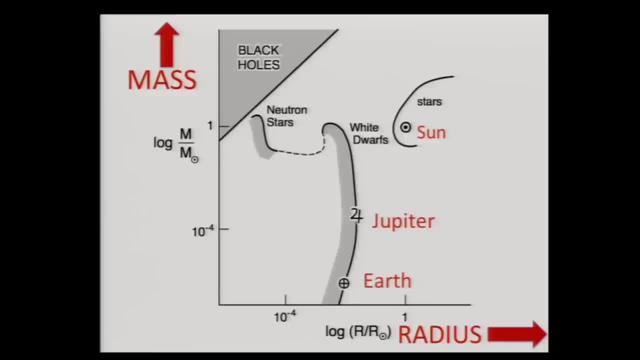 which have generated pressure in them which balances gravity. And so in the Sun we've got the outward pressure, thermal pressure, due to the creation of all the helium in the core of the Sun from the hydrogen there, nuclear fusion That's actually inflating the Sun. 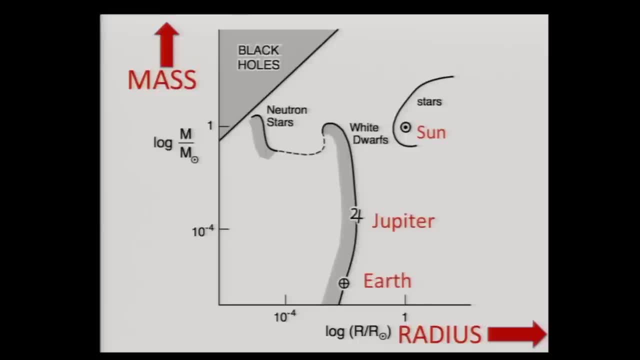 keeping it in balance, And the Sun's been like that for the last five billion years. But eventually you end up using up all the hydrogen in the core of the star and it then collapses. the core collapses and starts burning helium to carbon. 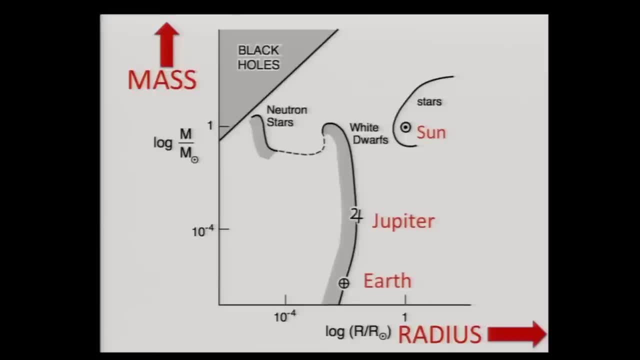 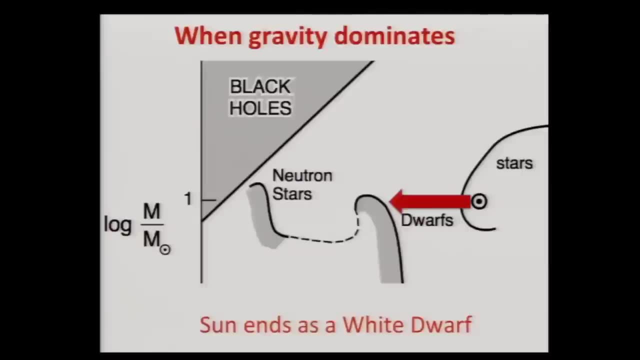 and eventually the Sun will die as a carbon-oxygen white dwarf. So there, I've represented this by an arrow. The Sun will end its life as a white dwarf. It will throw some of its outer envelope away, but it goes like that. 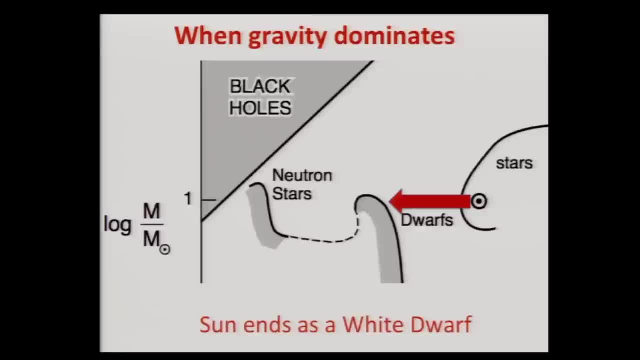 and it will get stuck on that bit there. But if you're a more massive star somewhere up here, then what happens is the only thing the core of a star can do is collapse all the way down and form the black hole. There's nothing else for it to do. 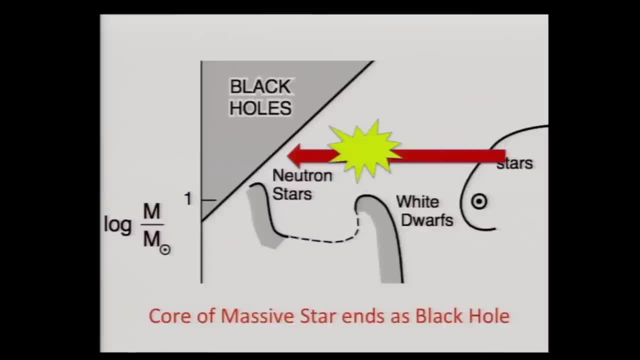 and in doing so, because the material of the star, the core of the star, collapses inwards. there's nothing to stop it collapsing down and there's an enormous amount of energy being released, And it does it very quickly. It collapses down in a matter of. 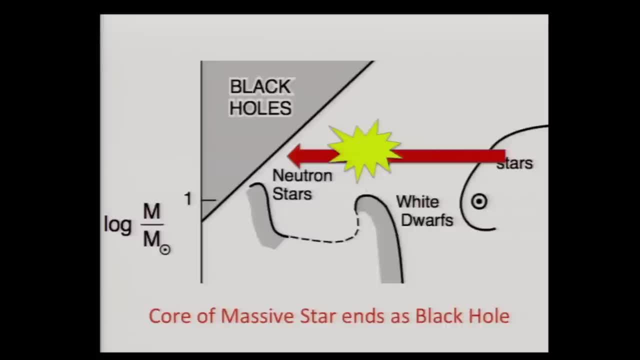 minutes and seconds, enormous amount of energy, vast explosion. That's what we call a supernova explosion. There is just one other one of these, and that is: if you're a medium-sized star, then you can actually go across here. 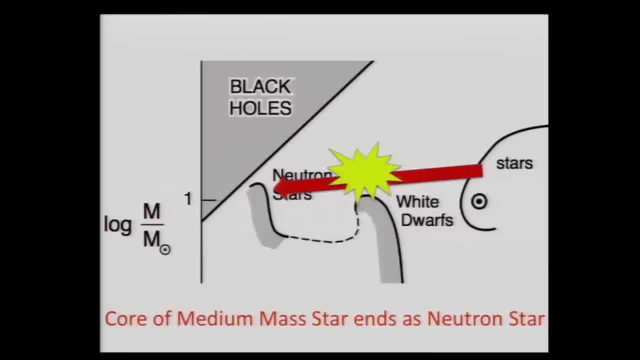 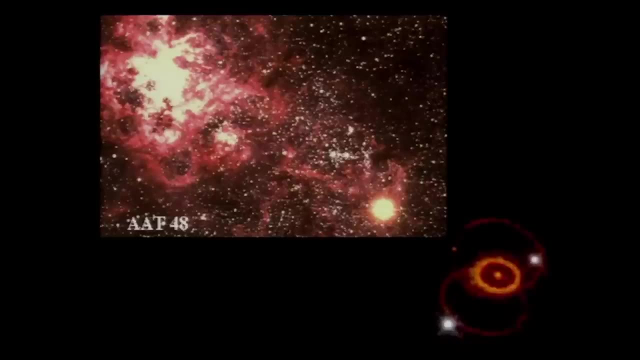 throwing off some of the mass on the way and you can end up as a neutron star. So I'm now going to introduce you to supernovae and neutron stars, starting off with the only supernova, That's, the supernova explosion, that the star exploded. 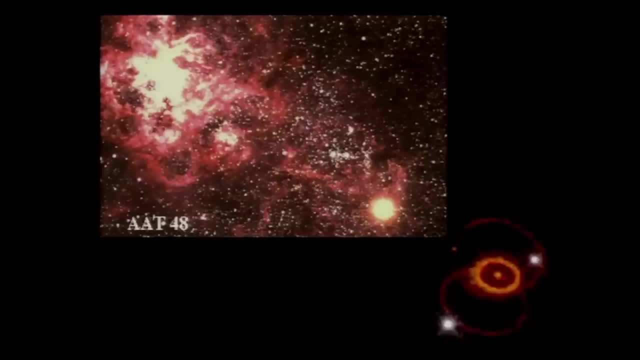 That's what it looked like beforehand. It's this thing in the middle. This star exploded in 1987, in February, in the nearby galaxy called the Large Magellanic Cloud. It's a satellite galaxy of our own. This nebula is a nebula of gas. 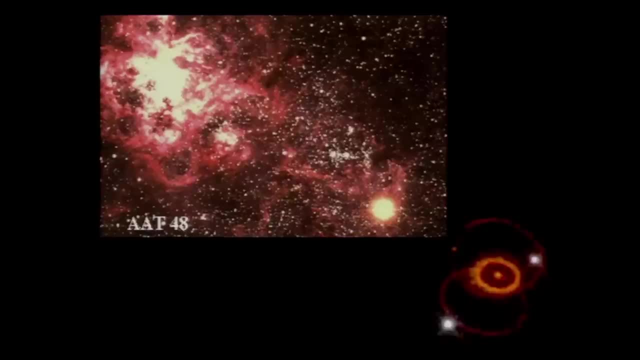 and you can see it in the light of hydrogen. there It's called the Tarantula Nebula because it looks a bit like a squash spider. Anyway, this thing was extremely bright and visible to the naked eye. It's the last one that's been visible. 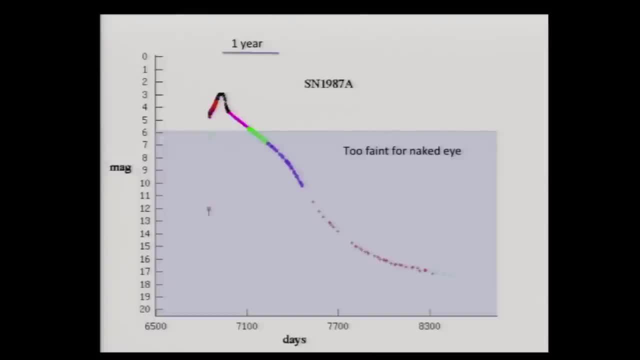 to the naked eye and this is just a plot of its brightness versus time. That's a year and you can see the thing actually was not observed down there and then suddenly, very quickly, it brightened up and made this brightness and dropped down like that. 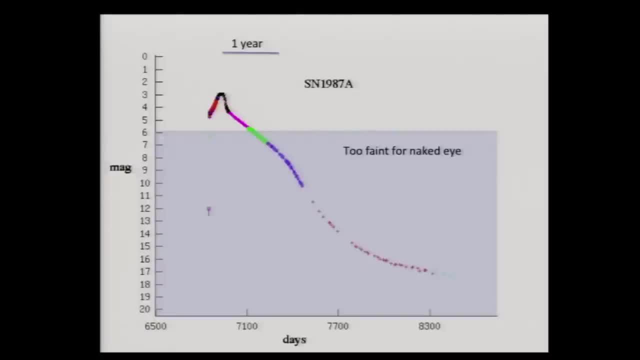 and when it's below this level it's too faint for the human eye. I actually was observing at the Anglo-Australian table a telescope in late 87 and saw this supernova through binoculars. I didn't come early enough to see it with the naked eye. 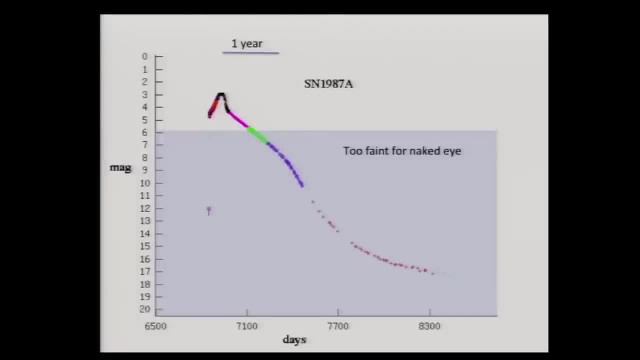 so I've never seen a naked-eye supernova. This part of the curve in this plot which is straight like this, is due to radioactive decay. When you get a supernova explosion, the temperatures are extremely high and they go and in the ejector. 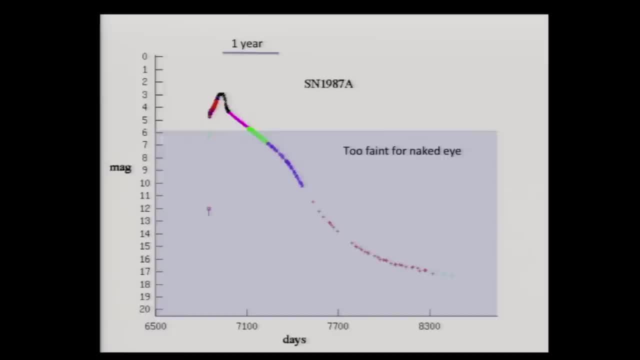 as it's all thrown out. there are lots of neutrons and that leads to many of the heavy elements, the elements greater than hydrogen and helium that we have around us- Most of us- I don't know if you know this, but the dominant element in your body. 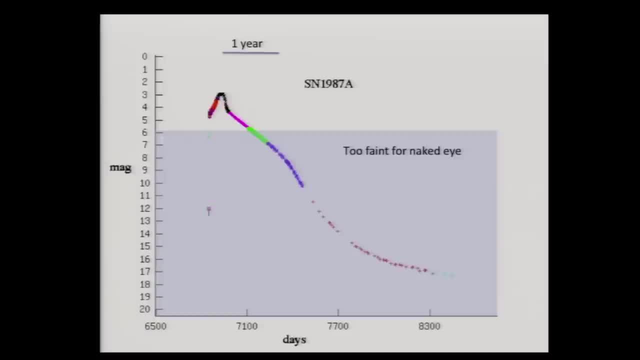 by mass. if I was to go around and ask you, most people would say carbon. Actually, you're wrong, it's oxygen. Now, if I was to get a stone and do the same, what's the dominant element in a stone? 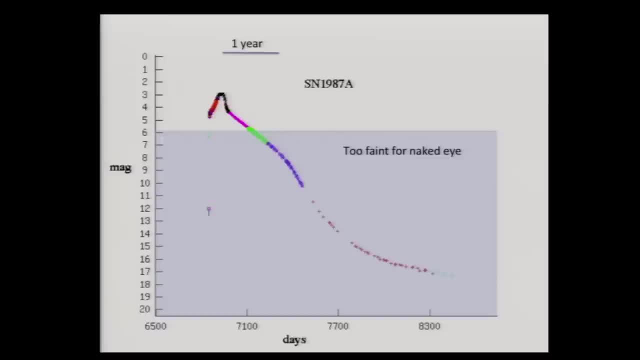 It's mostly oxygen. The geologist in the front there is nodding in approval, so I think I've got that right. Anyway, so oxygen, But in our bodies. most of the oxygen in our bodies was formed in one of these supernova explosions. 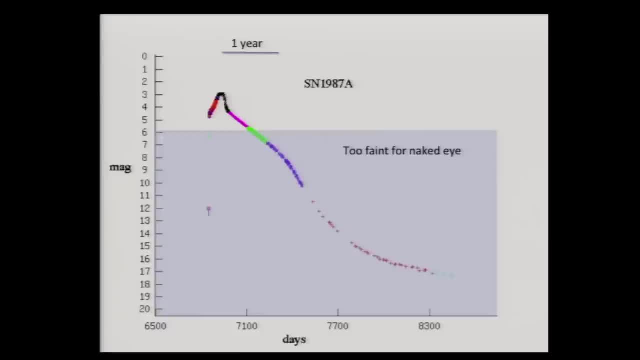 So you know all of this. we are star dust, et cetera, et cetera, but that's where most of the oxygen comes from, And about half of the iron in your blood comes from what's called a core collapse supernova. 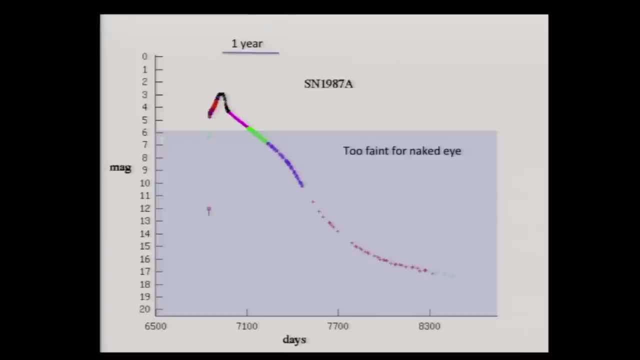 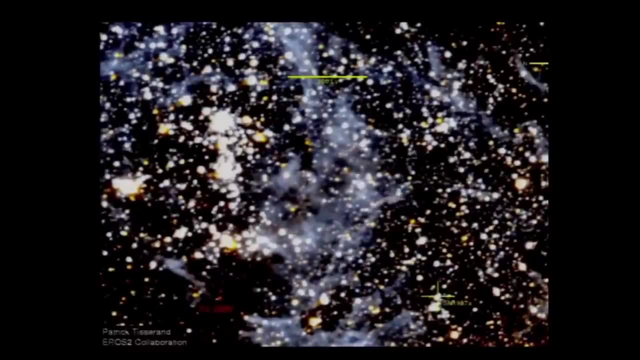 These are the supernovae where the core of the star has collapsed, as I've shown you- And this is a wonderful image- is made by the EROS2 Collaboration and this is speeded up images of the region. The supernova occurred here. 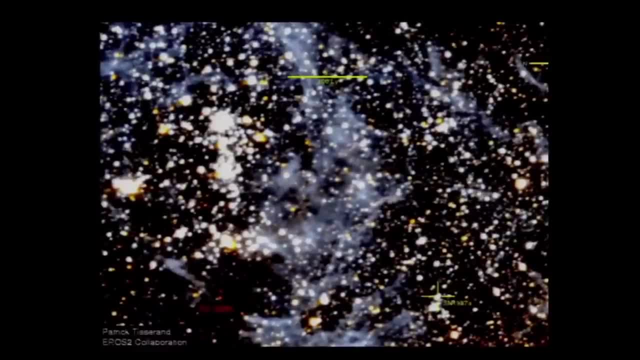 This is speeded up images over the subsequent, over the seven years from 1996 to 2002.. Can you see these ripples going outwards? These are just where the light from the supernova is now reflecting off of the star. 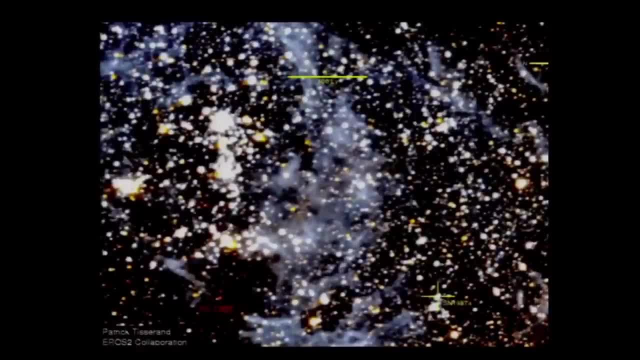 So these ripples are reflecting off the nebulae here. These nebulae have got dust in and if you shine a bright light on dust it shows up and it can reflect and so you're seeing the reflections and you can see them going across here. 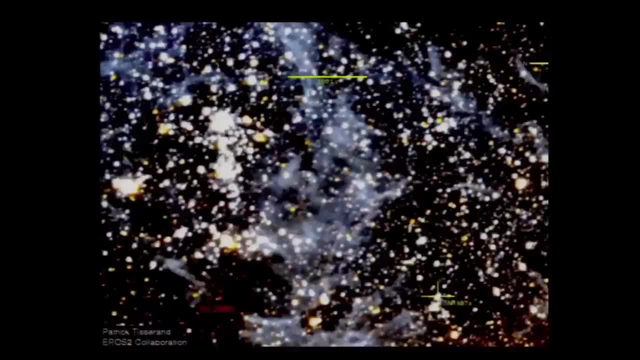 so they circle around there. So in a way, this means you can look back in time. if you see that, and you can actually go and measure its colour and so forth, you're actually looking at a reflection of your supernova. 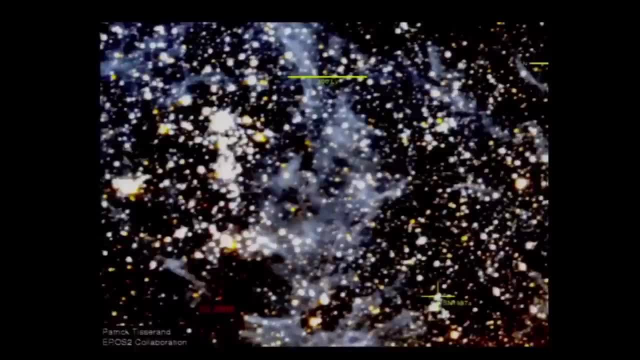 So when you're out there in a clear night and you shine a torch, around that torch light goes out into space and may reflect off dust grains and if your torch was really powerful, you can see it back again. But these you can see. 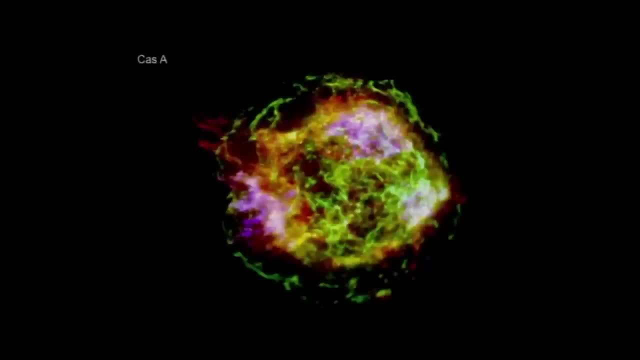 This is another core collapse supernova in our own galaxy, in the constellation of Cassiopeia, and this occurred in the 17th century and it's not clear that anybody saw it. There's still a squabble about whether anybody saw the flash from it. 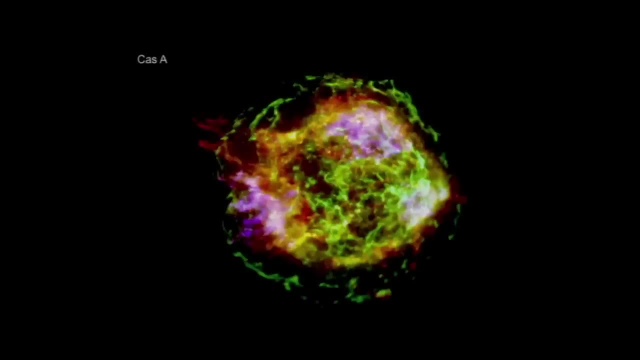 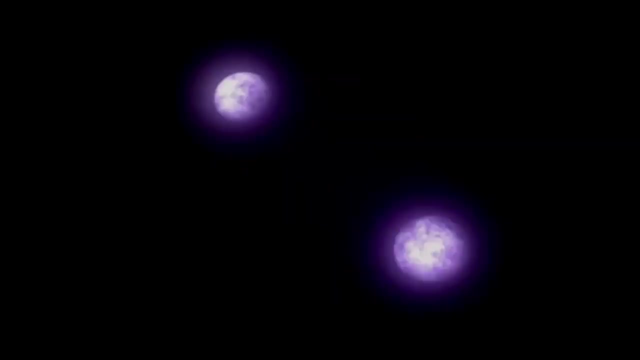 but you can see the outer shock wave as it's propagating out into the gas between the stars and you can see the inside of it there. Now there's another class of supernovae I just wanted to mention, because I'll be talking about mergers of binaries again. 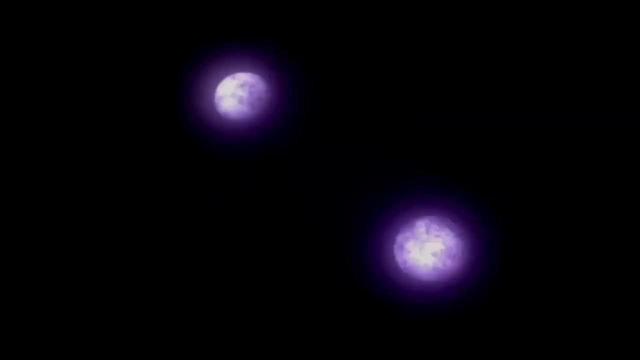 later in the talk- and these are white dwarfs. I said how the Sun is going to end its life as a white dwarf. Now, our Sun is unusual in a way because it's a single lone star. Most stars in the galaxy. 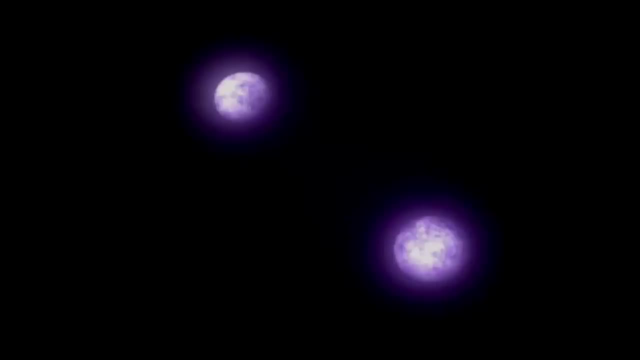 more than half of stars in the galaxy are multiple stars, meaning there's not just one star, there's several stars And sometimes there are two stars which are close together and both of them can evolve and become white dwarfs and they can be driven together. 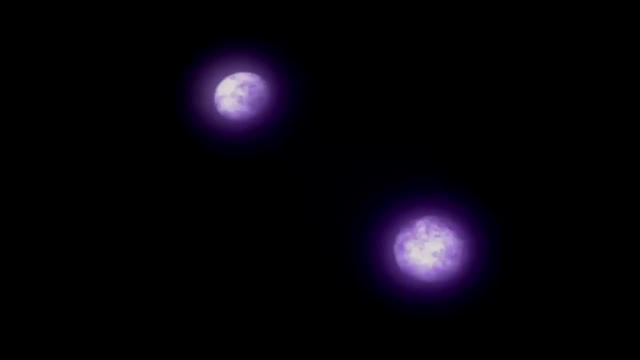 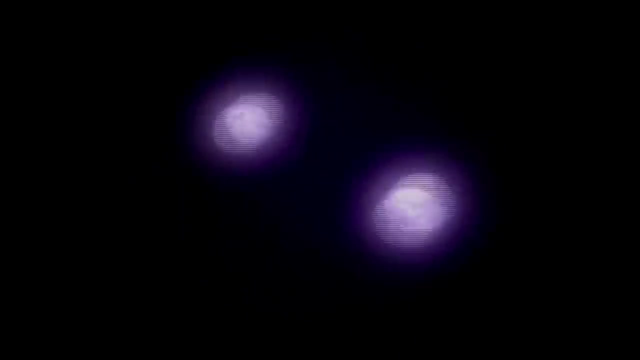 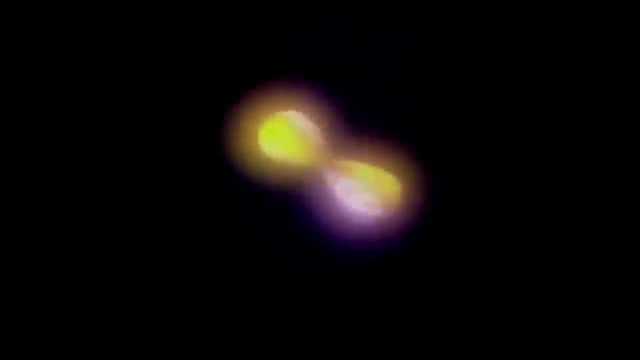 by the radiation, of by gravitational radiation, which is something I'll get to near the end of the lecture- And they can spiral together like this and when they do that, it leads to a giant thermonuclear explosion. where the brightness when it goes bang. 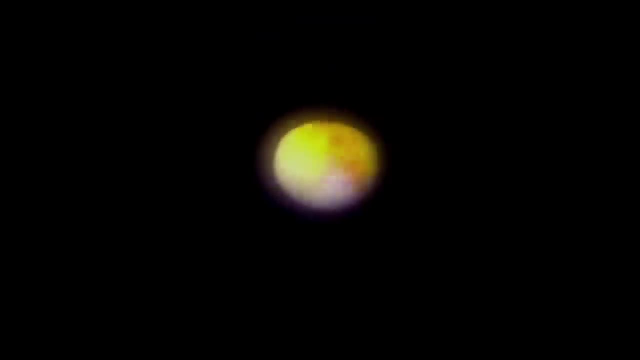 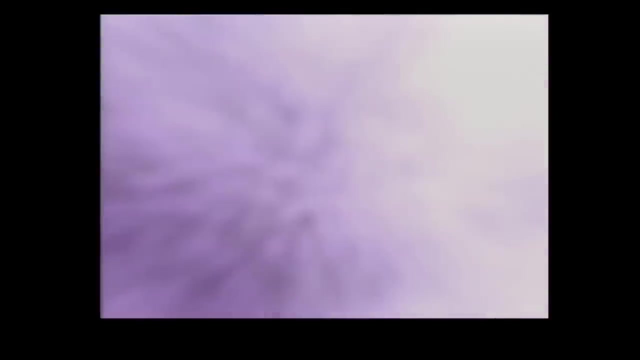 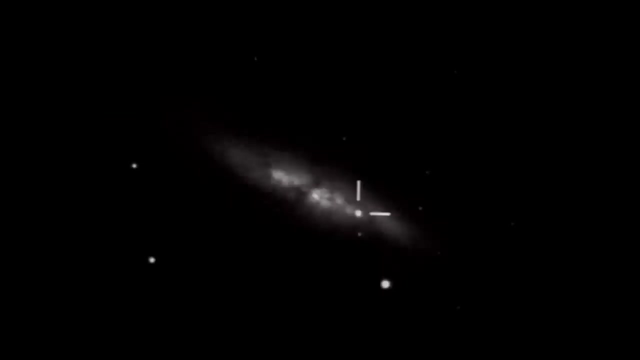 is about a billion times as bright as the Sun. That's its power, not how bright it appears to us, but is a billion times the power from the Sun. And there is a nearby galaxy, M82, with before and after when a supernova occurred back in 2012. 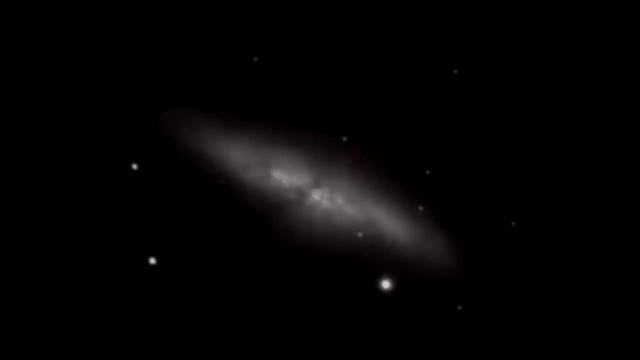 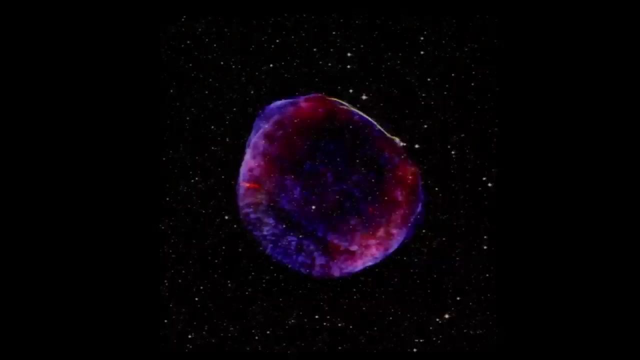 in that galaxy And that was this kind of merger of white dwarf supernova And those supernovae mostly leave iron behind And the other half of the iron in your blood comes from that kind of supernova. Now, the brightest flash that's been recorded 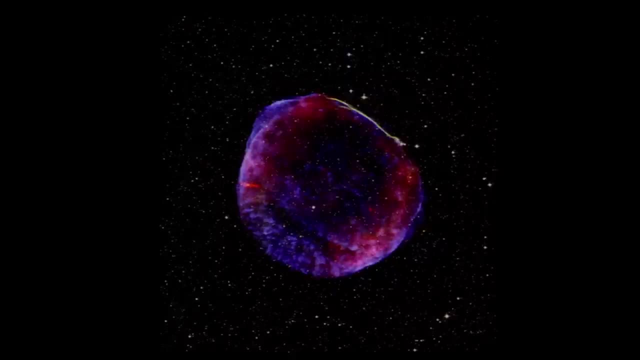 by anybody. flash to the eye occurred at the generation of this supernova remnant. This is the remnant of a supernova that occurred in 1006.. And it was seen the flash. the supernova explosion was actually seen by Korean, Chinese. 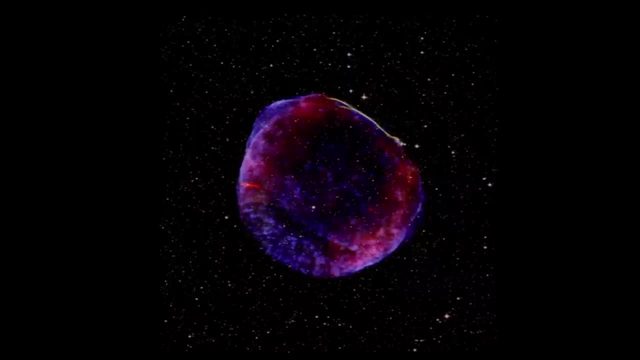 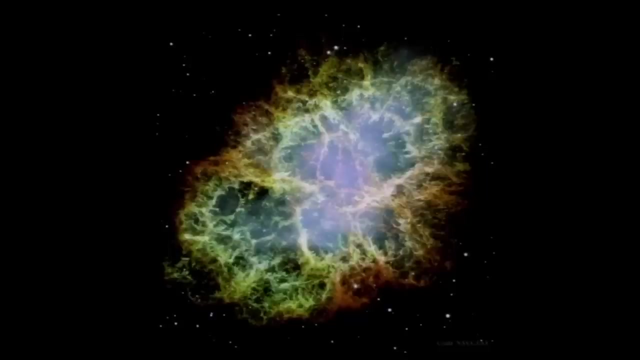 and other astronomers and recorded, And that's where it where it is now. This is the remnant of a poor, collapsed supernova and it's called the Crab Nebula because Herschel thought it looked a bit like a crab. 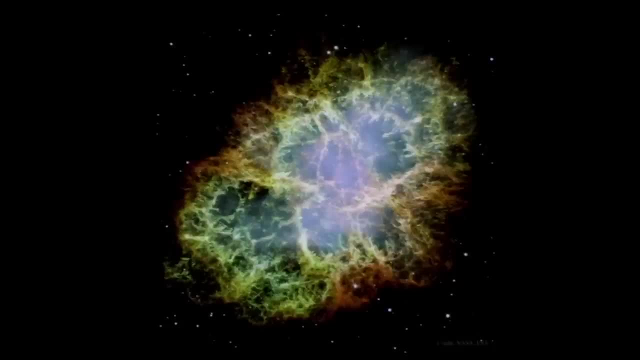 but I can't see that myself. But it's a very strange object and this is the remnant of the supernova that occurred in 1054 AD. This is in the constellation of Taurus and when it was going off it would have been easily visible in the daytime. 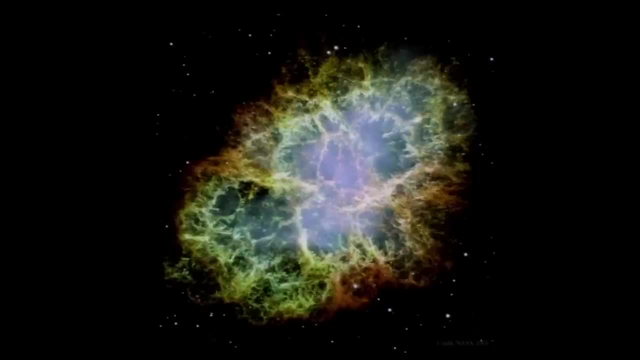 There are absolutely no records from England. Maybe everybody was going around looking at the ground all the time, or maybe it was cloudy all the time, But anyway it was not seen. but it was again recorded by Asian astronomers And I think it was also recorded. 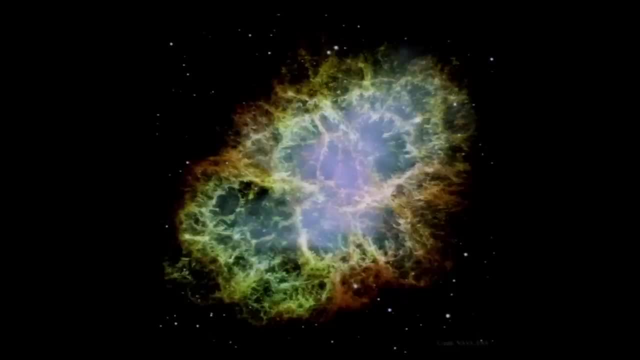 by some monks in Switzerland. Now this supernova of AD 1054, which is only 48 years after the 1006 one, so it was possible for somebody to have seen two supernovae in their lifetime- This one has left behind a neutron star. 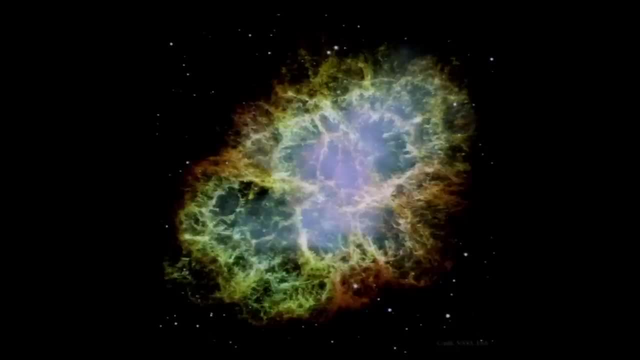 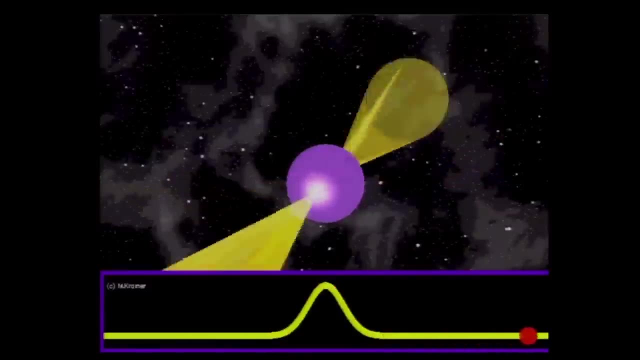 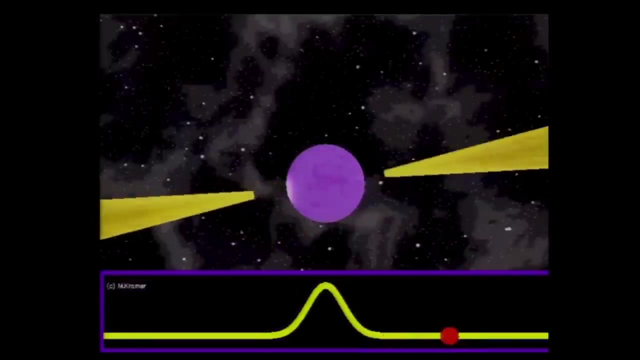 And it was long thought that there's something funny about one of the stars in the center of it, And it wasn't until 1968 it was realized it was a pulsar. A pulsar is essentially this collapsed object at the center. 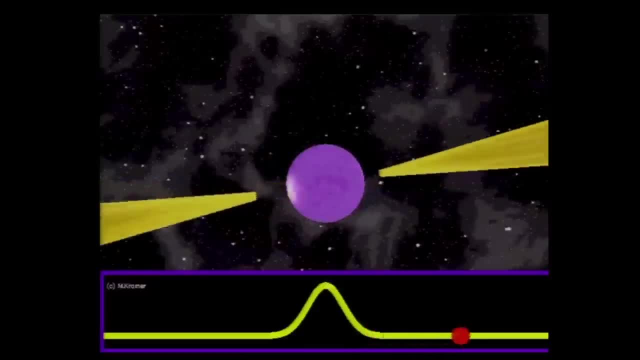 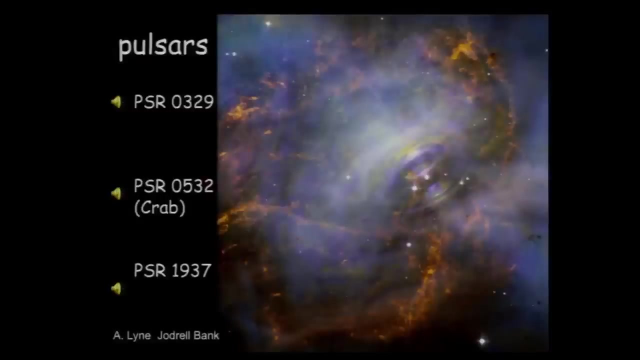 only it's highly magnetized And as it spins round it flashes at us, And it flashes in all wave bands, from the radio through to the gamma-ray band, Gamma-ray bands. And here is This, is the pulsar, that thing there. 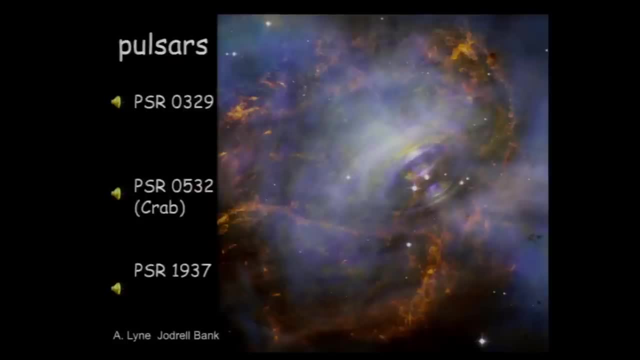 And you can see that it's done something to the nebula around it, And that's because it's a highly magnetized neutron star. The neutron star has got a size of a radius of only 10 kilometers, So it's about as big as London. 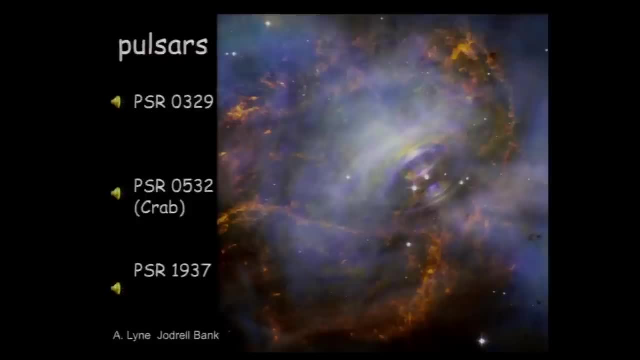 It's rotating at 30 times a second, So it's going spinning pretty fast. It's got a magnetic field of a million million Gauss, or million billion times the magnetic field in this room. I'm now going to just play you what it sounds like. 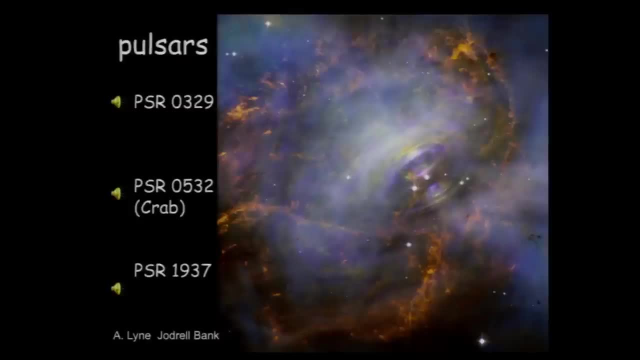 That's 30 times a second. There are pulsars out there that are much faster, And I'm now going to remind you of your last visit to the dentist, Because this one is 600 times a second. You ready, I thought you'd like it. 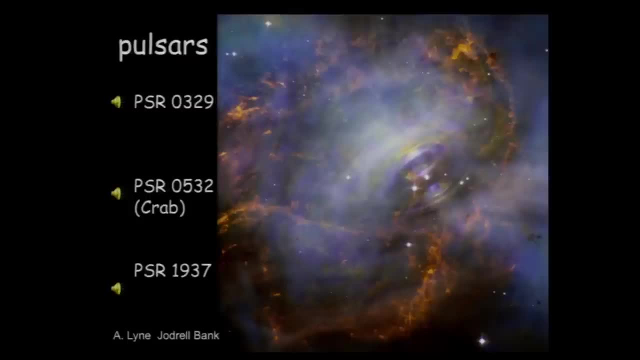 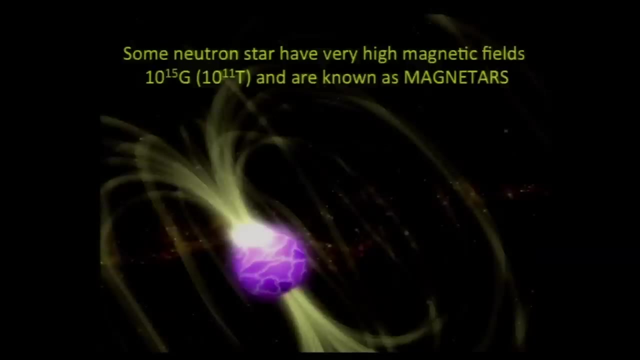 So these are pulsars. Pulsars are the dead remnants of explosions, Exploded massive or medium-mass stars, And they're quite common in our galaxy. There are also kinds of neutron stars which have got extremely high magnetic fields. There are a thousand times. 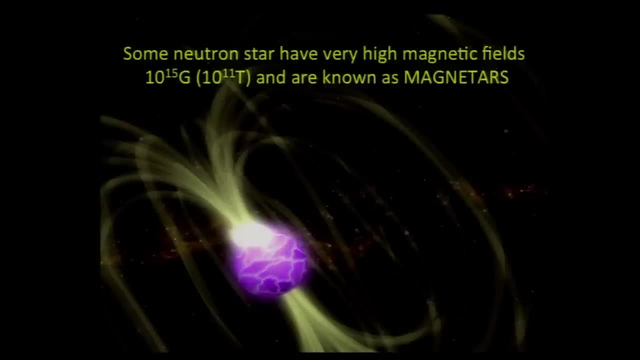 higher than the one I just talked about. So there are a thousand million million times the magnetic field in this room. These extremely high magnetic fields mean that the crust of the star is incredibly stressed by the magnetic field And sometimes it cracks and breaks. 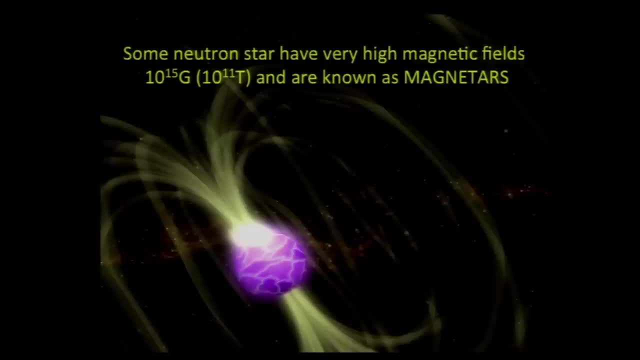 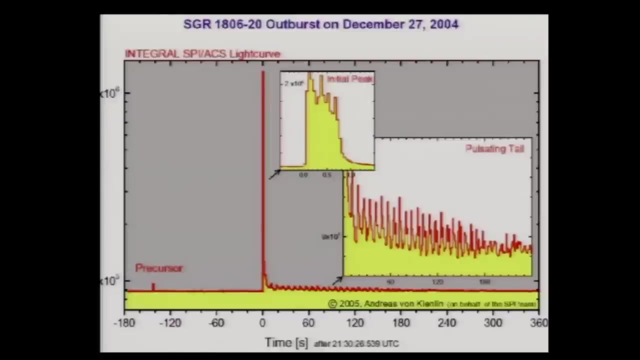 And that leads to an intense flash of radiation, Most of it in the gamma-ray and hard X-ray bounds, And these objects are known as magnetars And this is the most intense flash that's ever been recorded, Most powerful flash. Well, 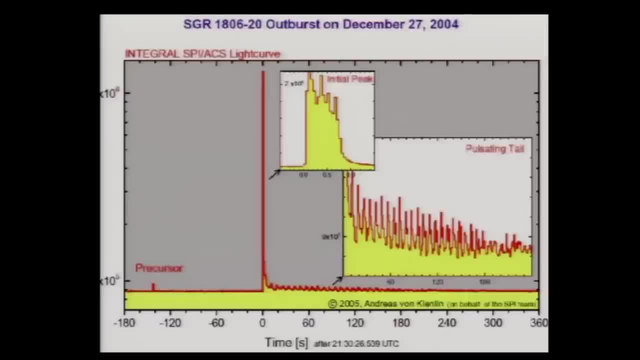 it's the brightest flash, this one, And it occurred in 2004, in December, And this is just a time where that is a minute, another minute and so forth, And this is this incredibly intense flash And indeed in this instrument, 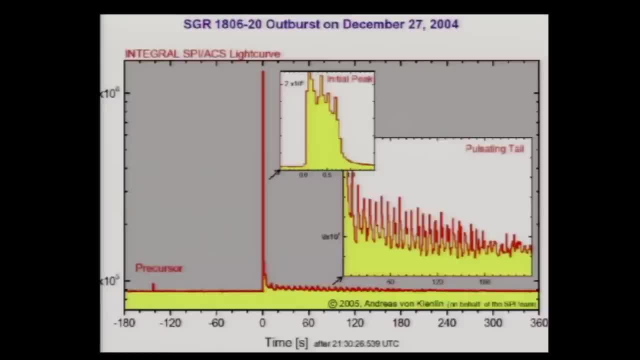 it's totally saturated, And the only way they got good measurements of the brightness of this flash is by looking at gamma rays reflected off the Moon, And the Moon is not very shiny at all in gamma rays. In fact, it mainly absorbs them. 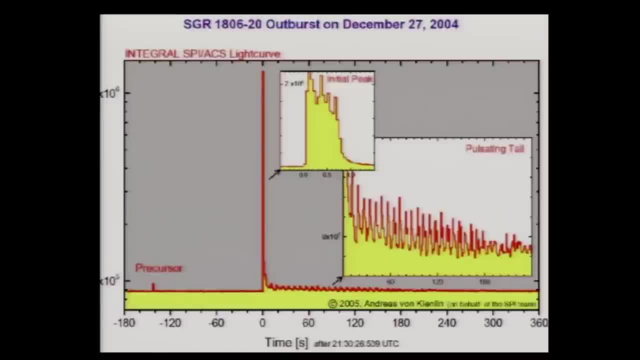 It's a very intense flash And, as they say, it's the brightest flash that's been seen, And it comes from the other side of the galaxy And, as it decayed, it showed a pulsation. Okay, can you see the pulsations there? Every five seconds. That's due to its spinning. These flashes of gamma rays hitting the Earth's atmosphere ionize the atmosphere and indeed the oscillations could be picked up by radio measurements of the outer atmosphere, outer ionosphere of the Earth. 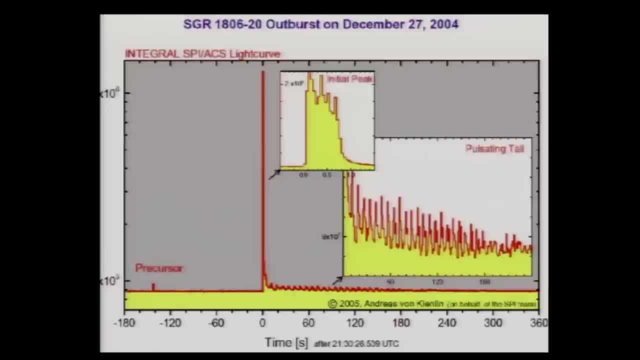 So it set the Earth's outer atmosphere ringing like a bell. So something the size of London, the other side of the galaxy, goes bang and causes our atmosphere to ring like a bell. Okay, Now let's talk about gamma ray astrology. We should all do. 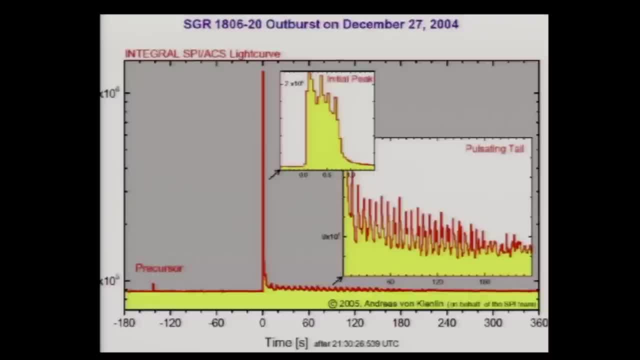 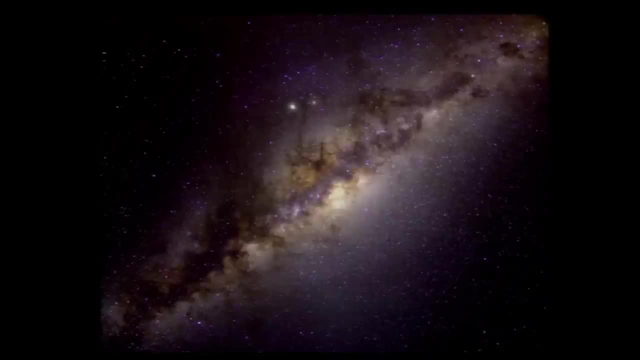 gamma ray astrology, because these are the things that really do affect you. I'm absolutely, 100% convinced that the position of Saturn in the solar system of the day you were born has got no influence, any influence whatsoever, on you personally. I'm now going to turn. 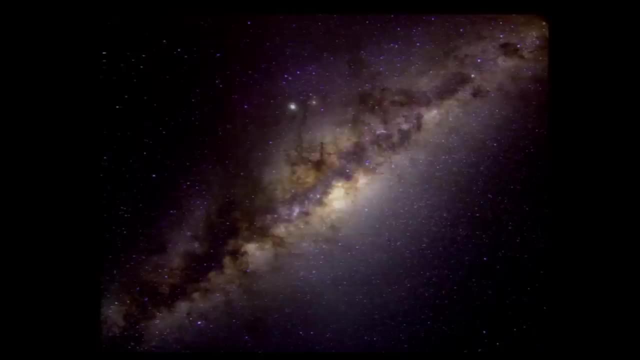 to some evidence for the one in the center of our galaxy. These are all stars in our galaxy. This is the Milky Way. The dark bands are due to dust and the center of our galaxy is there. Everything in our galaxy rotates around the center. 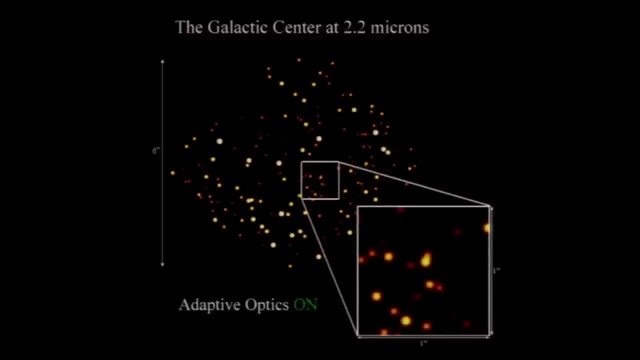 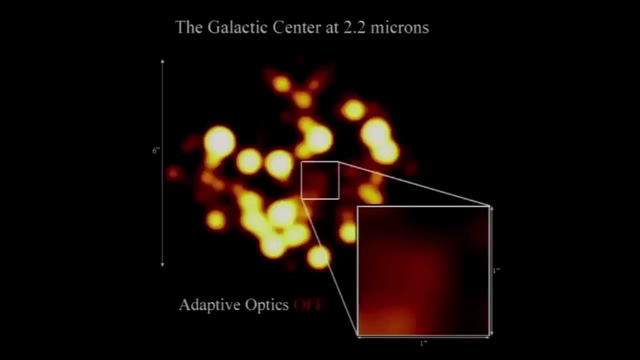 at about 230 kilometers per second. If you go in and look at the cluster of stars at the center of our galaxy, particularly in the infrared band, where the center is just there, you need to remove the flickering, the deviations caused by. 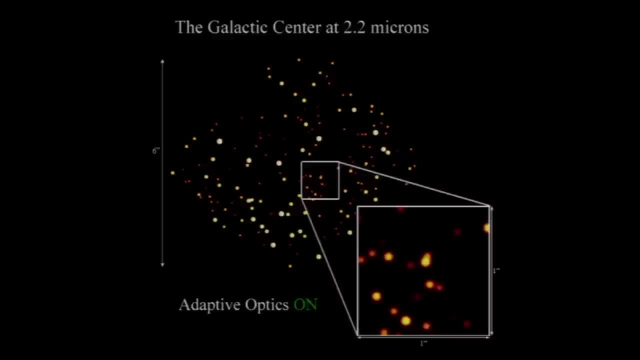 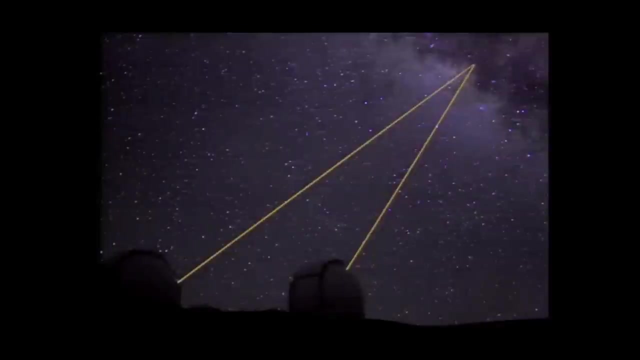 the Earth's atmosphere in order to do this. This is called adaptive optics, where basically you have you create a star in the outer atmosphere of the Earth and you sharpen your images up on that and as they switch it on, you can see the image gets. 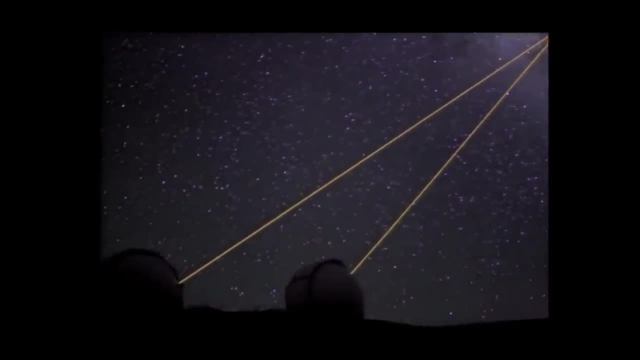 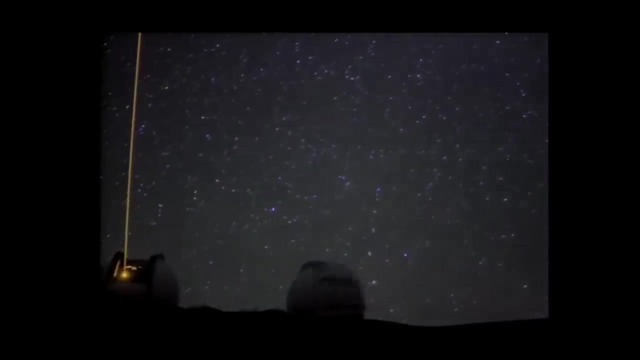 so that you can actually see the motion of the stars, You make the artificial star using these laser beams. These are the Keck telescopes on Hawaii shining laser beams at the galactic center. The galactic center is 25,000 light years away. 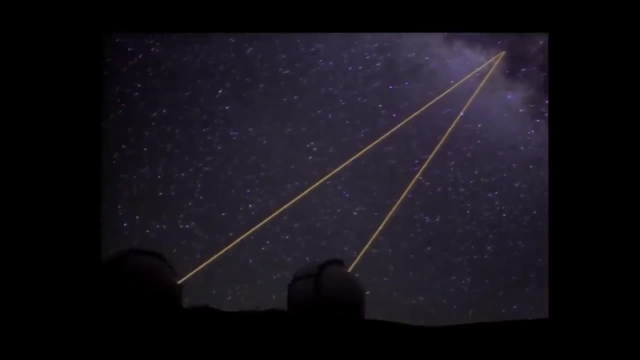 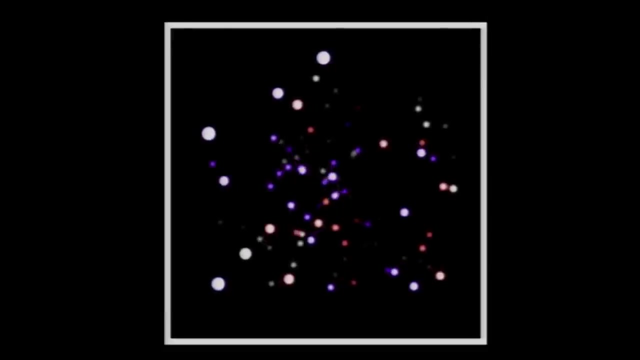 so if they were to send a signal it would take 25,000 years to get there. so I don't think if there's anybody at the galactic center they're going to take much notice of that. But anyway, here is what they can see. 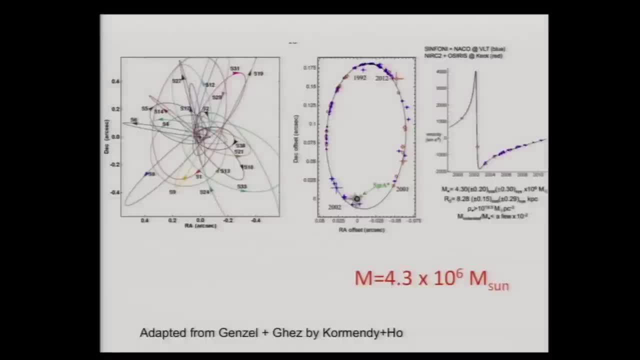 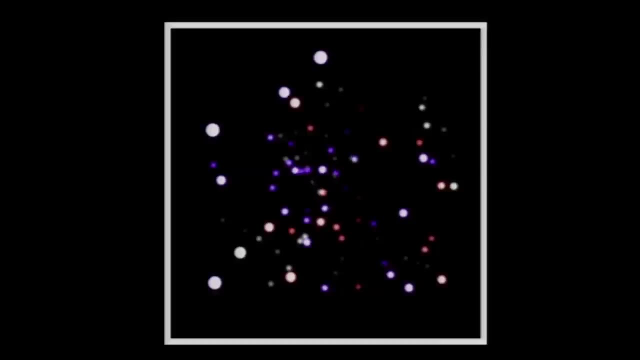 in terms of the motion of the stars and you see, the stars are doing something moving around the center here. If we now look at that, these are the actual plot of all the motion of those stars. and there's one of the stars I'll go back, it's this one. 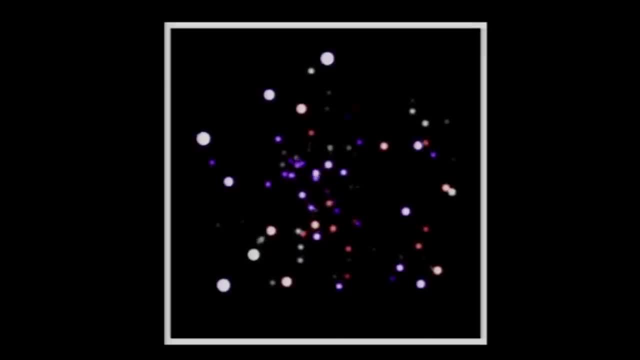 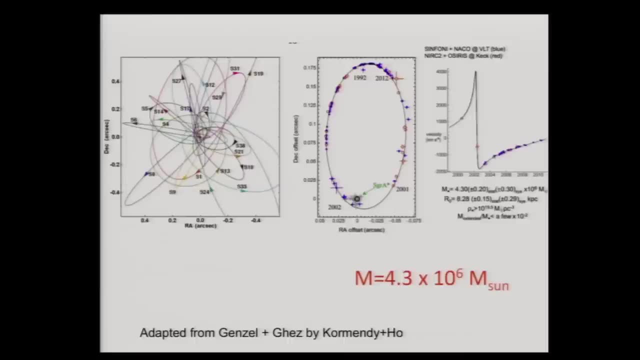 is orbiting the center about once every 15 years and that's a star, and when it was going close to this point, it's orbiting around this point in an elliptical orbit. when it's close to this point, it's traveling at 4,000 km per second. 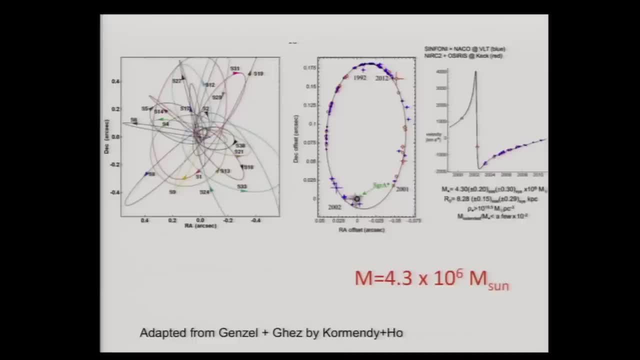 this is the radial velocity of it and these are the positions of it. Using Newton's equations of gravity, you can work out the mass of the object there. That mass turns out to be four million times the mass of the Sun, And yet it has to be a very compact. 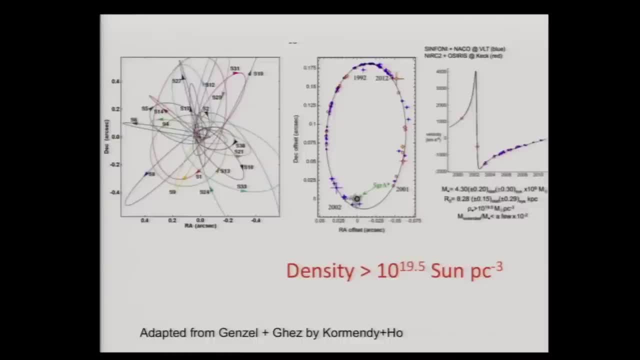 region because it follows an orbit very precisely. How compact does it have to be? It has to have a density which is more than 10 to the 19.5 times the mass of the Sun per cubic parsec. You probably don't know. 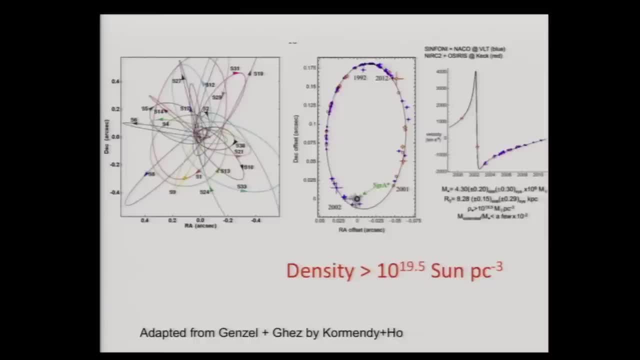 what a cubic parsec is. it's a distance measurement in astronomy. essentially, a parsec is the distance between us and the next star, approximately. so our local density of stars is one in these units. This is a hundred million million million times higher than the density 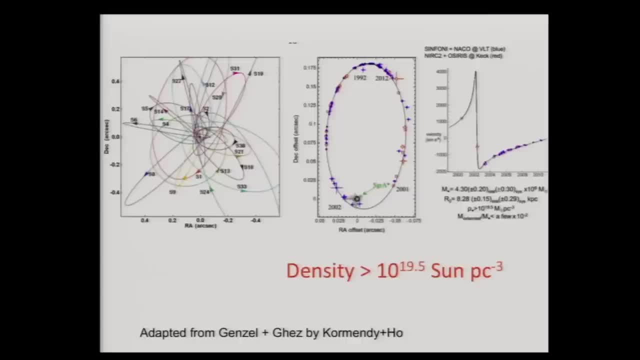 locally to us. It can't possibly be made of stars, because it will be incredibly bright. it can't even make it out of neutron stars. without the neutron stars colliding with each other. There's nothing known to physics that can be there, other than a black hole. 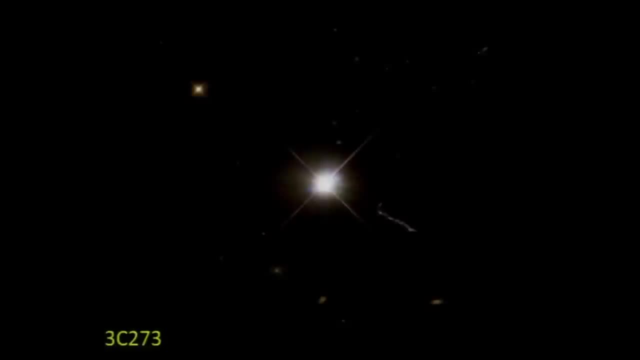 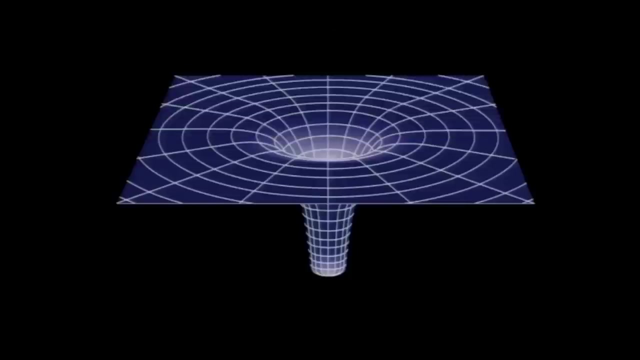 Now black holes also are powering quasars. but let me go on to the concept of the black hole. this is from Einstein, the idea that mass warps space-time, and here it's shown warping the space just in a two-dimensional representation. it's something where the 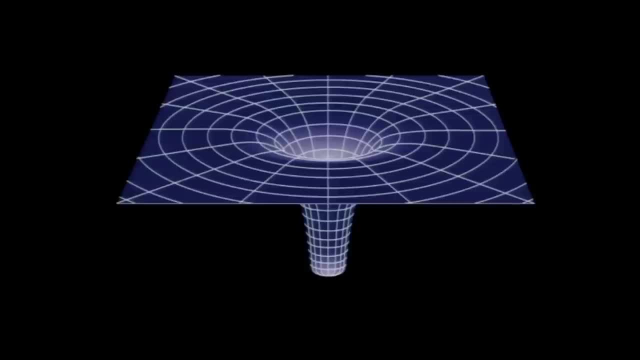 center has collapsed, warping the space around it, and there is an event horizon around it, a little bit like a waterfall. this is Niagara Falls, of course, but you've got to think about this edge round here as being a point beyond which you can't come back. 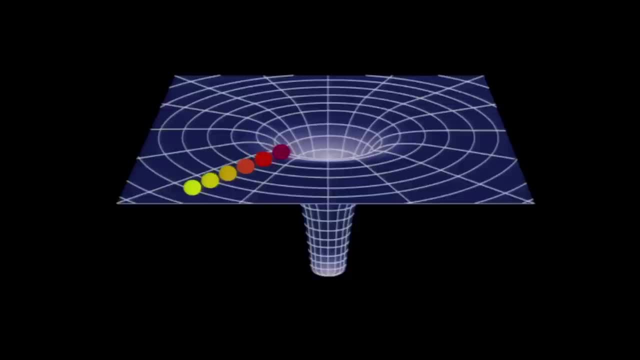 and we call that the event horizon. as you approach the event horizon and are observed by an outside observer, you go from looking yellow to red, you appear red-shifted and eventually time appears to stop. if you had a clock, your clock would appear to stop by the time it gets here. 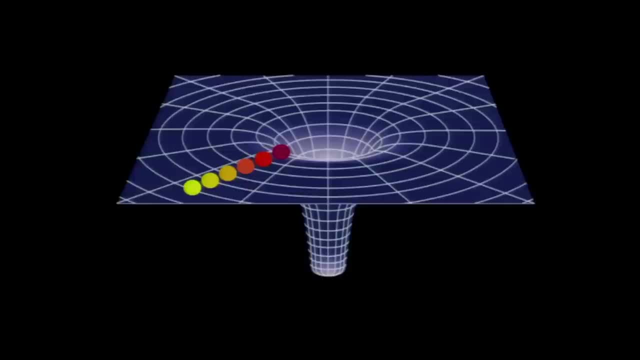 you never actually appear to the outside observer to fall into the black hole. so black holes were originally a theoretical concept and originated in the 1780s by a man named Mitchell, who was a fellow of Queens College but spent most of his time looking after a parish in Yorkshire. 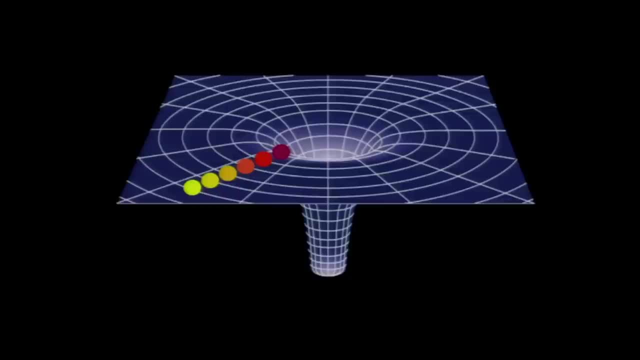 but he theorized that if he was to pack lots of suns together, lots of stars together, eventually they would have an escape velocity from the surface bigger than the speed of light and therefore you couldn't see them. that's a Newtonian argument which isn't right nowadays. 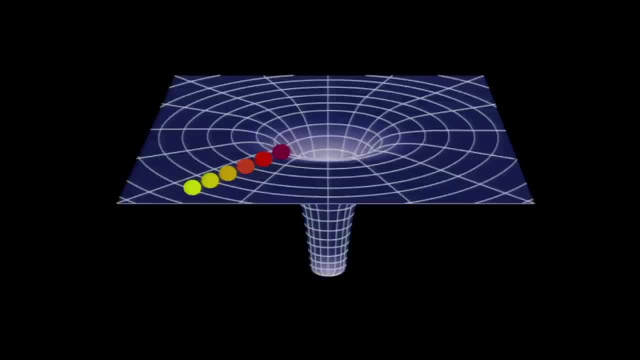 but Einstein came up with his general theory of relativity, and that gave rise to the concept of black holes. the equations were solved the following year, just 101 years ago, by Karl Schwarzschild, for a stationary point mass and then for a spinning object, back in 1963. 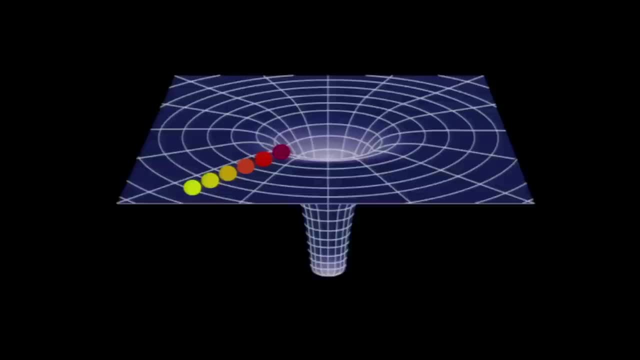 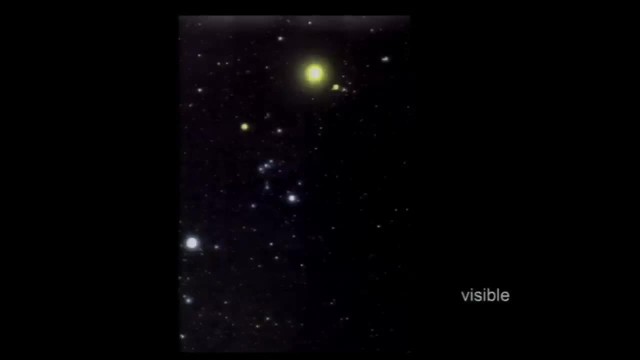 by Roy Kerr. I now want to show you a few examples of black holes. about black holes, by just showing you a picture of the sky. this is the visible sky and if there are any amateur astronomers amongst you, you'll recognize this pattern. this is the constellation of Orion. 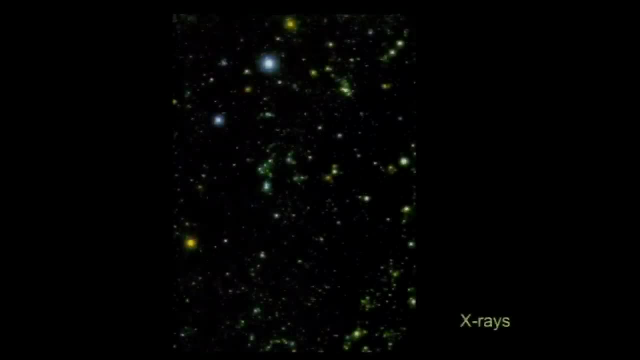 with Betelgeuse there and Rigel there, and that's the brightest star in the sky. Sirius, this is the moon, and that's the constellation of Taurus the bull, just like in the X-ray band. there it is, and then you can see the stars of Orion's belt. 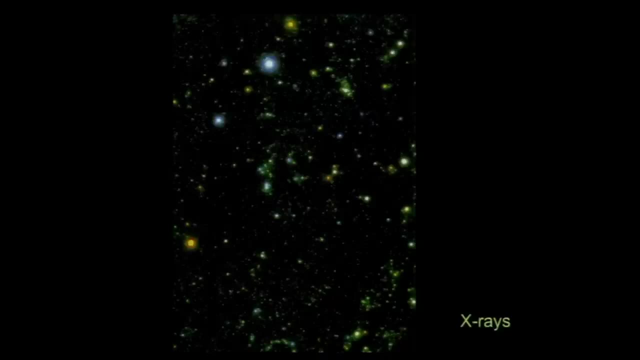 flip back, you can see Orion's belt, and they're showing up because of magnetic activity, like we can see on the sun. you cannot find Betelgeuse in this picture. the moon is that thing. this bright thing here is the Crab Nebula, which I've already shown you. 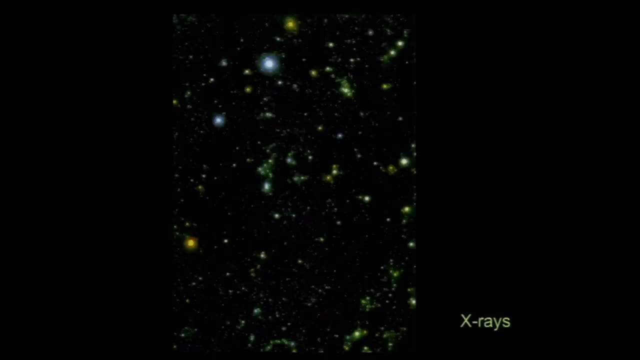 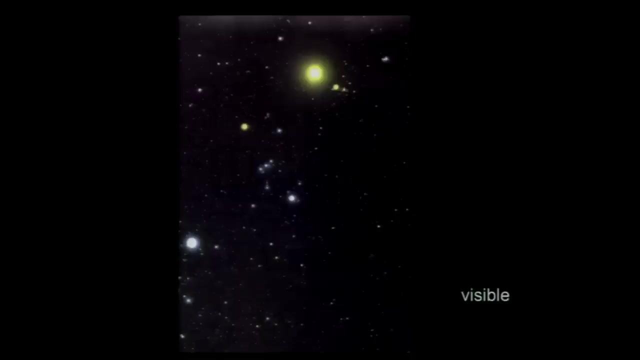 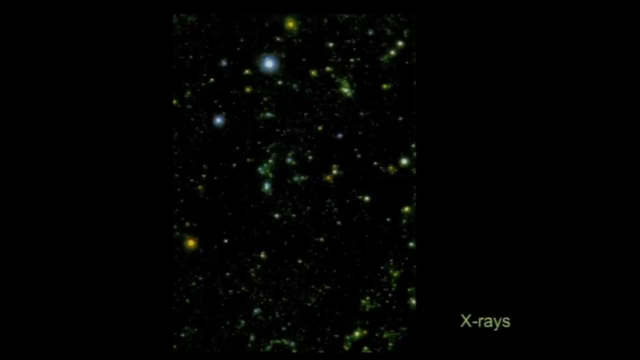 Sirius, but not Sirius A. this is its white dwarf companion, Sirius B. so in X-rays you see Sirius B, not this bright star which is Sirius A. they orbit each other every 50 years, so in this picture in X-rays you see dead objects, white dwarfs, neutron stars. 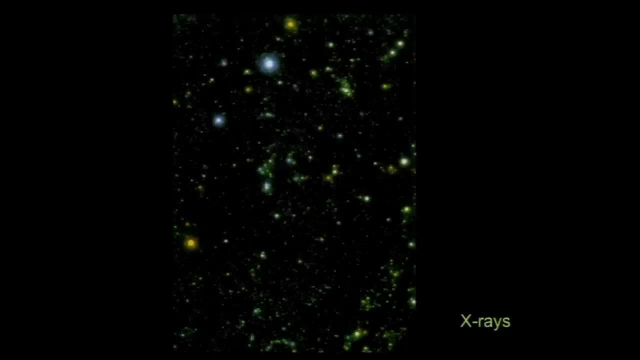 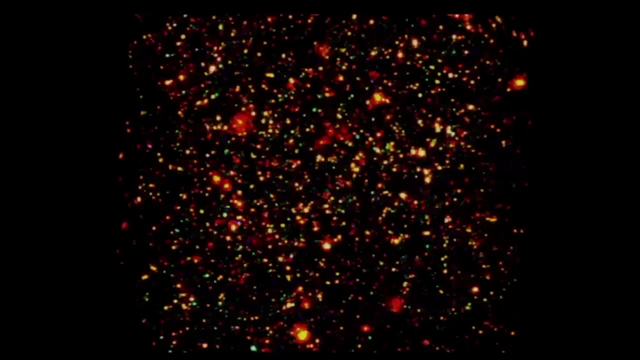 some active stars, magnetically active stars, and many, many black holes, and here we can see black holes. now I've just said things can fall into a black hole and you can't see them. they can't go out. how can you see black holes? you see black holes. because material falls into them. they are the ultimate thing to drop material into and you can release the greatest amount of energy by dropping material into a black hole, and this is just an X-ray image of a patch of sky and 95% of the dots there. 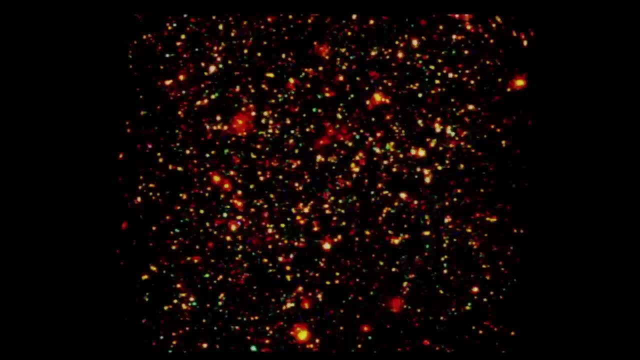 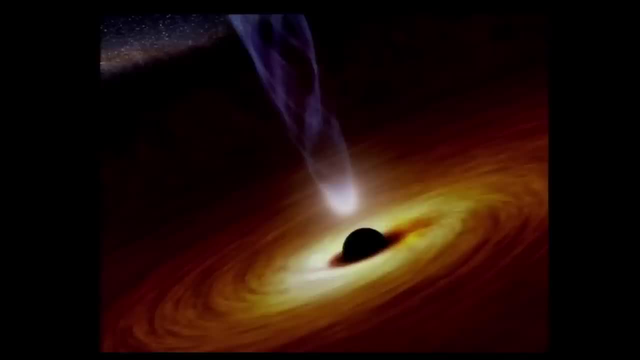 are black holes accreting material from their host galaxy. some of these things are clusters of galaxies, the big, fluffy ones. there is an artist's image of one of these black holes accreting material in the form of an accretion disk. we expect the matter to swirl around. 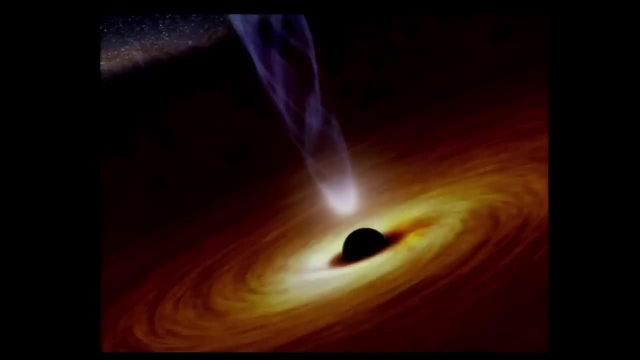 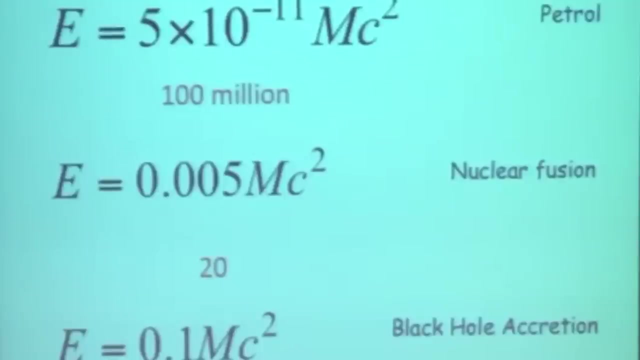 and sometimes the magnetic fields generate powerful jets that come out of them. so accretion, dropping matter into black holes, generates enormous amounts of power. and just to go through some numbers with you, this is: E equals MC, squared, but with an efficiency factor for chemical reactions, that is. 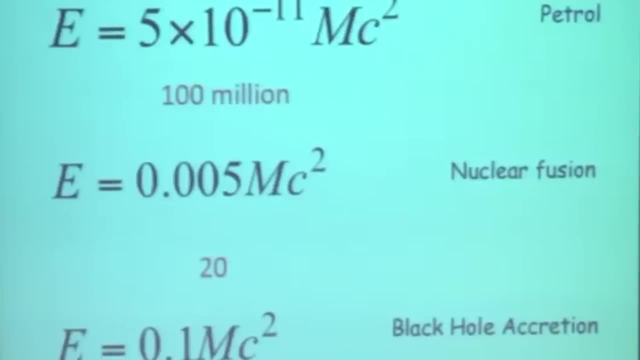 5 times 10 to the minus 11. it's a very small number. chemical reactions are very inefficient. in E equals MC squared. nuclear fusion is 100 million times better and that's what powers the sun so clearly. you're getting a lot of energy out for your mass. 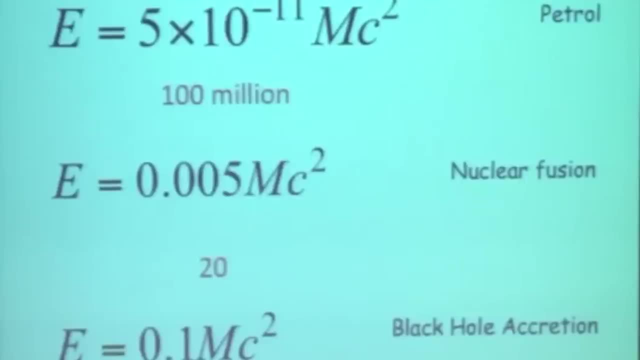 and indeed, if you were to take your petrol from your car and enable it to undergo nuclear fusion rather than chemical reactions, you'd go 100 million miles per gallon, or should we say 100 per gallon? you can go even 20 times better than that, if you can go to black hole accretion. 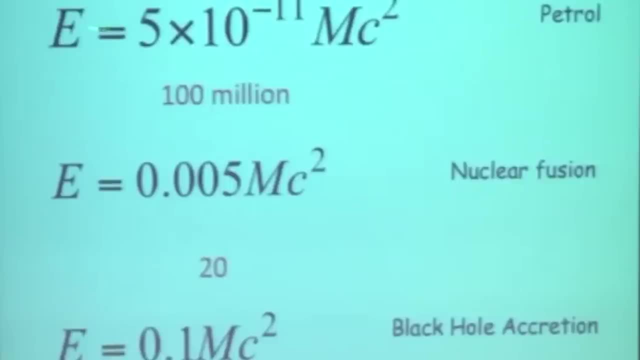 if you drop matter into a black hole, you can release more than 10% of its rest mass. so small amounts of matter in galaxies falling into black holes at the centers produces an enormous amount of power. I've shown you pictures of the black hole at the center. 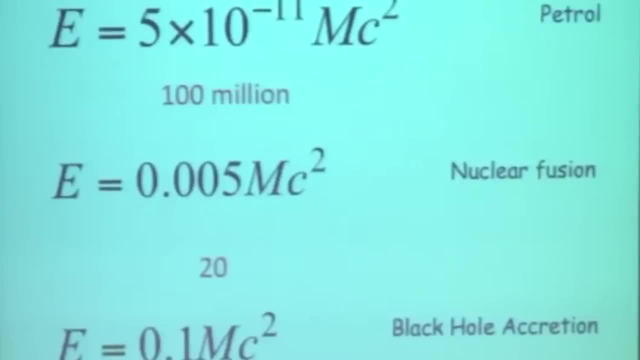 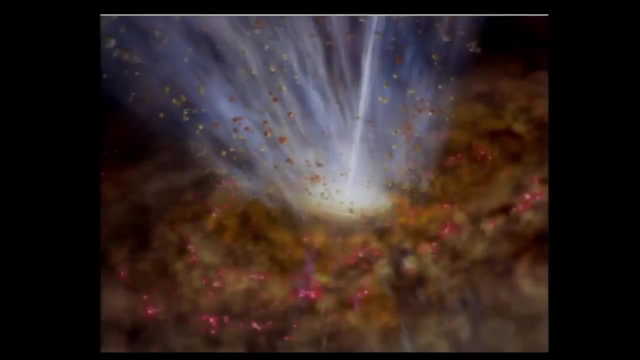 of our galaxy. it is not very bright. it's not got much material falling into it. in many other galaxies they are very bright and what they do in this brightness is essentially blast all the gas out of the galaxy, and we think that this is the reason why many of the elliptical galaxies 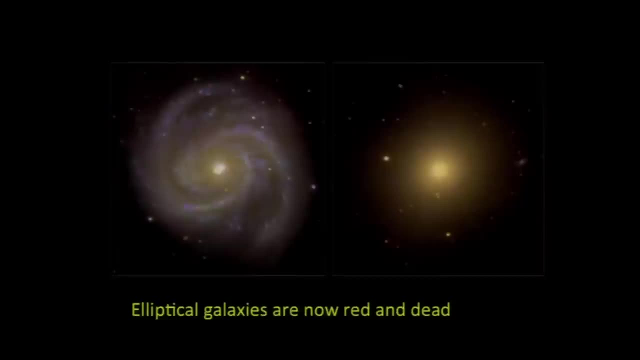 the most massive galaxies in the universe are mainly these big balls of stars. they all look now red and dead, unlike spiral galaxies, which have got lots of star formation. we think that's because the black hole at the centers of these galaxies has blown all the gas out. 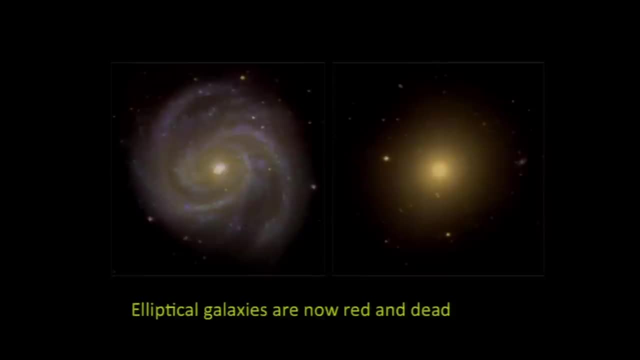 of the galaxy. in blowing all the gas out of the galaxy, they stop any new stars forming. there's no gas to form new stars. this is amazing. this has been a realization in the last 20 years. it's the black hole at the center of the galaxy. 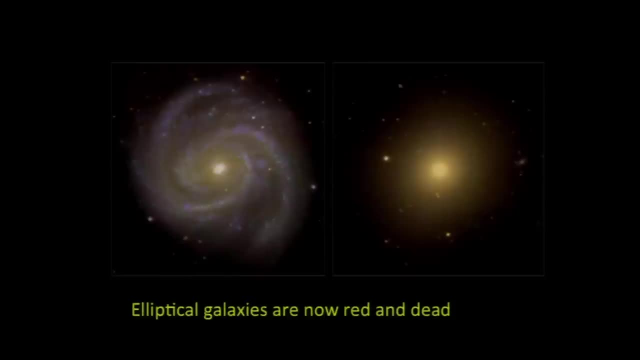 that controls the mass of the whole galaxy. when a galaxy ends its life, it's due to this tiny little thing. spatially tiny- it's actually got one thousandth of the mass of the galaxy- but it's physically very tiny. it's got a size- the black hole at the center. 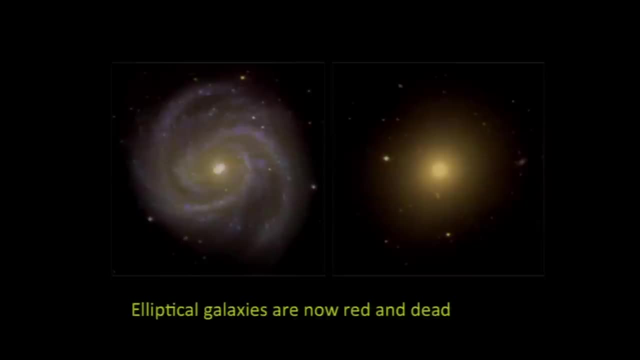 has a size compared to the size of the galaxy, a bit like the size of an orange compared to the size of the earth. that's an extreme for you. imagine something small controlling something that big. it's got a thousandth of the mass but small amounts of matter falling into it. 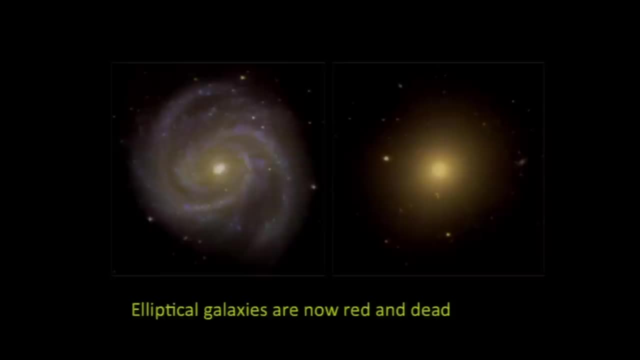 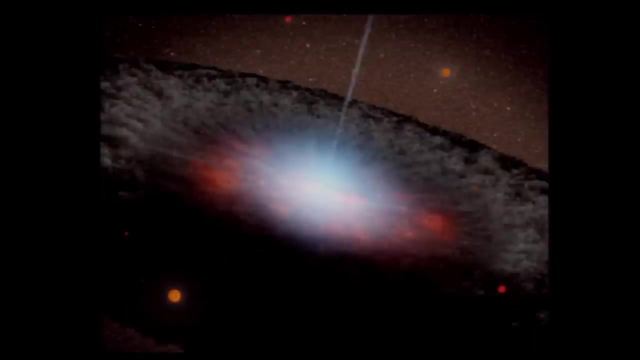 blast all gas out of the galaxy. that's what we think is happening in quasars. moving on, there are these jets that come out of them, often powered by the magnetic fields, and if we happen to look down the jet, those objects can look even brighter. so 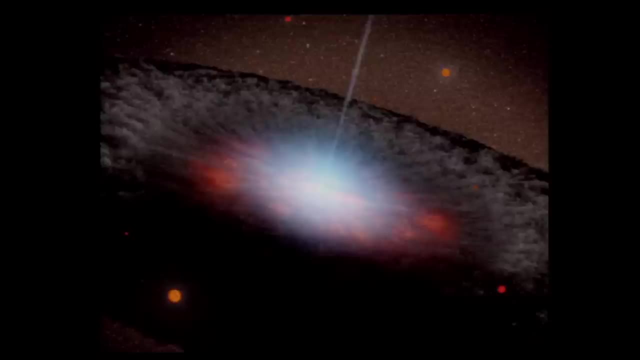 this is very bright, but if you look downward it's going to look very, very bright. and actually one of these objects at quite a high distance- and for anybody who's an amateur astronomer they might know about redshifts and redshift one- there was a quasar at redshift one. 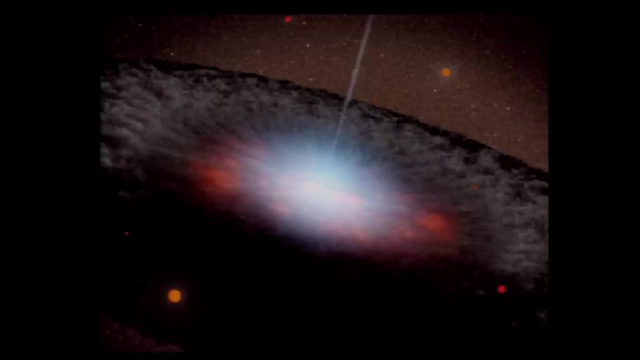 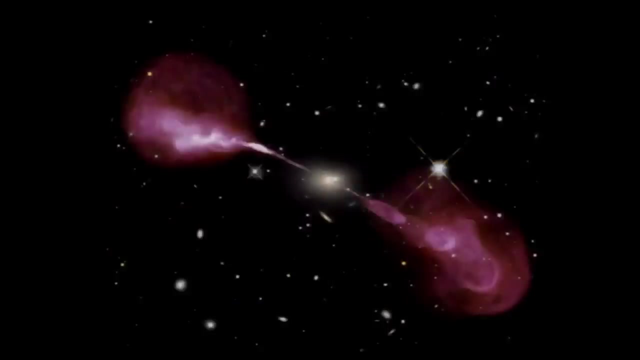 visible in binoculars just over Christmas because its jet pointing at us underwent an enormous flare. these jets can go out beyond the galaxies. this is a large galaxy and it's squirting these jets out either side, making these enormous lobes. this is actually emissions seen. 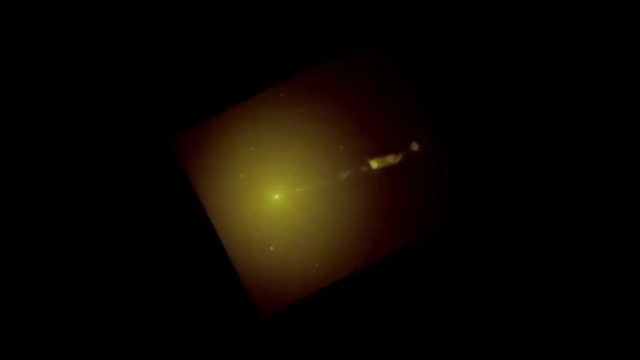 in radio wavelengths, overlaying on an optical picture of that region. now these jets can lead to interesting phenomena. this is the nearest jet that has been seen. it's in the constellation of Virgo, in a galaxy called M87. and here's this jet sticking out that side. 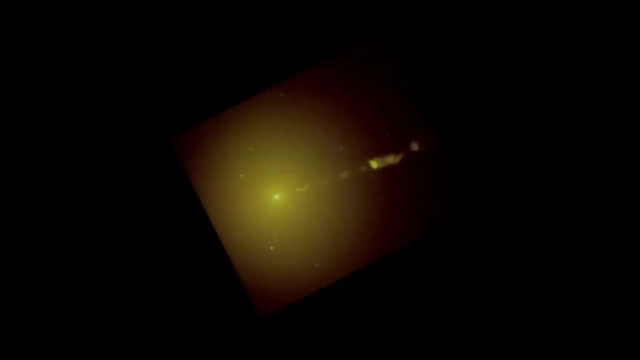 you cannot see a jet the other side. this was found a hundred years ago by Heber Curtis, who wrote that there is a thin white ray emerging from the nucleus of M87. he didn't know what it was, do you know? we don't actually know exactly what it is even now. 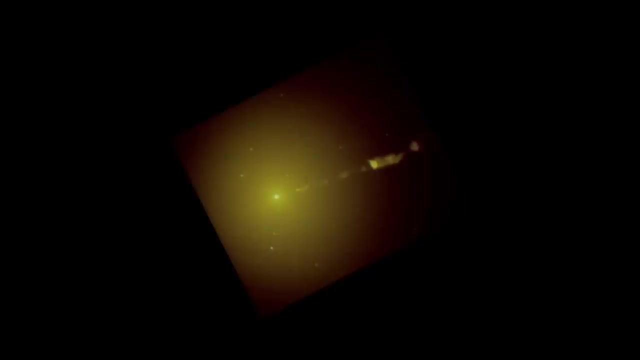 but we'll find out later. we know it's squirting electrons out. we know that because of all sorts of things, including the fact light is polarised- I'm not going to define what that is if you don't know- but basically that means it's got negative particles coming out. 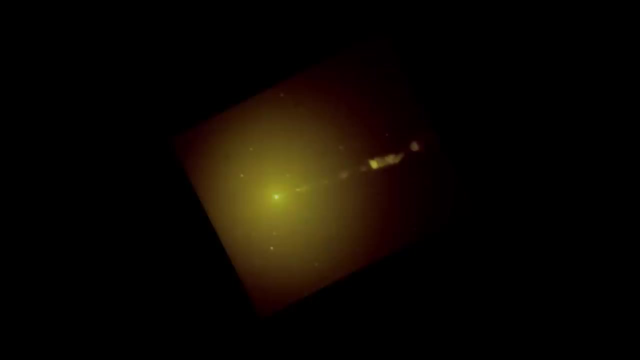 we don't know what the positive particles are coming out, whether they're protons or positrons. maybe it's squirting antimatter out, which is rather interesting. we cannot see the other side. we think they're jets going out. equally either side. we can see that one. 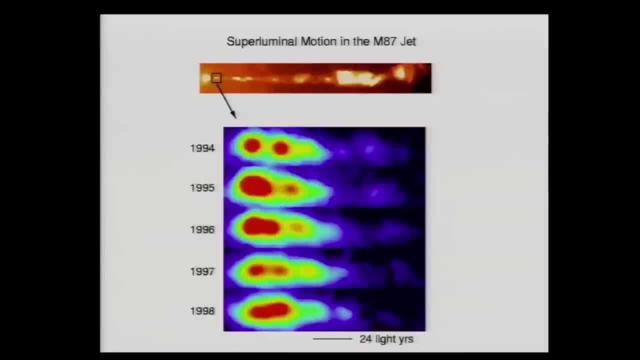 why can't we see the other one? well, we can perhaps start to understand it if we look at this Hubble image of it. it's been tipped round to make it level here, and there's the jet I've just shown you there. we're going to look at this bit of it. 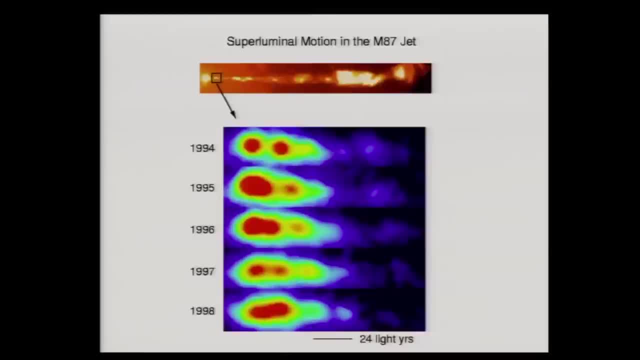 here and can you see, in the 90s Hubble saw something emitted and it's moved across like that. if you work out the distance it's moved, it's gone 24 light years. it's gone 24 light years in 4 years. so it's travelling at 6 times. 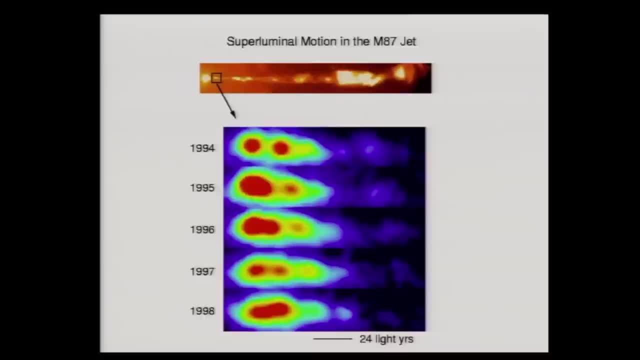 the speed of light. okay, is that? alright, I'll have one of those, please, because that's how I can travel around in space. it's superluminal, it's actually an optical illusion. even those ripples from the supernova were travelling faster than the speed of light. 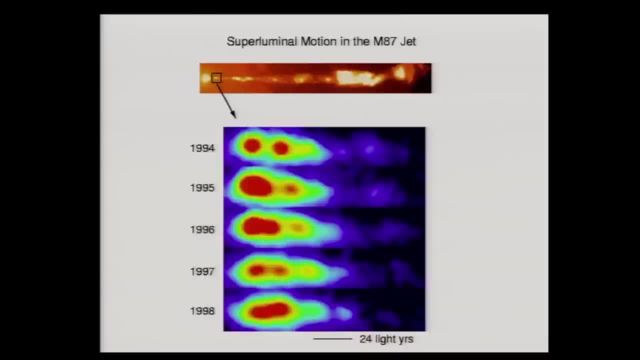 okay. it's due to the fact, in this case, that this jet is pointing towards us and the matter in the jets is travelling very, very fast. it's going very close to the speed of light, it's chasing the light beams and you can do a very simple geometrical 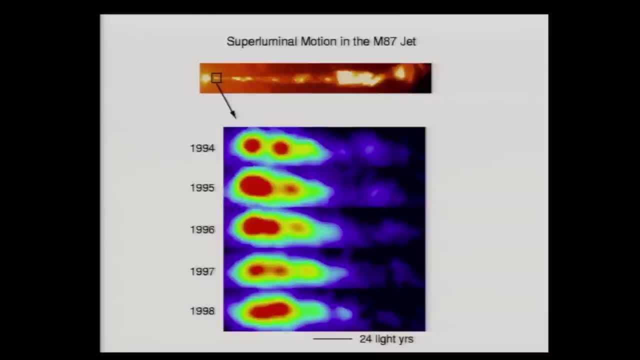 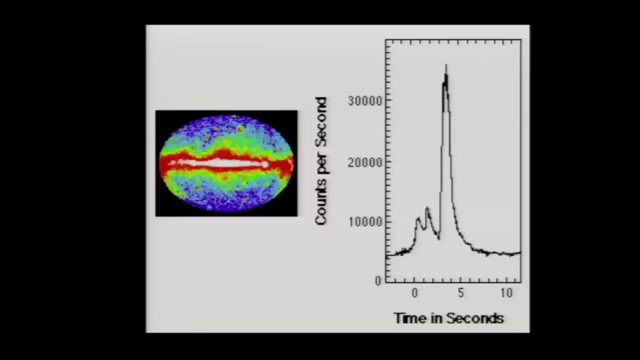 calculation, which I am not going to do here, show that you can end up with this apparent superluminal motion. now, the most amazing jets that we see are these ones, and they are associated with gamma ray bursts. these are intense flashes which were first found in the 1960s. 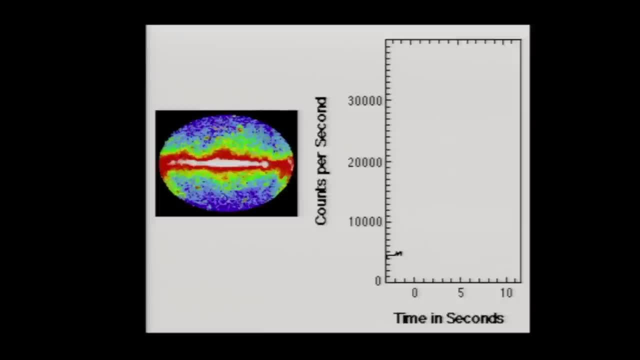 by the military, both the Russian- sorry, the Soviet- and the US military, were monitoring outer space, hoping to check that each other were not letting off nuclear bombs in space. these are monitoring satellites. they did find flashes of gamma rays that you would expect to see from a nuclear bomb, except. 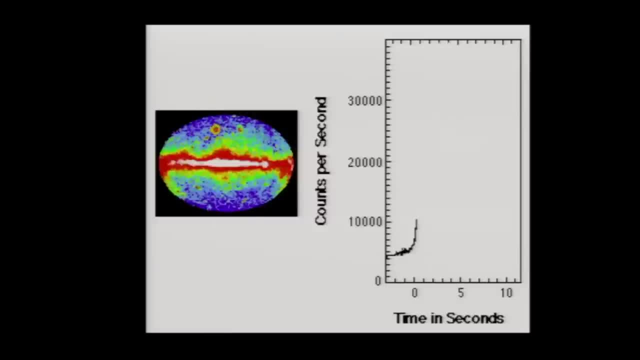 in these flashes of gamma rays clearly came from beyond the solar system. they did not come from nuclear weapons. I mean, people did at one point say, well, maybe their other intelligent life is letting off nuclear bombs, but no, that's not the answer. these flashes like this are associated. 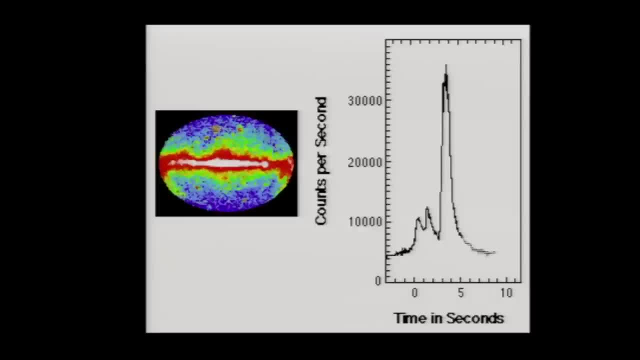 with the birth of black holes in stars and basically what happens is during the supernova collapse, forming a black hole. if the material is spinning very fast, it's able to make jets which squirt through the whole star and out through the star. and if it's shining, 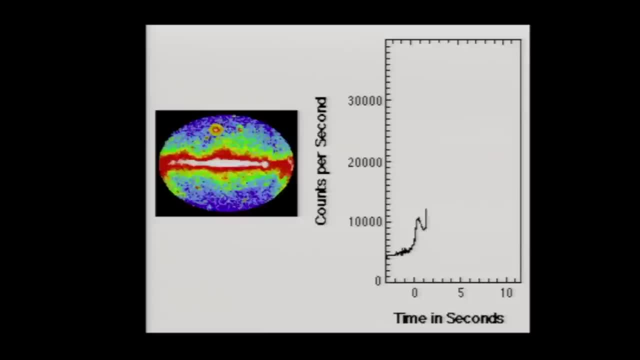 at us and I'm not going to point this laser beam at you, but you know, a laser beam pointed is very bright. along the laser beam. it's like having a laser beam shone at you. that's what we're seeing here. these things are very bright in. 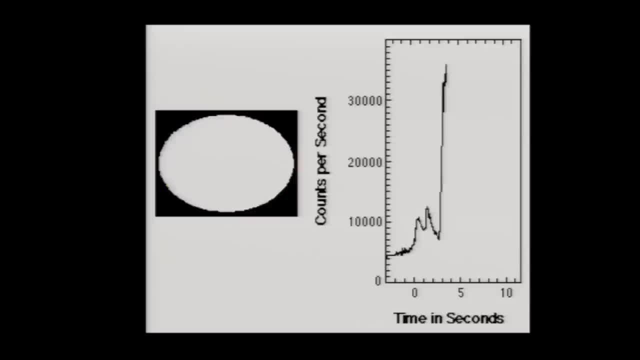 gamma rays. they're gamma ray bursts and, for anybody who knows about relativity, these jets have got a Lorentz factor of 100 and this thing has got a Lorentz factor of 10, but I'm not going to go any further in defining it. these 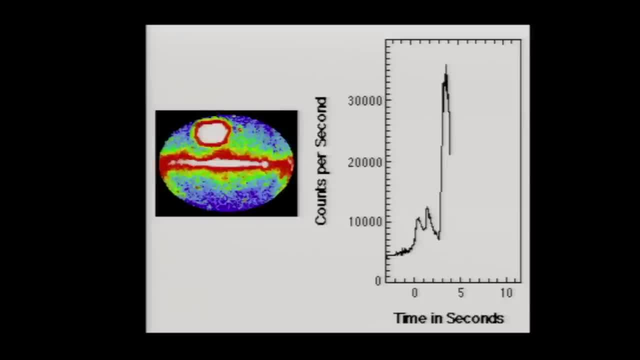 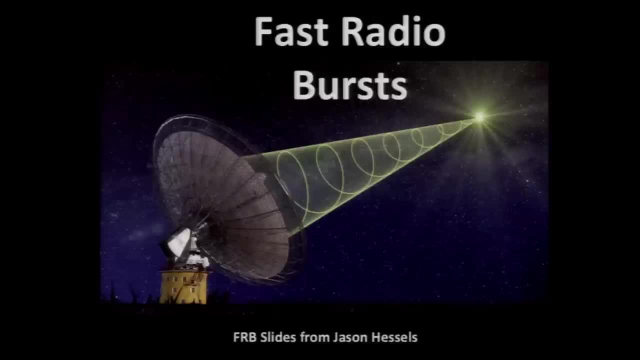 are extreme objects in the sense they've got extreme powers. now I'm going to on my last 10 minutes, I'm going to go through two final classes of objects. these are fast radio bursts. they're the mystery of 2017. they made the cover of nature in 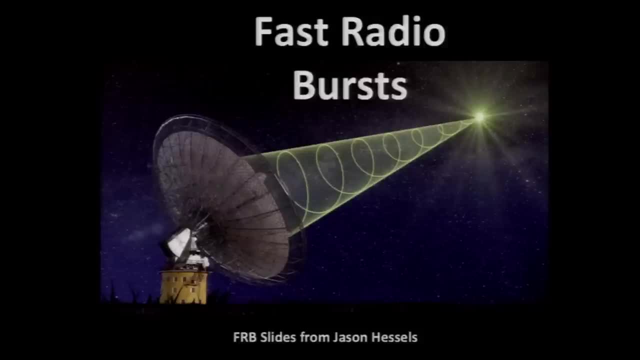 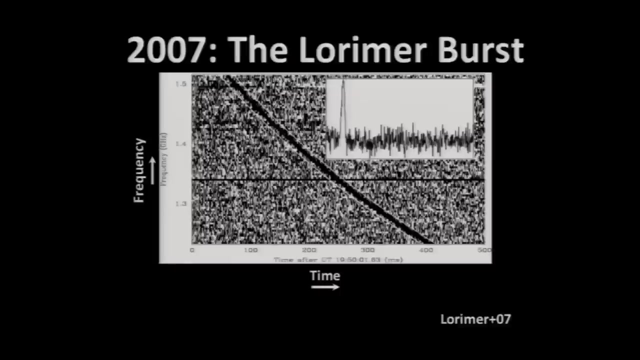 January, the first issue of nature this year. these fast radio bursts were discovered in, first discovered in 2007. these slides were given to me by Jason Hessels, a Dutch astronomer. now that's the Parkes radio telescope here in Australia and it picked up intense flashes. 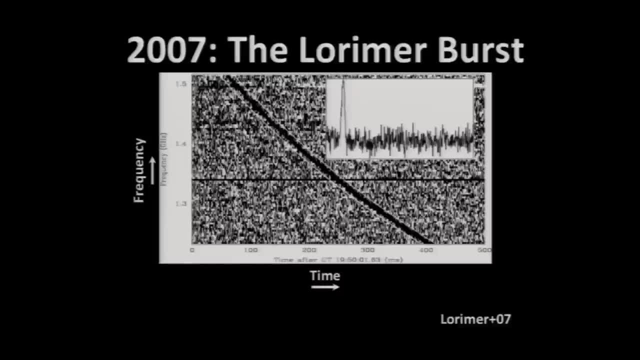 one intense flash in 2007. that's when it was published by Duncan Lorimer, so known as Lorimer burst. it's an intense, very bright flash. these are hundreds of that's: 100 milliseconds, 200 milliseconds, so that is half a second, so it's a very sharp. 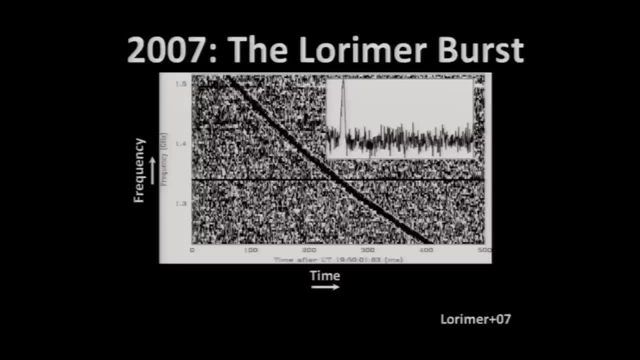 flash. it also changed. this is now frequency and it changed in frequency. so essentially in radio frequency it was first detected at high frequencies and then, you know, it decayed and was seen in the lower frequencies. this is called dispersion of the radiation. is characteristic of radio signals going through ionized. 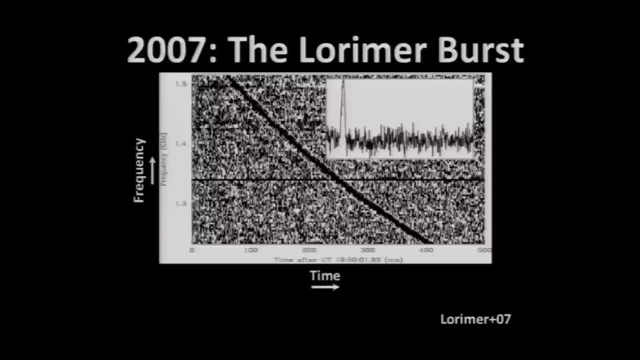 gas, and this looks like it could be the gas between the galaxies, or it could be gas associated with the thing itself. apart from the fact that the radio telescope was pointed at a particular region, they- Duncan Lorimer- had no idea what this is due to. it was clearly. 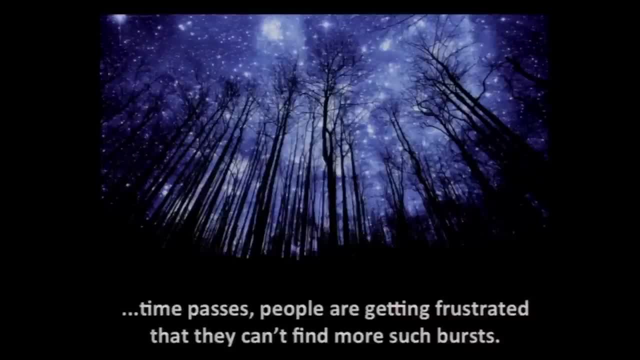 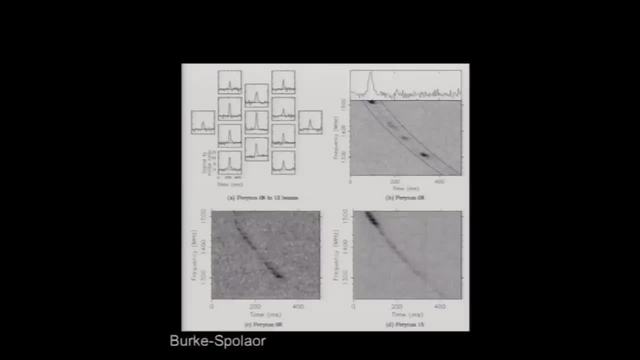 very sharp and very bright people then begun to wonder whether they there were any other ones time passes, people are getting frustrated. they can't find any more bursts. nobody found any more bursts. and then there was some burst, seen also from the park's radio telescope. they looked a bit like 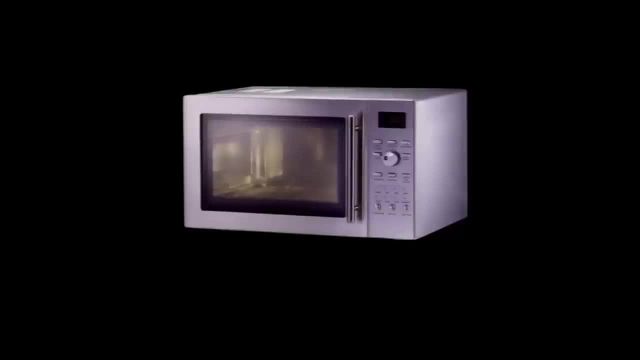 the original one, excepting they were a bit sort of spotty. there's something funny about they don't quite look right, and what they were due to was somebody opening a microwave door nearby. it took a while to work this out, but they're pretty certain that this one 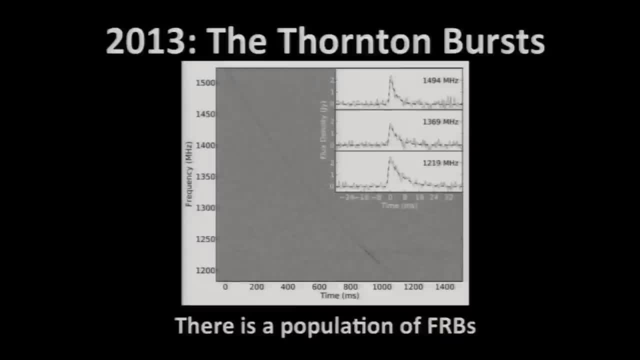 is not due to somebody opening a microwave door, okay, and so it remained as a big puzzle: what's going on here? until in 2013, another burst was seen, or, and a few other. this meant there's a population of fast radio bursts. people didn't know what they were. 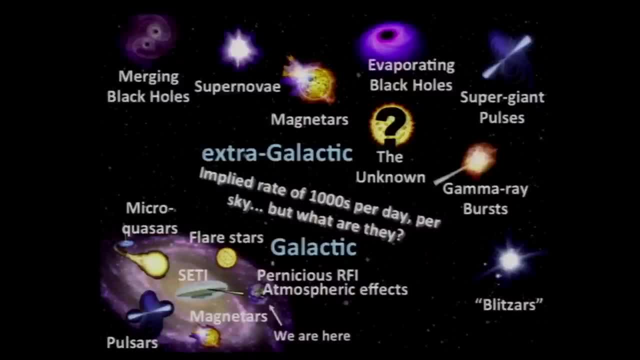 because these radio telescopes are only looking at a tiny patch of sky. there must be thousands of these over the whole sky per day. but what are they? and you could? these are all the ideas. are they pernicious? radio frequency interference or atmospheric effects, flare starts. 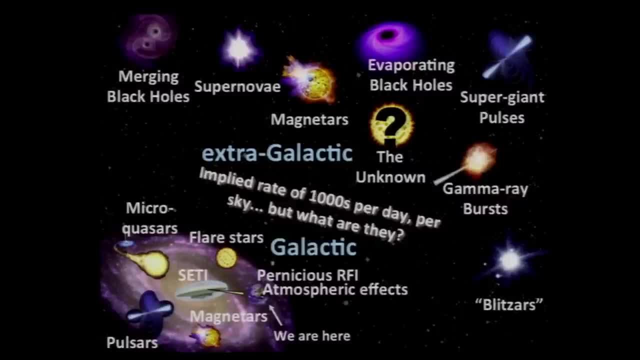 we've already heard about flares. are they micro quasars, pulsars, magnetars, or are they seti? are they little green people? okay, can they be something new? gamma ray bursts, super giant, pulsars from pulsars, evaporating black holes, Stephen Hawking, supernovae. 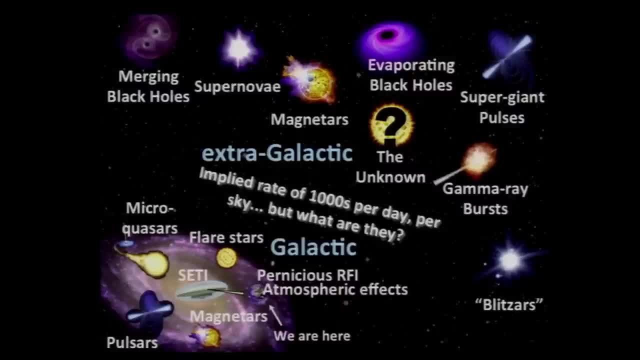 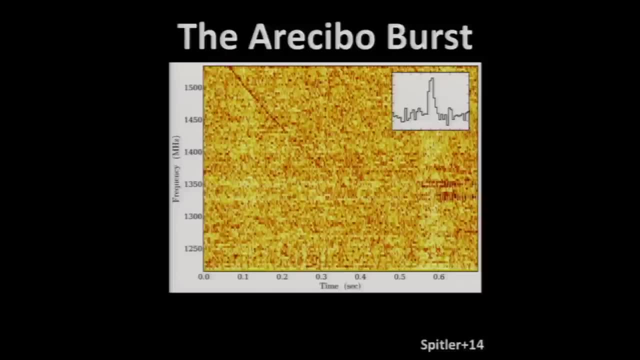 merging black holes. I'm going to talk about that in a minute. we don't know. and then another one was found from the Arecibo telescope. you can see it's not a great one, but there it is, and this is the start of making working out more what they are. this came. 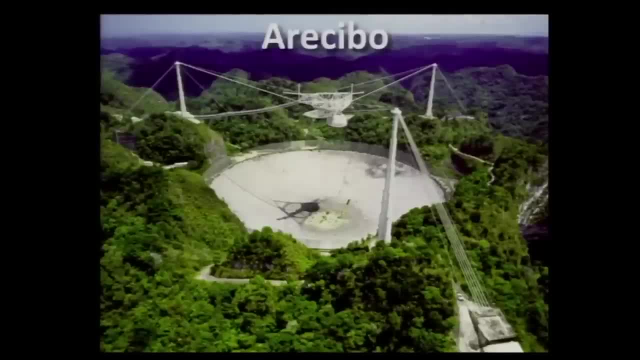 from this Arecibo telescope, which many of you remember, if you like watching Bond films. they fought on here during the film, and which film was it? GoldenEye. well done, thank you. yeah, I always remember the eye bit, because this is an eye on the sky. okay, so there we are. 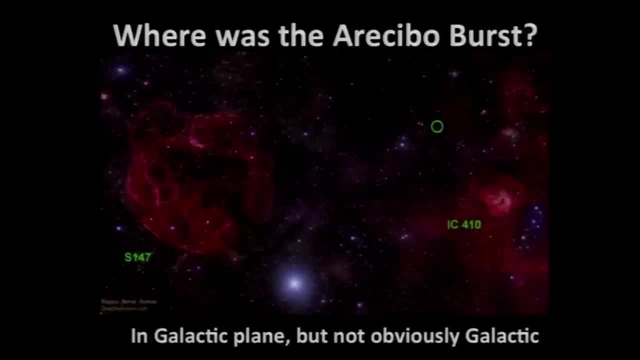 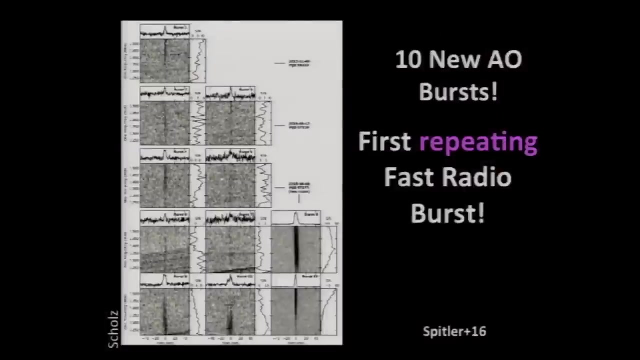 anyway, it came from there. okay, this is a globular cluster. this is the plane of our galaxy, the Milky Way. so it came along the plane of our galaxy. but it's not obvious. it's galactic, and then they found more from the same position, so it's not. 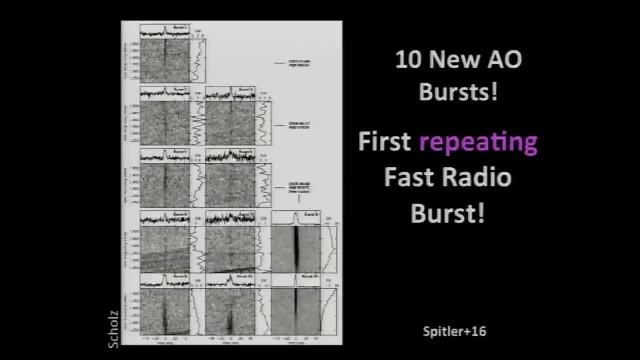 due to a cataclysmic explosion, something blowing itself to pieces. it's repeating and you can see there are many more of them. you may wonder why they're not all shaped like that. that's because somebody straightened them all up just to pack them all onto a. 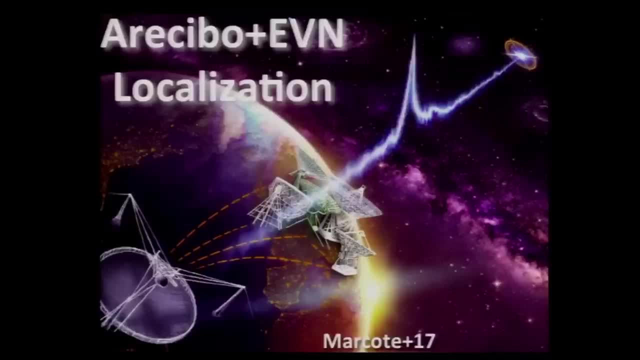 simple plot, so really important. it rules out the cataclysmic source. it's not a single explosion. it's due to a pulsar- on steroids perhaps. and they even worked out where it came from because it repeats. they even found there was a constant source at the same position. 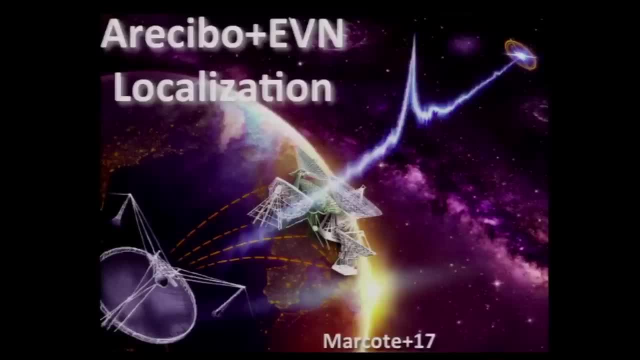 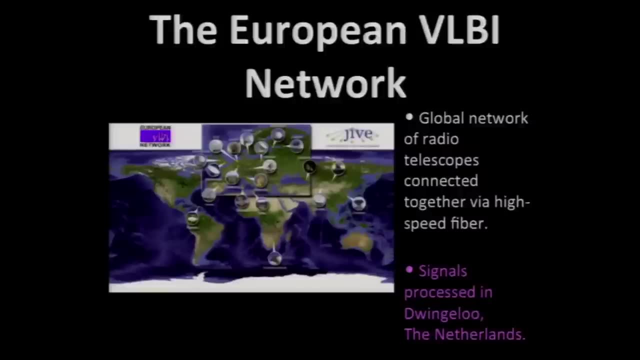 they were able to combine a whole load of radio telescopes- Arecibo and the European VLBI network- and there's a map of it and you probably can't read this, but this one here is it's. this one is Cambridge, so anybody who drove up the 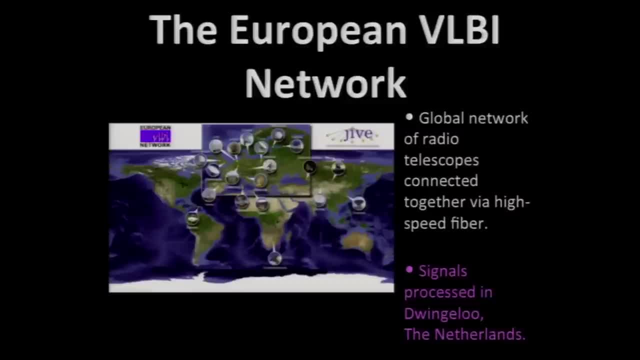 Barton Road will have driven past the telescope, the big dish. there is part of this, this European very long baseline interferometry network. by using all these telescopes at the same time, looking at the same patch of sky, they can get a very accurate position and the net result is: it came from. 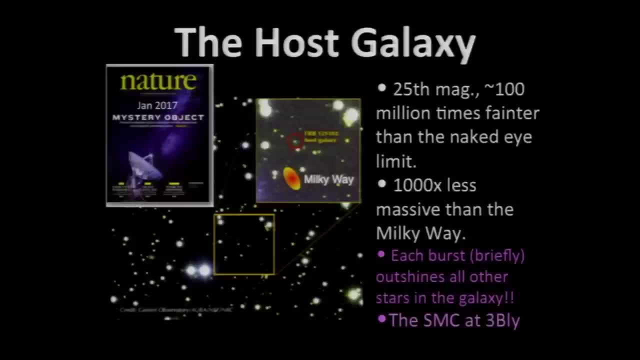 this object. it came from that object, and you can see it doesn't look very exciting, does it? so this burst came from there. this is the cover of the first nature of the year, and so this is where it comes from. it's a very faint object. it's a hundred million times fainter than the 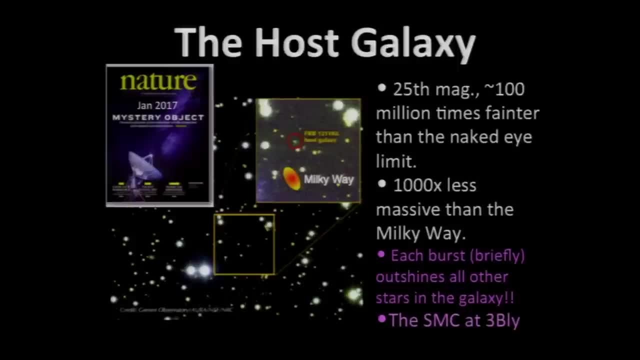 naked eye limit. the galaxy it comes from is a thousand times less massive than the Milky Way. I showed you that supernova 87A came from the large Magellanic cloud. the small Magellanic cloud has about this mass, so it came from a little tiny galaxy. 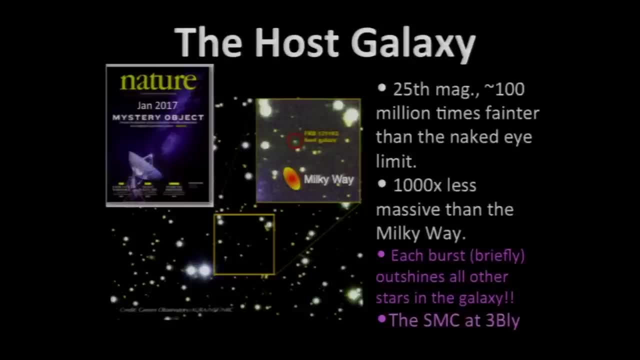 and each burst, when it goes briefly, outshines all the other stars in the galaxy and it looks like this object is the small Magellanic cloud, only at three billion light years. so these bursts we're looking at happened three billion years ago. what are they? we don't know. 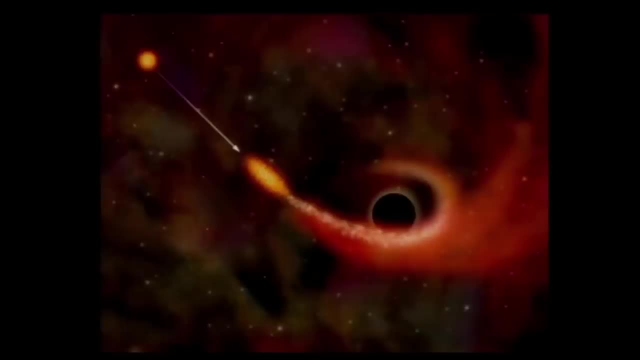 I think, and many people think, they are actually due to a very long magnetar. okay, if a magnetar were formed, you know, maybe 20 years ago- we don't, we never saw a supernova from there, but then maybe we wouldn't have done and maybe it's left behind one. 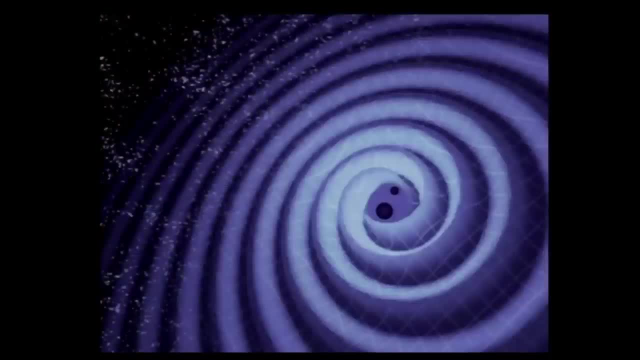 of these magnetars. it remains a puzzle now into the last part. one other class of flare that you can get is when a star strays close to a black hole and is ripped apart by the tides. I don't have time to talk about those, but I'm going to talk now. 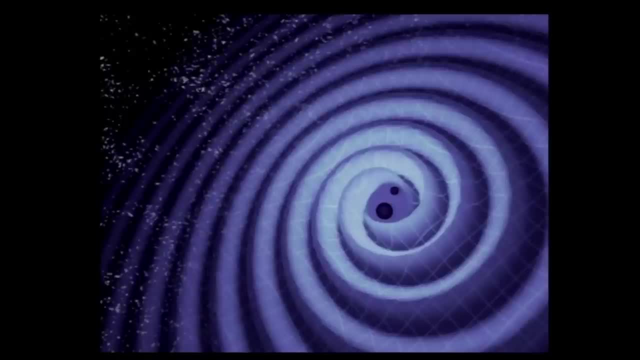 briefly about gravitational waves. when you get binary stars spiraling together, when they orbit each other, they cause warping of space time and they cause gravitational radiation and this is meant to represent ripples of space time flowing away from this binary system. you can get binary stars. 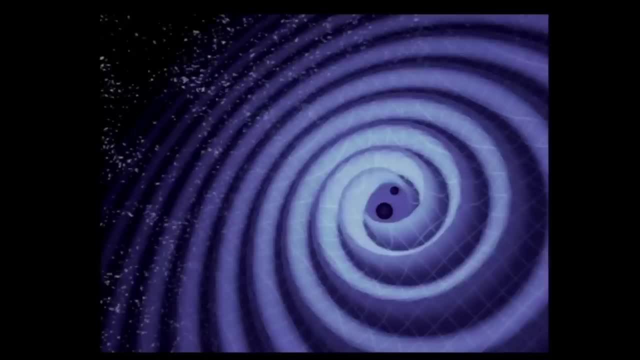 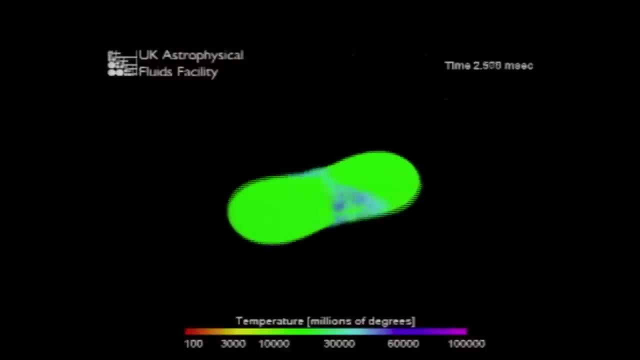 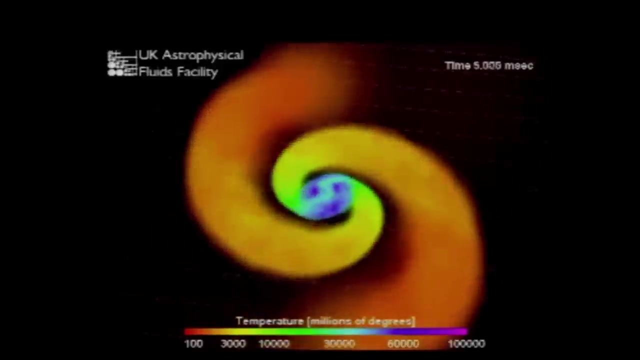 of different types. white dwarfs we've already spoken about, but you can also get neutron star and neutron star binaries. here they are, and these are the temperatures going up to 10,000, no, 100,000 billion degrees when you merge two neutron stars together. 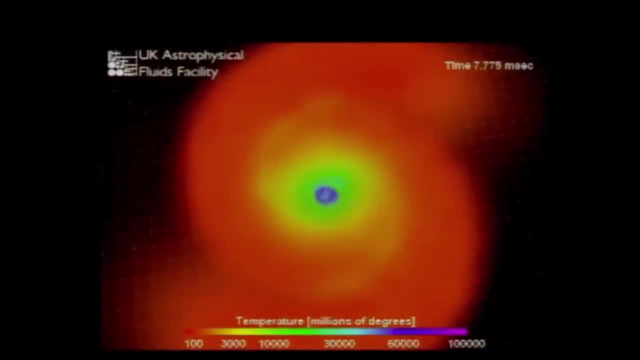 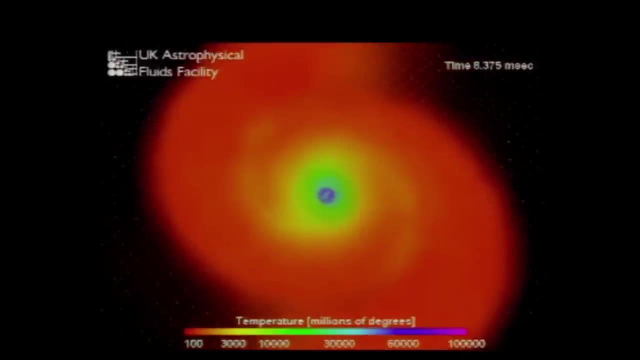 like this, you probably get a gamma ray burst and you also generate a lot of heavy elements. it turns out that in the generation of these heavier elements- I've talked about oxygen, I've talked about iron, but it's very difficult to get significant elements beyond iron out of supernovae- 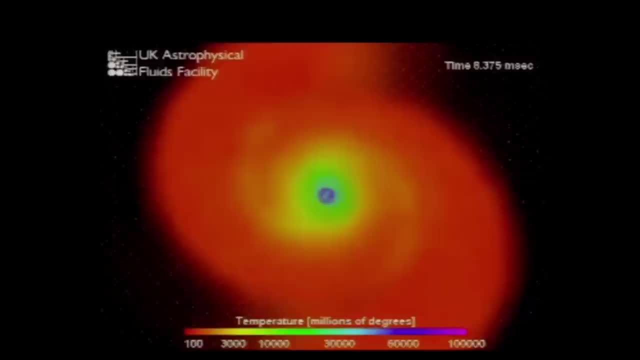 and it's been a big puzzle where gold comes from. I've got some gold. many of you will be wearing a bit of gold. that's where they come from: neutron star and neutron star mergers. that's the only way we can explain gold and when they do this. 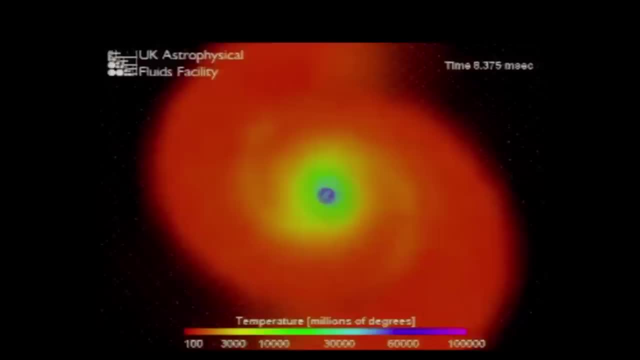 they generate a significant mass of gold- about a moon's mass of gold. now, before you sort of are thinking about a gold moon, it's probably spread in a load of bits and it'll be a very difficult thing to get hold of. but anyway, I'm just trying to say 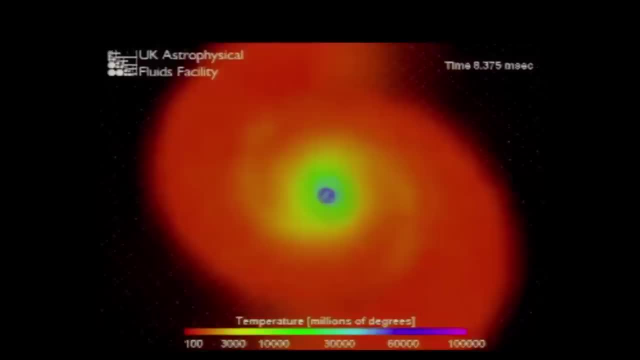 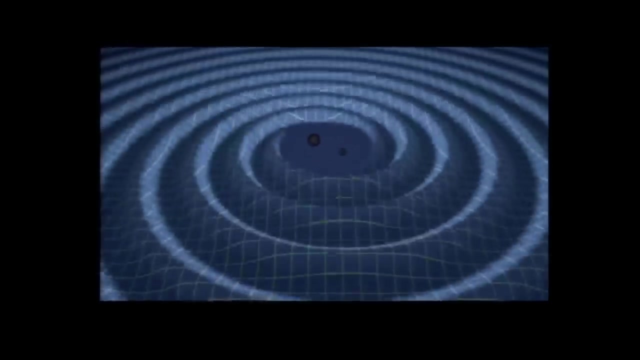 that all the things that you've got are actually connected with you. not you in your current form, but the atoms out of which you were made and the atoms out of which your jewellery is made. now go on to the final one. this is the ultimate one. this is the gravitational wave mergers. 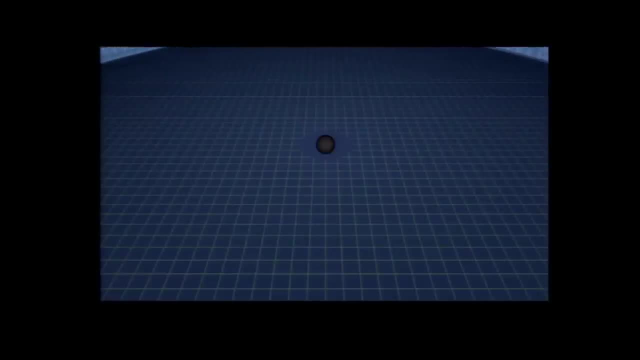 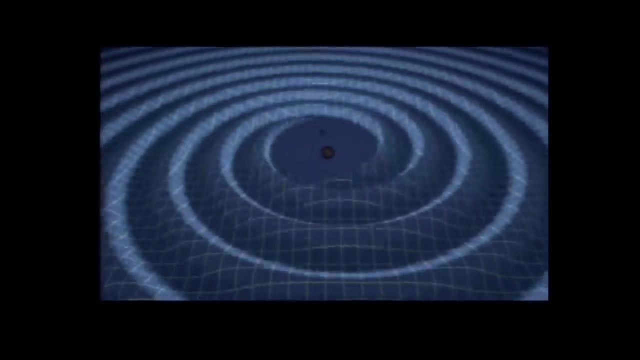 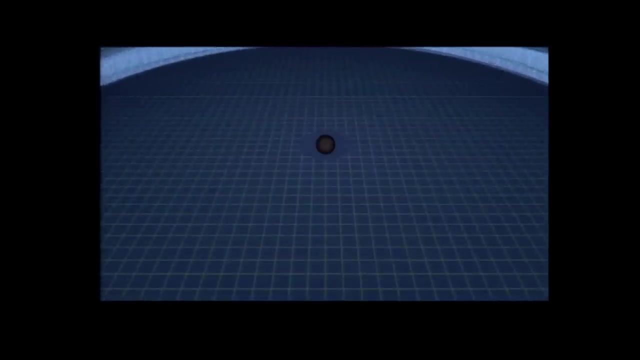 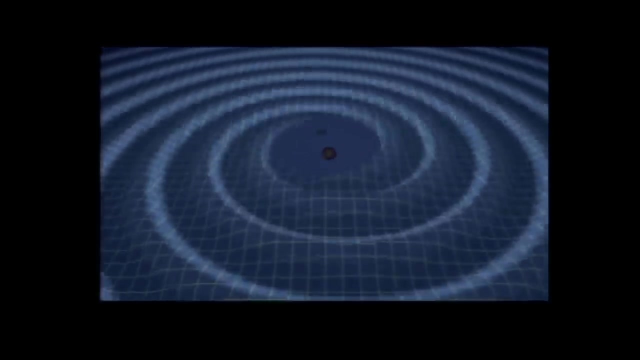 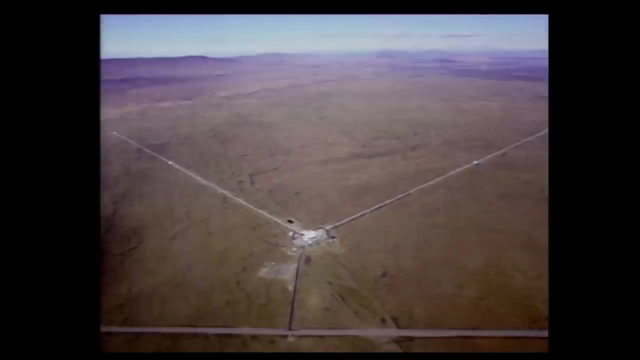 of black holes. two black holes can spiral together and, as they spiral together, leave behind a black hole. and the LIGO Virgo consortium have got instruments now which are the ultimate rulers- rulers in the sense of measuring inches, shall we say. these things are. this is LIGO. 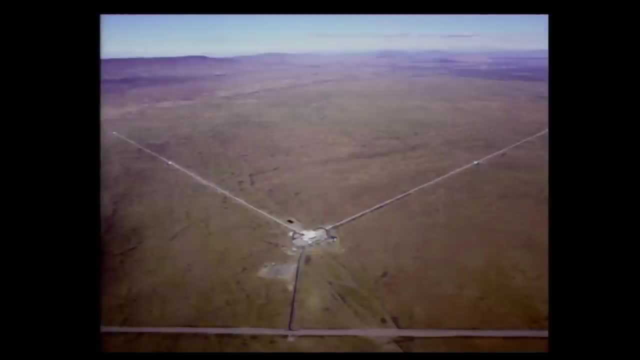 which consists of this cross of laser beams are shining up there. they are comparing these laser beams all the time. if you stretch that and don't stretch that one, then they'll get out of sync and you can detect that down here and you can detect changes in length. 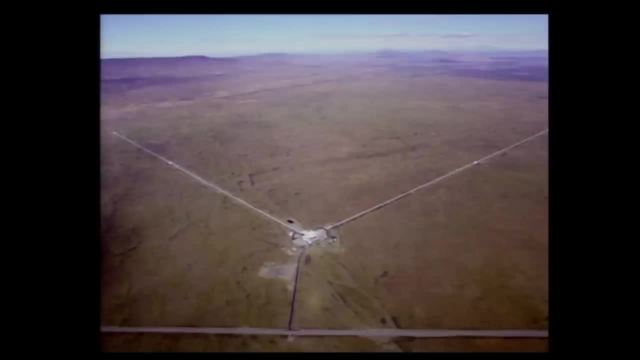 equivalent to an atom. the size of an atom versus the distance between the earth and the sun. that's the precision that they're making with these gravitational waves detectors. 10 to the minus 21, and they switched advanced LIGO on in September of 2015. 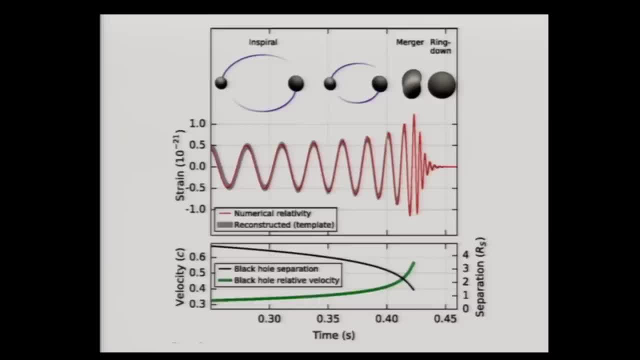 and within three days they had measured a merger. this is what it looks like. there's the oscillation. this is just a plot of theoretical plot of the strain. that's the relative motion of it. you can see the oscillation gets faster and faster. these two spiral closer. 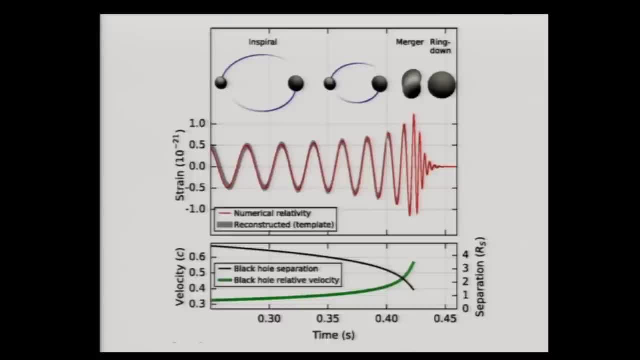 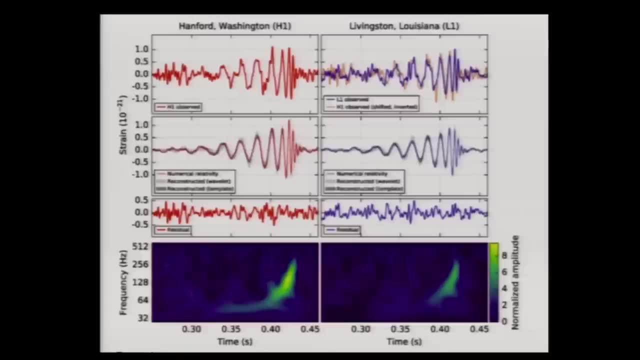 to each other. they merge and then ring down, and so we've got it like this. just to show you the data, here's the data like that you can see. this is frequency. that's time. you see it for only 0.2 of a second, but there's a. 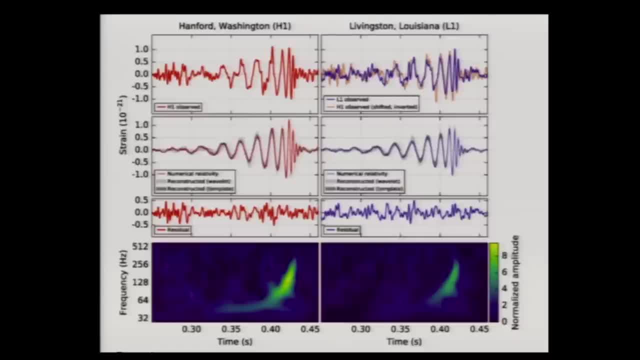 it starts off with a frequency of somewhere like 40 hertz and at the end it's gone up to almost 300 hertz. and that is this detector, which was in Hanford in Washington state, and this is the detector they had in Livingston, Louisiana. so they've got two of these. 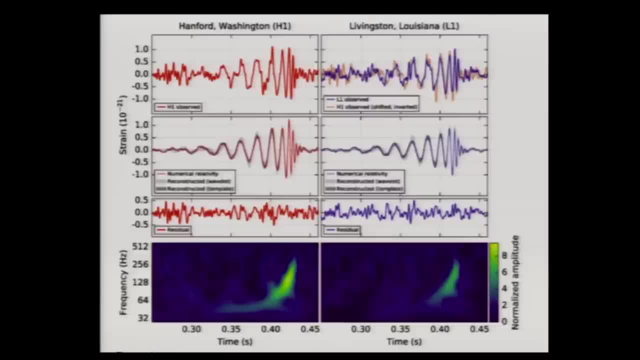 interferometers in the US and they were both working at the same time. they both saw the same signal and in fact you can take the signal from that one and plop it on top of the signal from that one and you see that they match at the same event. 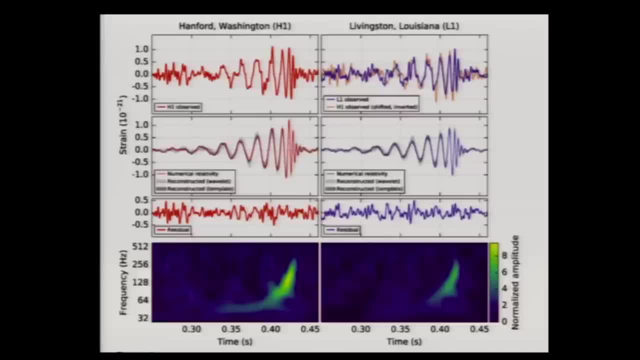 they were extremely lucky because this was the merger of two 13 solar mass black holes, two black holes of 30 solar masses merging together and they presumably formed one of a mass of about 60 solar masses. I say about because three solar masses was lost. it went into radiation. 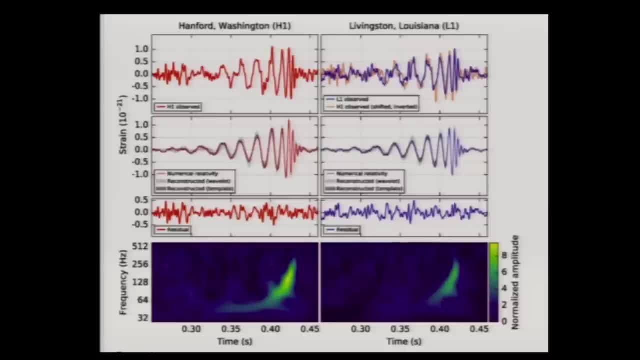 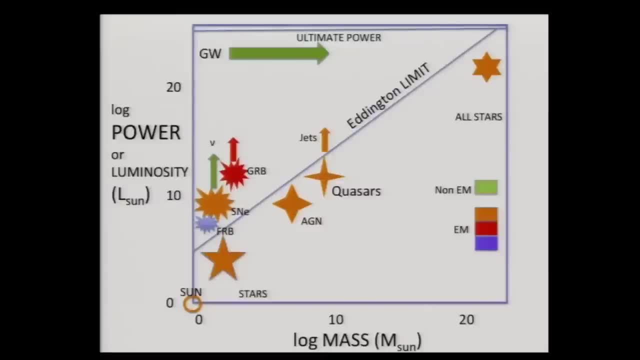 not into electromagnetic radiation. it went into gravitational radiation and this is where it sits in. this plot is the ultimate power is gravitational waves. that merger is up here. I put it at low mass because it's 30 solar mass objects. I've given it green because it's not electromagnetic. 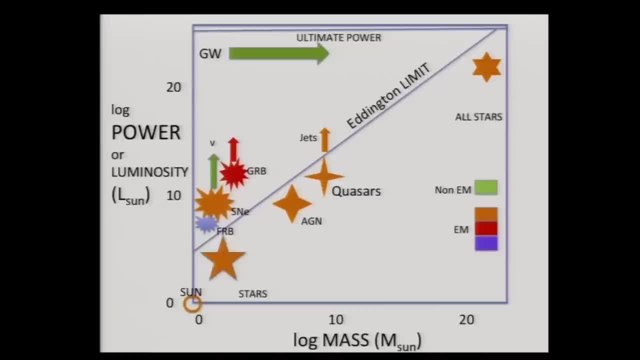 just for 0.2 of a second the amount of power out of this merging system. in terms of rippling space time, the power involved exceeded by more than a factor of 10 the total power from all the stars in all the galaxies in the universe. 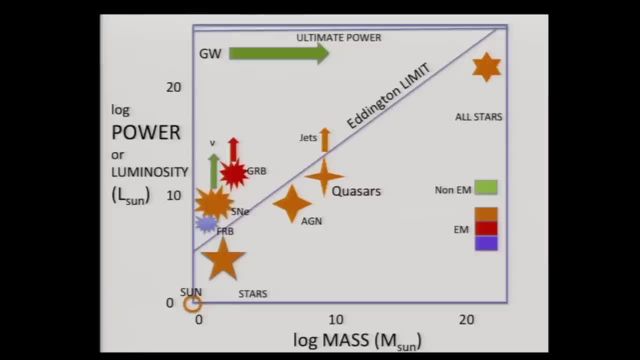 so that it got within 8% of the ultimate power c to the fifth over g. I've now put everything else I've talked about on this plot. there are quasars apparently can look brighter with jets, supernovae, gamma ray bursts, supernovae actually. 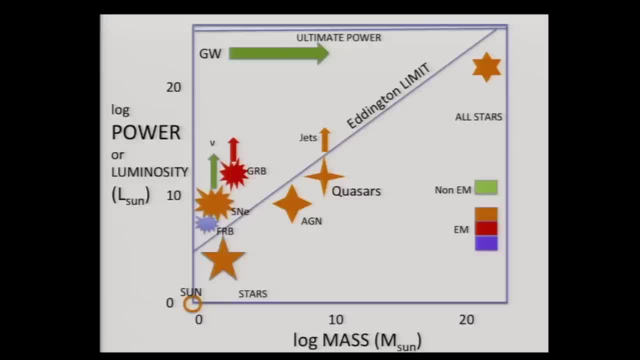 most of the power of a supernova comes out in neutrinos, and the 1987 a supernova collapse did create neutrinos, of which 30 were detected on earth. neutrinos: if you know anything about them, you know that they're ghostly particles which can go right through the earth. 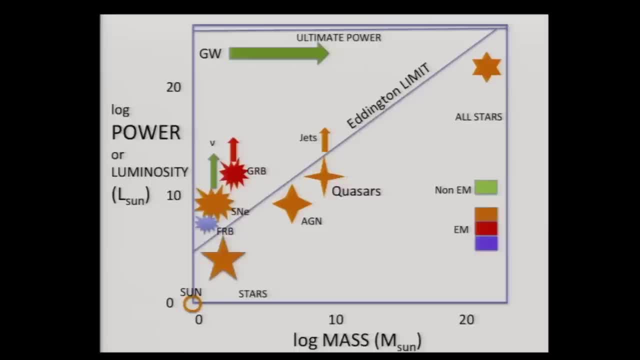 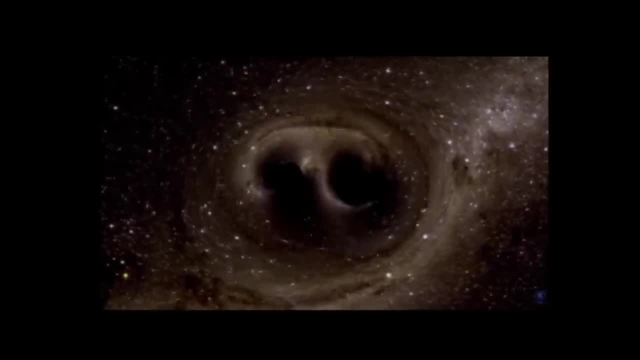 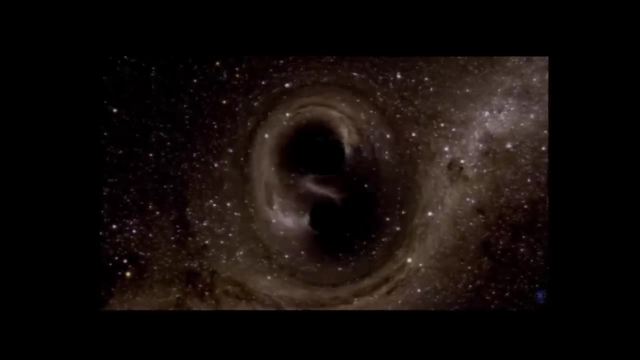 many times, and that's where power lies in the universe, and I'll just- I'm going to finish with a demonstration, but this is just a again representation of two black holes merging. if you were close enough to look at them against the milky way, it would look a bit like this: 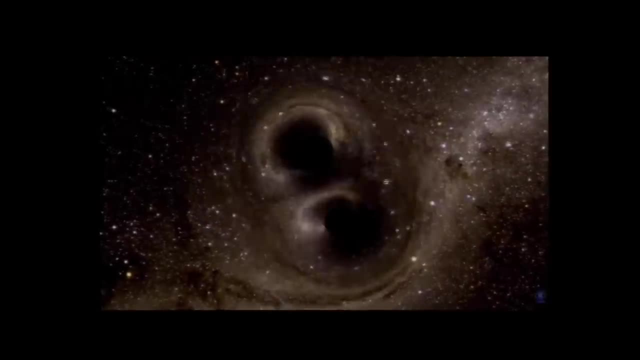 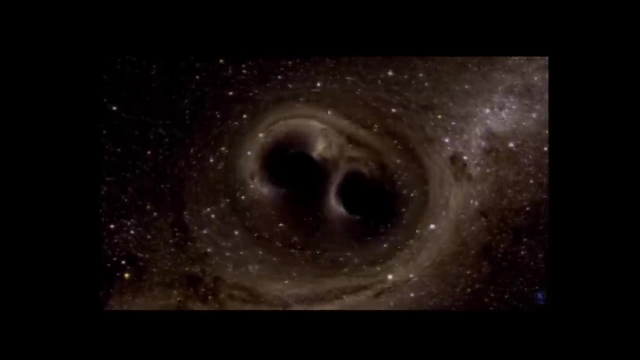 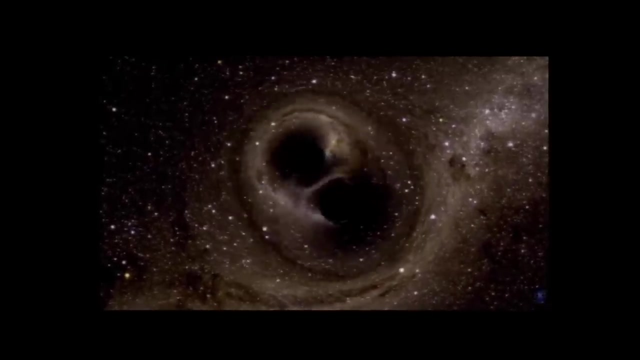 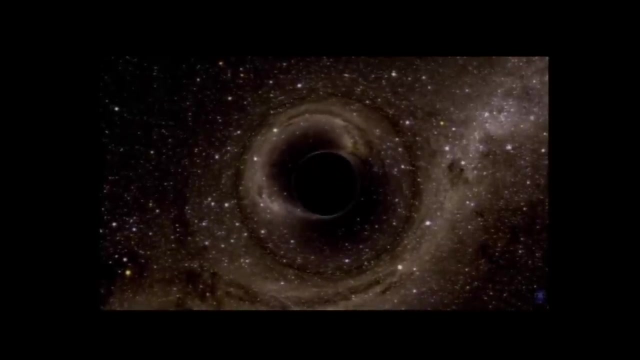 you wouldn't want to be this close, but okay, and here it goes, and space time stops wriggling and there we are, okay, and there's just a nice picture of the milky way. there's the large magellanic cloud and there's the small magellanic cloud. 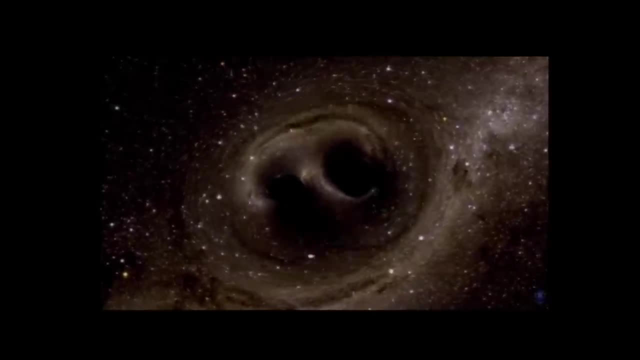 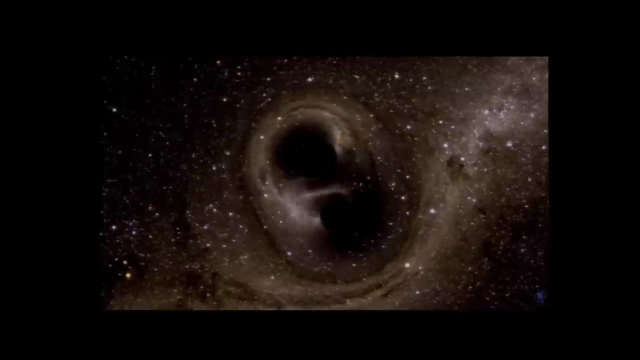 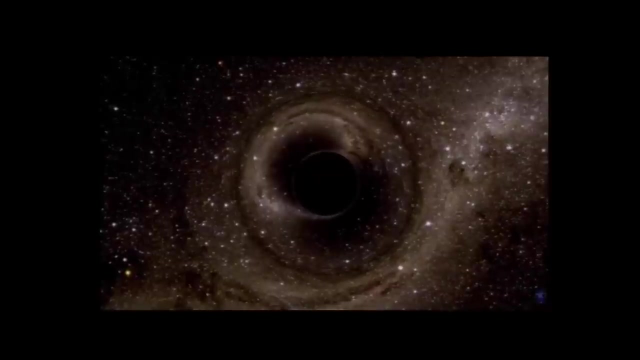 now I'm going to show you just a chirp. what happens? the oscillations got faster and faster and then stopped. that's called a chirp, and that device I'm about to show you actually produces a chirp. and this is your take home experiment. okay, 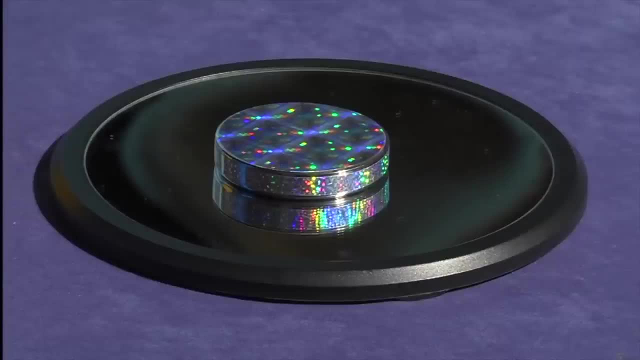 okay, now don't be worried about it's actually a toy. don't be worried about playing with toys. these are three Nobel Prize winners in physics: Richard Feynman, Wolfgang Pauli, Niels Bohr- two great physicists of the last century. they're looking at a toy, it's a top. 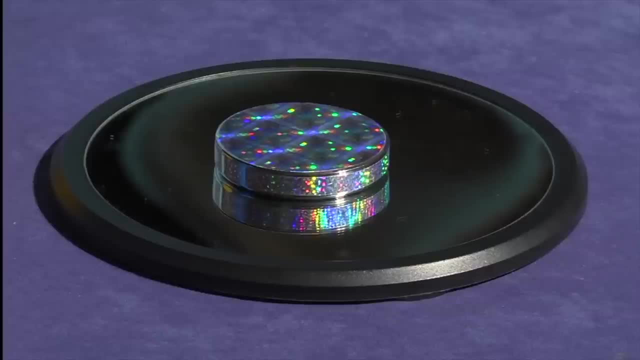 one that you spin and it flips over, if you know what I mean. and they're trying to work out what's going on. this guy, Richard Feynman, was actually watching somebody spinning a plate in the Cornell cafeteria and realised that the motion of the plate was peculiar. 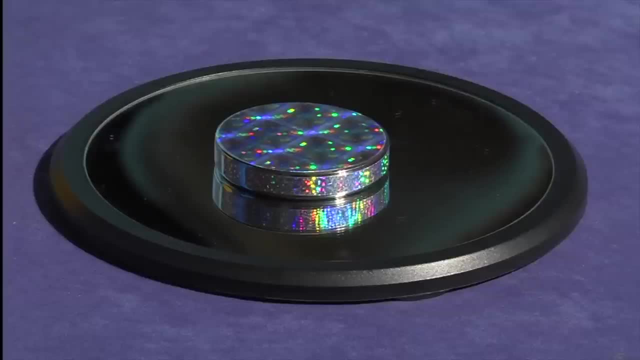 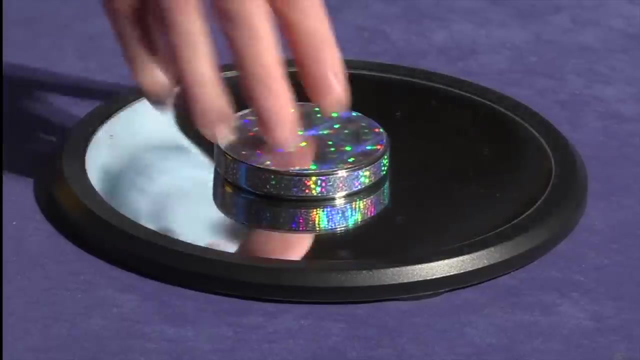 and he worked out what it was doing, and in his autobiography he points out that it broke through in his thoughts and ideas that led to his Nobel Prize. so what I want to do now is to show you a simple toy, and it's this thing here. it just consists of a 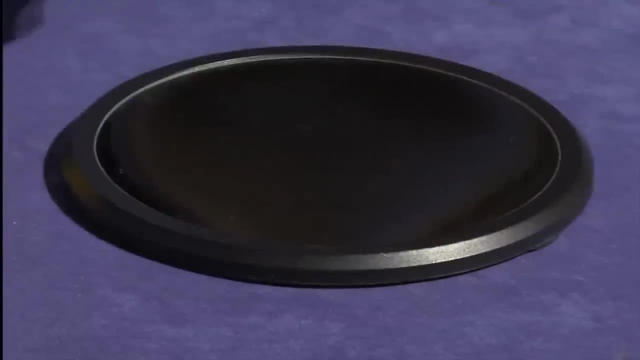 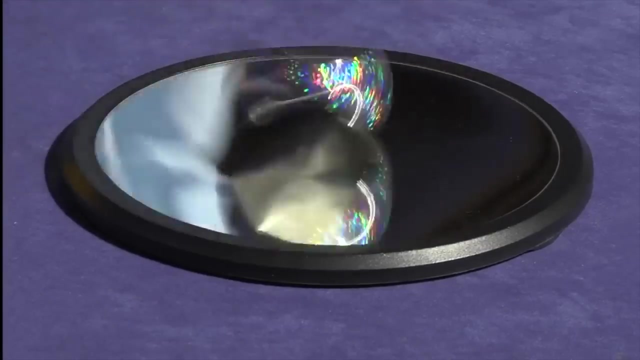 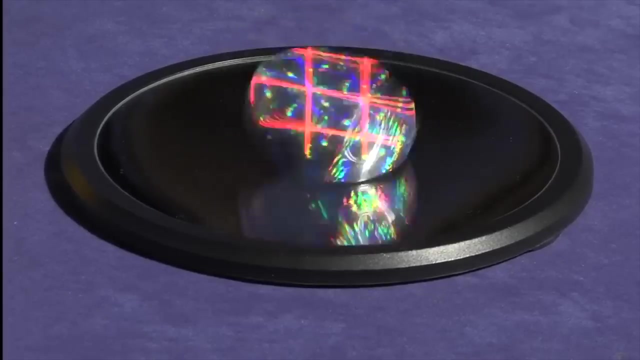 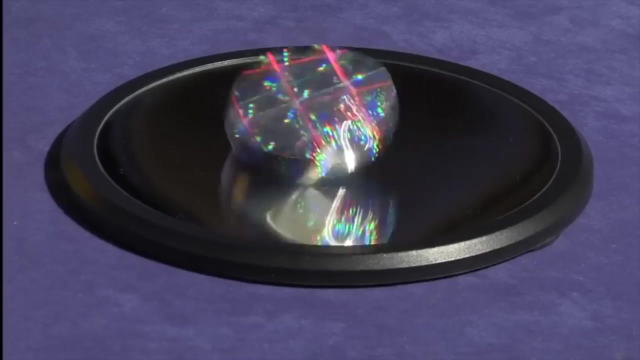 heavy disk and just a plate to put it on, and I'm going to spin it now and hopefully the camera will. okay, it's now spinning and you can do this at home with a dinner plate. okay, do it on the floor and the way in which it gets. 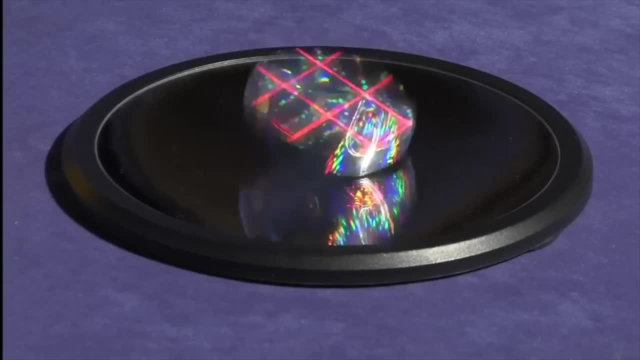 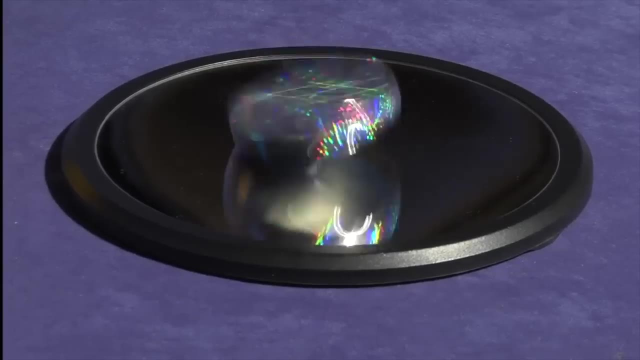 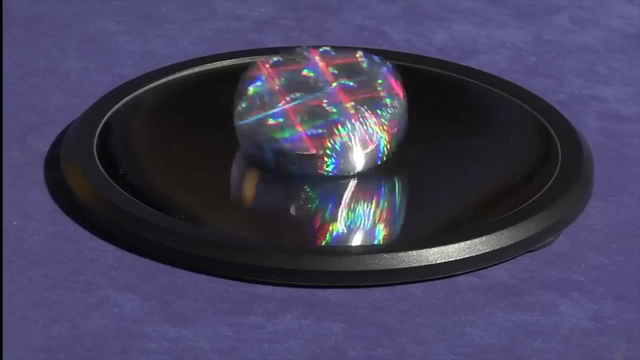 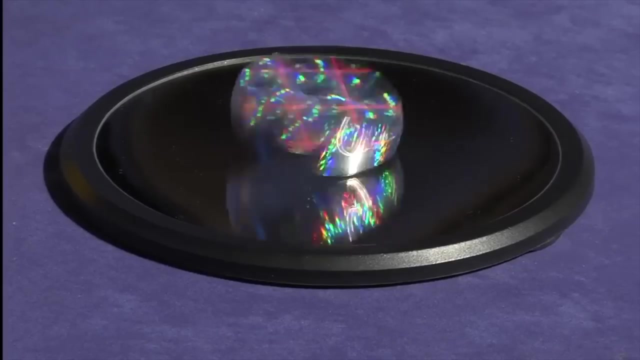 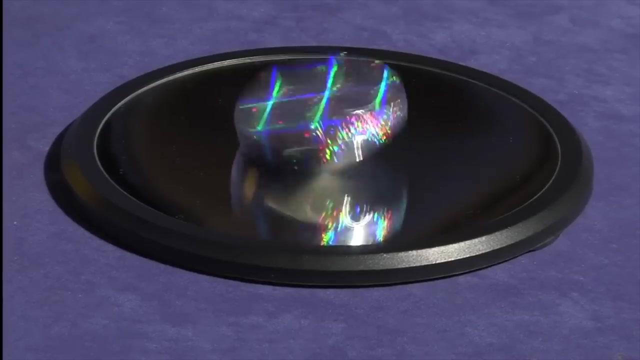 faster and faster. the rate of change of it is the same rate of change form as the merger of two black holes or two white walls put together. so it's going faster and faster and faster, and and and. it takes a long time, but when you do the plate on the floor, 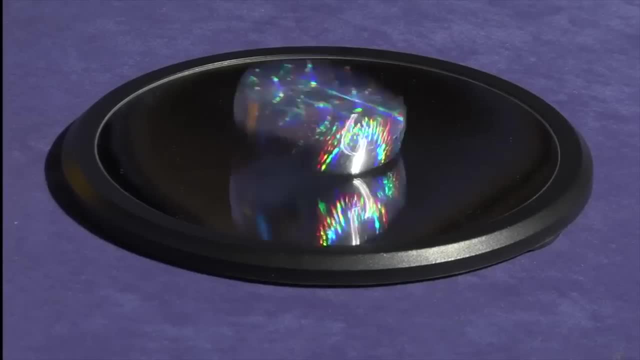 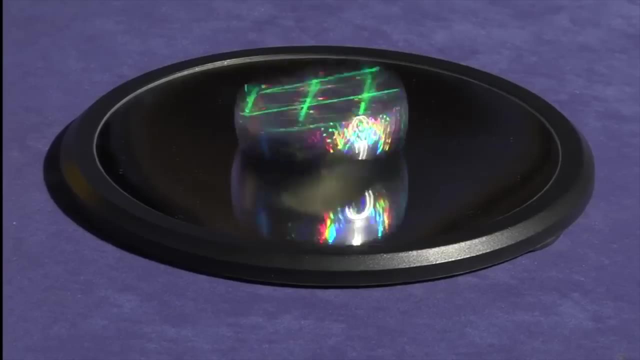 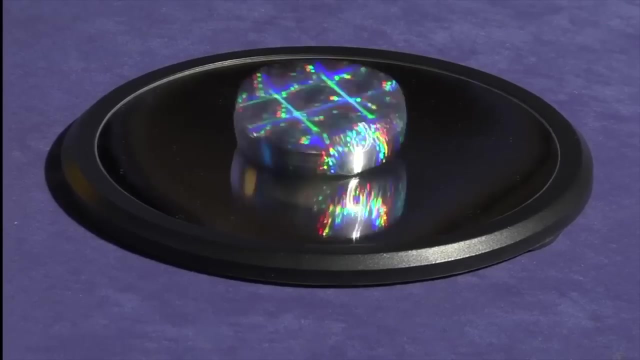 don't worry, it will happen quickly and you'll do it again because you realise you had the plate the long way round and this will end. that will be the end of the lecture. 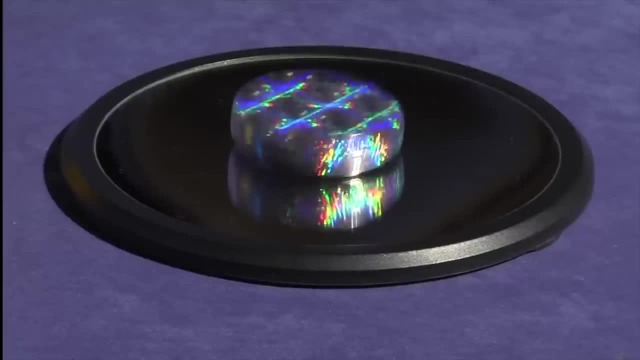 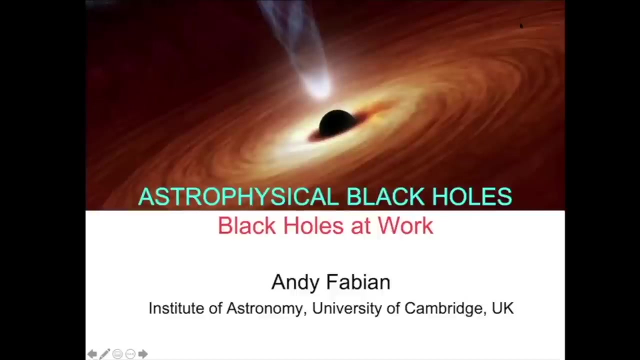 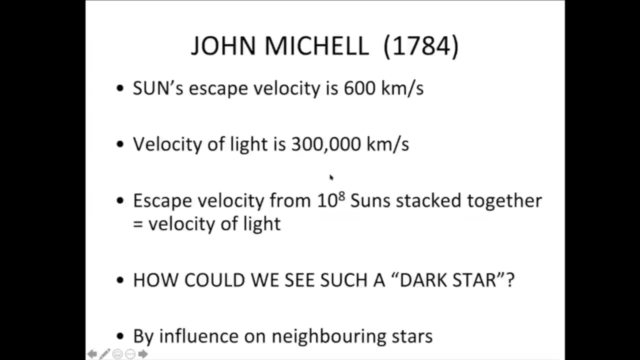 here in Cambridge. He went through a lot of simple physics to work this out, and you can do it yourself on the back of an envelope, but essentially the sun's escape velocity is 600 kilometers per. 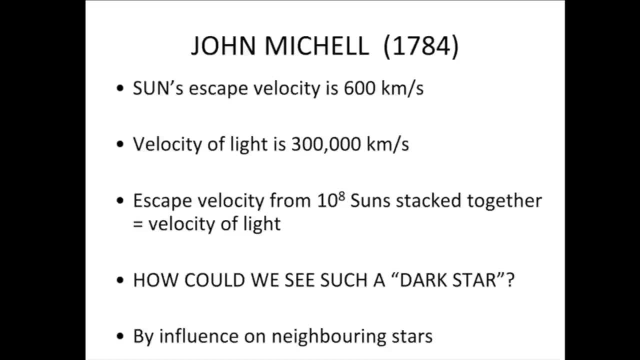 second, The escape velocity is what velocity you would need to shoot matter out if it was to escape from the sun's gravitational field altogether. So the escape velocity for the sun is 600 kilometers per second. Velocity of light is 300,000 kilometers per second, and I'm using modern numbers here, but 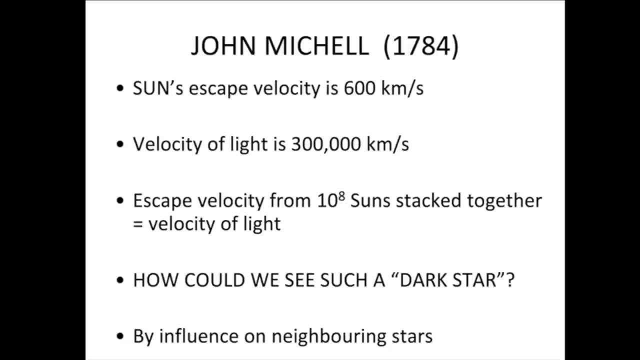 the numbers he used were not that different. This means that if you were to stack 100 million suns together, so- and don't ask me how you do it, but imagine you could- then what happens is the escape velocity. using Newtonian gravity, the escape velocity would then equal the velocity of light. 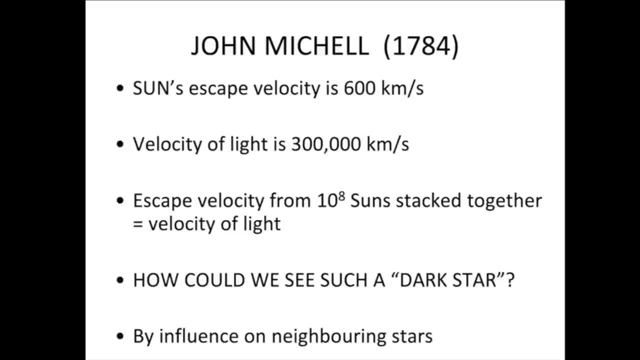 If you make an object more massive and compact, the escape velocity goes up and up, and so you get where the velocity of light is the value of this escape velocity from this object. Therefore, he concluded that Leinic could not escape from this object and therefore we wouldn't be able to see it. 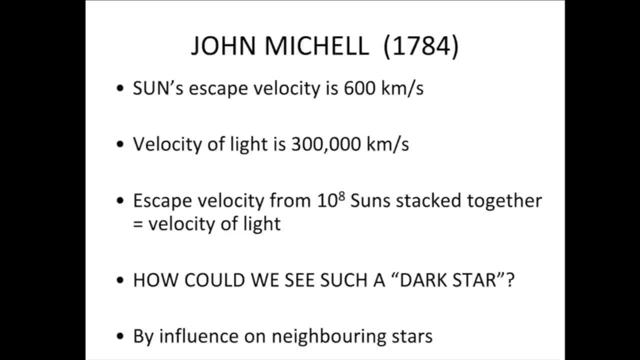 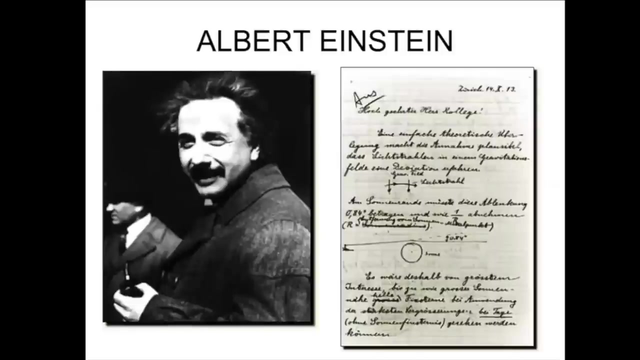 and he considered: how could we see such a dark star? and he suggested it would be by its influence, its gravitational influence. In other words, nearby objects would be gravitationally perturbed by this object and that's how we would infer that it's there. So this was a great idea. The next real step in black holes was with Albert. 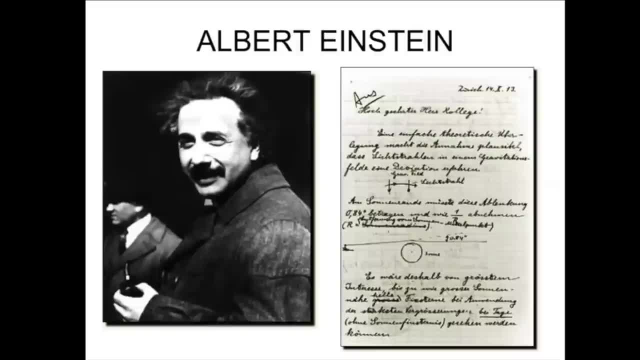 Einstein and his general theory of relativity. I've got here just a simple copy of a letter he wrote in 1913. It was 14th of October. It's soon going to be the 14th of October 2000, but this was over a hundred. 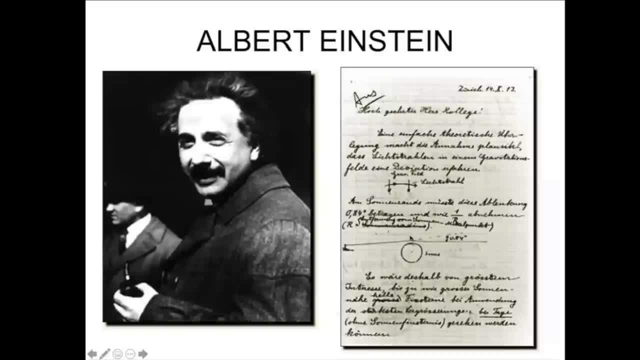 years ago, and you can see there he's musing about what happens if we have the sun. That's Zona, so that's the sun. An array of light that goes close to the sun is deflected by the gravitational field of the sun. It's deflected here by 0.8 arc, seconds of arc, and he's getting deflected. 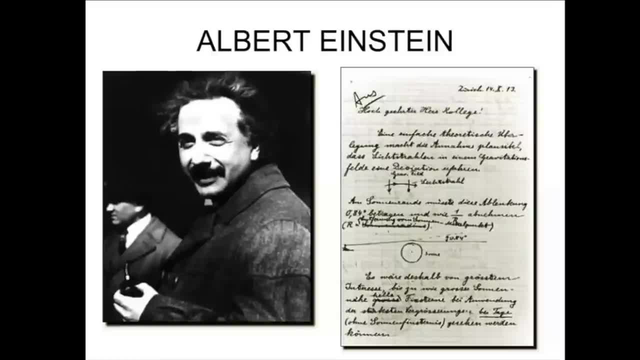 He's concluding that, basically, gravity, the gravitational field of the sun, would cause a light ray, which normally travels in a straight line, would perturb it and curb it downwards. Now it turns out he's got the wrong answer here Within a couple of years. 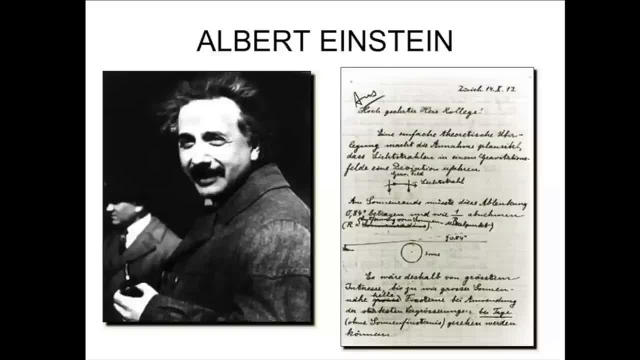 after writing this letter he'd come up to his general theory of relativity. and in that general theory of relativity he gets in fact a number which is twice that value. and actually the deflection of light by the sun was first measured in 1919 in a famous eclipse. 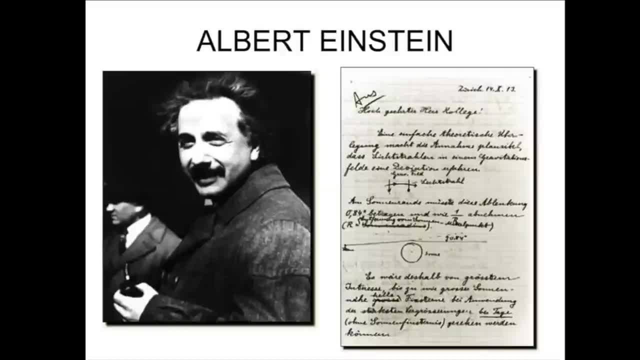 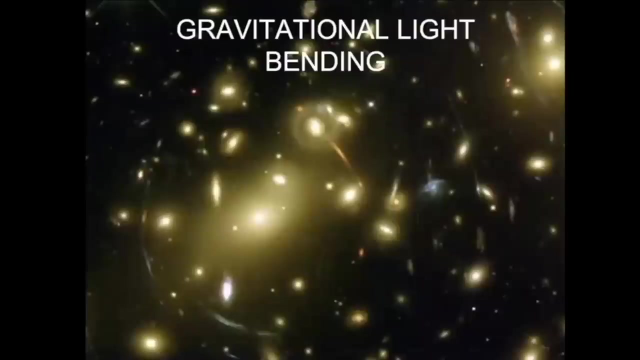 expedition led by Arthur Eddington, also from Cambridge, and that discovery of the bending of light by the sun was what really made Albert Einstein famous and also made people realise that general relativity is probably going to be our explanation of gravity. So what the general theory proposes is that basically, matter perturbs space-time- not just space as we can see with deflection of light, but it also perturbs the time, and we can then, just to show you now what we know about bending of light. this is a picture of a distant cluster of galaxies where there's a very large aggregation of mass in a relative distance from each other. 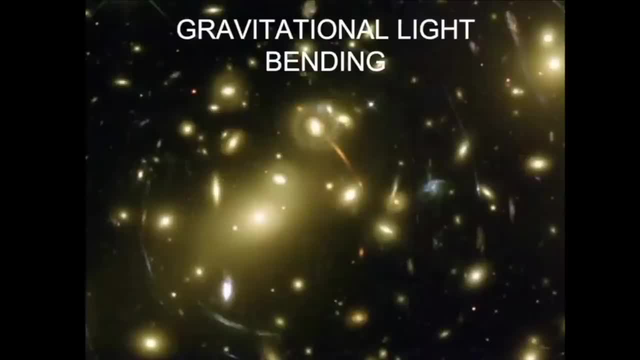 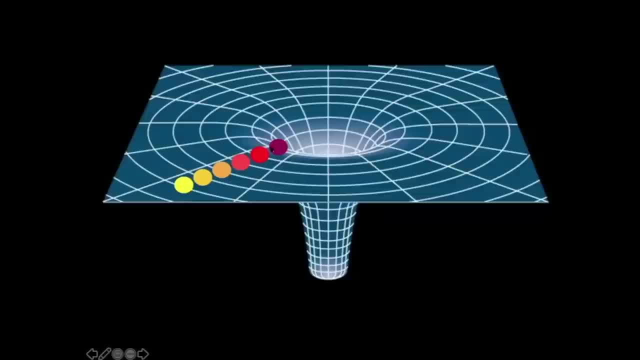 This is a picture of a distant cluster of galaxies where there's a very large aggregation of mass in a relative distance from each other. we would see the clock appear to slow down and it would turn redder until we couldn't see it. and essentially what happens is that if you throw things into 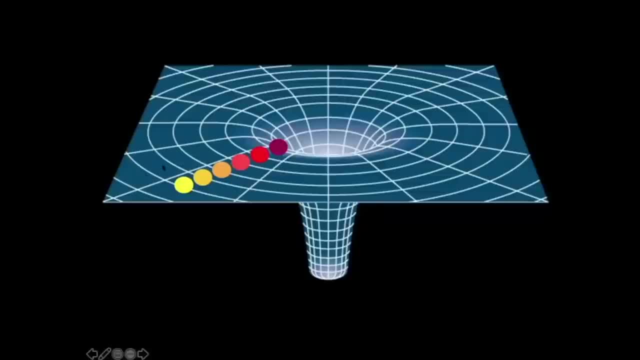 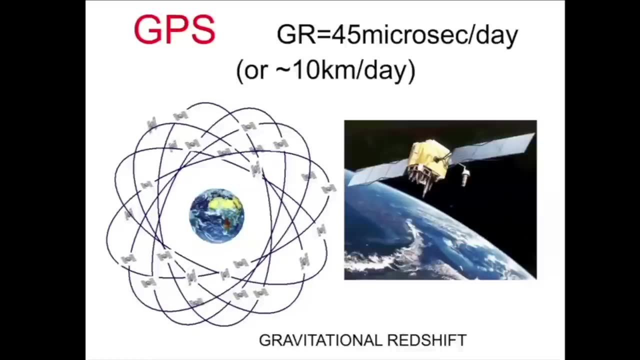 black holes. they would vanish from view as they approach the event horizon. now, this so-called gravitational redshift is something that's around, even around the earth and around any mast. and, in terms of the earth, the GPS satellites, the ones that give the signals for a sat-nav. they are orbiting the earth and they're 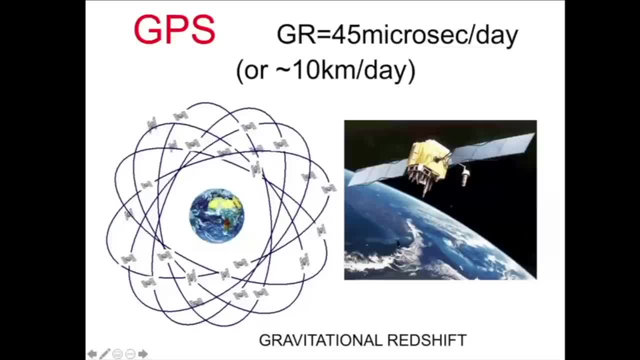 essentially very good clocks which your sat-nav detects signals from, and it's all working in terms of clocks and timing. now it turns out- because that's above the earth's surface, then the grab- that there's a gravitational redshift between it and the surface of the earth. if you were at the satellite, it would appear, looking down at the 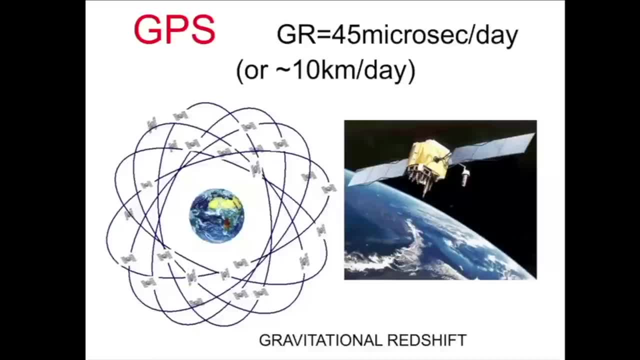 earth, as though Earth's clocks are running slightly slow and similarly, if we look at that satellite clocks we would also expect there to be. they would appear to be running slightly fast. and there's a correction has to be applied, and it's applied by your sat-nav. the correction is: 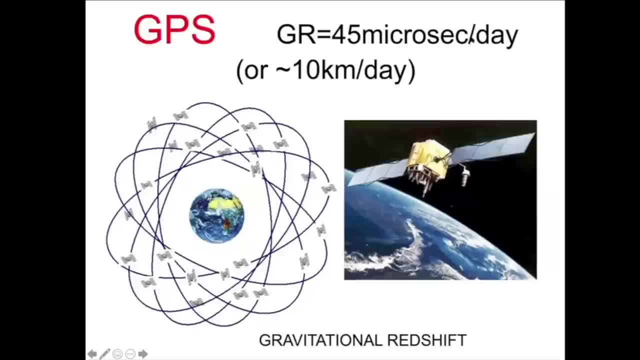 45 microseconds per day, which map might sound irrelevant, but in terms of if you drive around, it would correspond to an error of 10 kilometers per day and that is unacceptable with a sat-nav. so these corrections, general relativity, is corrected for within a sat-nav so that this is just the time effect that we 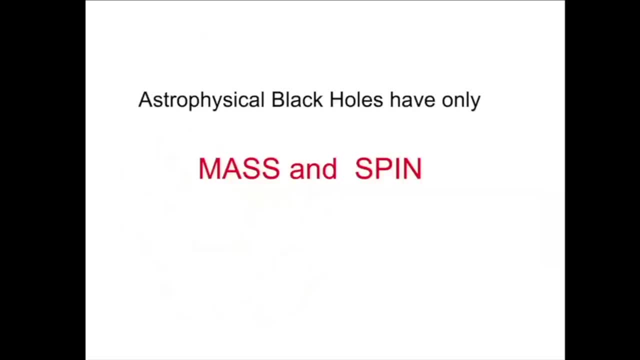 we've got there now. astrophysical black holes have only got mass and spin. the event horizon is three kilometers per solar mass. the known black holes, the known astrophysical black holes, are either of stellar mass somewhere between three and a hundred and fifty solar masses, or there's synchromasses between. 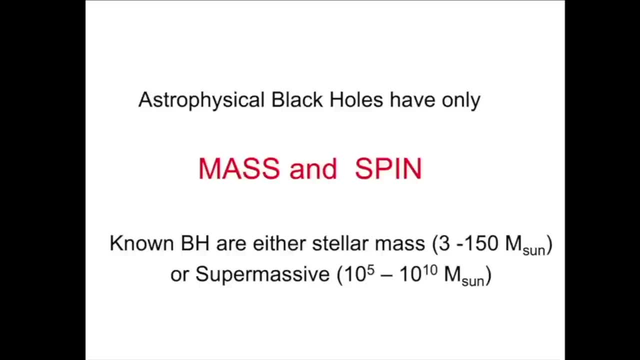 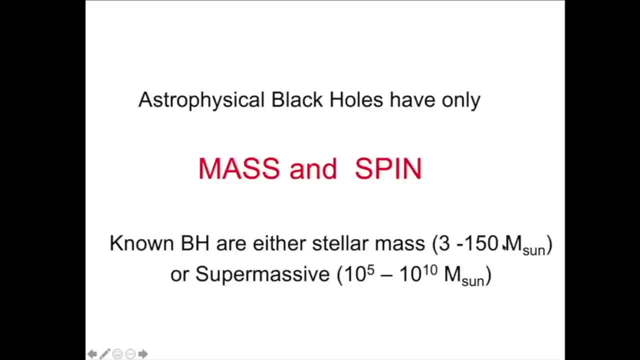 there are discussions about ones below that limit. the hundred and fifty solar limit, the hundred and fifty solar mass comes from gravitational wave work. that mass comes from gravitational wave work. that I'll just touch on at the end. and three, I'll just touch on at the end, and three solar masses. well, uncertainties there. 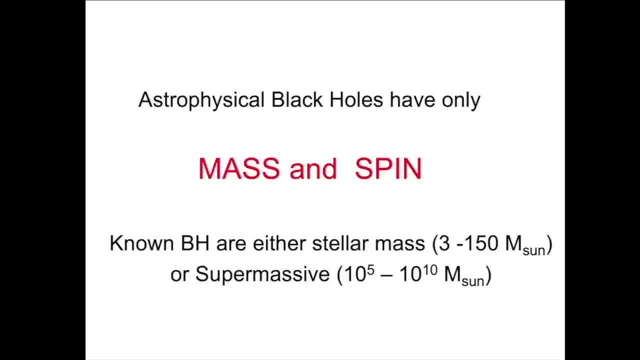 solar masses. well, uncertainties there there may be. they may exist outside there may be. they may exist outside those ranges, and people are very keen to those ranges and people are very keen to find ones in between a hundred and fifty, find ones in between a hundred and fifty and a hundred thousand, but so far they've 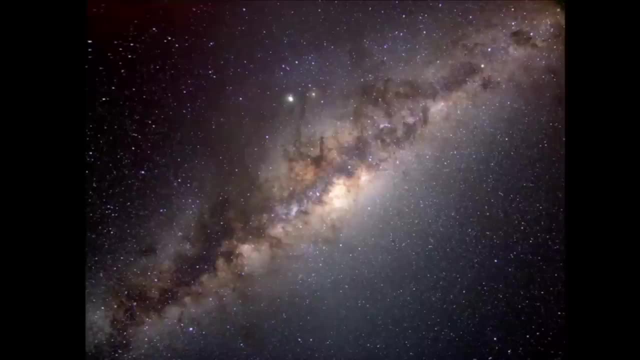 and a hundred thousand, but so far they've not been trapped. how do we know that the not been trapped? how do we know that the black holes are there? how do we observe black holes are there? how do we observe well, the best observed object best well, the best observed object, best observed black holes in terms of 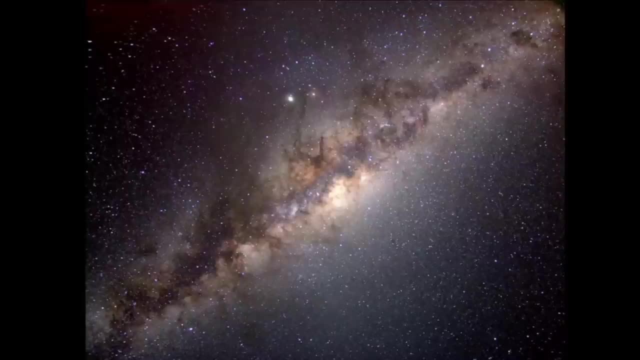 observed black holes. in terms of measuring its mass and properties, is the measuring its mass and properties is the one at the center of our galaxy, this one at the center of our galaxy, this lovely picture of the Milky Way, showing lovely picture of the Milky Way, showing the center of the mid Milky Way and the. 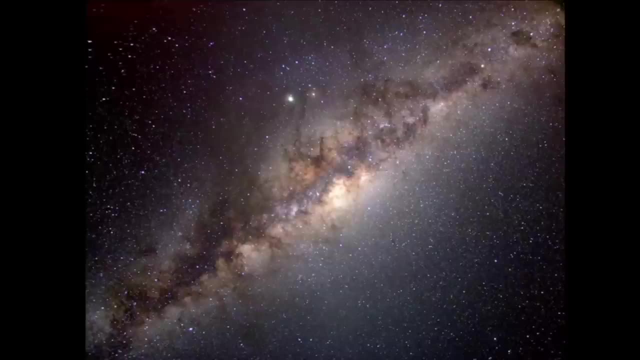 the center of the mid Milky Way and the constellation of Sagittarius shows you. constellation of Sagittarius shows you where we need to look. we need to look where we need to look. we need to look right in the center of our galaxy, right in the center of our galaxy. remember that we live in a 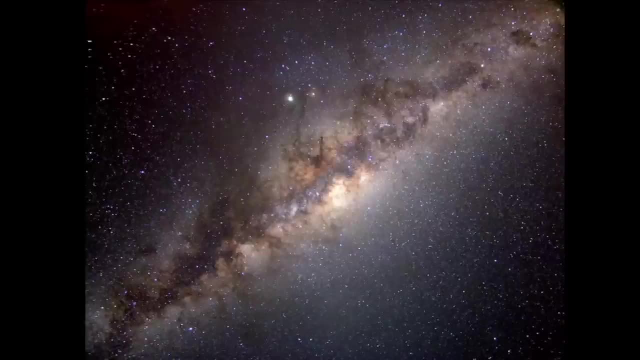 remember that we live in a spiral galaxy. we're all orbiting around that spiral galaxy. we're all orbiting around that galaxy, the center of the galaxy, at galaxy, the center of the galaxy, at around 220 kilometers per second. we go around 220 kilometers per second. we go around the earth at 30 kilometers per 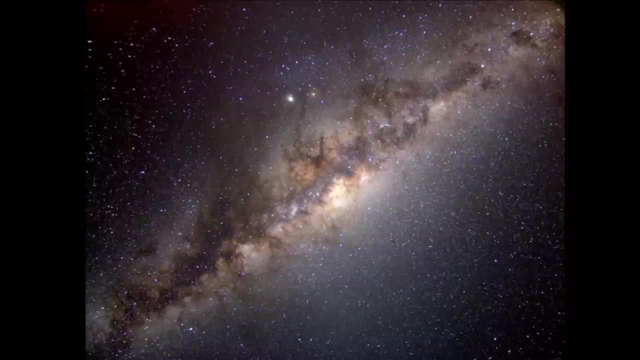 around the earth at 30 kilometers per second and we go around the center of second and we go around the center of the galaxy at 220 kilometers per second. the galaxy at 220 kilometers per second, and virtually all of these stars are, and virtually all of these stars are doing the same as well. we're all. 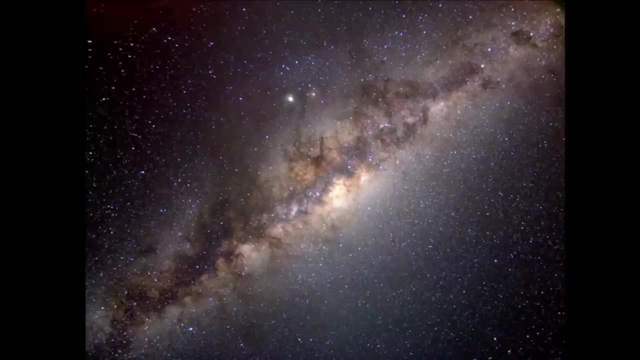 doing the same as well. we're all flattened into a disk. now we can't see flattened into a disk. now we can't see into the center because of all these into the center, because of all these desk clouds. but, as in Avena's talk, the 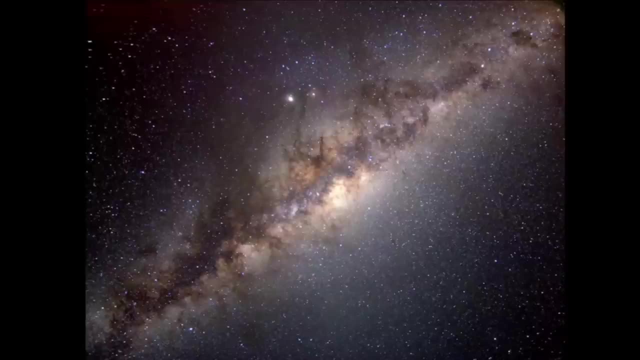 desk clouds. but, as in Avena's talk, the we've just heard, if you go into the we've just heard, if you go into the infrared, you can see through the dust infrared, you can see through the dust and that's what astronomers have been and that's what astronomers have been doing over the last 20 to 30 years. and 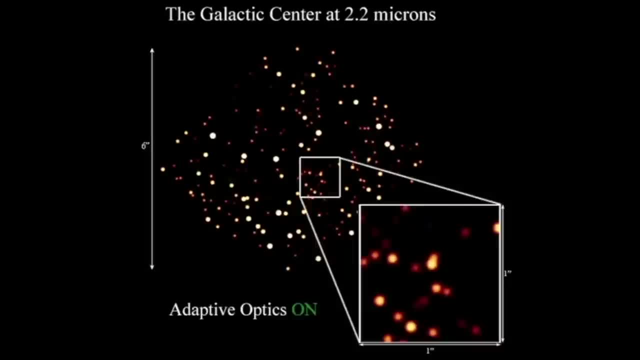 doing over the last 20 to 30 years, and this is what the galactic center looks. this is what the galactic center looks like at 2 microns. that's the wavelength like at 2 microns. that's the wavelength. I'm talking about what they've got there. 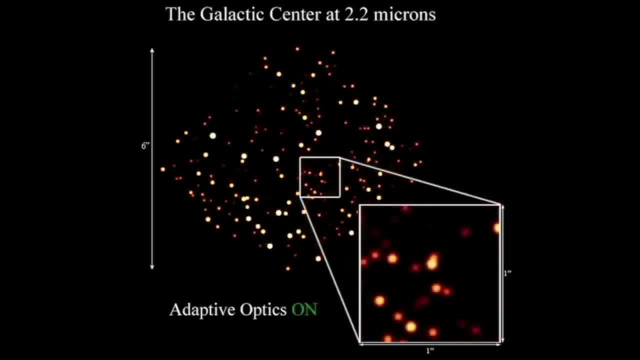 I'm talking about what they've got there is using adaptive optics, where what is using adaptive optics, where what you've got to do is take out the sort of. you've got to do is take out the sort of twinkling, that effect that our twinkling, that effect that our atmosphere causes on. 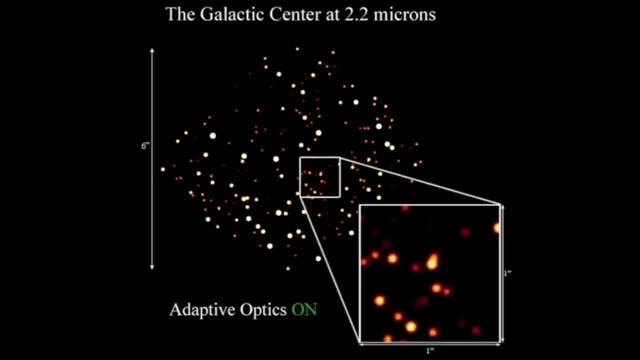 atmosphere causes on atmosphere causes on light from distant objects. you're all light from distant objects. you're all light from distant objects. you're all familiar with looking at stars and them familiar with looking at stars and them familiar with looking at stars and them twinkling. that twinkling effect is due. 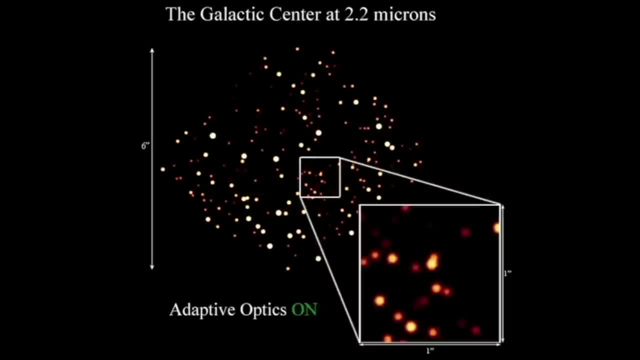 twinkling. that twinkling effect is due twinkling, that twinkling effect is due to the Earth's atmosphere and due to to the Earth's atmosphere and due to to the Earth's atmosphere and due to different patches of the atmosphere, different patches of the atmosphere, different patches of the atmosphere being at different temperatures, is 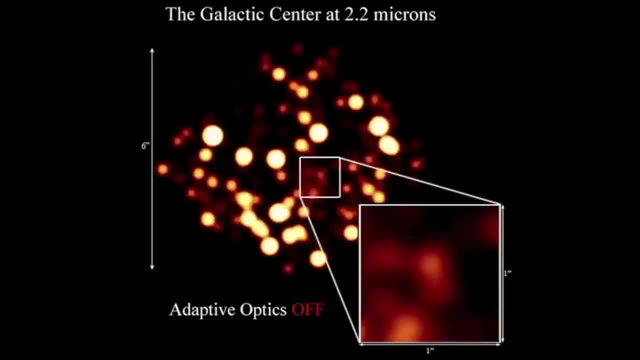 being at different temperatures is. being at different temperatures is differential refraction. you've got to try differential refraction. you've got to try differential refraction. you've got to try and get rid of that. they do that using. and get rid of that. they do that using. 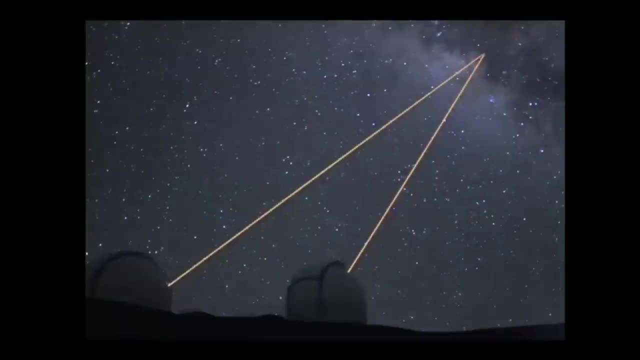 and get rid of that. they do that using adaptive optics. one way to do that is adaptive optics. one way to do that is adaptive optics. one way to do that is is to create an artificial star in your is, to create an artificial star in your is to create an artificial star in your observing field, and then you correct your. 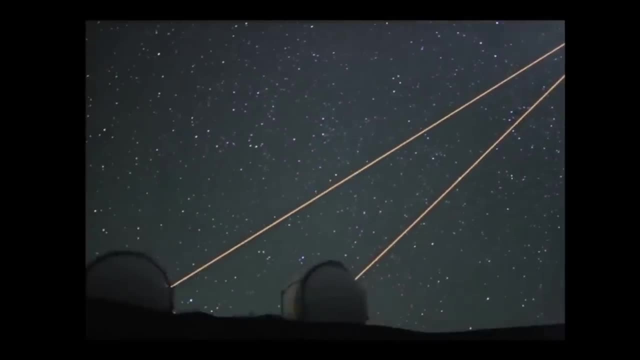 observing field, and then you correct your observing field, and then you correct your telescope to make the artificial star telescope, to make the artificial star telescope, to make the artificial star perfectly round and small, and then perfectly round and small, and then perfectly round and small, and then you'll correct everything else in the 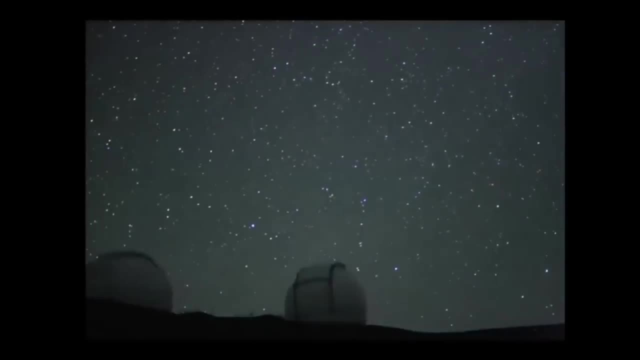 you'll correct everything else in the. you'll correct everything else in the field and to make the artificial star field and to make the artificial star field and to make the artificial star. you can use your telescope, you've got in. you can use your telescope, you've got in. 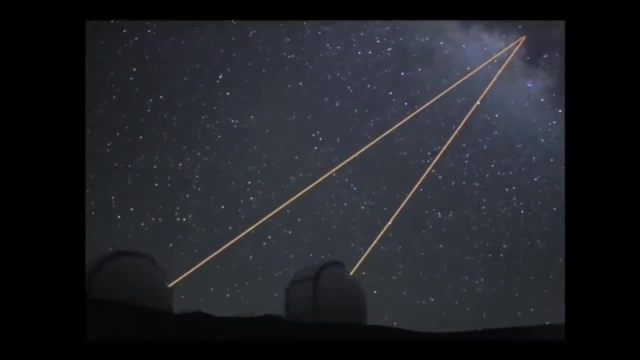 you can use your telescope. you've got in your telescope. have a laser beam that is your telescope. have a laser beam that is your telescope. have a laser beam that is shining up and at an altitude of about shining up and at an altitude of about shining up and at an altitude of about 70 kilometers. 70 kilometers it can cause. 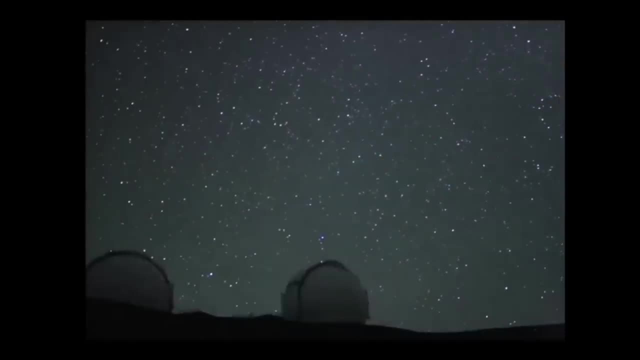 70 kilometers, 70 kilometers. it can cause 70 kilometers, 70 kilometers. it can cause fluorescence sodium, fluorescence in the fluorescence sodium, fluorescence in the fluorescence sodium, fluorescence in the very upper atmosphere and create the very upper atmosphere and create the very upper atmosphere and create the artificial star. so that's these. 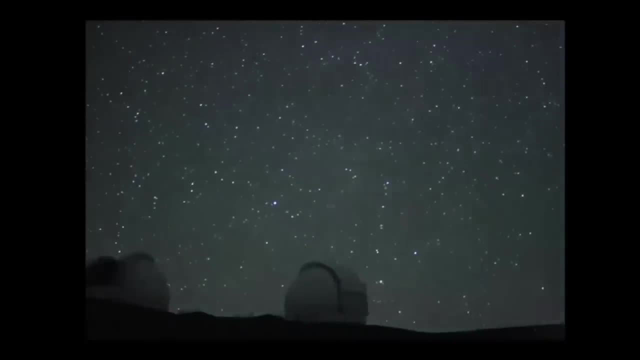 artificial star. so that's these artificial star. so that's these astronomers here are that's not looking astronomers here are that's not looking astronomers here are that's not looking at the galactic center, but they're now at the galactic center, but they're now. 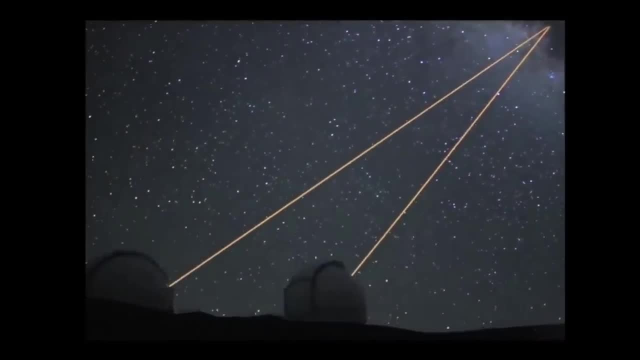 at the galactic center. but they're now looking at the galactic center and they looking at the galactic center, and they looking at the galactic center and they are going to make this artificial star, are going to make this artificial star, are going to make this artificial star and enable adaptive optics to make this. 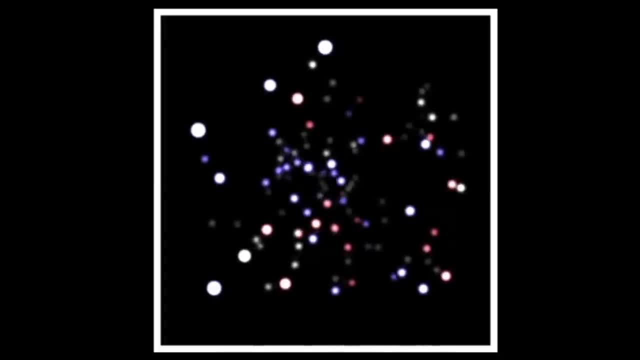 and enable adaptive optics to make this and enable adaptive optics to make this correction, and what has come out of correction and what has come out of correction and what has come out of looking at this over 30 years is a. looking at this over 30 years is a. 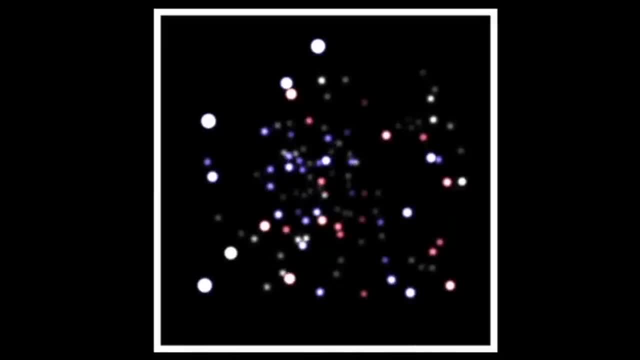 looking at this over 30 years, is a total image like this is: this is total image. like this is: this is total image. like this is: this is computer-generated and you're seeing 30 computer-generated and you're seeing 30 computer-generated and you're seeing 30 years worth of movement. what they saw, 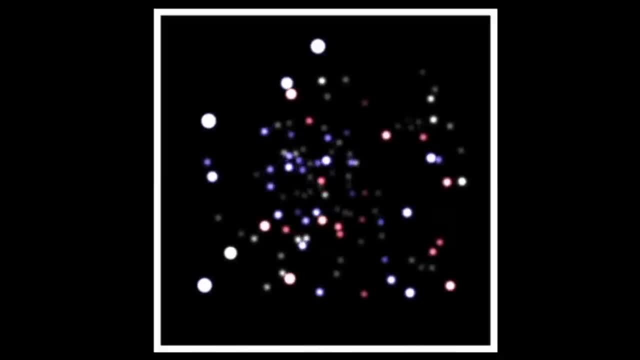 years worth of movement. what they saw: years worth of movement. what they saw was the fact that the stars near the was the fact that the stars near the was the fact that the stars near the center are moving. look at this star here. center are moving. look at this star here. 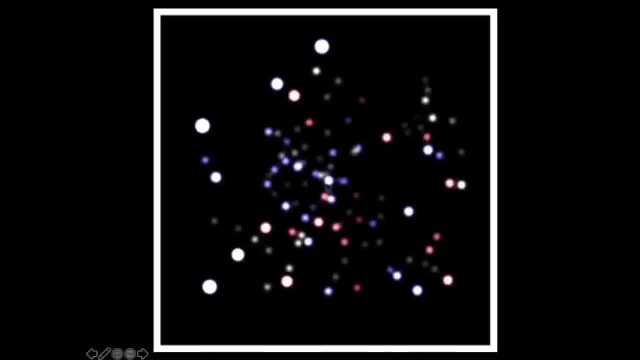 center are moving. look at this star here. you see how it's swinging round and you see how it's swinging round and you see how it's swinging round and going fast there. there's obviously going fast there. there's obviously going fast there. there's obviously something here, just about there, which 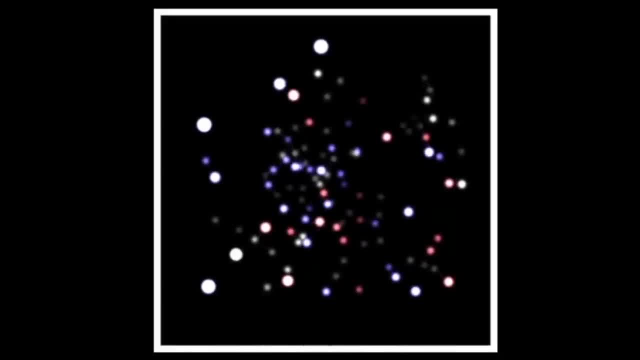 something here, just about there, which something here, just about there, which things are swinging round, yet you can't. things are swinging round, yet you can't. things are swinging round, yet you can't see it. this is the black hole at the. see it, this is the black hole at the. 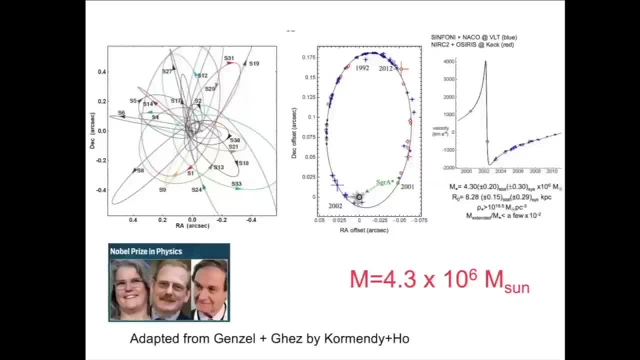 see it, this is the black hole at the center of our galaxy and this was what center of our galaxy and this was what center of our galaxy, and this was what was awarded. the Nobel Prize in physics was awarded. the Nobel Prize in physics was awarded the Nobel Prize in physics. last week, the Nobel Prize in physics went. 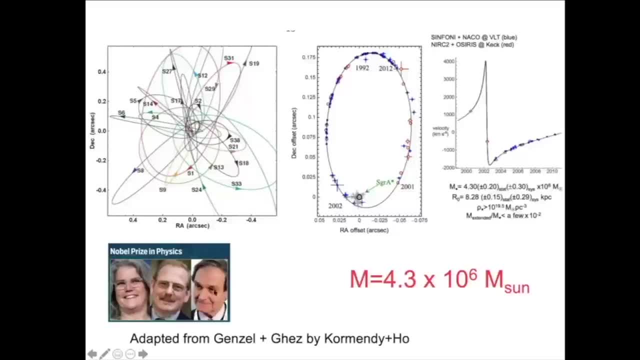 last week the Nobel Prize in physics went. last week the Nobel Prize in physics went to Andrea gets Reinhardt Gensel and to Andrea gets Reinhardt Gensel and to Andrea gets Reinhardt Gensel and Roger Penrose. he's a mathematical, Roger Penrose, he's a mathematical. 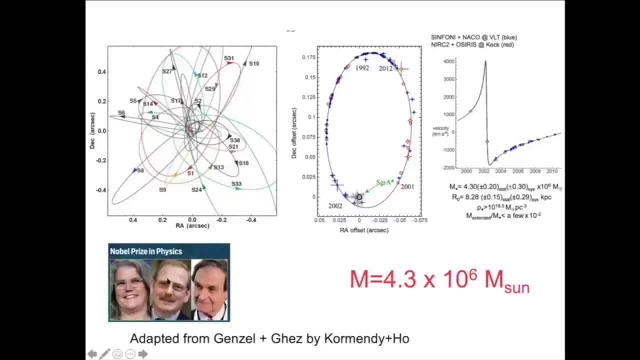 Roger Penrose. he's a mathematical physicist in Oxford. Reinhardt is at physicist in Oxford. Reinhardt is at physicist in Oxford. Reinhardt is at Munich and Andrea's Los Angeles and Munich and Andrea's Los Angeles, and Munich and Andrea's Los Angeles- and they were using these two are the. 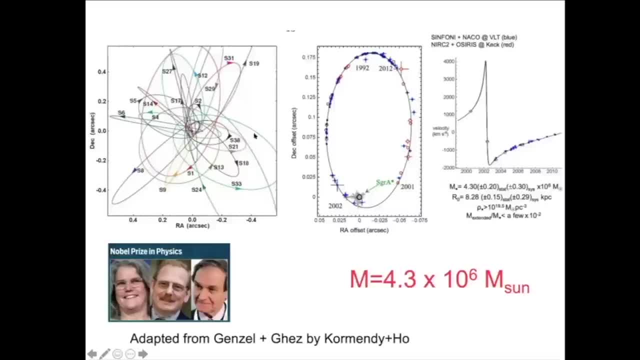 they were using. these two are the they were using. these two are the observers who came up with results. such observers who came up with results. such observers who came up with results such as shown here. these are the orbits of observers who came up with results such as shown here. these are the orbits of 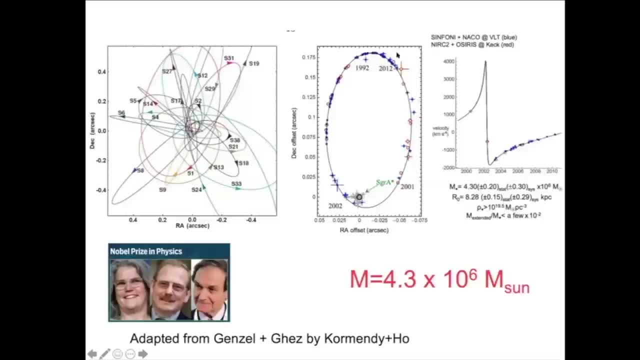 observers who came up with results such as shown here. these are the orbits of the stars around the black hole. and here's the stars around the black hole. and here's the stars around the black hole. and here's that s2 star I showed you going round in. 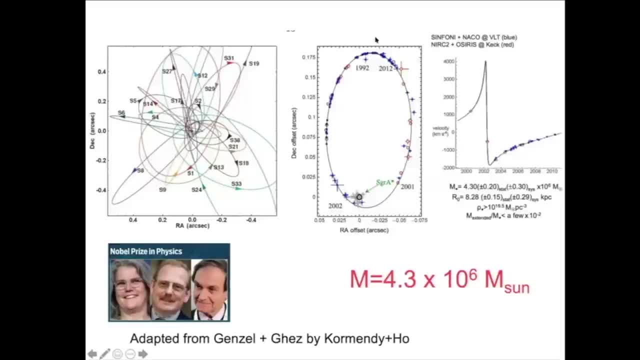 that s2 star. I showed you going round in that s2 star. I showed you going round in a 16-year orbit and here is the orbit, a 16-year orbit, and here is the orbit, a 16-year orbit, and here is the orbit there, and this is the focus of the orbit. 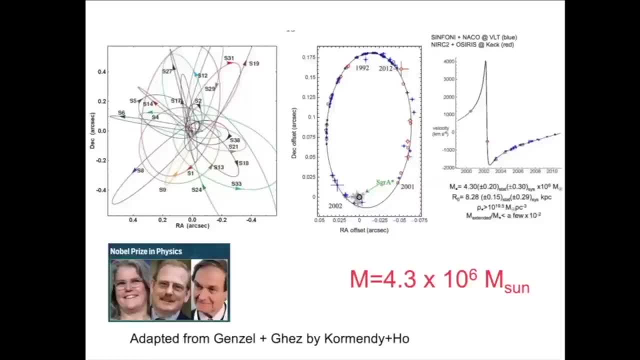 there and this is the focus of the orbit there, and this is the focus of the orbit. that's where Sajay star it's. that's the. that's where Sajay star it's, that's the. that's where Sajay star it's. that's the object to the center. that's coincident. 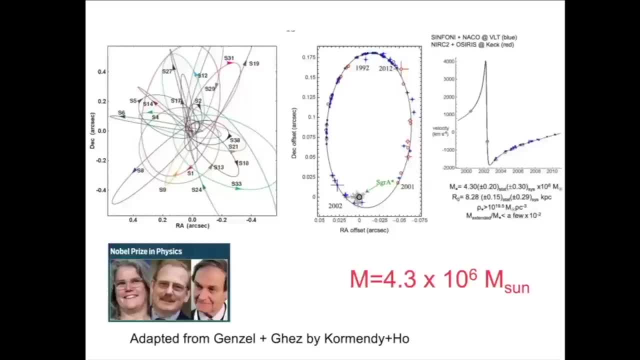 object to the center. that's coincident. object to the center: that's coincident, and, and you can also see it flickering, and. and you can also see it flickering, and. and you can also see it flickering in the x-ray band, but it's not always. 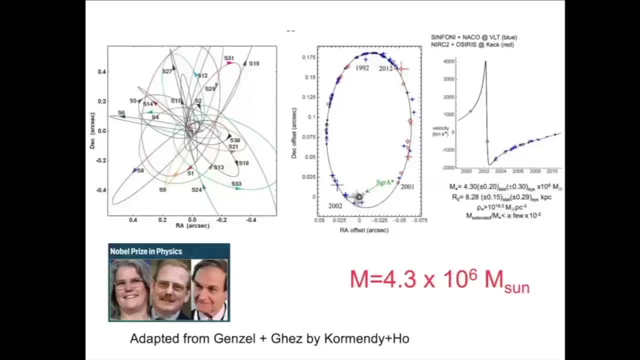 in the x-ray band but it's not always in the x-ray band but it's not always flickering there and it's been known flickering there and it's been known flickering there and it's been known about for some years and its name is. 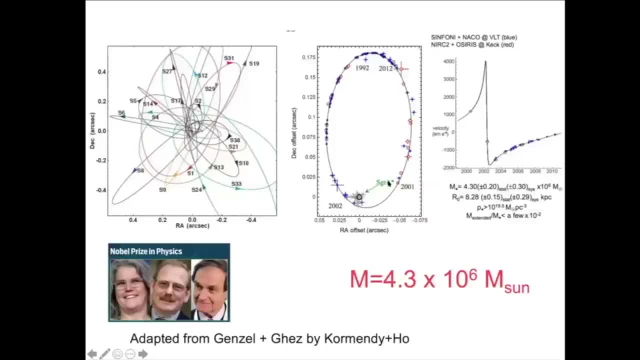 about for some years and its name is about for some years, and its name is: it's the radio source. a that means the it's the radio source. a that means the it's the radio source. a that means the brightest that will particular source in, brightest that will particular source in. 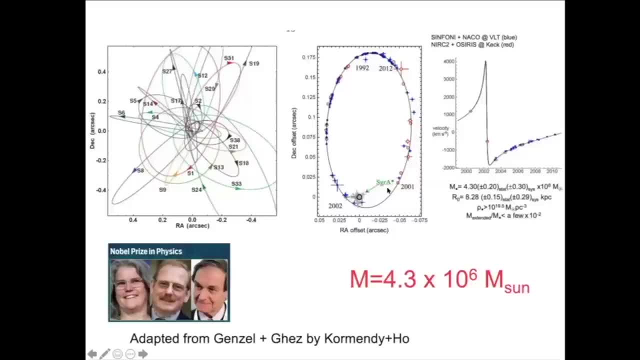 brightest that will. particular source in the constellation of Sagittarius and a. the constellation of Sagittarius and a. the constellation of Sagittarius and a star. because it's got something star. because it's got something star, because it's got something peculiar about it. now you can just use. 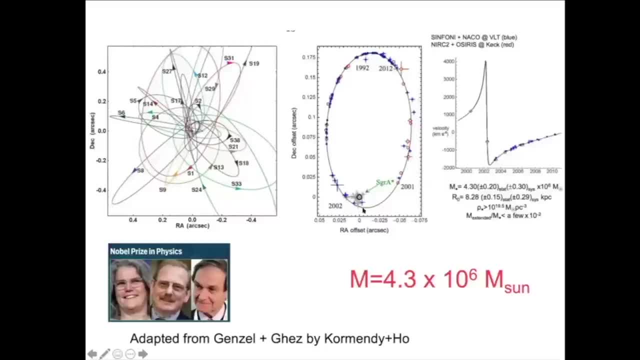 peculiar about it now. you can just use peculiar about it now. you can just use Newton's laws to solve the orbit and Newton's laws to solve the orbit and Newton's laws to solve the orbit and work out the mass of this object and it work out the mass of this object and it. 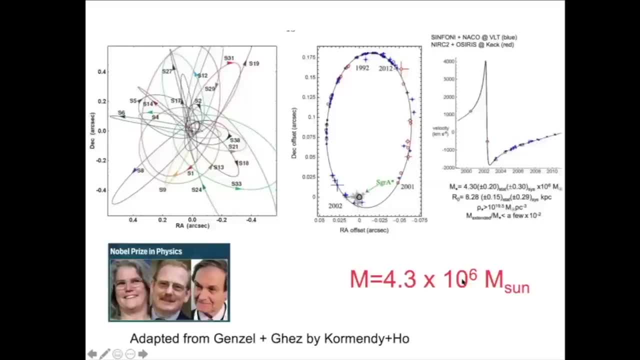 work out the mass of this object and it turns out to be 4.3 times 10 to the 6, turns out to be 4.3 times 10 to the 6, turns out to be 4.3 times 10 to the 6. solar masses: 4 million solar masses. and. 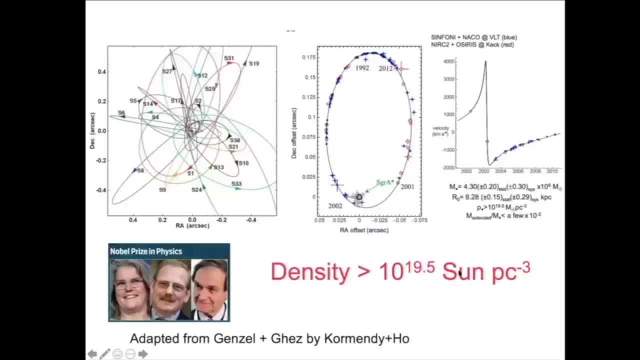 solar masses- 4 million solar masses. and solar masses- 4 million solar masses. and it's of course it there and you can also. it's of course it there, and you can also. it's of course it there and you can also work out from how good the orbit is. 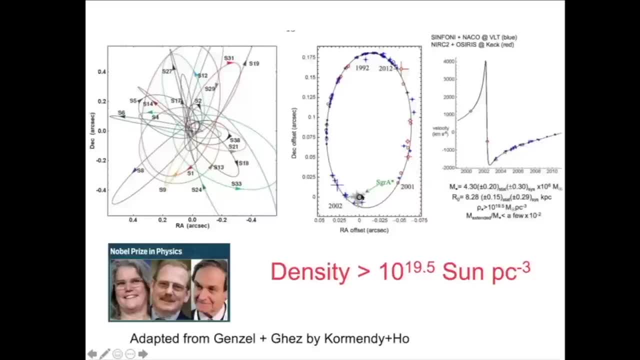 work out from how good the orbit is. work out from how good the orbit is around here. imagine that this is a around here. imagine that this is a around here. imagine that this is a distributed object. what is it the minimum distributed object? what is it the minimum? 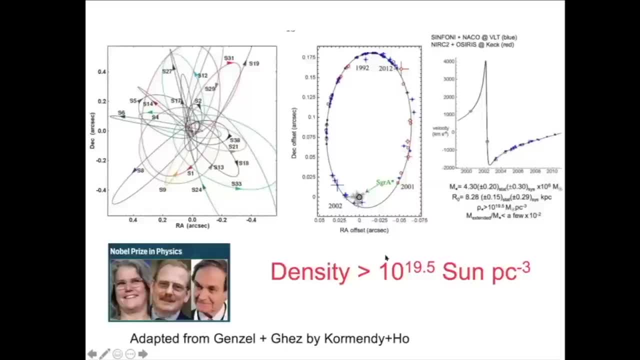 distributed. object: what is it? the minimum density it could have and that density density it could have, and that density density it could have, and that density turns out to be 10 to the 19 and a half turns out to be 10 to the 19 and a half. 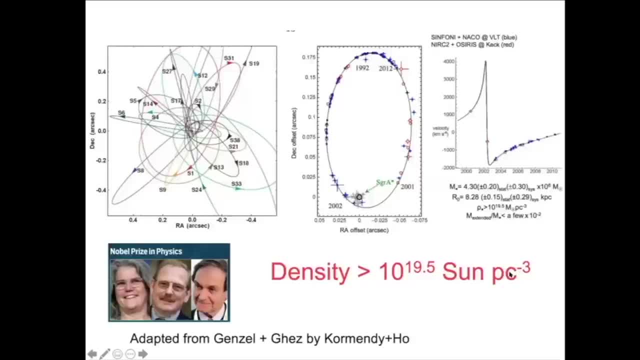 turns out to be 10 to the 19 and a half stars per cubic parsec. stars of the mass stars per cubic parsec. stars of the mass stars per cubic parsec. stars of the mass of the Sun. now that is a phenomenal of the Sun. now that is a phenomenal. 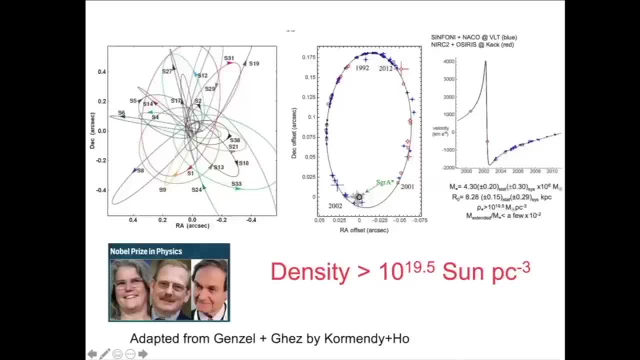 of the Sun. now that is a phenomenal density. remember the local density of density. remember the local density of density. remember the local density of stars around us is around 1 per 10 cubic stars around us is around 1 per 10 cubic stars around us is around 1 per 10 cubic parsecs. now, a parsec is an astronomical. 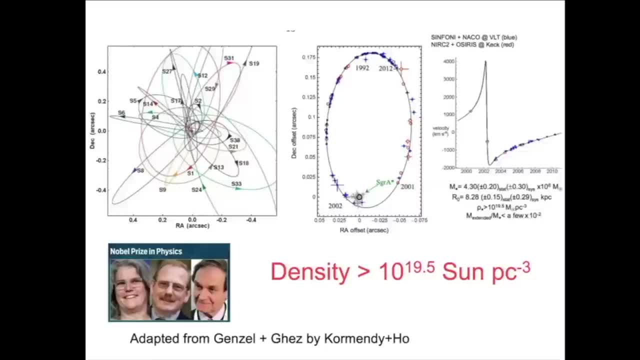 parsecs. now a parsec is an astronomical parsecs. now a parsec is an astronomical distance and it's roughly the distance distance and it's roughly the distance distance and it's roughly the distance to their nearest style and we are in a to their nearest style and we are in a. 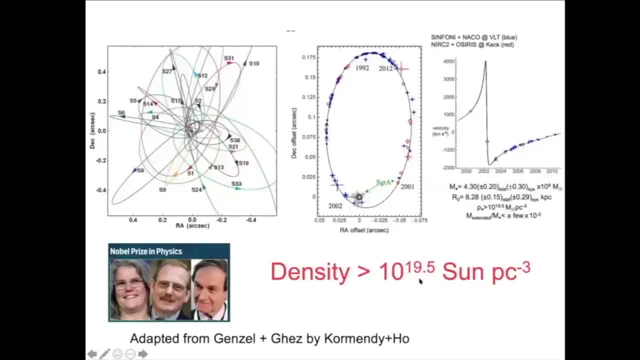 to their nearest style. and we are in a very isolated patch. so it's very, very isolated patch. so it's very, very isolated patch. so it's very difficult to think what else you could. difficult to think what else you could. difficult to think what else you could put there. indeed, you can't even put up. 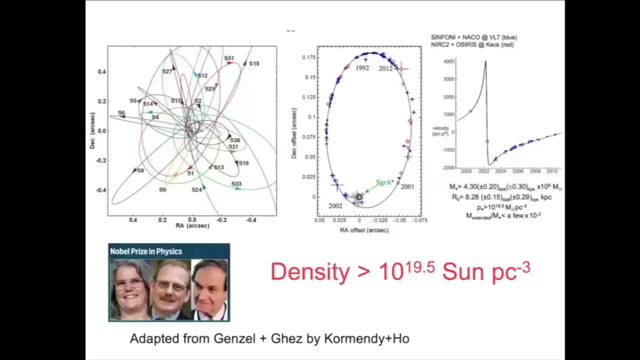 put there, indeed, you can't even put up. put there, indeed, you can't even put up- a ton of, can't put 20, 10 to the 20 a ton of. can't put 20, 10 to the 20 a ton of. can't put 20, 10 to the 20 neutron stars there, or anything like that. 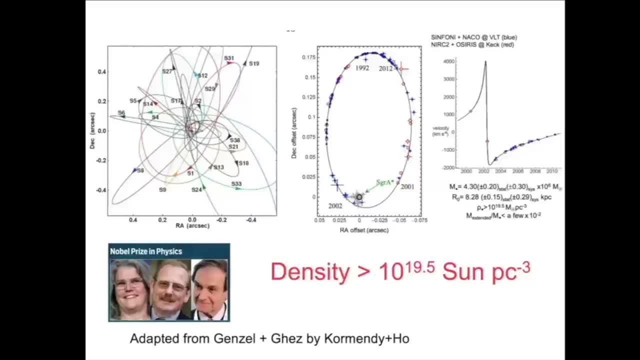 neutron stars there or anything like that. neutron stars there, or anything like that. they would all collide with each other. they would all collide with each other. they would all collide with each other and make a terrible mess- the only thing, and make a terrible mess, the only thing. 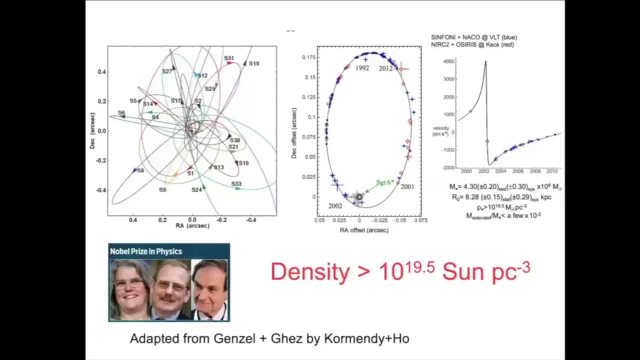 and make a terrible mess. the only thing known to physics that can't fit in there, known to physics that can't fit in there, known to physics that can't fit in there is a black hole and um, i just show that is a black hole and um, i just show that. 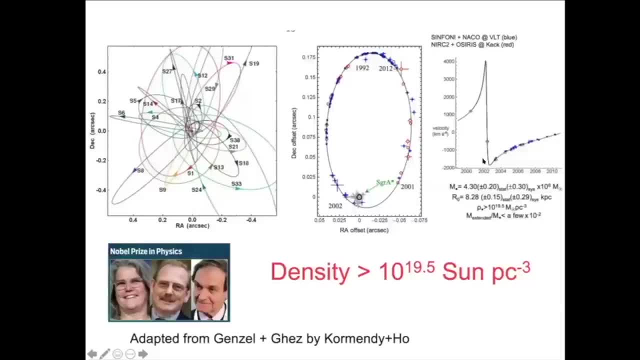 is a black hole and, um, i just show that plot. that's showing the velocity. you plot. that's showing the velocity. you plot that's showing the velocity you can measure from, can measure from, can measure from: spectroscopy: the velocity of the stars. spectroscopy: the velocity of the stars. 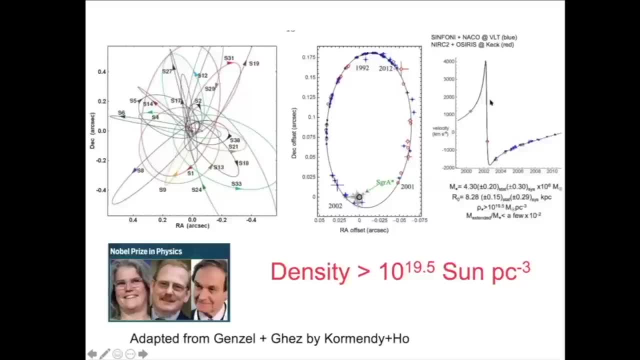 spectroscopy, the velocity of the stars and you can see the velocity of that and you can see the velocity of that and you can see the velocity of that particular star goes up to 4 000, and so particular star goes up to 4 000 and so. 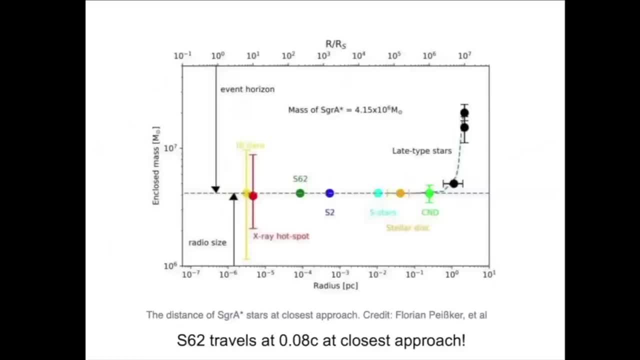 particular star goes up to 4 000 and so forth, forth, forth. back this august 2020, back this august 2020, back this august 2020. the group led by this person here, the group led by this person here, the group led by this person here, florian um found an inner star. 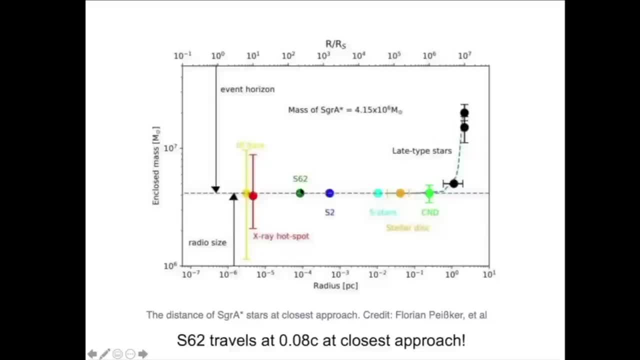 florian um found an inner star. florian um found an inner star. s62 was actually moving faster. s62 was actually moving faster. s62 was actually moving faster than the s2 star. s2 is here, than the s2 star. s2 is here, than the s2 star. s2 is here, a bit further out. this one's quite a bit. 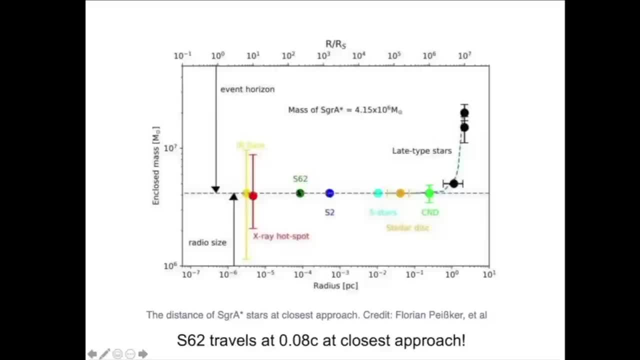 a bit further out. this one's quite a bit a bit further out. this one's quite a bit further closer into the black hole and further closer into the black hole, and further closer into the black hole, and at its close approach, closest approach, at its close approach, closest approach. 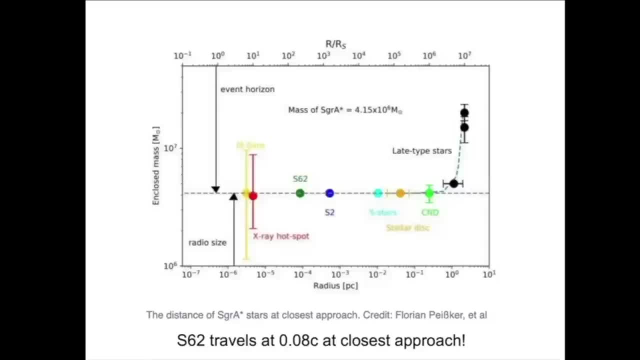 at its close approach, closest approach. it's traveling at eight percent of the. it's traveling at eight percent of the. it's traveling at eight percent of the speed of light. it's traveling at like speed of light. it's traveling at like speed of light. it's traveling at like 25 000 kilometers per second. 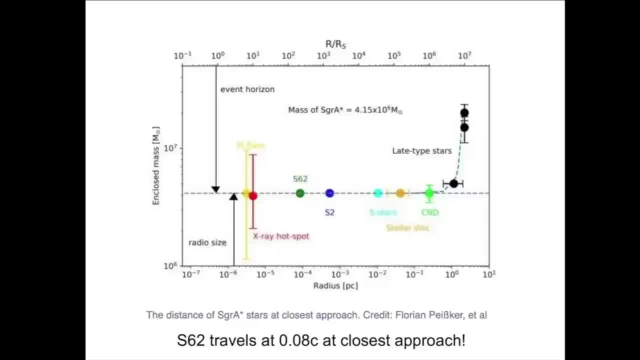 25 000 kilometers per second. 25 000 kilometers per second. so there's clearly something very so, there's clearly something very so, there's clearly something very special in the center of our galaxy, special in the center of our galaxy, special in the center of our galaxy. and this s62 star is pushing those. 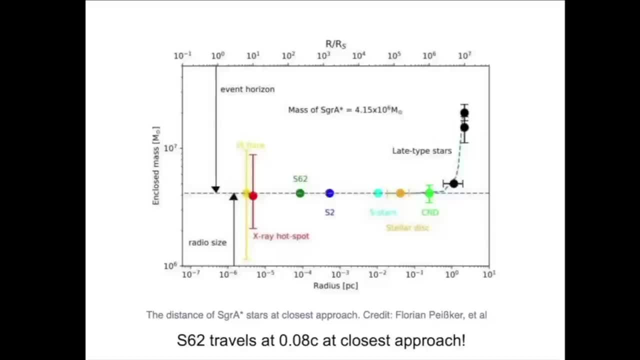 and this s62 star is pushing those, and this s62 star is pushing those densities up, densities up, densities up by a very large amount. i think there are by a very large amount, i think there are by a very large amount. i think there are basically very few physicists, and 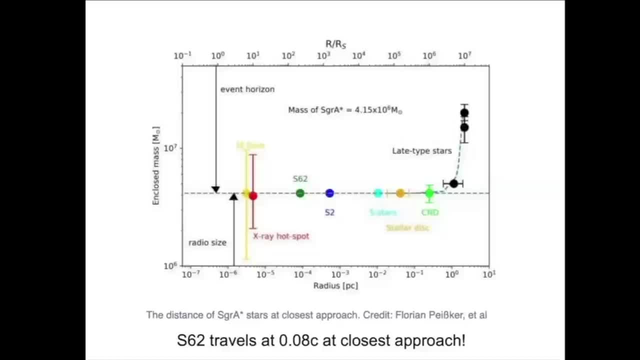 basically very few physicists, and basically very few physicists and astronomers, astronomers, astronomers who think this is not a black hole, who think this is not a black hole, who think this is not a black hole? what about all the other galaxies? let's. what about all the other galaxies? let's. 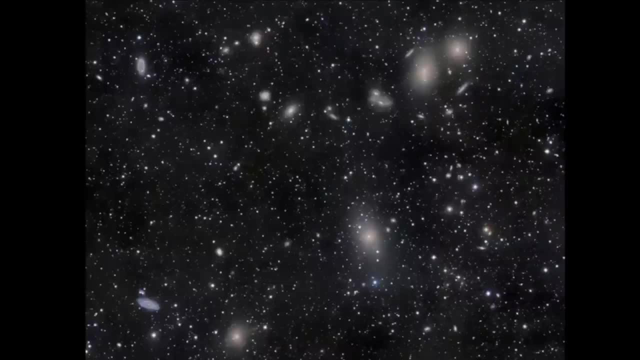 what about all the other galaxies? let's look at this, look at this, look at this field of stars and galaxies, all the fuzzy field of stars and galaxies, all the fuzzy field of stars and galaxies, all the fuzzy objects and galaxies, objects and galaxies, objects and galaxies at the point sources are stars in our 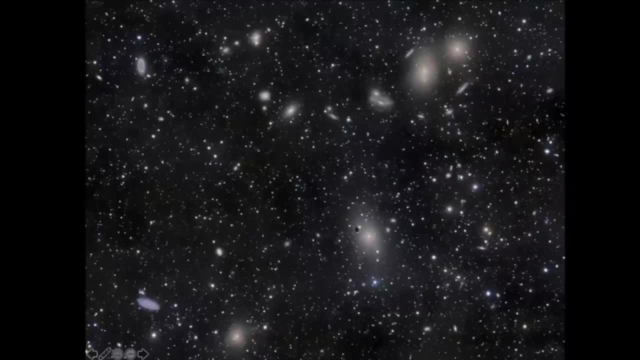 at the point sources are stars in our at the point sources are stars in our own galaxy, own galaxy, own galaxy. now, this is a big galaxy. this is the now. this is a big galaxy. this is the now. this is a big galaxy. this is the actually the center of what we call the. 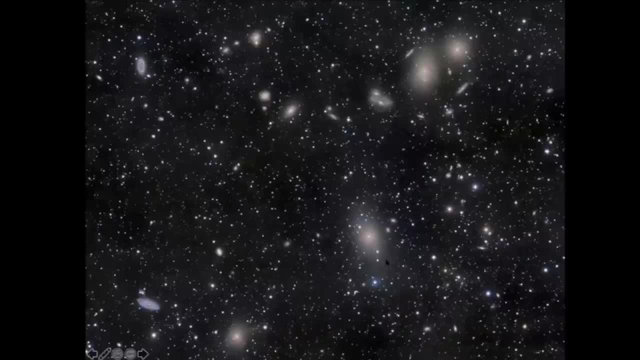 actually the center of what we call the, actually the center of what we call the virgo cluster, virgo cluster, virgo cluster- and it's the nearest cluster of galaxies and it's the nearest cluster of galaxies and it's the nearest cluster of galaxies to us. it's about 50 million light years. 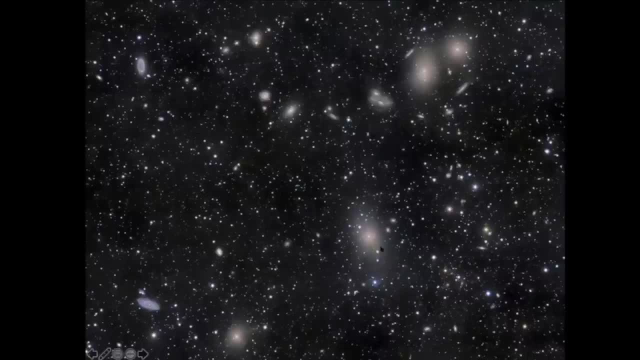 to us, it's about 50 million light years. to us, it's about 50 million light years away, away, away. and this large galaxy at the center of, and this large galaxy at the center of, and this large galaxy at the center of, it, m87, it, m87. 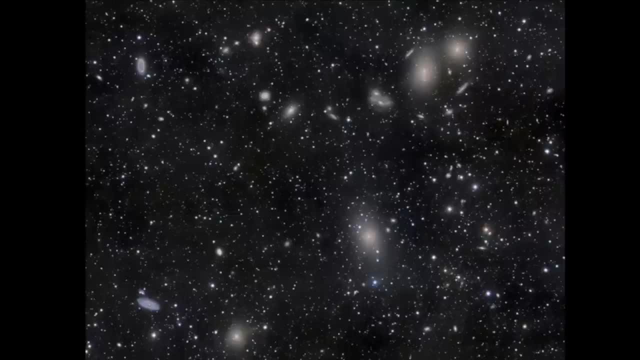 it. m87, we're going to look at two. but what about? we're going to look at two? but what about? we're going to look at two? but what about that? has that got a black hole in that? has that got a black hole in that? has that got a black hole in? astronomers have looked at all of these. 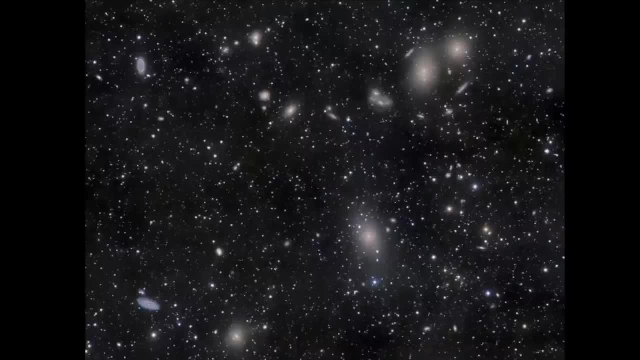 astronomers have looked at all of these. astronomers have looked at all of these carefully, with carefully, with carefully, with a wide range of telescopes different a wide range of telescopes different a wide range of telescopes, different wavelengths, wavelengths, wavelengths, and concluded that they all have black. 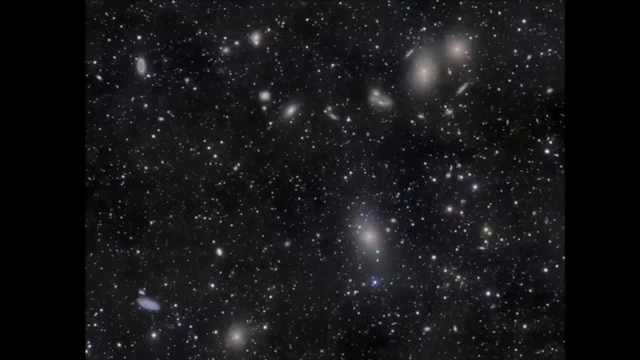 and concluded that they all have black. and concluded that they all have black holes at the centers, holes at the centers, holes at the centers- sometimes they're very active black holes, sometimes they're very active black holes. sometimes they're very active black holes and sometimes they're not. we'll talk. 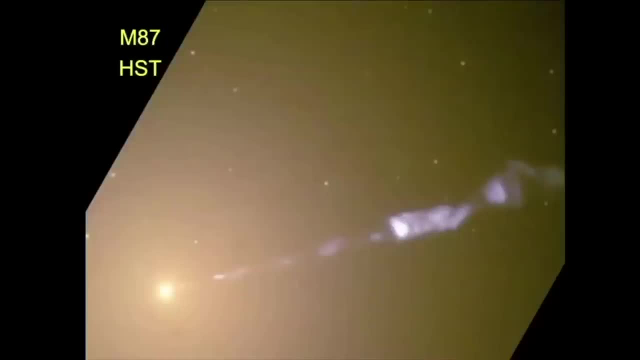 and sometimes they're not. we'll talk and sometimes they're not. we'll talk about what active means in a minute, about what active means in a minute, about what active means in a minute. m87 is an active black hole. m87 is an active black hole. 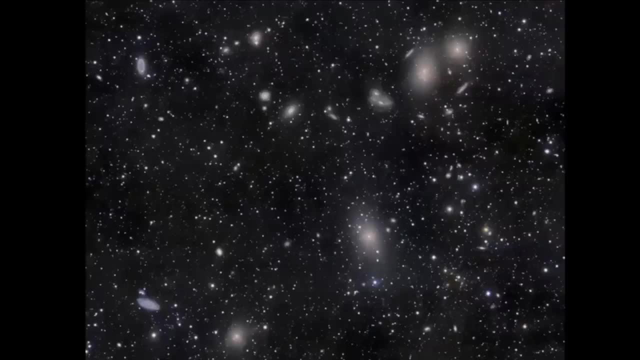 m87 is an active black hole. that's the one at the center of this. that's the one at the center of this. that's the one at the center of this galaxy, galaxy, galaxy. the hat and um it's uh got the jet. the hat and um it's uh got the jet. 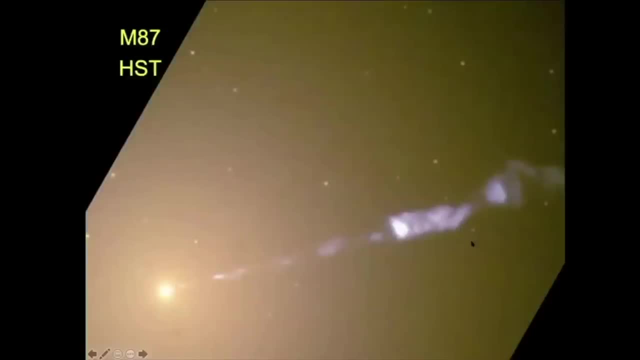 the hat and um it's uh, got the jet sticking out a bit. this jet was first sticking out a bit. this jet was first sticking out a bit. this jet was first seen, seen. seen in 1970 by this american astronomer, in 1970, by this american astronomer. 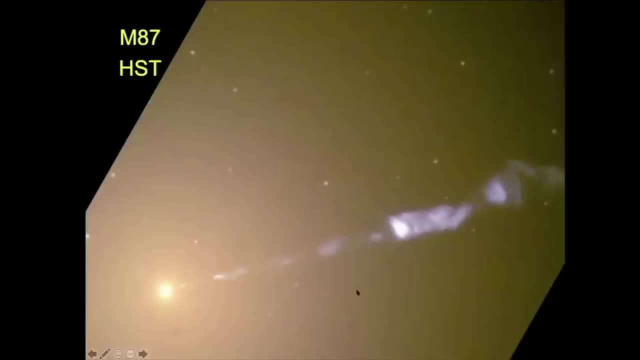 in 1970, by this american astronomer, keeper curtis, keeper curtis, keeper curtis, and he's spoken of a light ray, and he's spoken of a light ray, and he's spoken of a light ray, um, um, um, seen at the center of this galaxy. notice. 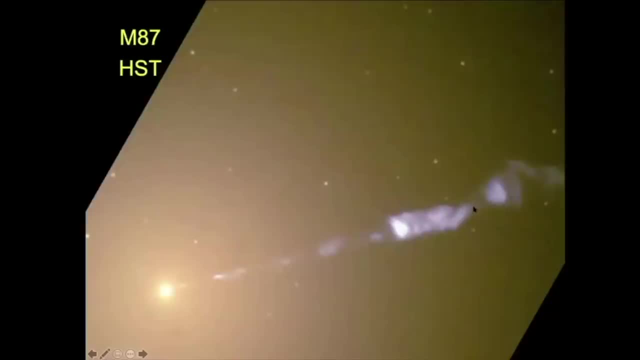 seen at the center of this galaxy notice. seen at the center of this galaxy notice. it doesn't continue. the other side it's. it doesn't continue. the other side it's, it doesn't continue. the other side, it's just sticking out like this, just sticking out like this. 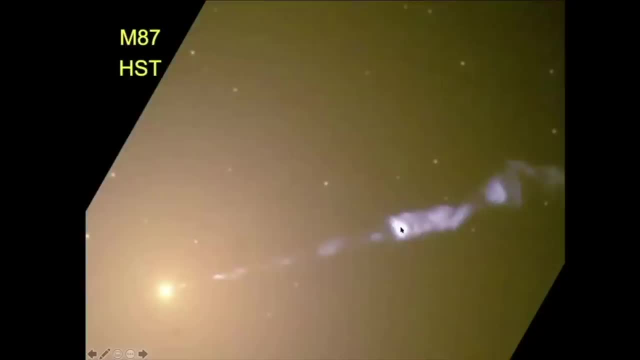 just sticking out like this, and this is quite large and you can see, and this is quite large and you can see, and this is quite large and you can see it relatively easily, it relatively easily, it relatively easily in a relatively small telescope you can. in a relatively small telescope you can. 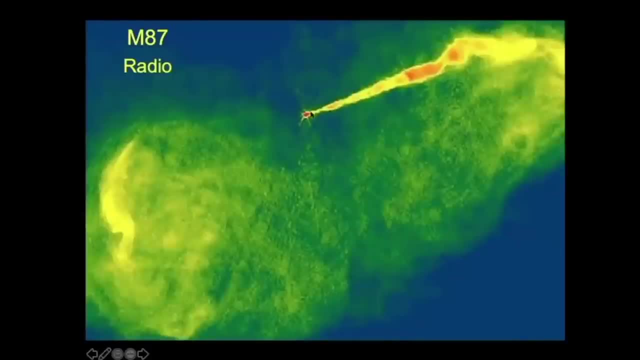 in a relatively small telescope. you can see it in a radio telescope. see it in a radio telescope, see it in a radio telescope, because it's we've got lots of radio, because it's we've got lots of radio, because it's we've got lots of radio emission, you can't see it going the. 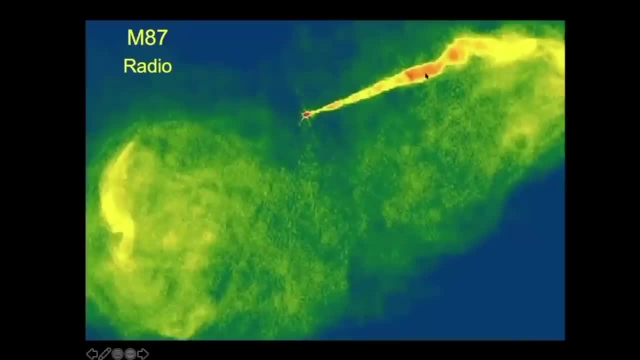 emission. you can't see it going. the emission. you can't see it going the other side, other side, other side. this is because this is the jet of this, is because this is the jet of this, is because this is the jet of plasma being squirted out of the center. 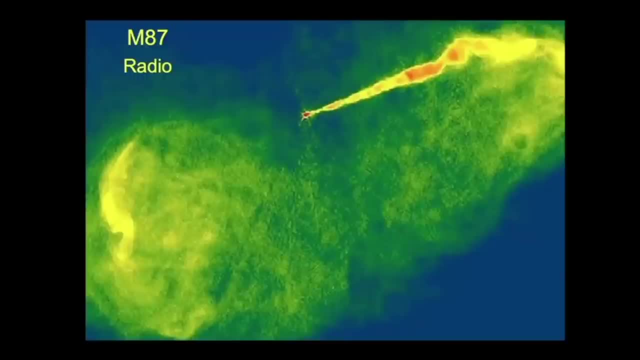 plasma being squirted out of the center. plasma being squirted out of the center by this active center, this active, by this active center, this active by this active center, this active nucleus and it's squirting out at a nucleus and it's squirting out at a 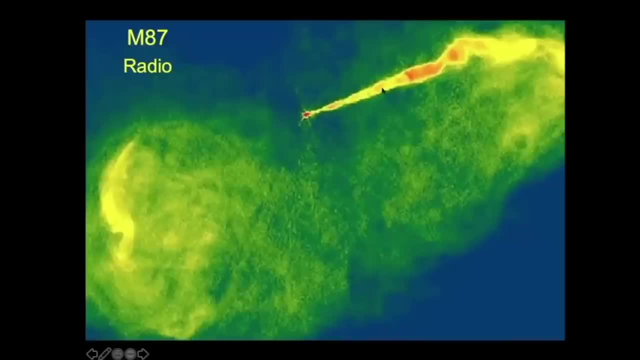 nucleus and it's squirting out at a relativistic speed of about 10 times relativistic speed of about 10 times relativistic speed of about 10 times. it's at 0.999c. it's at 0.999c. it's at 0.999c and, due to special relativity, it's also. 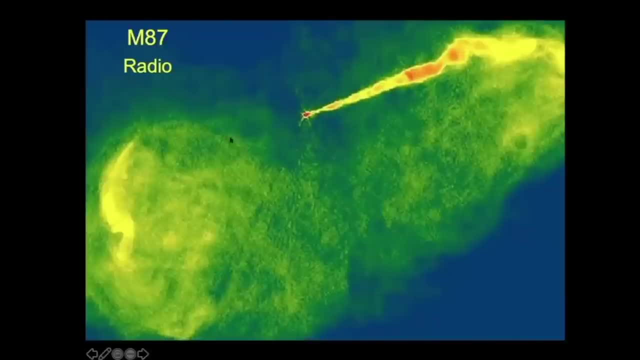 and due to special relativity, it's also- and due to special relativity, it's also- squirting out the other side and you squirting out the other side, and you squirting out the other side and you can't see the other side, because it's a. 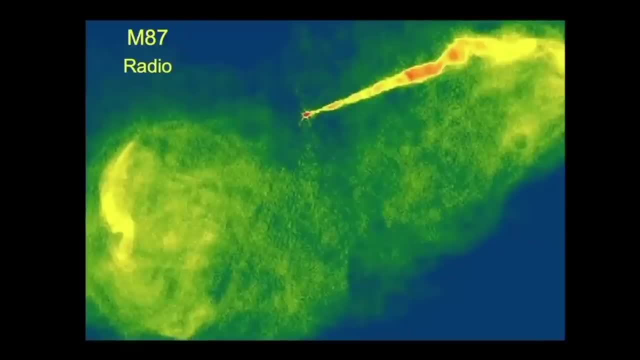 can't see the other side because it's a. can't see the other side because it's a vibration of light. light is vibration of light. light is vibration of light. light is, if you've got an object moving very. if you've got an object moving very. 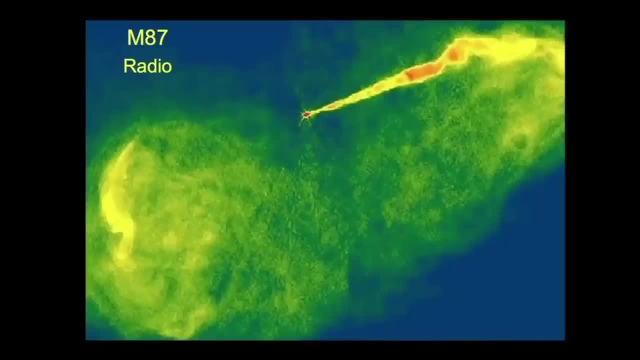 if you've got an object moving very fast, it throws the fast. it throws the fast, it throws the radiation from it in the direction. it's radiation from it in the direction, it's radiation from it in the direction it's traveling, traveling, traveling. so this is m87 and 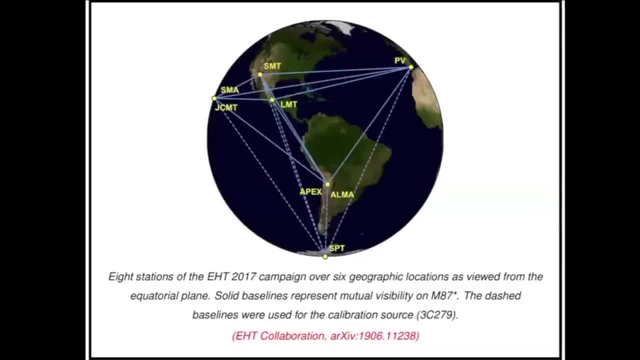 so this is m87 and so this is m87. and in using the same technique that we, in using the same technique that we, in using the same technique that we heard about in the last talk by evina, heard about in the last talk by evina, 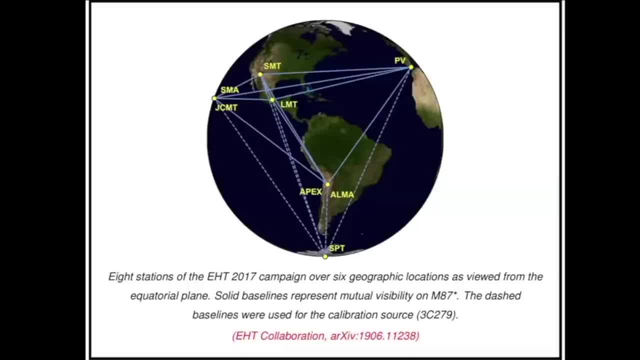 heard about in the last talk by evina, which is interferometry where you have. which is interferometry where you have, which is interferometry where you have radio telescopes spaced apart, radio telescopes spaced apart, radio telescopes spaced apart. she was talking about them spaced apart. 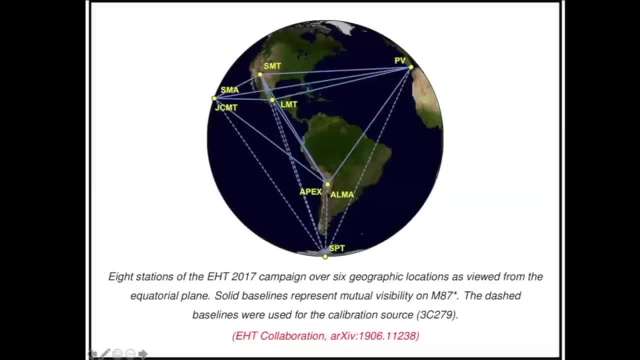 she was talking about them spaced apart. she was talking about them spaced apart by 15 kilometers, by 15 kilometers, by 15 kilometers. there's the alma telescope there, there's the alma telescope there, there's the alma telescope there, which may be spaced apart 15 kilometers. 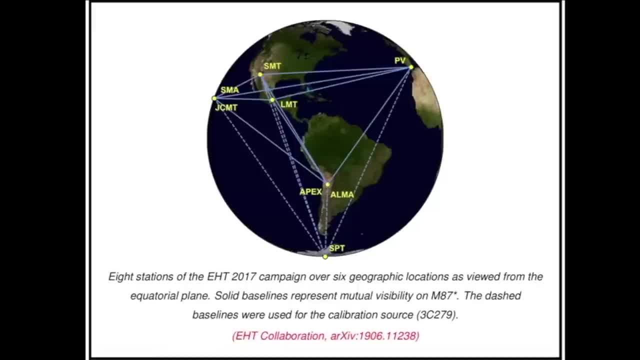 which may be spaced apart 15 kilometers, which may be spaced apart 15 kilometers. now we've got to. we want to go and look. now we've got to. we want to go and look. now we've got to. we want to go and look at very tiny things. we want to increase. 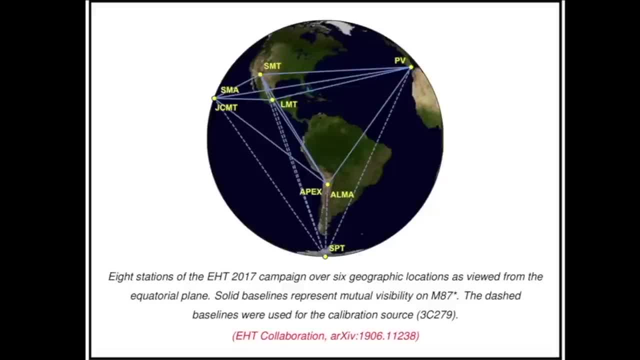 at very tiny things. we want to increase at very tiny things. we want to increase the resolution of the telescope, the resolution of the telescope, the resolution of the telescope, by thousands, to about a 10 000 to 100 000. by thousands, to about a 10 000 to 100 000. 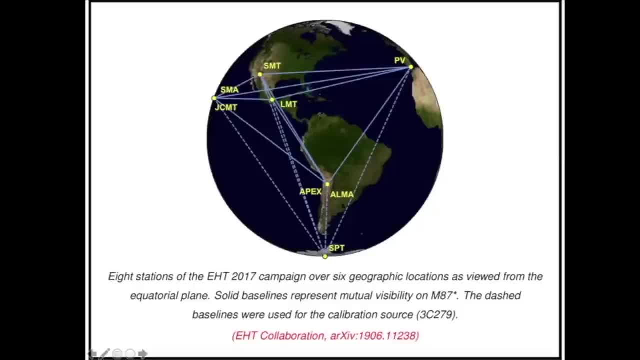 by thousands, to about a 10 000 to 100 000. what we do is we make use of telescopes. what we do is we make use of telescopes. what we do is we make use of telescopes spaced all over the earth. spaced all over the earth. 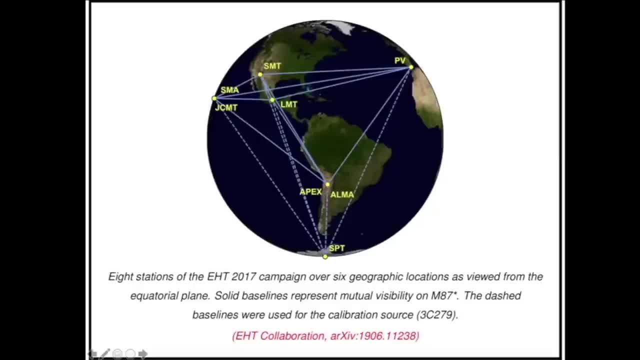 spaced all over the earth. so there's ones in hawaii ones in. so there's ones in hawaii ones in. so there's ones in hawaii ones in california, one in mexico, california, one in mexico, california, one in mexico, alma down there, and one in spain. 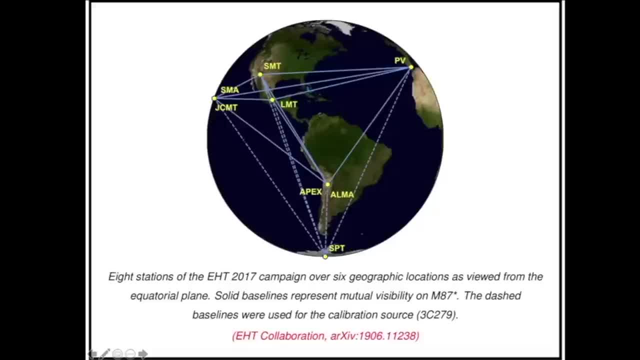 alma down there and one in spain. alma down there and one in spain. and also for calibration they use one of, and also for calibration they use one of, and also for calibration they use one of. the south pole, the south pole, the south pole. they use all of those telescopes together. 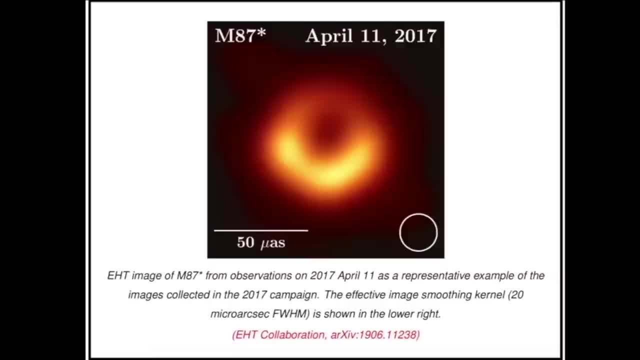 they use all of those telescopes together. they use all of those telescopes together, and out of that they got an image, and out of that they got an image, and out of that they got an image of m87, of m87, of m87, the center, and this is 50 micro arc. 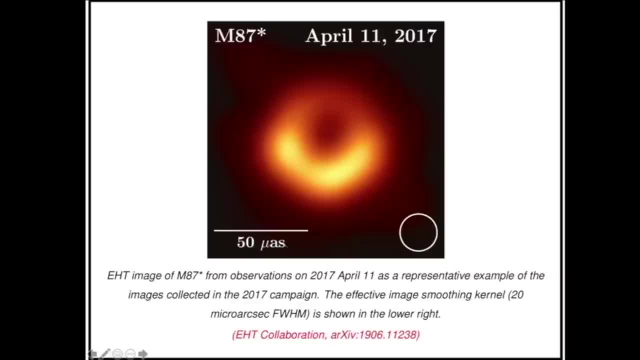 the center and this is 50 micro arc the center, and this is 50 micro arc seconds. seconds seconds. that is a very, very, very small angle. that is a very, very, very small angle. that is a very, very, very small angle. and so they, and so they. 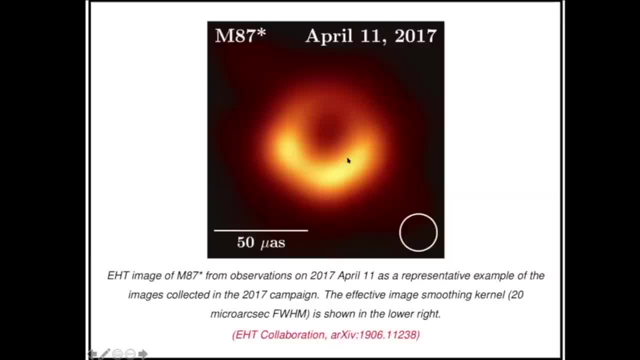 and so they. this was the observation in april. the. this was the observation in april. the. this was the observation in april: the 11th, 11th, 11th, but they announced the results, uh, last, but they announced the results, uh, last, but they announced the results, uh, last year of this ring and uh, this is. 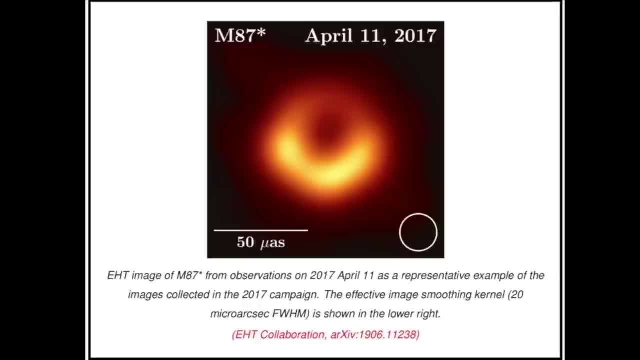 year of this ring and uh. this is year of this ring and uh. this is generally thought of, generally thought of, generally thought of as the image of a black hole, this as the image of a black hole, this as the image of a black hole. this yellow is not the black hole, the black. 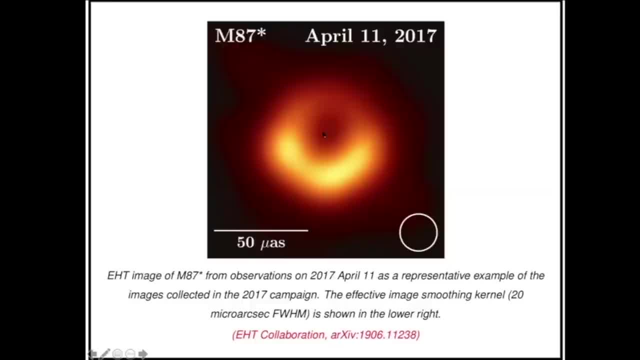 yellow is not the black hole. the black yellow is not the black hole. the black hole is the thing in the middle hole is the thing in the middle hole, is the thing in the middle. we can't actually see the black hole we. we can't actually see the black hole we. 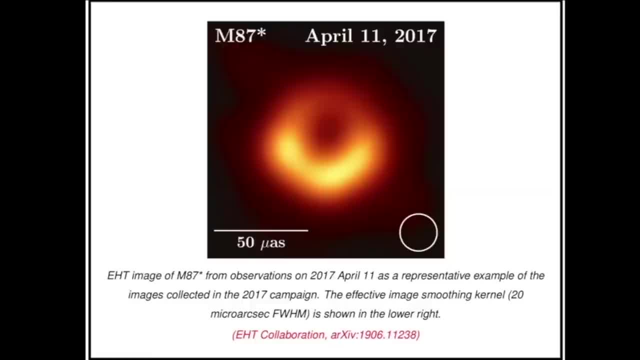 we can't actually see the black hole. we can only see matter swirling around it. can only see matter swirling around it. can only see matter swirling around it. okay, you can't see a black hole, you can. okay, you can't see a black hole, you can. okay, you can't see a black hole, you can only tell a black hole is there by the 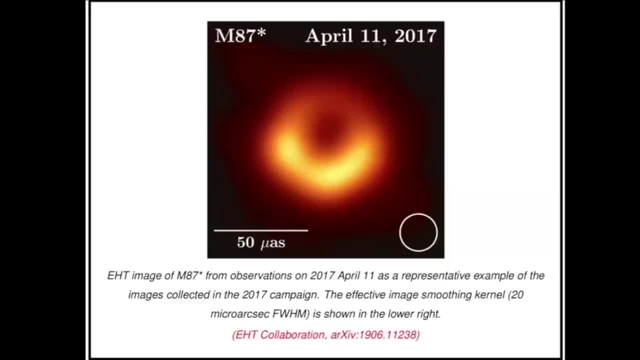 only tell a black hole is there by the only tell a black hole is there by the motion and material around it. motion and material around it, motion and material around it, just as john mitchell said, just as john mitchell said, just as john mitchell said now going and looking at many other, 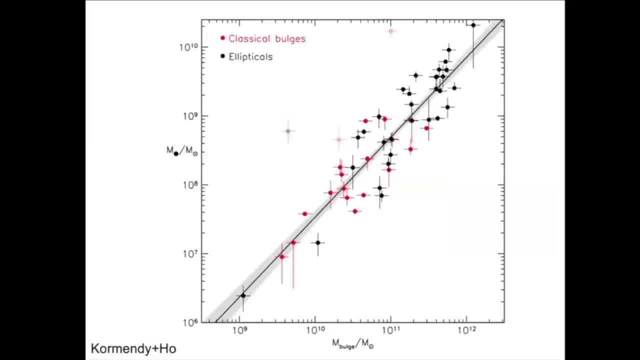 now going and looking at many other now going and looking at many other black holes in many other galaxies. black holes in many other galaxies. black holes in many other galaxies over the last 20 years we ended up with over the last 20 years we ended up with. 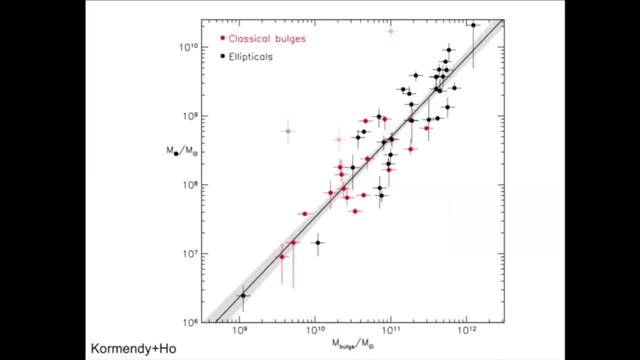 over the last 20 years. we ended up with this, this, this correlation which uh for astronomy is a correlation which uh for astronomy is a correlation which uh for astronomy is a pretty good correlation. i'll tell you pretty good correlation. i'll tell you pretty good correlation. i'll tell you, and it's about, got four orders of. 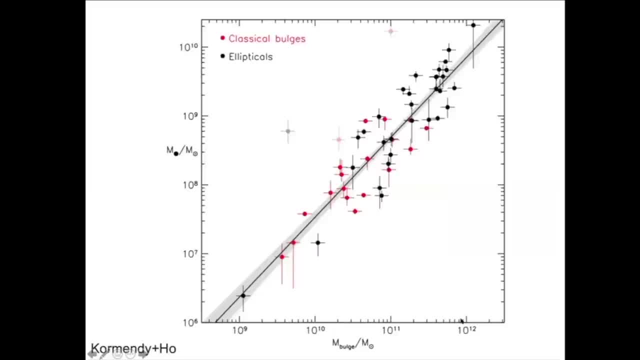 and it's about got four orders of, and it's about got four orders of magnitude down here and four orders of magnitude down here and four orders of magnitude down here and four orders of magnitude cross here, magnitude cross here, magnitude cross here, and it's a and it's a. 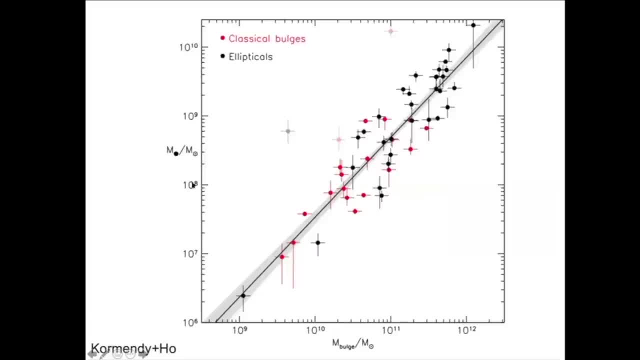 and it's a it's a logarithmic correlation where it's. it's a logarithmic correlation where it's. it's a logarithmic correlation where it's jumping by a factor of 10 in each of jumping by a factor of 10 in each of. 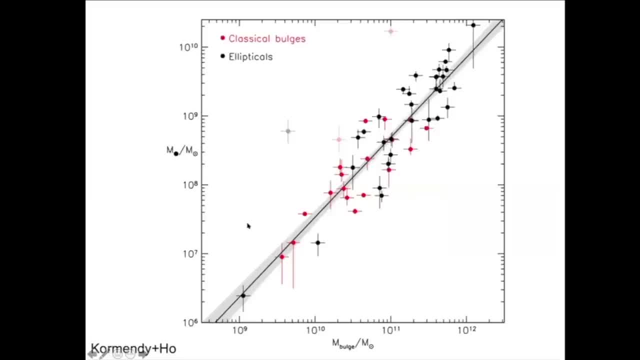 jumping by a factor of 10 in each of these, these, these axis points, axis points, axis points and basically, if you look at a black and basically if you look at a black, and basically if you look at a black hole of mass, 10 billion solar masses, it 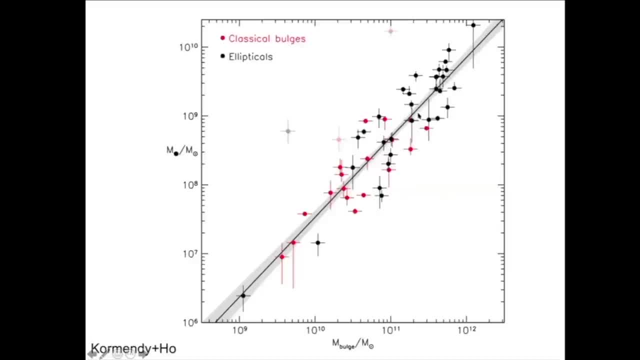 hole of mass: 10 billion solar masses. it hole of mass- 10 billion solar masses. it lives in a galaxy that is like 200 times lives in a galaxy that is like 200 times lives in a galaxy that is like 200 times galaxies. and when it talks about the 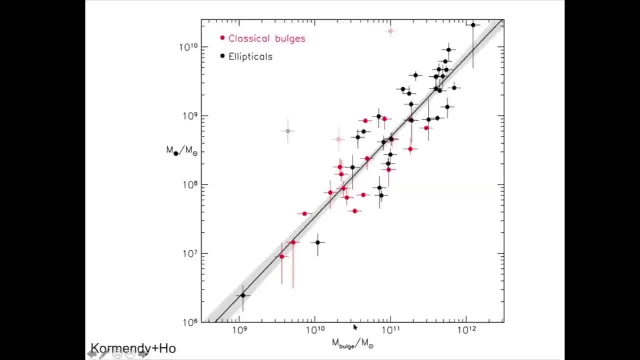 galaxies. and when it talks about the galaxies and when it talks about the mass of the bulge, it's talking about the mass of the bulge. it's talking about the mass of the bulge. it's talking about the mass of the central spherical part of. 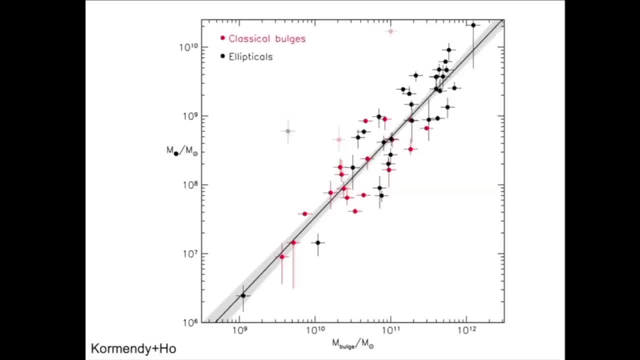 mass of the central spherical part of mass of the central spherical part of the galaxy. if it's a spiral galaxy, we're the galaxy. if it's a spiral galaxy, we're the galaxy. if it's a spiral galaxy, we're not worried about the spiral arms, we're. 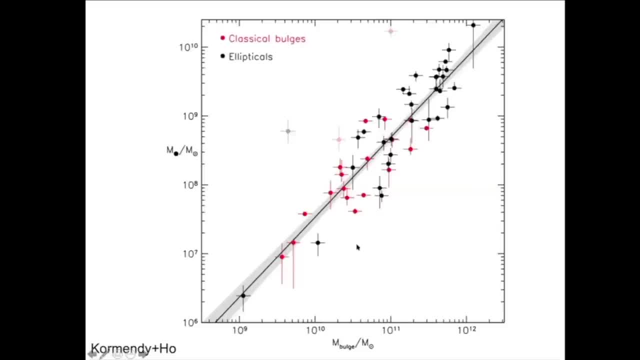 not worried about the spiral arms. we're not worried about the spiral arms. we're looking at the bulge at the center, looking at the bulge at the center, looking at the bulge at the center and the ratio between the mass of the and the ratio between the mass of the. 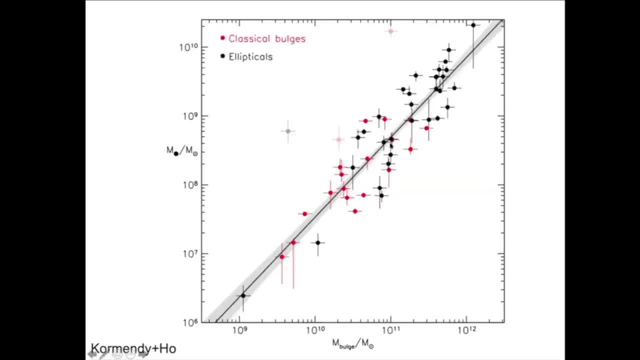 and the ratio between the mass of the black hole, black hole, black hole to the mass of the bulge is typically a to. the mass of the bulge is typically a to. the mass of the bulge is typically a factor of factor of factor of several hundred. 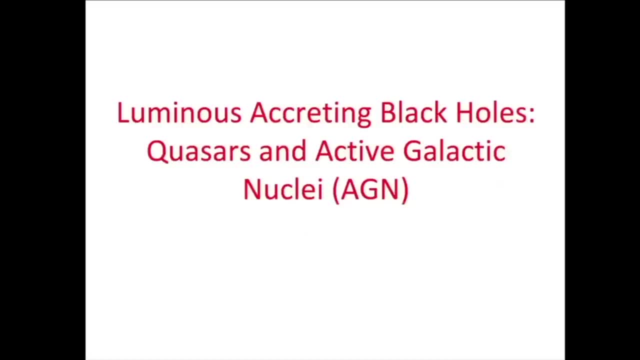 several hundred, several hundred. i know what to jump to talking about. i know what to jump to talking about. i know what to jump to talking about: luminous, secreting black holes, luminous, secreting black holes, luminous, secreting black holes, and they're called quasars and active. 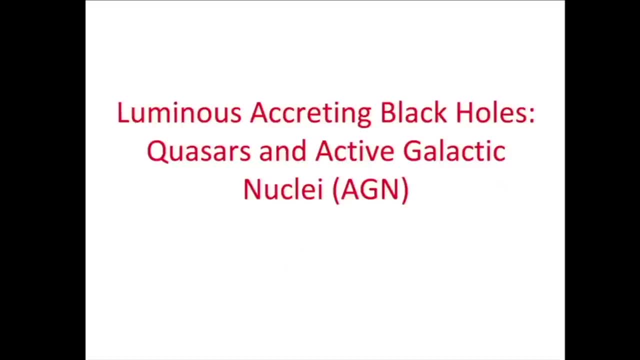 and they're called quasars and active, and they're called quasars and active, galactic nuclei, galactic nuclei, galactic nuclei and creating. by that i'm talking about and creating. by that i'm talking about and creating. by that i'm talking about matter falling into the black holes. 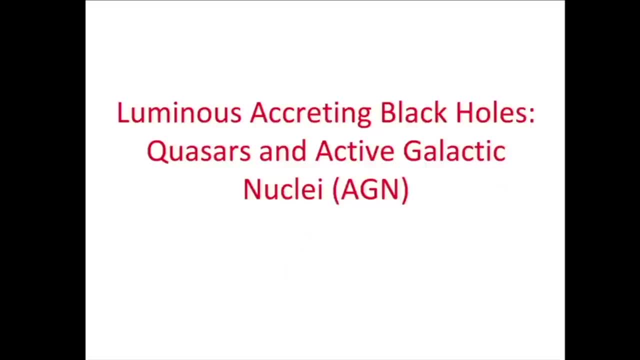 matter falling into the black holes matter falling into the black holes and as it falls into the black holes. and as it falls into the black holes. and as it falls into the black holes, it doesn't fall just directly radially. it doesn't fall just directly radially. 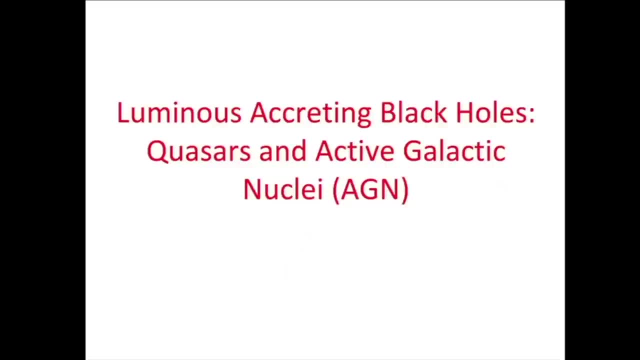 it doesn't fall just directly, radially, into the black holes, into the black holes, into the black holes. it swirls around the black holes and it swirls around the black holes and it swirls around the black holes, and lots of collisions and lots of friction. 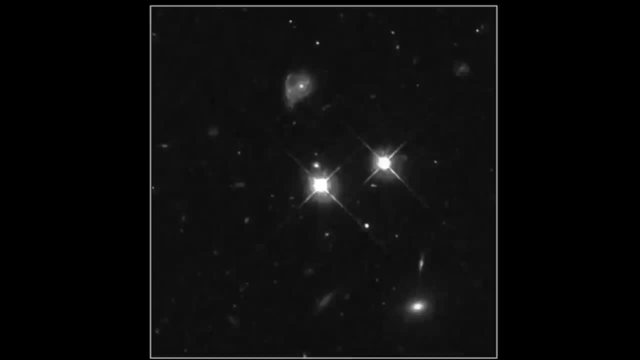 lots of collisions and lots of friction, lots of collisions and lots of friction, and they give rise to lots of radiation and they give rise to lots of radiation and they give rise to lots of radiation. this is a picture from hubble. this is a picture from hubble. 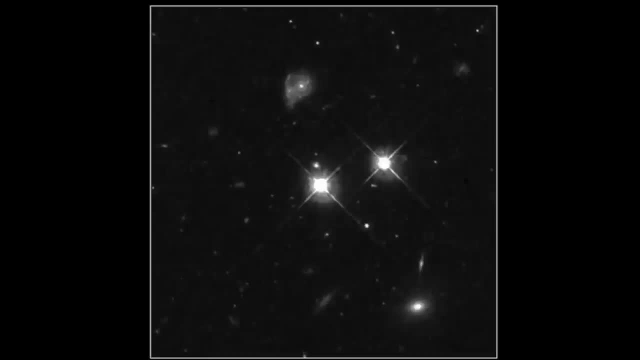 this is a picture from hubble of just a field with a quasar in, of just a field with a quasar in, of just a field with a quasar in and a bright star. this is the quasar and a bright star. this is the quasar. 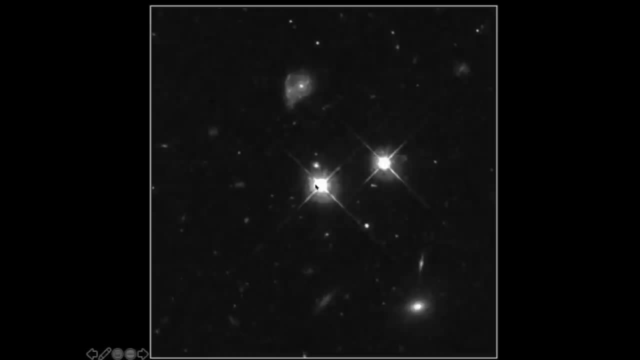 and a bright star. this is the quasar that's the bright star. now this quasar that's the bright star. now this quasar that's the bright star. now this quasar turns out to be a million times further, turns out to be a million times further. 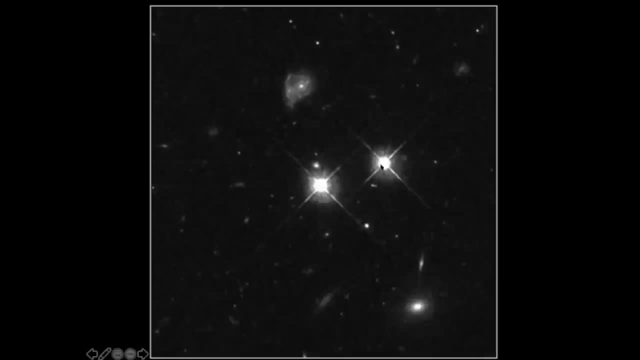 turns out to be a million times further away, away away than the star from the inverse square law, than the star from the inverse square law, than the star from the inverse square law. it's therefore a trillion times more. it's therefore a trillion times more. it's therefore a trillion times more luminous. a trillion is 10 to the 12th. 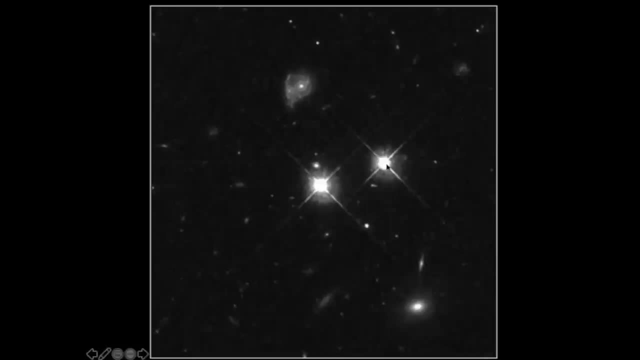 luminous a trillion is 10 to the 12th luminous a trillion is 10 to the 12th. 10 to the 12 times more luminous than the 10 to the 12 times more luminous than the 10 to the 12 times more luminous than the star now. 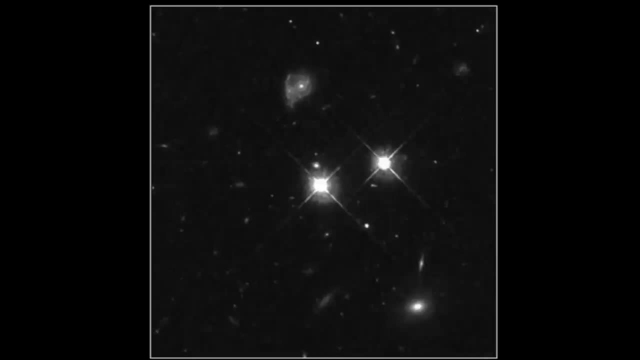 star now, star now. all the galaxy has got a hundred billion. all the galaxy has got a hundred billion. all the galaxy has got a hundred billion stars in 10 to the 11 stars, stars in 10 to the 11 stars, stars in 10 to the 11 stars. so this is 10 times more luminous. 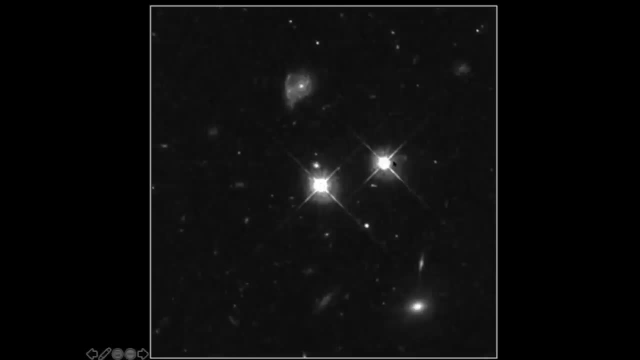 so this is 10 times more luminous. so this is 10 times more luminous, 10 times more luminous than a whole, 10 times more luminous than a whole, 10 times more luminous than a whole galaxy, galaxy, galaxy. so these things are often quite distant. 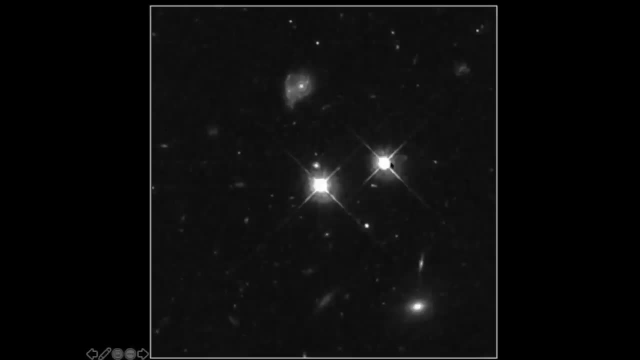 so these things are often quite distant. so these things are often quite distant, and and and very luminous, they're very luminous. what very luminous. they're very luminous. what very luminous, they're very luminous. what is going on is going on, is going on. you can't explain this with stellar. 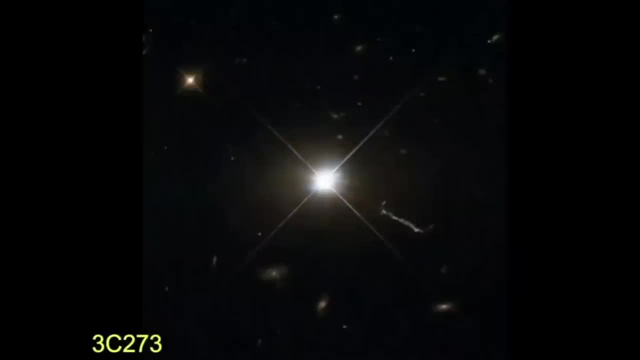 you can't explain this with stellar, you can't explain this with stellar. processes, processes, processes, in particular. the first one found 3c273 in particular. the first one found 3c273. in particular, the first one found 3c273, which was found in 1963 and identified. 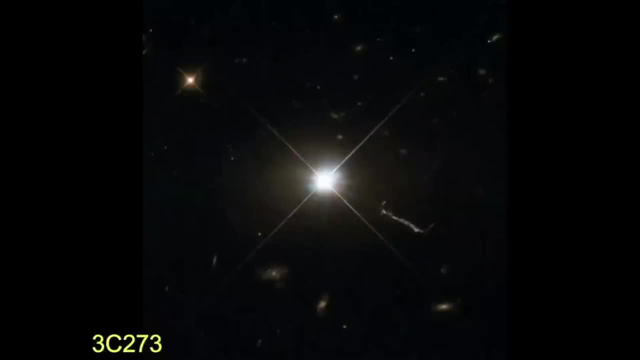 which was found in 1963 and identified, which was found in 1963 and identified by martin schmidt, by martin schmidt, by martin schmidt, and it was the same year that roy kerr, and it was the same year that roy kerr, and it was the same year that roy kerr found his solution to the spinning black. 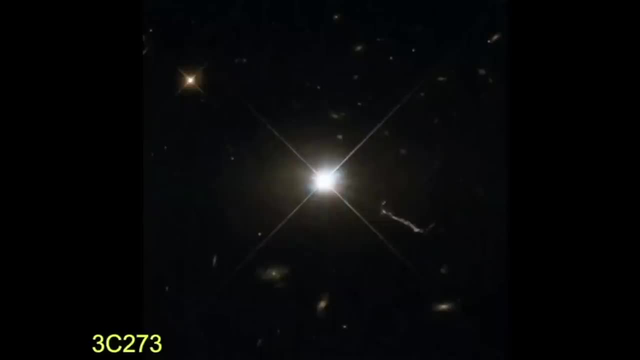 found his solution to the spinning black, found his solution to the spinning black, hole, hole hole. so 1963 is special for us. so 1963 is special for us, so 1963 is special for us. then here what we can see: 3c273. 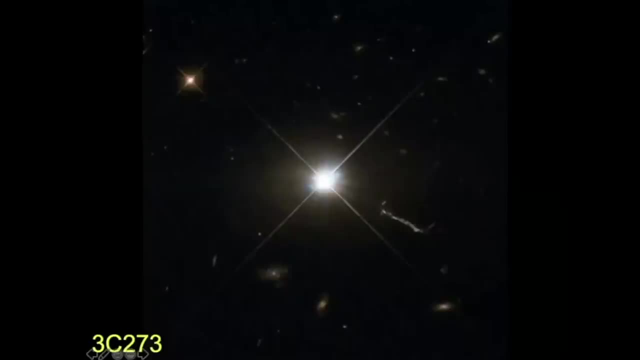 then here what we can see: 3c273. then here what we can see: 3c273: hubble image: the same diffraction spikes. hubble image: the same diffraction spikes. hubble image: the same diffraction spikes which are due to the instrument, due to. 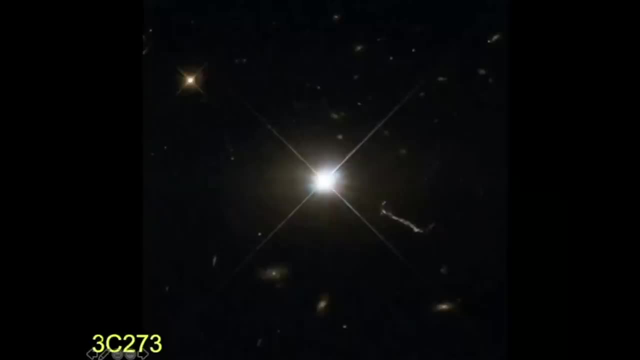 which are due to the instrument, due to which are due to the instrument, due to the optics of the telescope, the optics of the telescope, the optics of the telescope, um, and this is the in the third um and this is the in the third um and this is the in the third cambridge catalogue of uh radio sources. 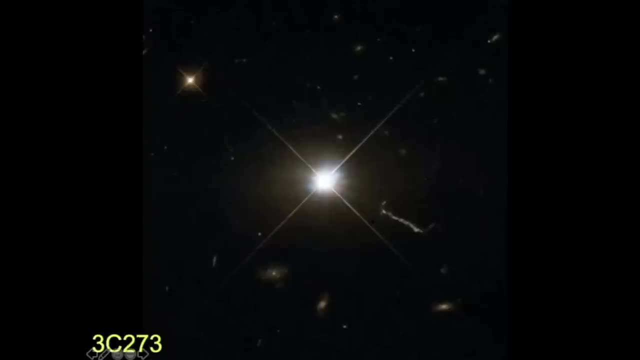 cambridge catalogue of uh radio sources. cambridge catalogue of uh radio sources. it's number 273, so it's a radio source. it's number 273, so it's a radio source. it's number 273, so it's a radio source as well as well. 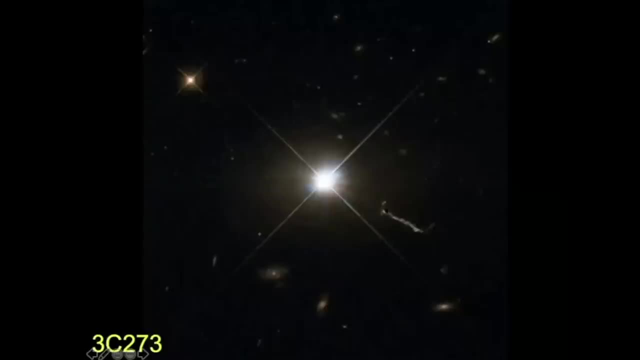 as well. and this strange structure actually if, and this strange structure actually if, and this strange structure actually if you look, you look, you look very, very carefully, particularly with very, very carefully, particularly with very, very carefully, particularly with other wavelengths like the radio, or the other wavelengths like the radio or the 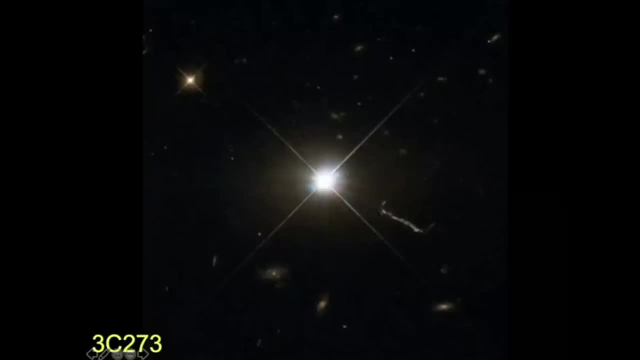 other wavelengths, like the radio or the x-ray, you'll find it continues right. x-ray: you'll find it continues right. x-ray: you'll find it continues right back to there, back to there, back to there. it's a jet of material squirted out. it's a jet of material squirted out. 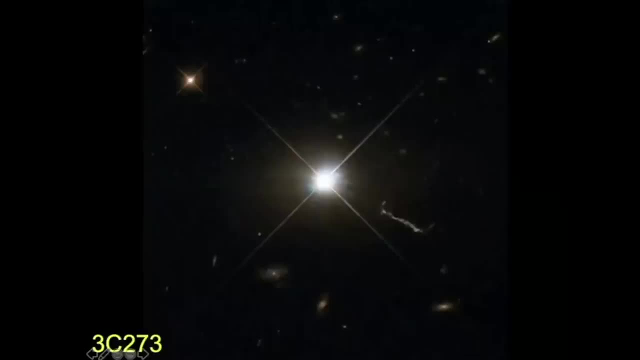 it's a jet of material squirted out again, at, again, at, again, at very high velocities. it's squirted out very high velocities. it's squirted out very high velocities. it's squirted out from the central object, from the central object, from the central object. these objects, these are known as quasars. 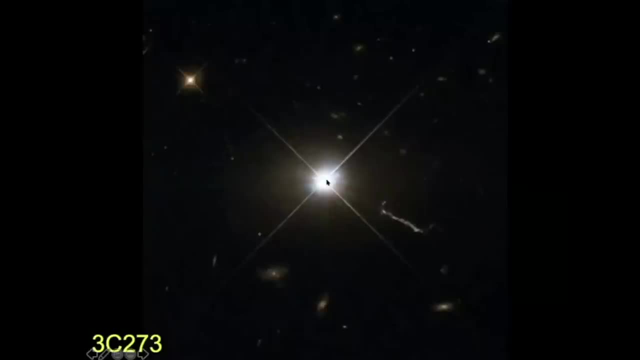 these objects, these are known as quasars. these objects- these are known as quasars- and three c273 after it was discovered and three c273 after it was discovered and three c273 after it was discovered, was, was, was also. it was actually more luminous, it's. 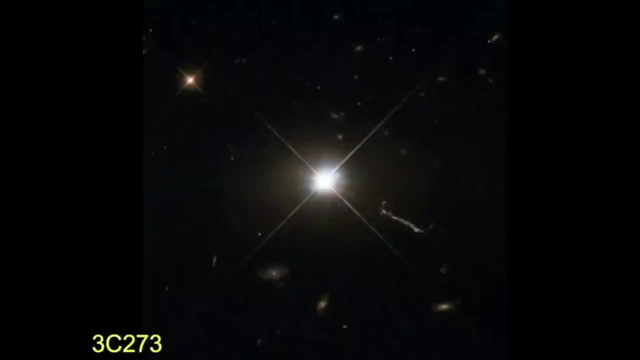 also, it was actually more luminous. it's also: it was actually more luminous. it's: it's 10 to the 13 so many luminosities. it's 10 to the 13 so many luminosities. it's 10 to the 13 so many luminosities. it's a hundred times more lumens that. 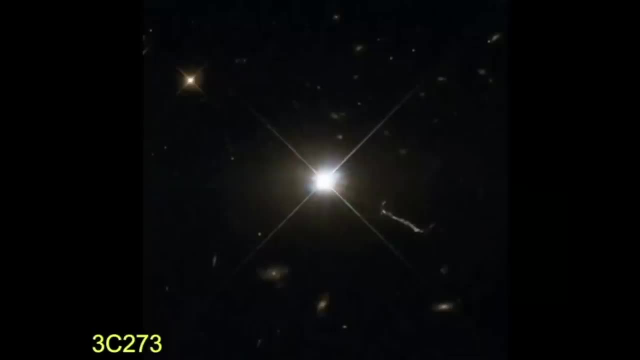 it's a hundred times more lumens, that it's a hundred times more lumens that all of our galaxy put together, all of our galaxy put together, all of our galaxy put together. and our galaxy extends and our galaxy extends and our galaxy extends. it's his stars extend over a distance. 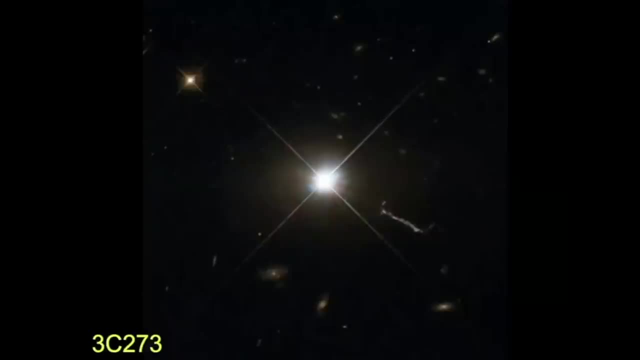 it's his stars extend over a distance. it's his stars extend over a distance which is about 30 000 light years, which is about 30 000 light years, which is about 30 000 light years. now it was seen that three c273. 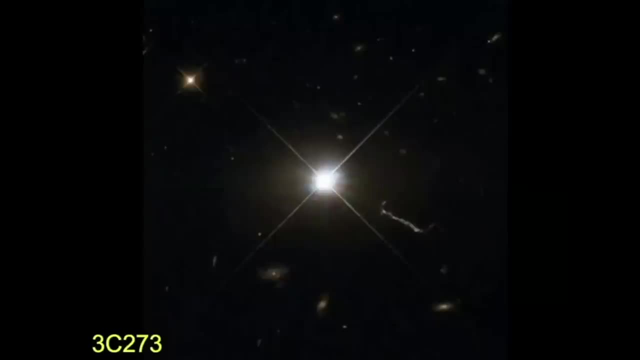 now it was seen that three c273. now it was seen that three c273 varies in brightness over a week, varies in brightness over a week. varies in brightness over a week. how can something as big as thousands of, how can something as big as thousands of, how can something as big as thousands of light years? 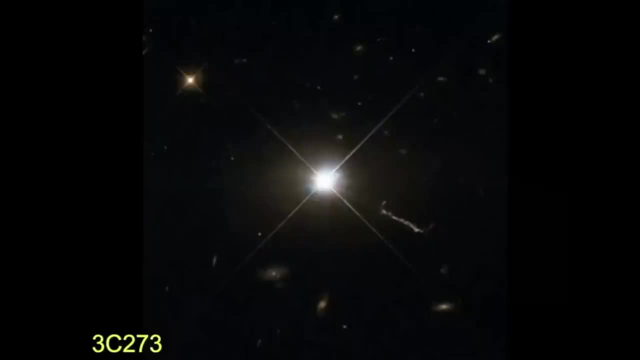 light years. light years vary on time scales of a week. the only vary on time scales of a week. the only vary on time scales of a week. the only way from causality is to make the thing way from causality is to make the thing way from causality is to make the thing very small. 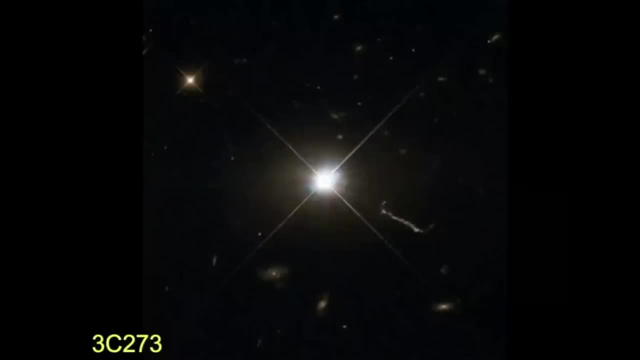 very small, very small. it has to be smaller than a light week. it has to be smaller than a light week. it has to be smaller than a light week across. it has to be smaller than the across. it has to be smaller than the across. it has to be smaller than the solar system. 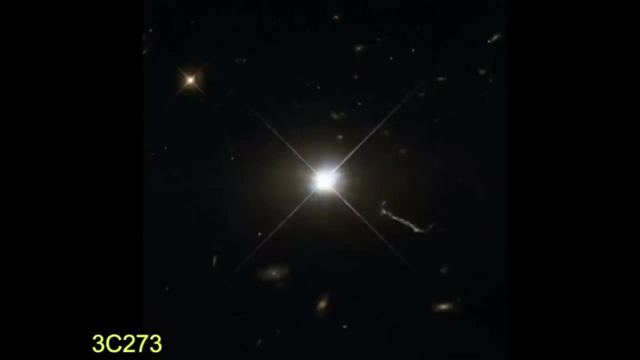 solar system. solar system. this object has to be smaller than the. this object has to be smaller than the. this object has to be smaller than the solar system. solar system. solar system, and yet produce 10 or 100 times more. and yet produce 10 or 100 times more. 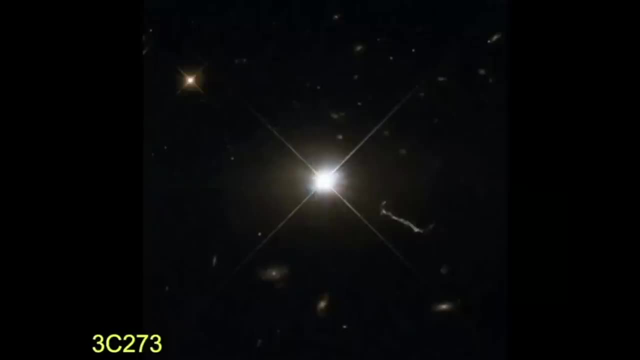 and yet produce 10 or 100 times more power, power, power than a whole galaxy. it's something very than a whole galaxy. it's something very than a whole galaxy. it's something very special, special, special, and we think it consists, consists of a, and we think it consists, consists of a. 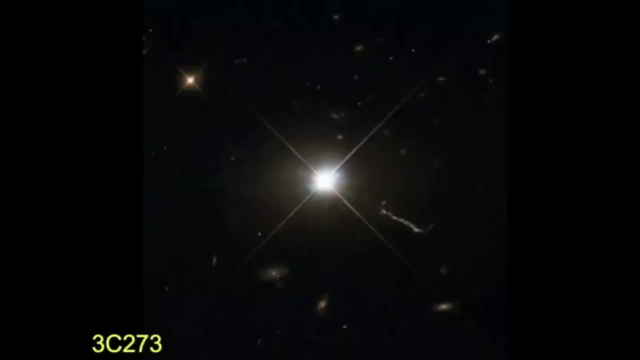 and we think it consists consists of a very, very, very massive black hole into which matter is massive black hole into which matter is massive black hole into which matter is stringing. in fact, they're all over the sky, quasars. in fact, they're all over the sky, quasars. 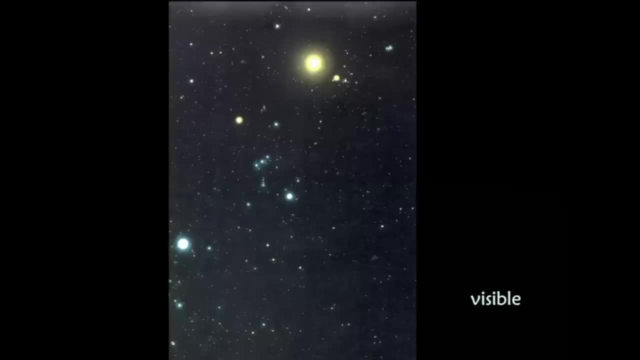 in fact, they're all over the sky. quasars are all over the sky, are all over the sky, are all over the sky. quasars are all over the sky. let's go back to the visible. let's go back to the visible. let's go back to the visible picture of the sky. 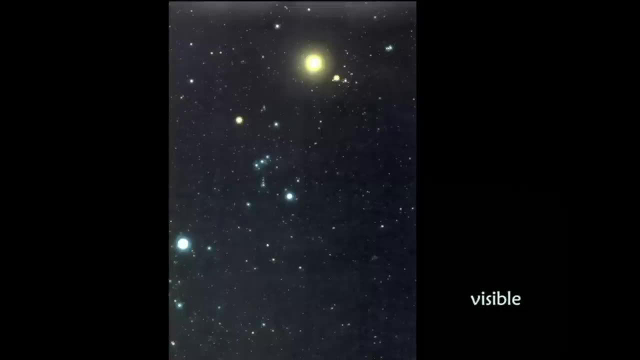 picture of the sky. picture of the sky. it's very similar to the one avena. it's very similar to the one avena. it's very similar to the one avena showed where you can see the showed, where you can see the showed, where you can see the constellation of orion. 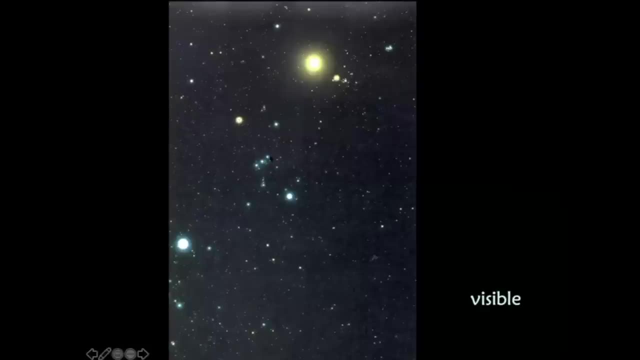 constellation of orion. constellation of orion. here's beetlejuice rigel. here's beetlejuice rigel. here's beetlejuice rigel. the stars of orion, the sword. the stars of orion, the sword, the stars of orion, the sword, the brightest star in the sky, sirius. 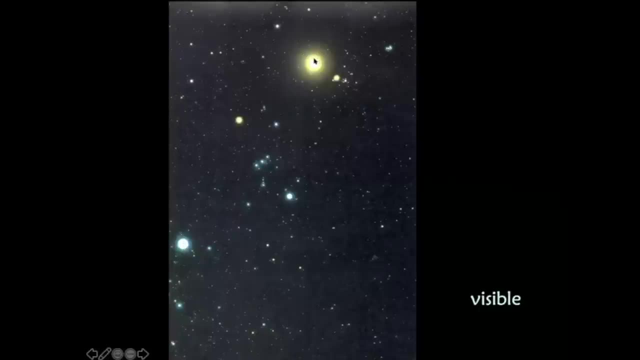 the brightest star in the sky, sirius. the brightest star in the sky, sirius, and the moon and the moon and the moon. let's now look in the x-ray band. x-rays. let's now look in the x-ray band. x-rays- let's now look in the x-ray band. x-rays are more energetic photons, the visible. 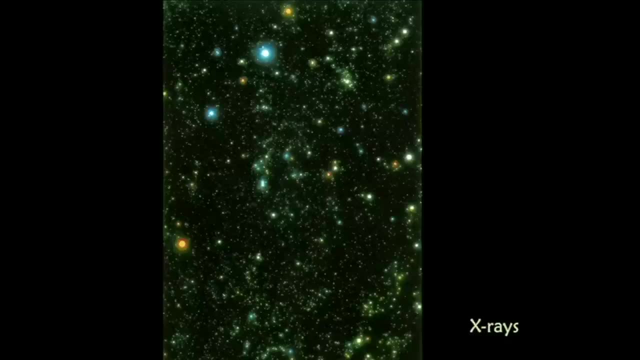 are more energetic photons. the visible are more energetic photons. the visible light, by a factor of thousands of ten light, by a factor of thousands of ten light, by a factor of thousands of ten thousand, thousand, thousand. they look at, they come from objects. they look at, they come from objects. 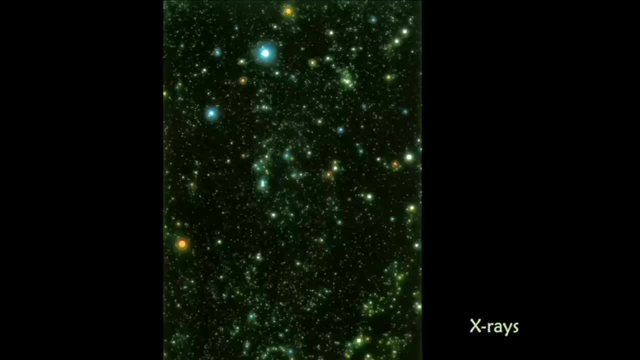 they look at. they come from objects which are a thousand to ten thousand, which are a thousand to ten thousand, which are a thousand to ten thousand times hotter than stars, times hotter than stars, times hotter than stars. stars are thousands of degrees, these are. stars are thousands of degrees, these are. 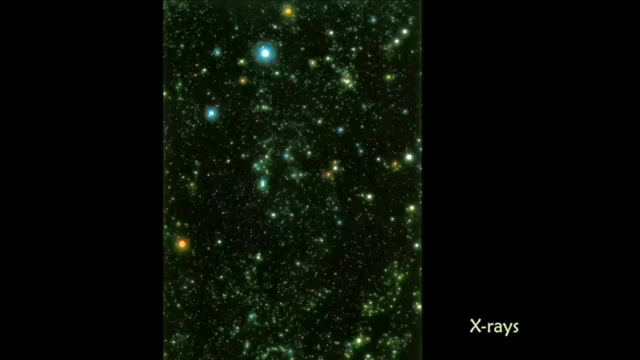 stars are thousands of degrees. these are millions to tens of millions of degrees, millions to tens of millions of degrees, millions to tens of millions of degrees. they in particular come from very compact. they in particular come from very compact. they in particular come from very compact objects, objects. 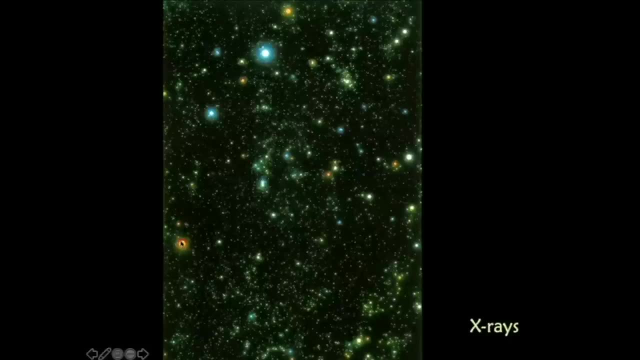 objects. this is serious in x-rays. you're not. this is serious in x-rays, you're not. this is serious in x-rays. you're not. looking at the same object as in this. looking at the same object as in this. looking at the same object as in this one. 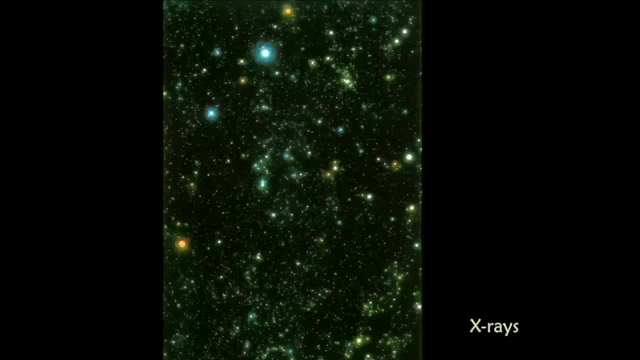 one one. it's not the same object. this is a. it's not the same object. this is a. it's not the same object. this is a binary star, binary star, binary star, serious a. the one you can see as the this as the. the one you can see as the this as the. 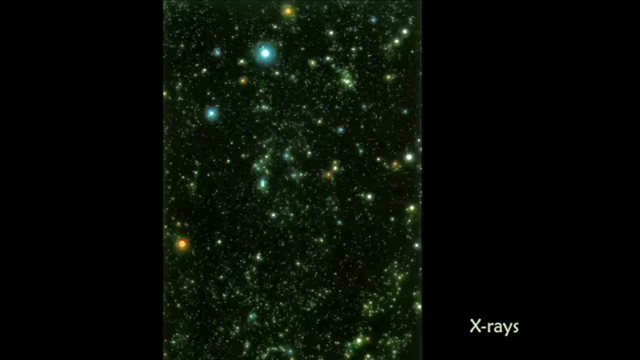 the one you can see as the this: as the star in the sky. star in the sky. star in the sky as a companion that goes around it every, as a companion that goes around it every, as a companion that goes around it every 49.9 years. 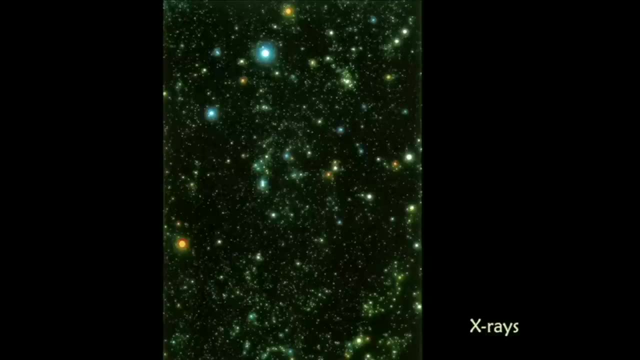 49.9 years. 49.9 years. the companion is a dead star, a white. the companion is a dead star, a white. the companion is a dead star, a white dwarf in x-rays. that's what you see as dwarf in x-rays. that's what you see as. 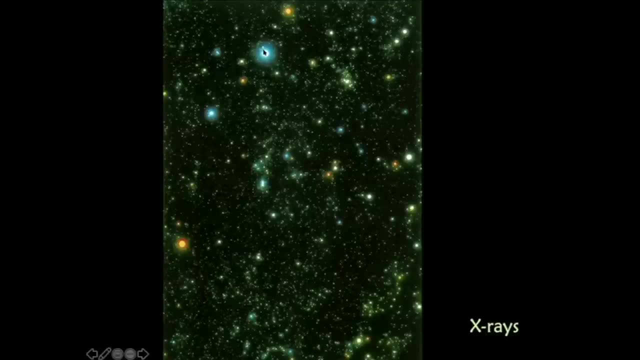 dwarf in x-rays. that's what you see as brightest, brightest, brightest. if you go here, if you go here, if you go here. that that that you remember there's a bright object up. you remember there's a bright object up. you remember there's a bright object up there. 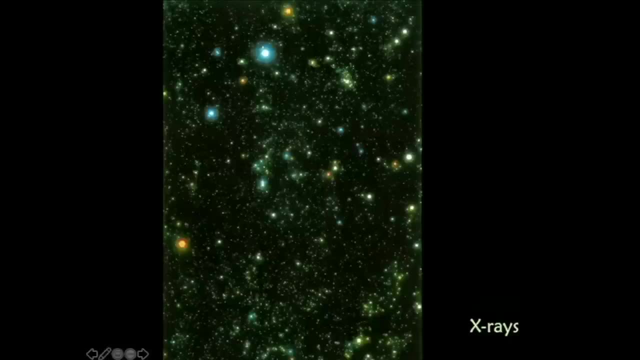 there, there, that's, that's, that's, that's the moon, but in x-rays that's the moon, but in x-rays that's the moon, but in x-rays, the moment is very faint. the moment is very faint, the moment is very faint. this object is the crab nebula. it's a. 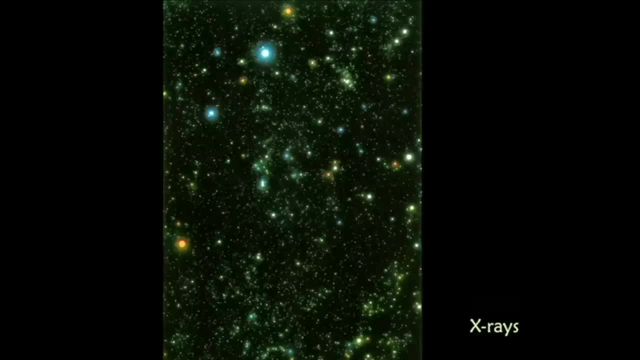 this object is the crab nebula. it's a. this object is the crab nebula. it's a ex. it's the result of a supernova ex. it's the result of a supernova ex. it's the result of a supernova explosion, explosion, explosion from which a neutron star, a spinning. 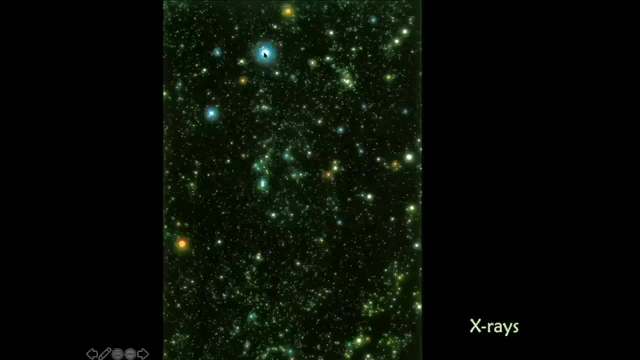 from which a neutron star, a spinning from which a neutron star, a spinning neutron star image which is a pulsar neutron star image which is a pulsar neutron star image which is a pulsar. so that's what's giving rise to that. so that's what's giving rise to that. 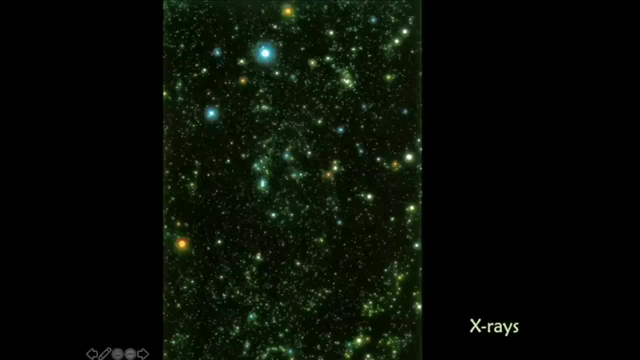 so that's what's giving rise to that, and, and, and, basically, although you can see some of basically, although you can see some of basically, although you can see some of these stars, like the stars in orion's, these stars, like the stars in orion's- 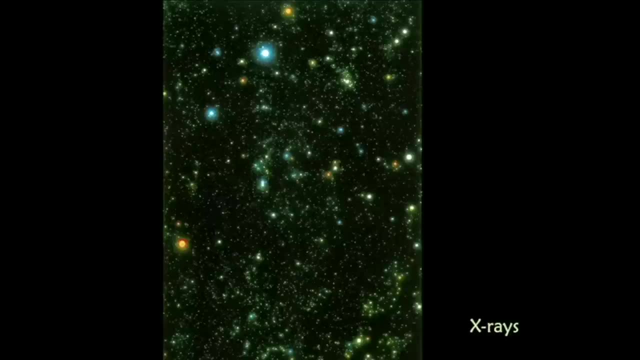 these stars, like the stars in orion's belt. you can see them because they've belt. you can see them because they've belt. you can see them because they've got tangled magnetic fields in them. got tangled magnetic fields in them. got tangled magnetic fields in them. basically, most of these objects down here. 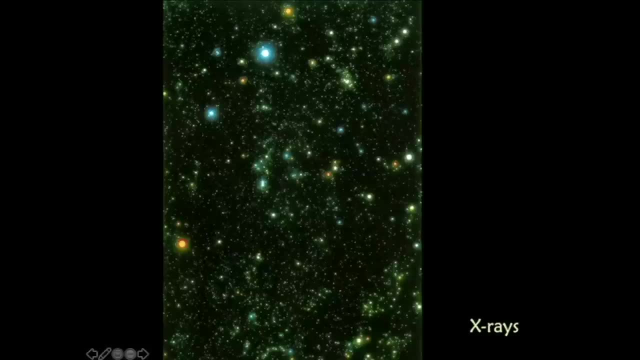 basically, most of these objects down here, basically most of these objects down here- are background, are background, are background, creating black holes in distant galaxies, creating black holes in distant galaxies, creating black holes in distant galaxies. this is what makes up the x-ray. this is what makes up the x-ray. 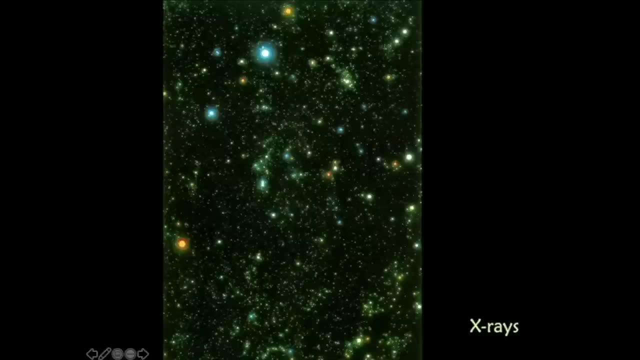 this is what makes up the x-ray background, that i studied for my background, that i studied for my background, that i studied for my when i was a student and i didn't know when i was a student and i didn't know when i was a student and i didn't know this. i was looking at the sum total of 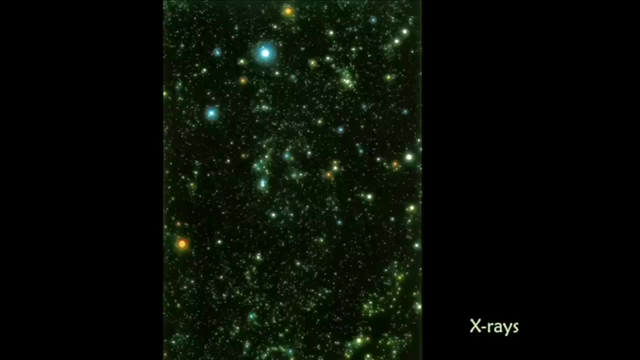 this. i was looking at the sum total of this. i was looking at the sum total of all the emission from accreting black, all the emission from accreting black, all the emission from accreting black, holes, holes, holes, and that's an xnm image where we're 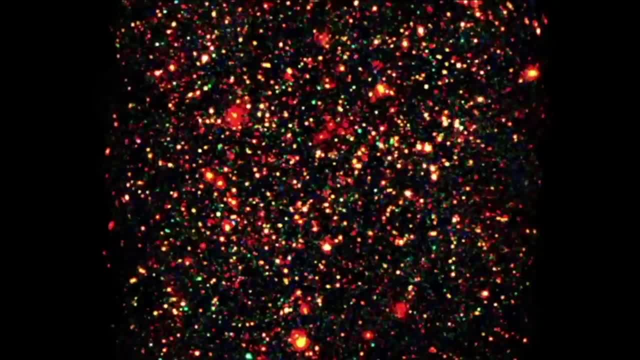 and that's an xnm image where we're and that's an xnm image where we're looking, looking, looking, now, now, now. this is an x-ray european satellite. this is an x-ray european satellite. this is an x-ray european satellite xmm, which shows us many, many accreting. 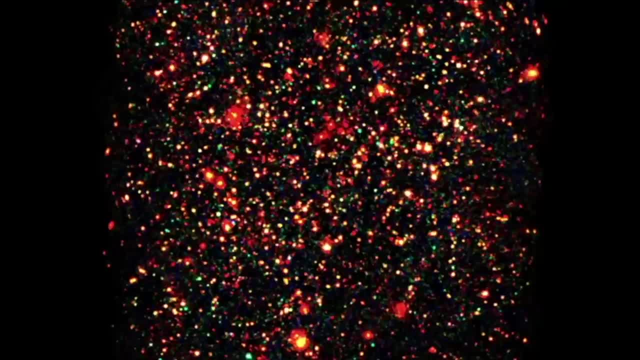 xmm, which shows us many, many accreting xmm, which shows us many, many accreting black holes in the sky, black holes in the sky, black holes in the sky, and and clusters of galaxies and and clusters of galaxies and and clusters of galaxies. and, by the way, there is an indian. 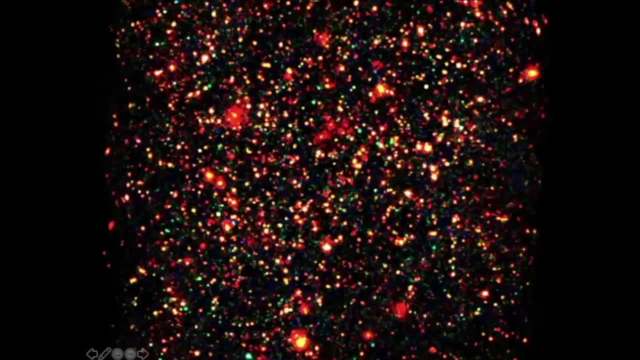 and, by the way, there is an indian. and, by the way, there is an indian satellite, astrosat, which is devoted to satellite astrosat, which is devoted to satellite astrosat, which is devoted to x-ray astronomy, and you can look that x-ray astronomy and you can look that. 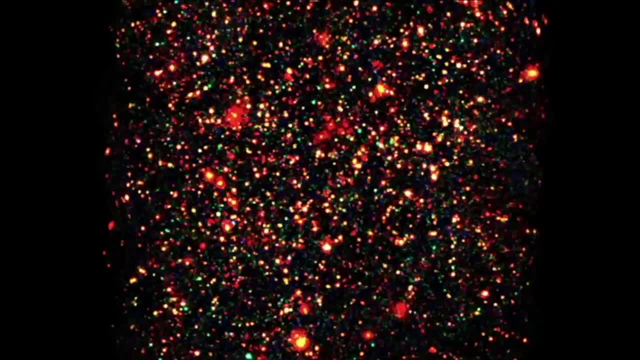 x-ray astronomy and you can look that up and see some exciting results from up. and see some exciting results from up and see some exciting results from there, there, there, this is a schematic of what it looks. this is a schematic of what it looks. this is a schematic of what it looks like with one of these accreting black. 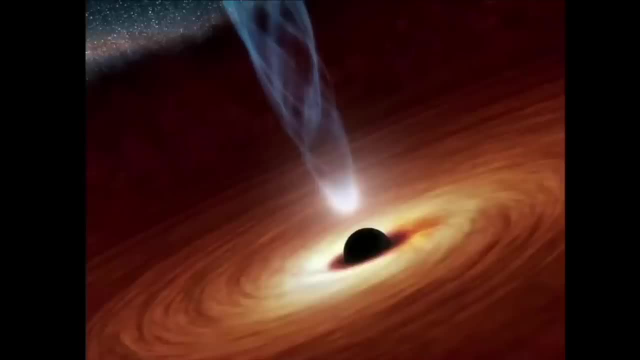 like with one of these accreting black, like with one of these accreting black holes, holes, holes, basically, basically. basically, the black hole is at the center, the black hole is at the center, the black hole is at the center and material is swirling around it. 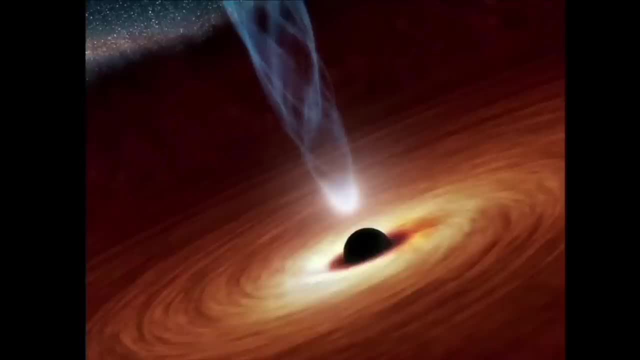 and material is swirling around it. and material is swirling around it because of angular momentum, everything because of angular momentum, everything because of angular momentum, everything sort of orbiting around everything else, sort of orbiting around everything else, sort of orbiting around everything else. you can't fall directly into a black hole. 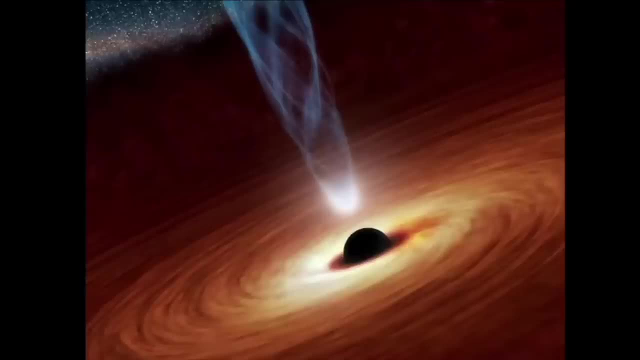 you can't fall directly into a black hole. you can't fall directly into a black hole. the sun is going around the earth. is the sun is going around the earth? is the sun is going around the earth? is going around the sun at 30 kilometers per 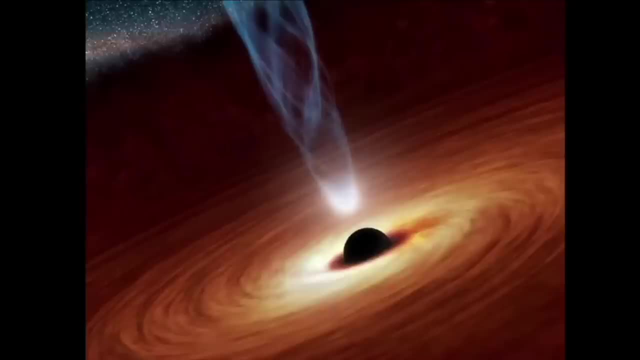 going around the sun at 30 kilometers per. going around the sun at 30 kilometers per second. it doesn't fall into the sun. second, it doesn't fall into the sun. second, it doesn't fall into the sun because you need to get rid of that. 30. 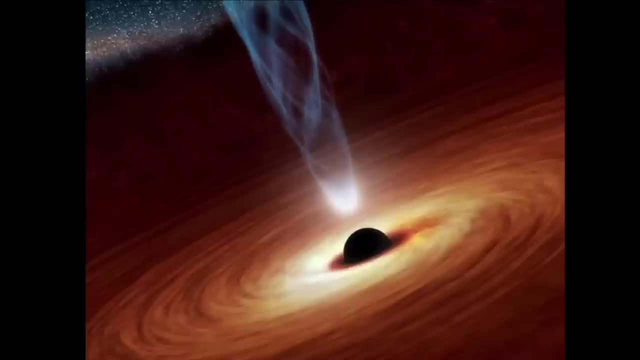 because you need to get rid of that 30, because you need to get rid of that 30. kilometers per second to do so, kilometers per second to do so, kilometers per second to do so. and indeed our most powerful rockets, and indeed our most powerful rockets, and indeed our most powerful rockets, can't get steady anything up. 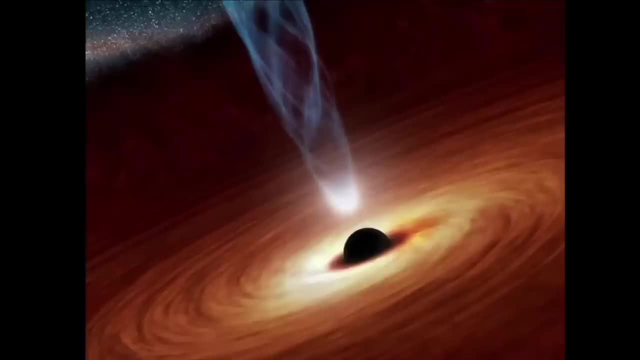 can't get steady anything up. can't get steady anything up to 30 kilometers per second. so we to 30 kilometers per second. so we to 30 kilometers per second. so we couldn't fire a missile into the sun. couldn't fire a missile into the sun. 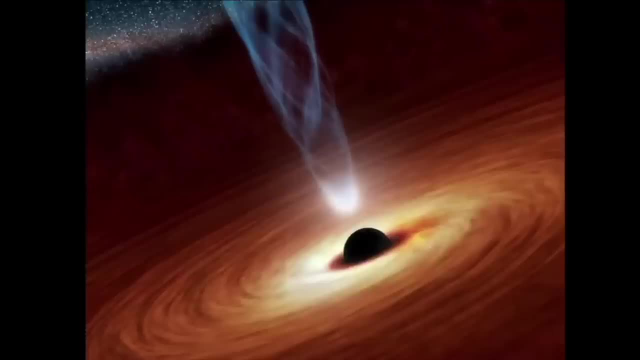 couldn't fire a missile into the sun, even if we wanted to do that. there are, even if we wanted to do that. there are, even if we wanted to do that there are ways of doing it, but it doesn't involve ways of doing it, but it doesn't involve 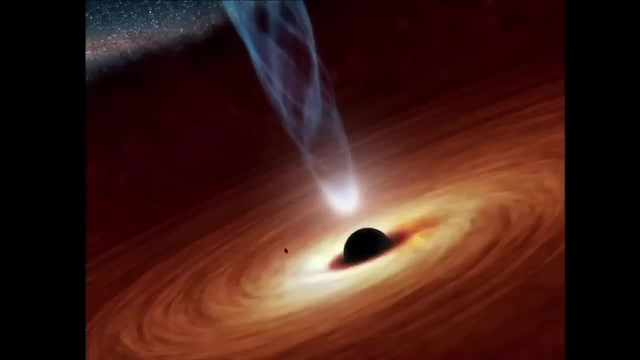 ways of doing it, but it doesn't involve firing it straight at the sun. firing it straight at the sun, firing it straight at the sun, and so angular momentum is preventing, and so angular momentum is preventing, and so angular momentum is preventing the matters going into the black hole. 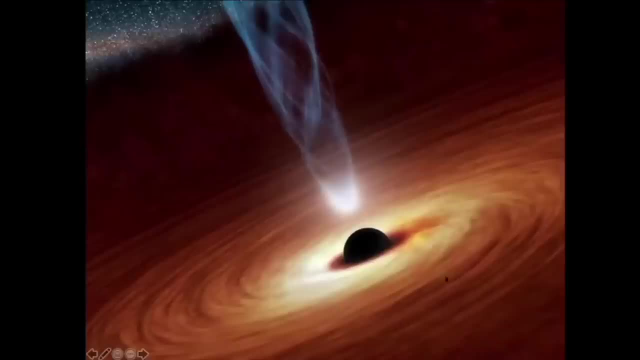 the matters going into the black hole, the matters going into the black hole, and it falls into this. disc discs are and it falls into this. disc discs are and it falls into this. disc discs are quite common in the universe and these quite common in the universe, and these. 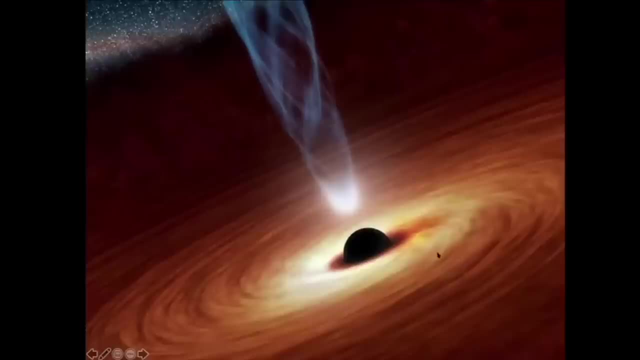 quite common in the universe. and these are the material in the disc as you go. are the material in the disc as you go. are the material in the disc as you go inwards: the material in you know inwards, inwards: the material in you know inwards. 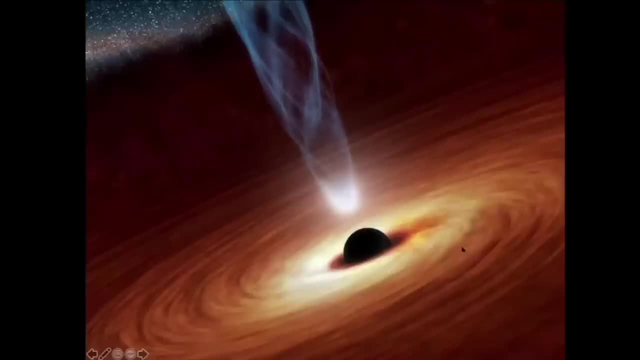 inwards. the material in, you know, inwards is moving faster than the material is moving, faster than the material is moving, faster than the material outwards. and therefore, if you've got some outwards and therefore if you've got some outwards, and therefore if you've got some friction, there's going to be a lot of. 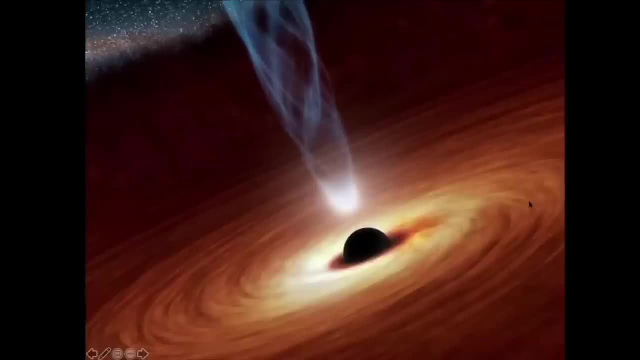 friction. there's going to be a lot of friction. there's going to be a lot of viscous energy release, and it gets hot viscous energy release and it gets hot viscous energy release and it gets hot and indeed these discs get very hot and indeed these discs get very hot. 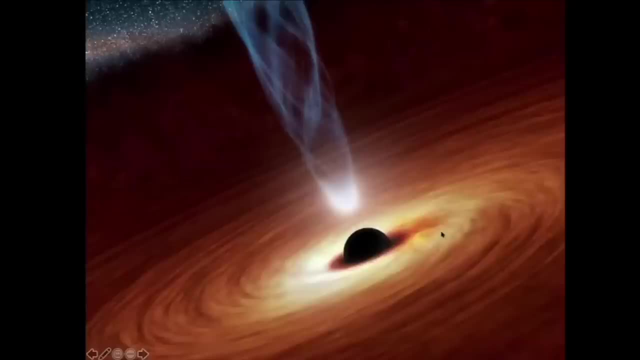 and indeed these discs get very hot. they've also got lots of strong magnetic. they've also got lots of strong magnetic. they've also got lots of strong magnetic fields and those fields and those fields and those magnetic fields get knotted up in the magnetic fields get knotted up in the 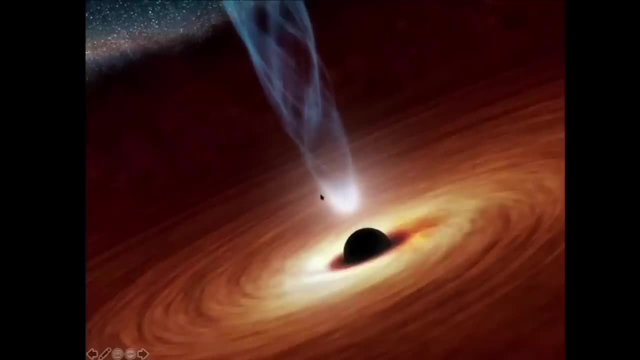 magnetic fields get knotted up in the center, center, center, and they release enormous amount of power, and they release enormous amount of power and they release enormous amount of power in a region we call the corona, in a region we call the corona, in a region we call the corona, and this is a very bright, hard x-ray. 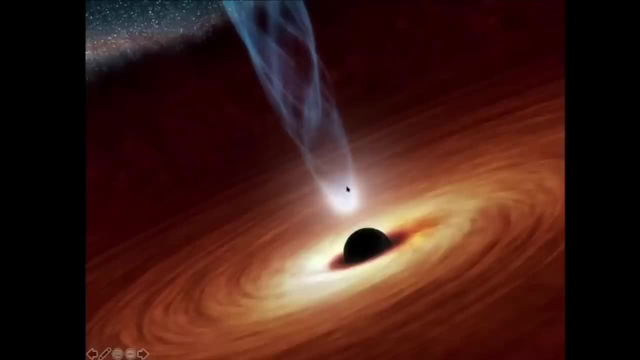 and this is a very bright, hard x-ray, and this is a very bright, hard x-ray source, a source of high energy extra source, a source of high energy extra source, a source of high energy extra x-rays- those x-rays then shine down. x-rays- those x-rays then shine down. 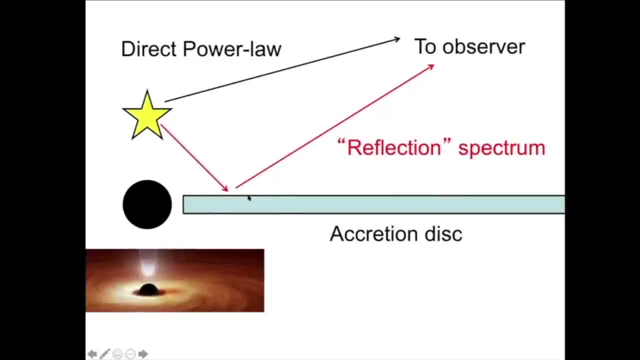 x-rays. those x-rays then shine down onto the accretion disk, onto the accretion disk, onto the accretion disk, and irradiate it, and they cause and irradiate it, and they cause, and irradiate it, and they cause fluorescence which we call the. 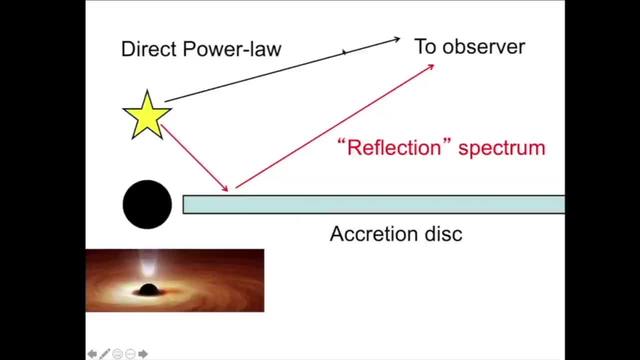 fluorescence, which we call the fluorescence, which we call the reflection spectrum. so the observer reflection spectrum, so the observer reflection spectrum. so the observer sees this hard x-ray emission and it sees this hard x-ray emission and it sees this hard x-ray emission and it also sees emission from the surface of. 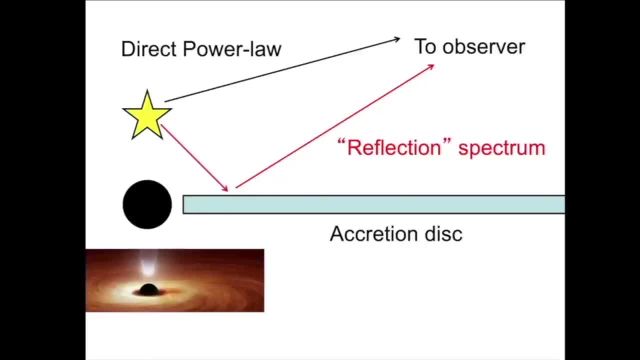 also sees emission from the surface of, also sees emission from the surface of the accretion disk, the accretion disk, the accretion disk, and we see that it also produces a very, and we see that it also produces a very and we see that it also produces a very strong iron line. 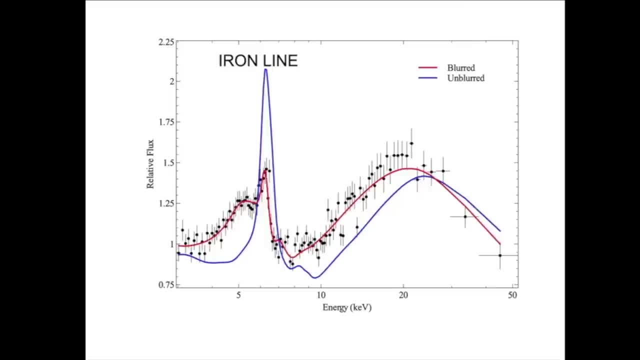 strong iron line, strong iron line, and this is a spectrum, one of my, and this is a spectrum one of my, and this is a spectrum one of my students made a few years back, students made a few years back, students made a few years back of the iron line from the 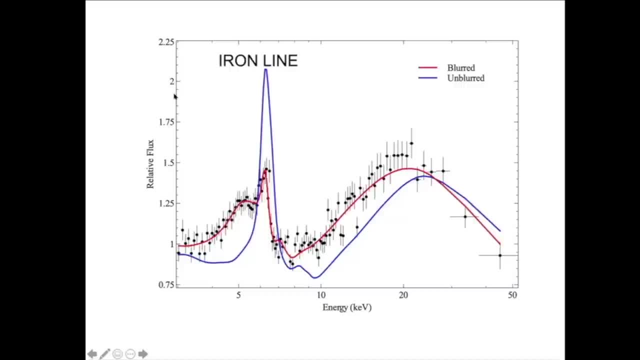 of the iron line, from the of the iron line, from the t, creating black hole, creating black hole, creating black hole. we were actually at and going around. we were actually at and going around. we were actually at and going around with the disc, with the disc, with the disc, but because we're outside the system, 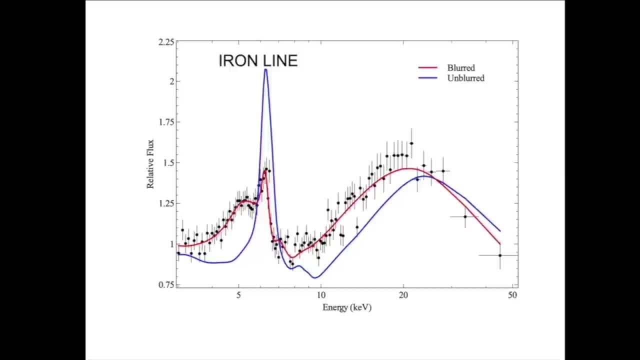 but because we're outside the system, but because we're outside the system, we're looking down at the emission which we're looking down at, the emission which we're looking down at, the emission which is swirling round, is swirling round, is swirling round and it's going up to half the speed of 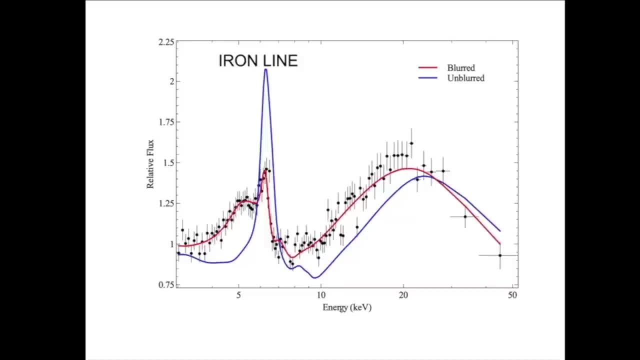 and it's going up to half the speed of, and it's going up to half the speed of light, which is what happens in accretion light, which is what happens in accretion light, which is what happens in accretion flow, flow, flow. then we're seeing large velocities and 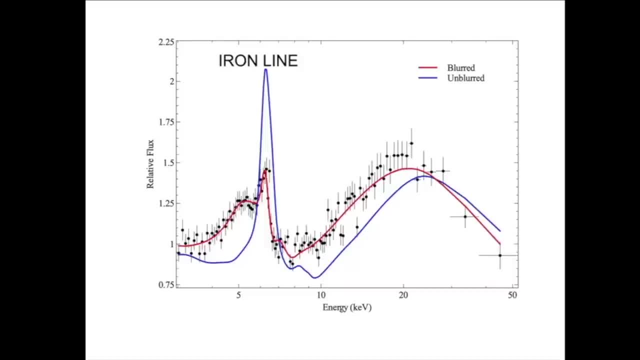 then we're seeing large velocities. and then we're seeing large velocities and there's a lot of doppler shift, which there's a lot of doppler shift, which there's a lot of doppler shift which broadens this iron line, broadens this iron line. 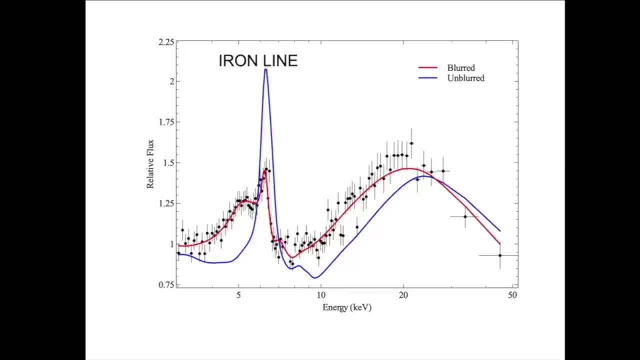 broadens this iron line, and then because we're very close to, and then because we're very close to, and then because we're very close to the black hole, there's an enormous the black hole. there's an enormous the black hole. there's an enormous amount of gravitational redshift. 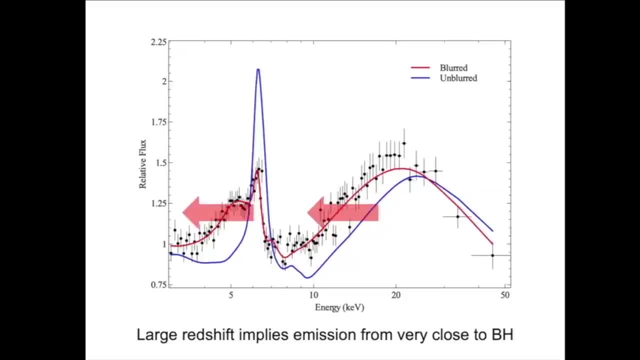 amount of gravitational redshift, amount of gravitational redshift and we can measure that redshift the and we can measure that redshift the and we can measure that redshift the amount of the redshift. we see amount of the redshift. we see amount of the redshift. we see, and the large redshift implies the. 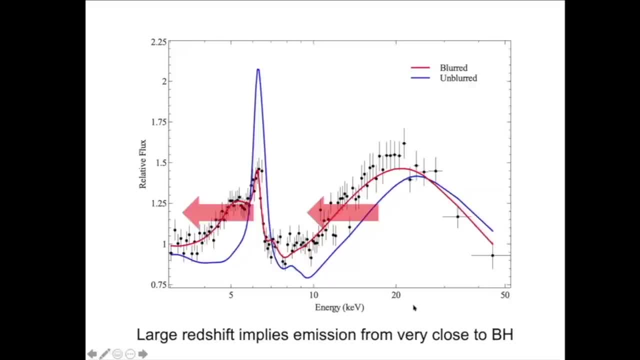 and the large redshift implies the and the large redshift implies the emission is, emission is emission is very close to the black hole if we say very close to the black hole. if we say very close to the black hole if we say the radius of the event horizon. 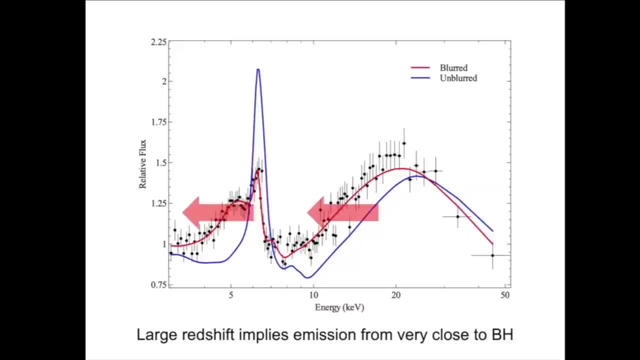 the radius of the event horizon. the radius of the event horizon is a gravitational radius. this emission is a gravitational radius. this emission is a gravitational radius. this emission is all coming, is all coming, is all coming from within two or three gravitational, from within two or three gravitational. 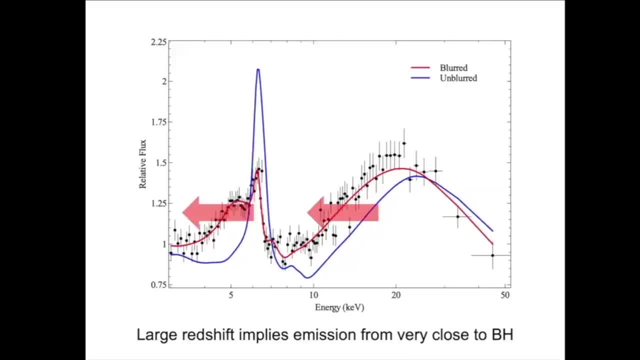 from within two or three gravitational radii. we're looking right in close radii. we're looking right in close radii. we're looking right in close to the black hole and we can start to to the black hole, and we can start to to the black hole and we can start to understand the flow of the matter. that's. 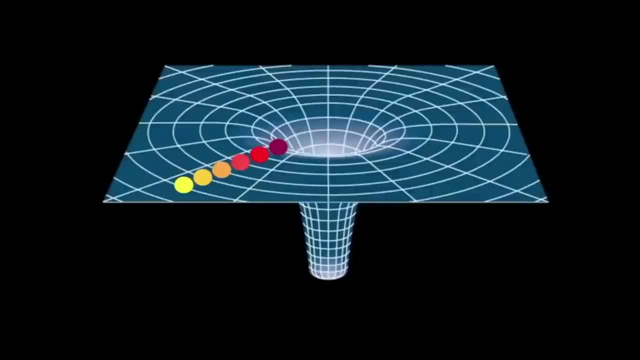 understand the flow of the matter. that's understand the flow of the matter that's close in, close in, close in and in terms of this object, we can, and in terms of this object, we can and in terms of this object we can actually measure the spin of the black. 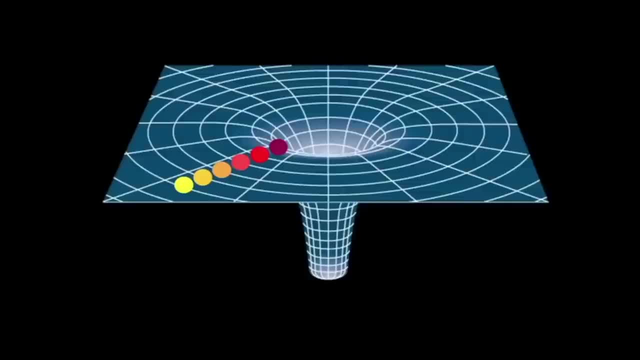 actually measure the spin of the black, actually measure the spin of the black hole, hole, hole. this is just to emphasize, if you can, this is just to emphasize, if you can, this is just to emphasize- if you can measure the red shift, then you can start to measure the spin. 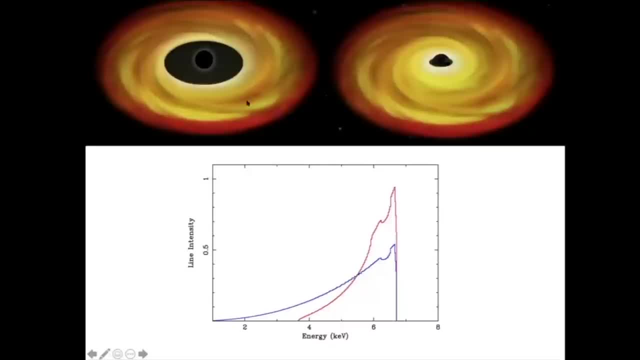 then you can start to measure the spin. then you can start to measure the spin and the way it works just briefly. and the way it works just briefly and the way it works just briefly, is the accretion flow around a non? is the accretion flow around a non? 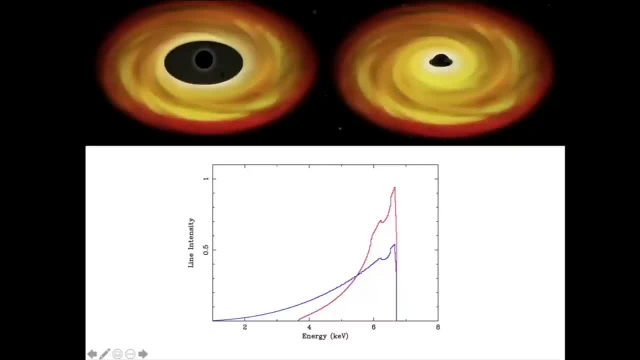 is the accretion flow around a non spinning black hole, the slant shield spinning black hole. the slant shield spinning black hole, the slant shield black hole, which is this one black hole, which is this one black hole, which is this one, has to stop, basically. 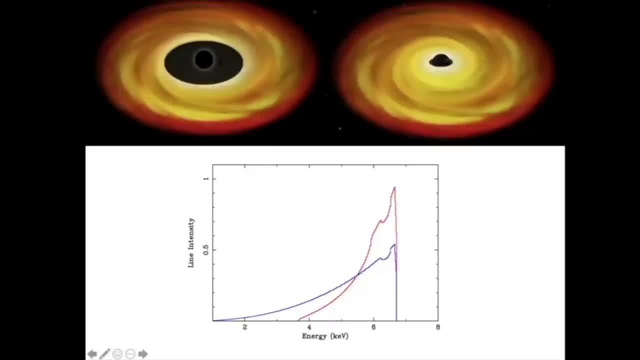 has to stop, basically has to stop, basically away from the black hole, and then away from the black hole, and then away from the black hole, and then there's an innermost radius, and it then there's an innermost radius, and it then there's an innermost radius and it then plunges inwards. 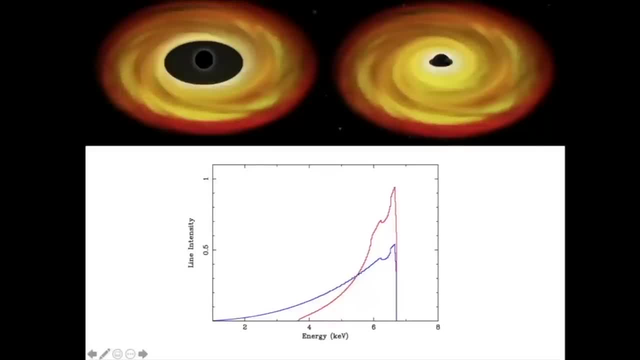 plunges inwards, plunges inwards, and that's due to the nature of the physics, and that's due to the nature of the physics, and that's due to the nature of the physics. but if you have a rapidly spinning, but if you have a rapidly spinning, 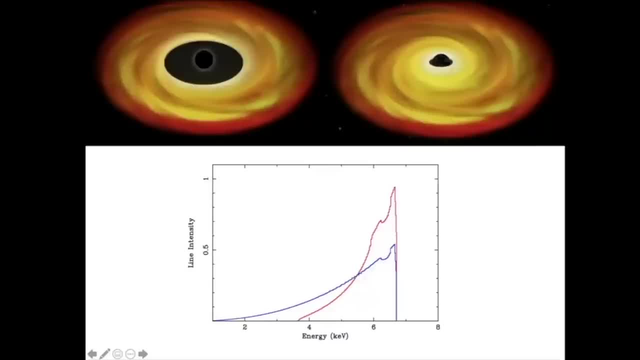 but if you have a rapidly spinning black hole, it drags the material in black hole. it drags the material in black hole. it drags the material in right close to it and you therefore get right close to it, and you therefore get right close to it and you therefore get the disc extending much further in. 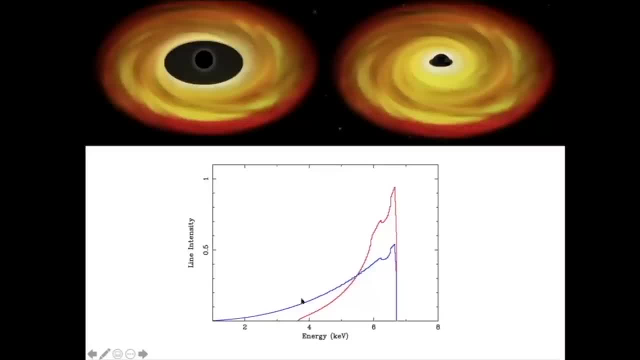 the disc extending much further in, the disc extending much further in, and that gives you more gravitational and that gives you more gravitational and that gives you more gravitational redshift. so the blue one here has got redshift. so the blue one here has got redshift. so the blue one here has got this and this is x-ray energies and the 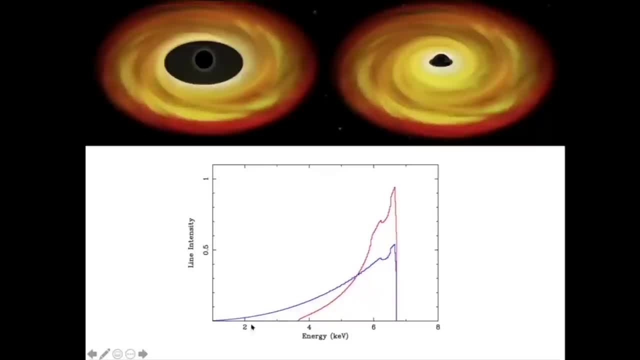 this and this is x-ray energies, and the this and this is x-ray energies. and the red shift means it's going to lower. red shift means it's going to lower. red shift means it's going to lower energies, energies, energies. this one is an emission line. you'd 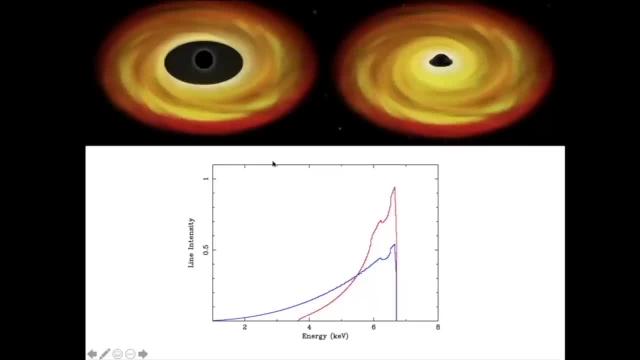 this one is an emission line you'd. this one is an emission line you'd expect to see from this disc and the red expect to see from this disc and the red expect to see from this disc. and the red is the one from that disc which is the. 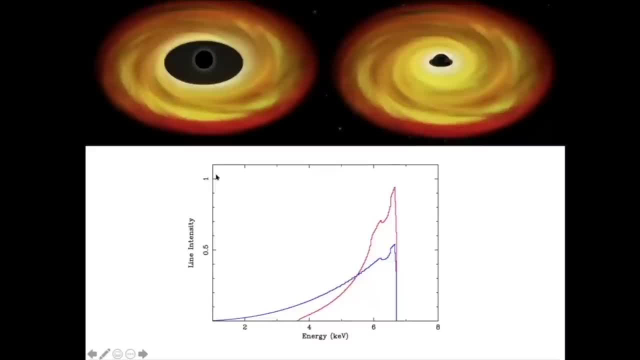 is the one from that disc which is the is the one from that disc which is the non-spinning one, and we're seeing in the non-spinning one and we're seeing in the non-spinning one and we're seeing in the previous plot, previous plot. 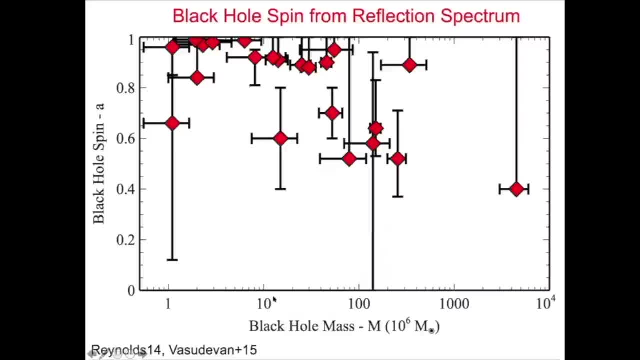 previous plot, something like this. so we know the spin, something like this. so we know the spin. something like this. so we know the spin is very high, is very high, and many of us have been working on and many of us have been working on and many of us have been working on this. 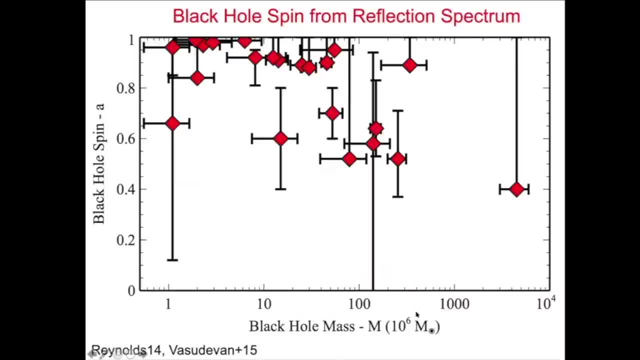 this, this coming up with the black hole spin, coming up with the black hole spin, coming up with the black hole spin and black hole mass for a very large and black hole mass for a very large and black hole mass for a very large number of blank holes, and we hope to do. 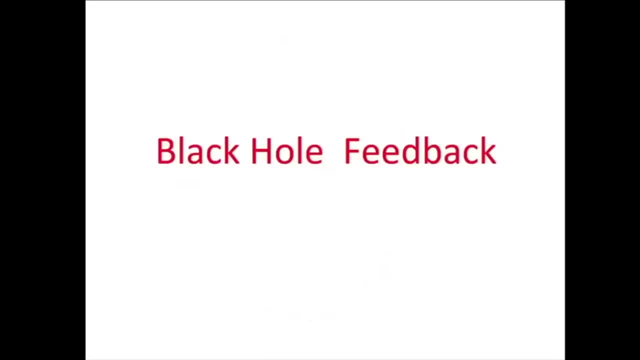 number of blank holes and we hope to do number of blank holes and we hope to do more over the more, over the more, over the coming years. now i talked about black coming years. now i talked about black coming years. now i talked about black holes at work. 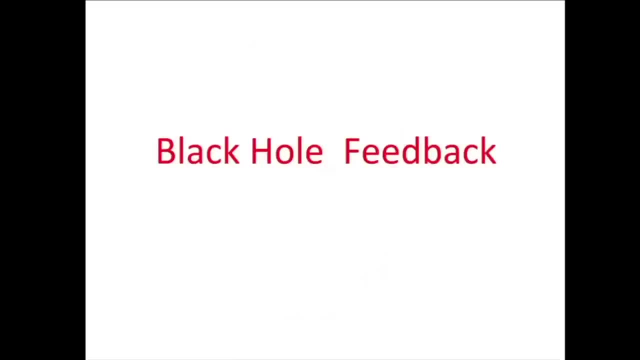 holes at work, holes at work. what's going on with black holes when? what's going on with black holes when? what's going on with black holes when they are in the middle of these objects? they are in the middle of these objects. they are in the middle of these objects. there's something called black hole. 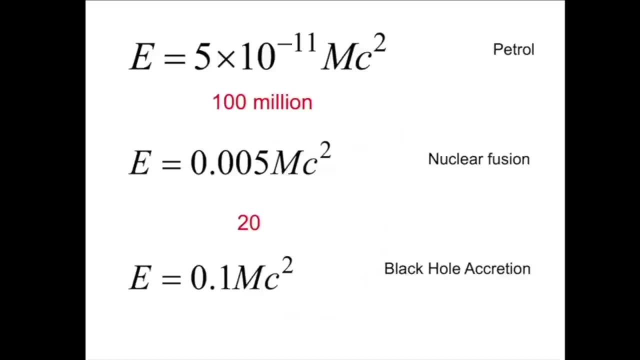 there's something called black hole. there's something called black hole feedback, feedback, feedback. i want to talk now about the amount of. i want to talk now about the amount of. i want to talk now about the amount of energy you get out from dropping energy you get out from dropping. 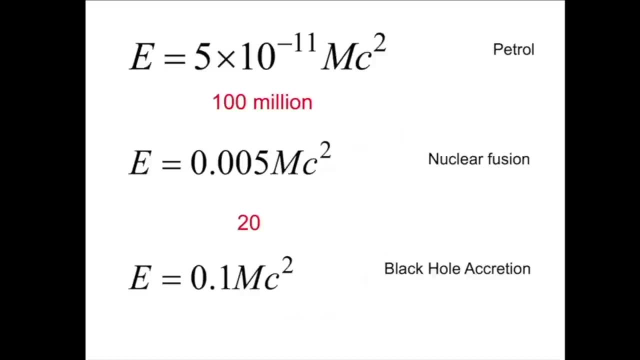 energy you get out from dropping material into a black hole, material into a black hole, material into a black hole. okay, and i'm going to use an equation. okay, and i'm going to use an equation. okay, and i'm going to use an equation now. e equals m. 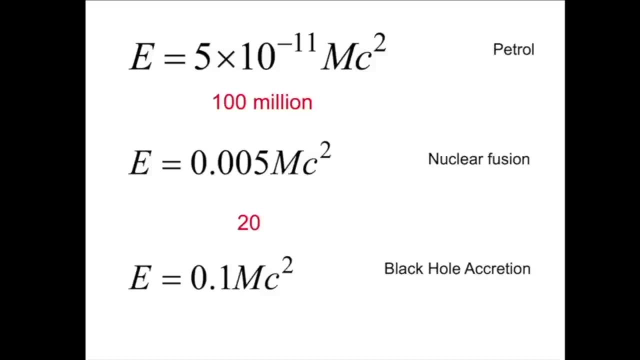 now e equals m. now e equals m c. you all heard that equation e equals m. you all heard that equation e equals m. you all heard that equation e equals m and the basically the rest mass energy and the basically the rest mass energy and the basically the rest mass energy of something. 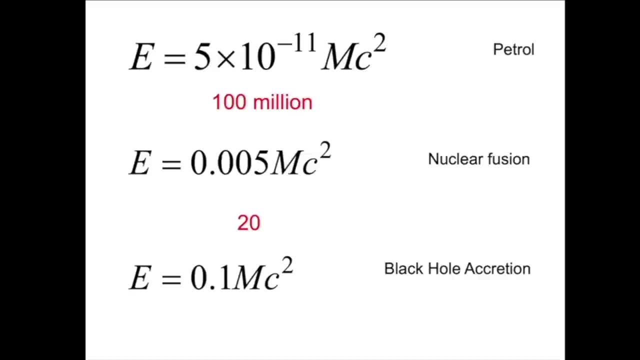 of something, of something, is m c squared? is m c squared? is m c squared when you think about chemical reactions, when you think about chemical reactions, when you think about chemical reactions, there is energy release, there is energy release, there is energy release and that energy is associated. 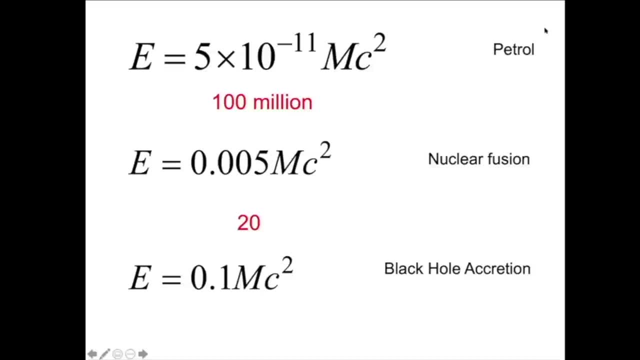 and that energy is associated and that energy is associated, there is a very tiny change in the mass. there is a very tiny change in the mass. there is a very tiny change in the mass of the objects. if you could actually of the objects, if you could actually 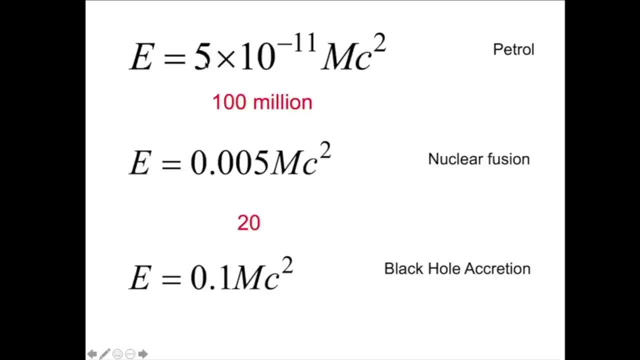 of the objects, if you could actually measure it, measure it, measure it. the energy has a mass and that the energy has a mass, and that the energy has a mass and that corresponds to 5, corresponds to 5, corresponds to 5 times 10, to the minus 11 mc squared. 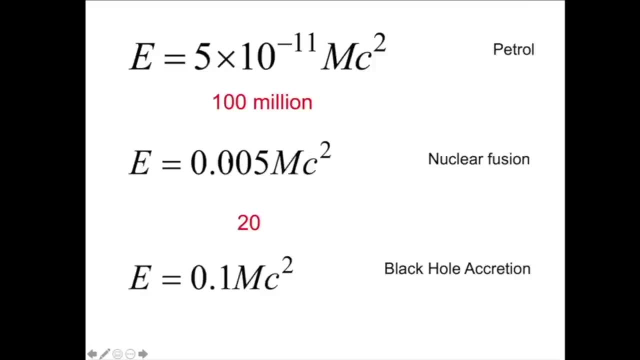 times 10 to the minus 11 mc squared. times 10 to the minus 11 mc squared: that's petrol. that's petrol. that's petrol. nuclear fusion is 0.005 mc squared. nuclear fusion is 0.005 mc squared. nuclear fusion is 0.005 mc squared. black hole accretion is 0.1 mc squared. 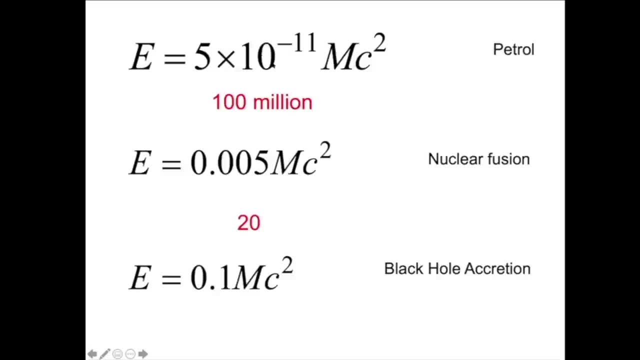 black hole accretion is 0.1 mc squared. black hole accretion is 0.1 mc squared. okay, okay, okay. so this means but the difference between. so this means but the difference between. so this means: but the difference between these two is 100 million the difference. 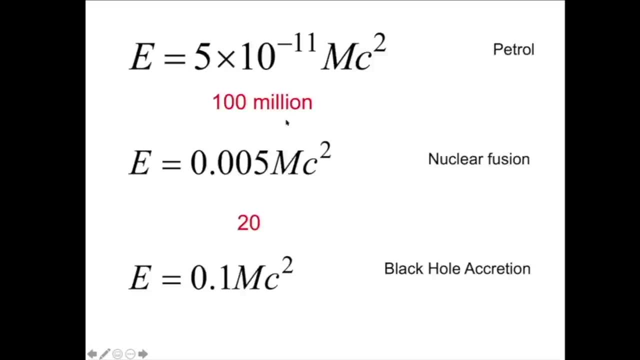 these two is 100 million. the difference these two is 100 million. the difference there is there is, there is 20.. so this means that if you 20.. so this means that if you 20.. so this means that if you, so that would be 2 000 million or 2. 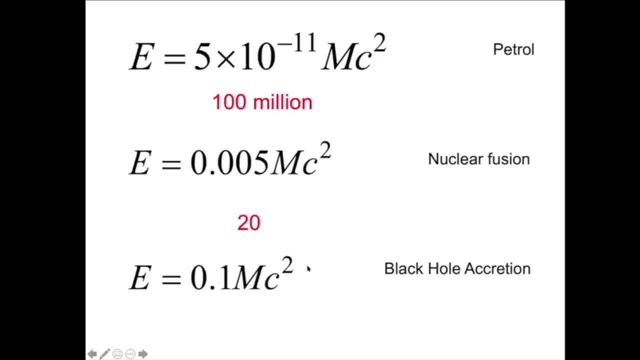 so that would be 2 000 million, or 2, so that would be 2 000 million or 2 billion, billion, billion. so actually, if you could have a black, so actually if you could have a black, so actually if you could have a black hole in your car. 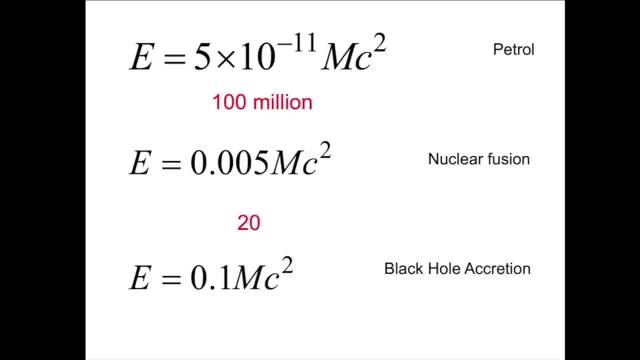 hole in your car. hole in your car. you could go 2 billion times further on. you could go 2 billion times further on. you could go 2 billion times further on a gallon of petrol, a gallon of petrol, a gallon of petrol, but of course you couldn't get a black. 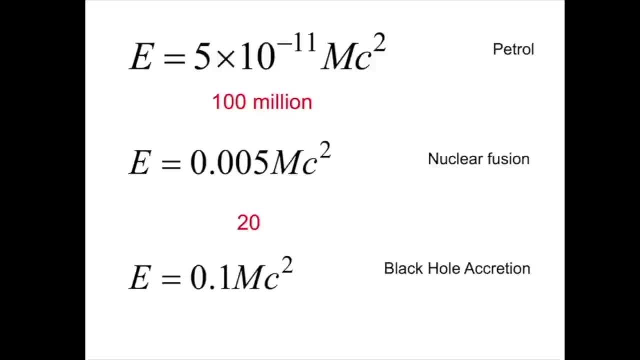 but of course you couldn't get a black. but of course you couldn't get a black hole in your car. nobody knows how to do hole in your car. nobody knows how to do hole in your car. nobody knows how to do anything like that. i don't anticipate. 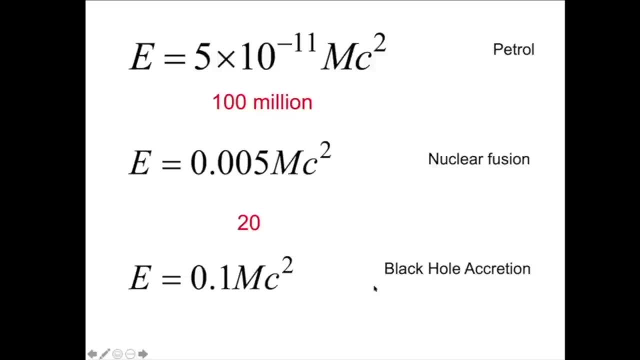 anything like that. i don't anticipate anything like that. i don't anticipate this being the solution to the energy, this being the solution to the energy, this being the solution to the energy crisis, or anything like that. i'm just crisis, or anything like that, i'm just. 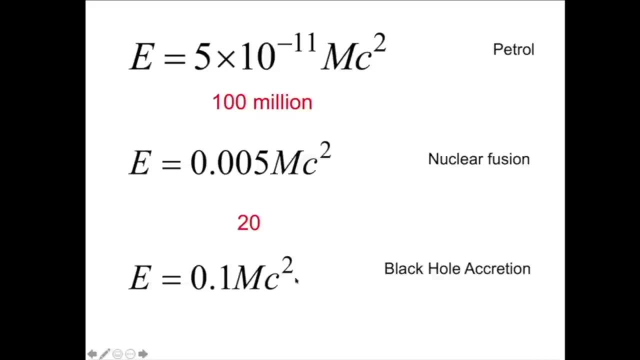 crisis or anything like that. i'm just making the point here. it's that this is making the point here. it's that this is making the point here. it's that this is the the the most efficient way of releasing energy. most efficient way of releasing energy, most efficient way of releasing energy, apart from pure matter: antimatter. 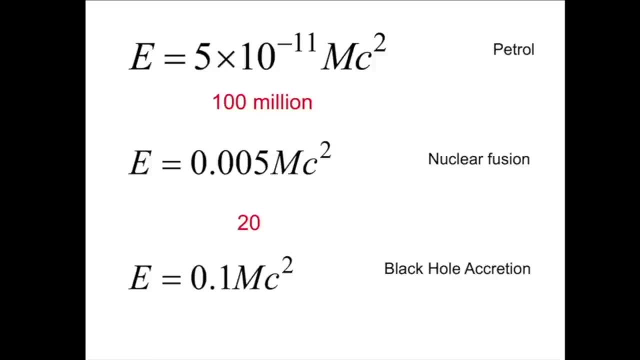 apart from pure matter, antimatter. apart from pure matter, antimatter. annihilation which can achieve mc squared, annihilation which can achieve mc squared, annihilation which can achieve mc squared, but of course there's very little, but of course there's very little, but of course there's very little antimatter in our universe. and i would 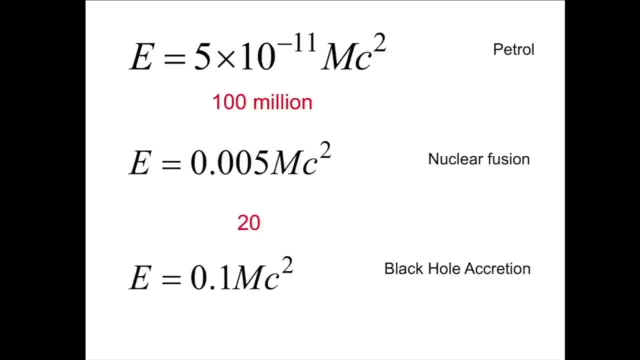 antimatter in our universe and i would antimatter in our universe and i would say thankfully, say thankfully, say thankfully there's very little antimatter in our. there's very little antimatter in our. there's very little antimatter in our universe. if you want to get very 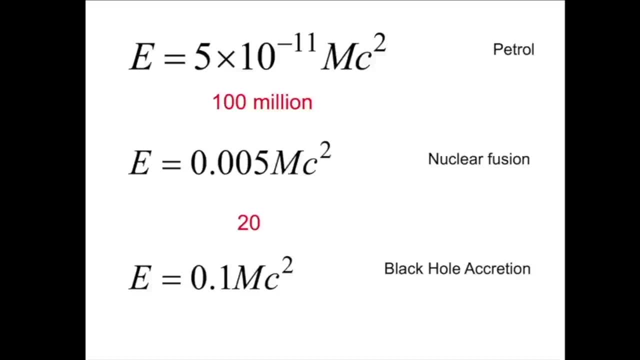 universe. if you want to get very universe, if you want to get very large energies, you can get out them out, large energies, you can get out them out, large energies. you can get out them out through black hole accretion. it's why, through black hole accretion, it's why 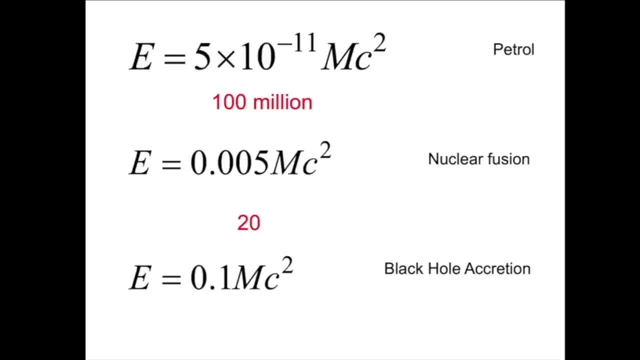 through black hole accretion. it's why, when matter falls into a black hole, it, when matter falls into a black hole, it, when matter falls into a black hole, it can lead to extremely high luminosities, can lead to extremely high luminosities, can lead to extremely high luminosities, and it's something to ponder about that. 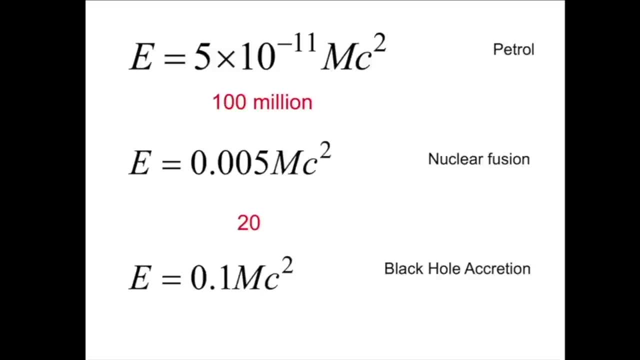 and it's something to ponder about that, and it's something to ponder about that: black holes are the blackest, darkest black holes are the blackest, darkest black holes are the blackest, darkest objects in the universe, objects in the universe, objects in the universe and immediately around them. 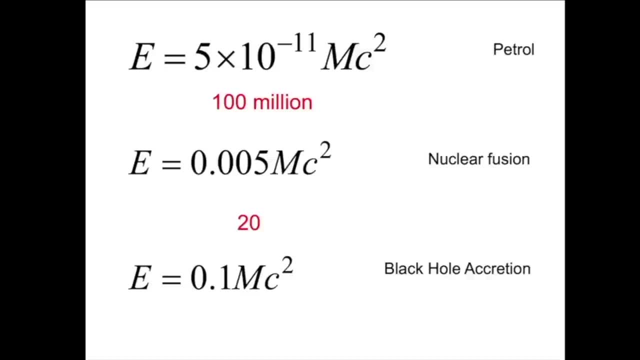 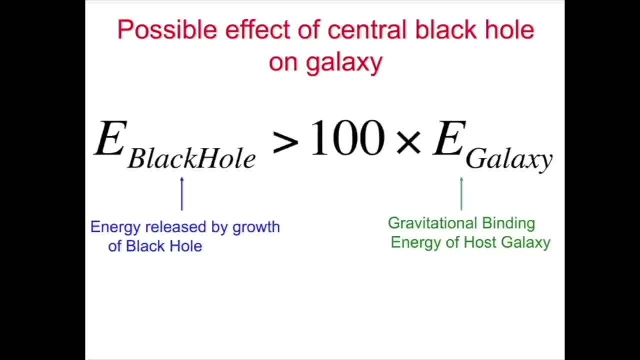 and immediately around them, and immediately around them, they can be the most luminous objects. they can be the most luminous objects. they can be the most luminous objects in the universe, in the universe, in the universe. they're right next to each other. now, what we can do is look at the amount. 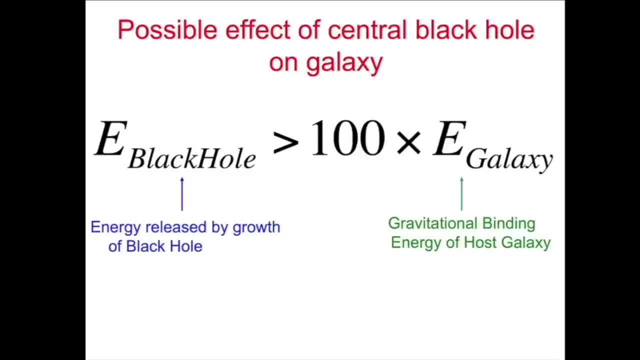 now, what we can do is look at the amount. now, what we can do is look at the amount of energy, of energy, of energy that's released as we grow a black hole. that's released as we grow a black hole that's released as we grow a black hole. black holes have grown in mass up to a 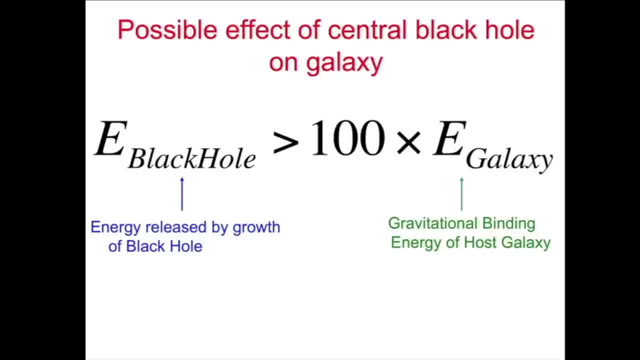 black holes have grown in mass up to a black holes have grown in mass up to a billion solar masses, billion solar masses, billion solar masses, through accretion by matter, falling through accretion by matter, falling through accretion by matter, falling into them, into them. 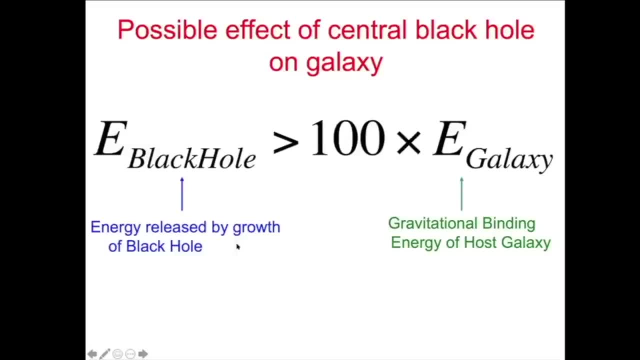 into them and the total energy release to grow a and the total energy release to grow a and the total energy release to grow a black hole in the galaxy, black hole in the galaxy, black hole in the galaxy actually is more than a hundred times, actually is more than a hundred times. 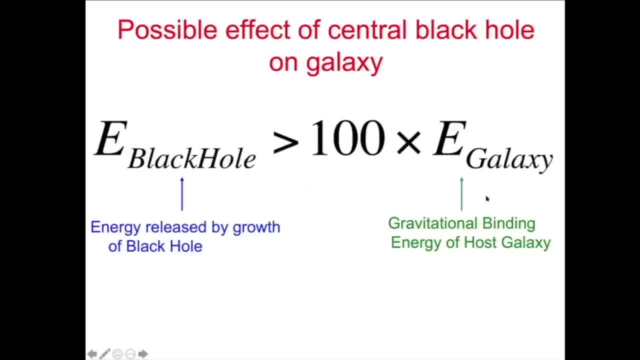 actually is more than a hundred times bigger than the bigger than the bigger than the binding energy of the galaxy. what i mean binding energy of the galaxy, what i mean binding energy of the galaxy, what i mean by that is by that is by that is, how much energy would i need to throw the? 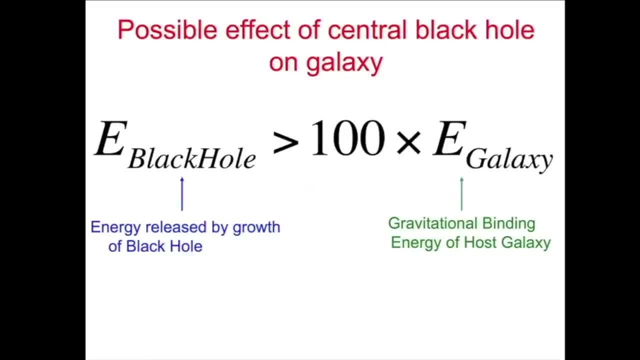 how much energy would i need to throw the? how much energy would i need to throw the galaxy galaxy, galaxy back out into space, in in its constituent, back out into space, in in its constituent. back out into space, in in its constituent parts, parts, parts? now, that means, if we can couple some of 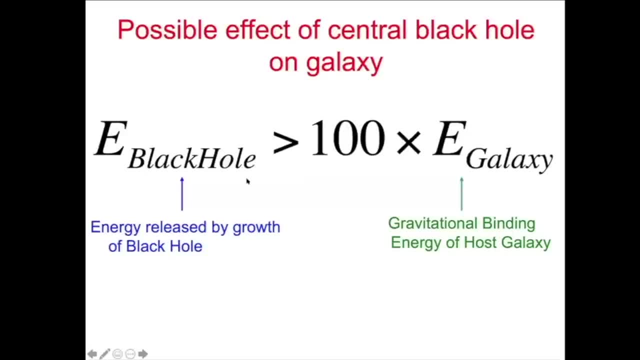 now. that means if we can couple some of now. that means if we can couple some of that energy to the galaxy, we can affect that energy to the galaxy. we can affect that energy to the galaxy. we can affect the galaxy, the galaxy, the galaxy. now we can't couple the energy from the. 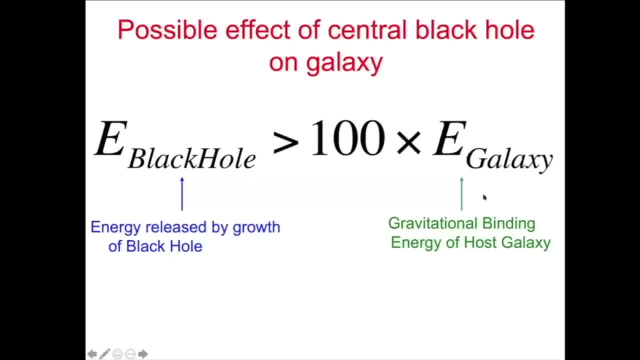 now we can't couple the energy from the now we can't couple the energy from the black hole, black hole, black hole- to the distant stars in the galaxy, to the distant stars in the galaxy, to the distant stars in the galaxy. there's no way of doing it, there's. 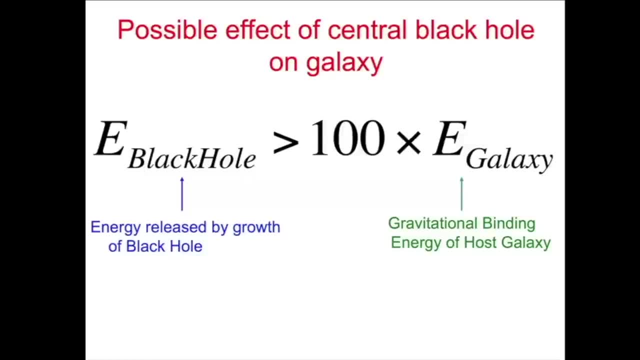 there's no way of doing it. there's? there's no way of doing it. there's galaxy: the stars are far too small. galaxy, the stars are far too small. galaxy, the stars are far too small and massive to be. you know you can't. and massive to be. you know you can't. 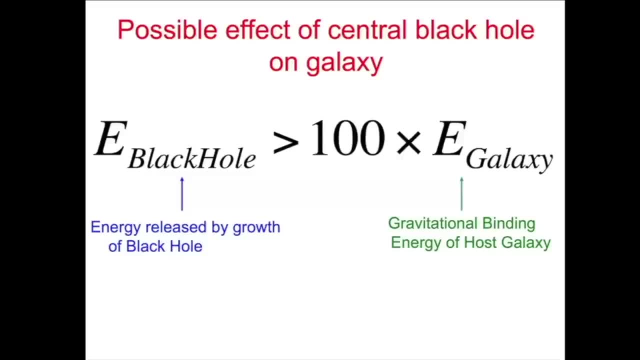 and massive to be. you know you can't. there's no way you can make them. there's no way you can make them. there's no way you can make them interact. but what you can do is to interact. but what you can do is to interact, but what you can do is to affect, affect the gas in the galaxy. 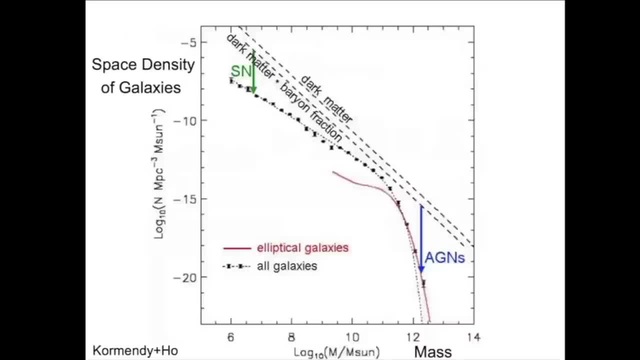 affect, affect the gas in the galaxy. affect, affect the gas in the galaxy, and that's where this next plot comes. and that's where this next plot comes and that's where this next plot comes. in it looks like a complicated plot and in it looks like a complicated plot and 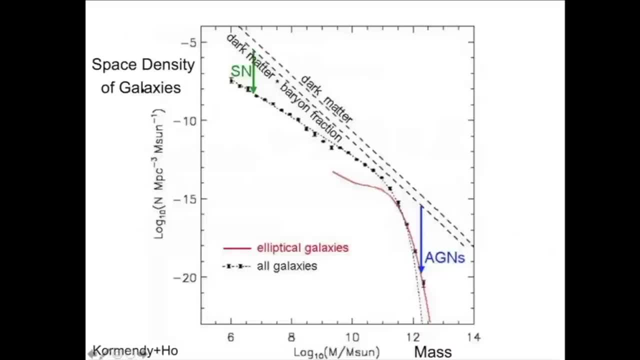 in. it looks like a complicated plot and i'm sorry about that. i'm sorry about that. i'm sorry about that, but it's actually very simple. it's, but it's actually very simple. it's, but it's actually very simple. it's actually the space density of galaxies. 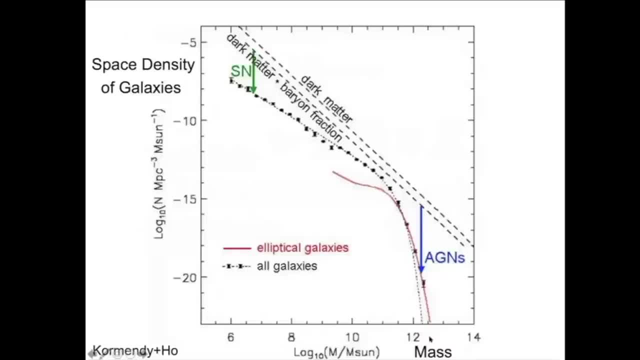 actually the space density of galaxies, actually the space density of galaxies as a function of the mass, and it's just as a function of the mass. and it's just as a function of the mass. and it's just a log log and you don't need to look at. 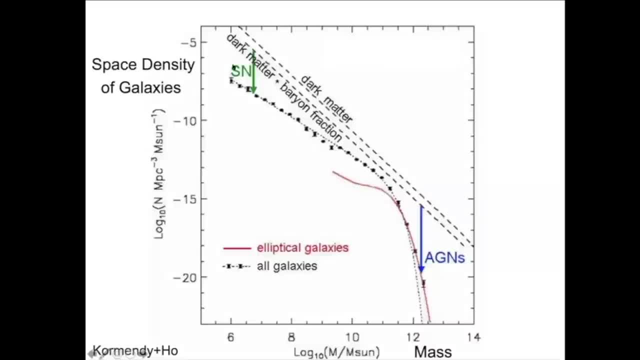 a log log and you don't need to look at a log log and you don't need to look at the units or anything like that, the units or anything like that, the units or anything like that. so there are lots of small galaxies in. so there are lots of small galaxies in. 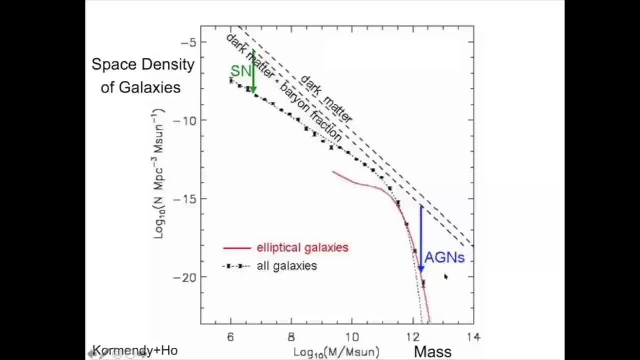 so there are lots of small galaxies in the universe, a very small few big the universe, a very small few big the universe, a very small few big galaxies in the universe, galaxies in the universe, galaxies in the universe. now, naively, you would actually expect. now, naively, you would actually expect. 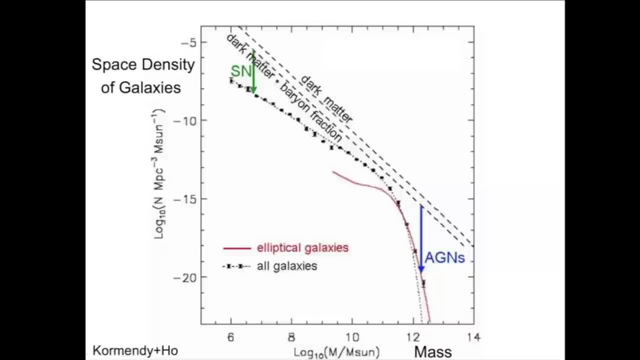 now, naively, you would actually expect that the distribution of the space, that the distribution of the space, that the distribution of the space density of galaxies with mass density, of galaxies with mass density of galaxies with mass, to parallel that the dark matter, i'm not. to parallel that the dark matter, i'm not. 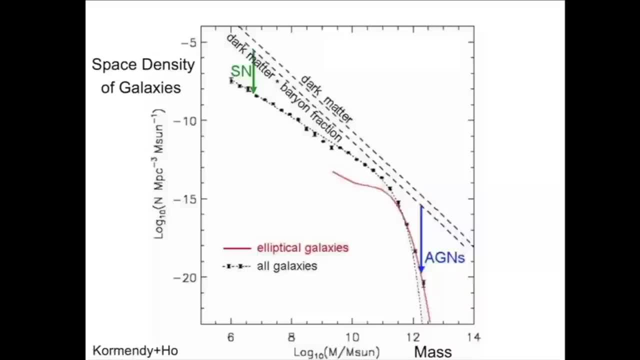 to parallel that: the dark matter. i'm not going to talk about going to talk, about going to talk about what dark matter is, because i don't know what dark matter is, because i don't know what dark matter is, because i don't know. but there's something in the universe. 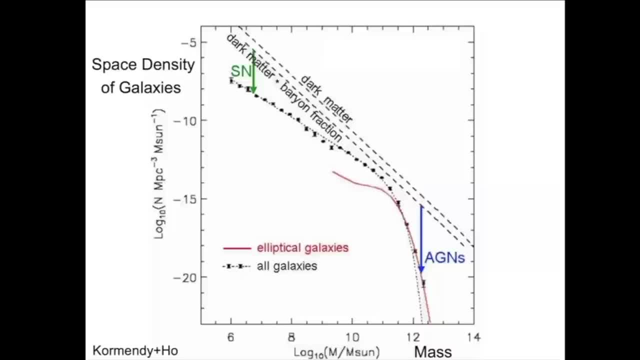 but there's something in the universe, but there's something in the universe called dark matter, that only interacts, called dark matter, that only interacts, called dark matter, that only interacts with us through gravity, with us through gravity, with us through gravity. we can't see it, which is why it's called. 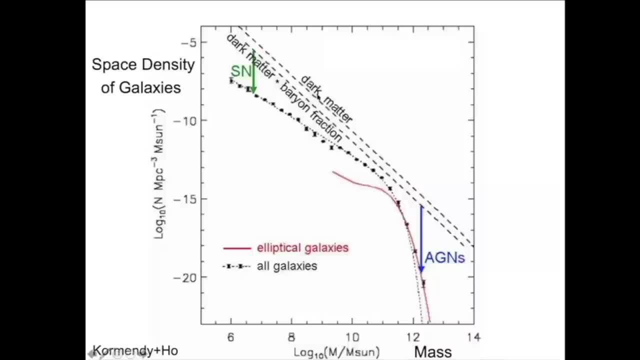 we can't see it, which is why it's called we can't see it, which is why it's called dark matter, dark matter, dark matter now. dark matter now. dark matter now. dark matter in the universe, in the universe, in the universe has grown and clumped together. it's 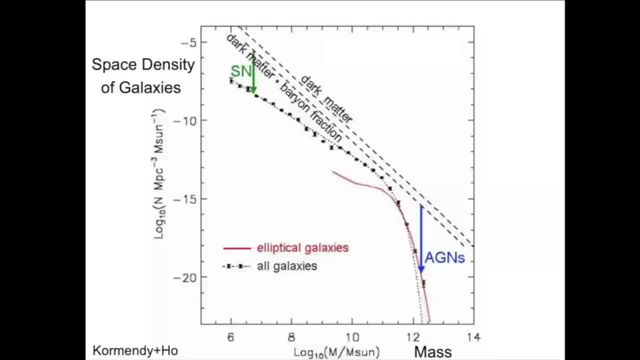 has grown and clumped together. it's has grown and clumped together. it's formed a whole distribution of clumps in formed, a whole distribution of clumps in formed, a whole distribution of clumps in the universe. we can infer that and we the universe. we can infer that and we. 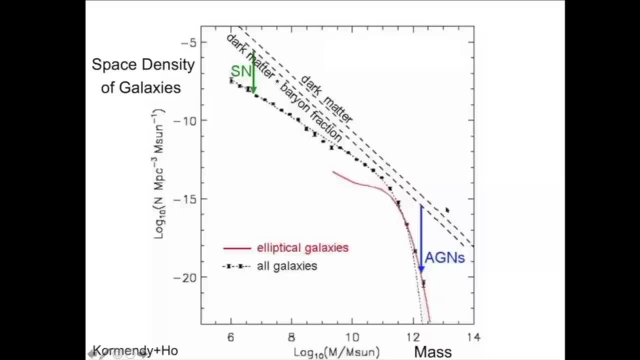 the universe. we can infer that and we know what it looks like and basically know what it looks like and basically know what it looks like and basically that's what that spectrum is that comes. that's what that spectrum is that comes. that's what that spectrum is that comes down there. 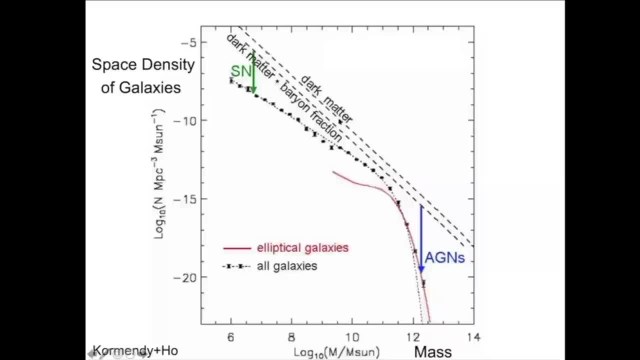 down there, down there, then, when you, then, when you, then, when you drop matter, when the matter in the drop matter, when the matter in the drop matter, when the matter in the universe, the gas in the universe, the universe, the gas in the universe, the universe, the gas in the universe, the baryons as we call them. 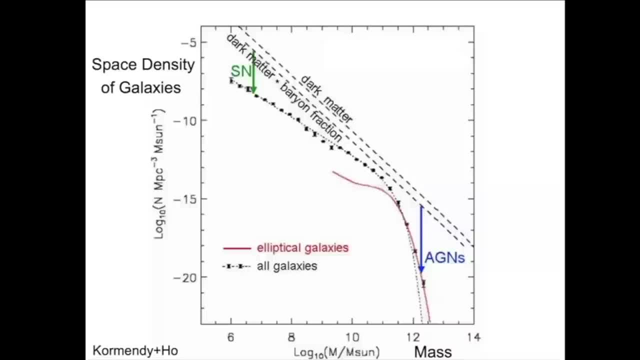 baryons as we call them. baryons as we call them, they will then fall into these potential. they will then fall into these potential. they will then fall into these potential wells of the clumps of dark matter. wells of the clumps of dark matter. 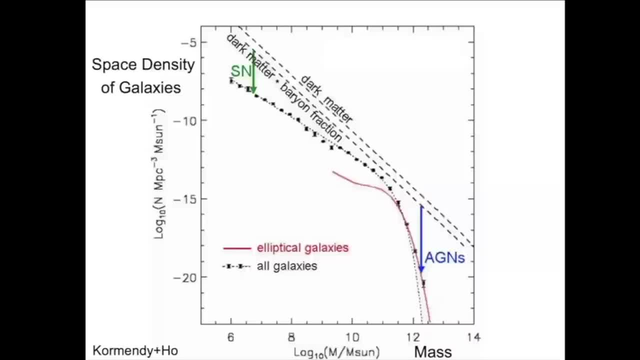 wells, of the clumps of dark matter, and if they can cool and form stars, and if they can cool and form stars, and if they can cool and form stars, we then call them galaxies, we then call them galaxies, we then call them galaxies, and so we would expect all galaxies. 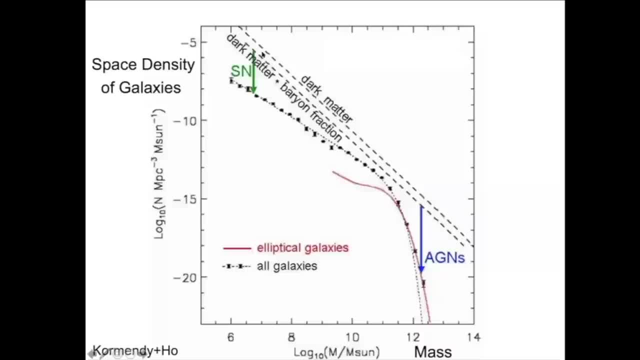 and so we would expect all galaxies, and so we would expect all galaxies to have the spectrum that looks like, to have the spectrum that looks like, to have the spectrum that looks like this, this, this, if that's all there was to galaxy, if that's all there was to galaxy. 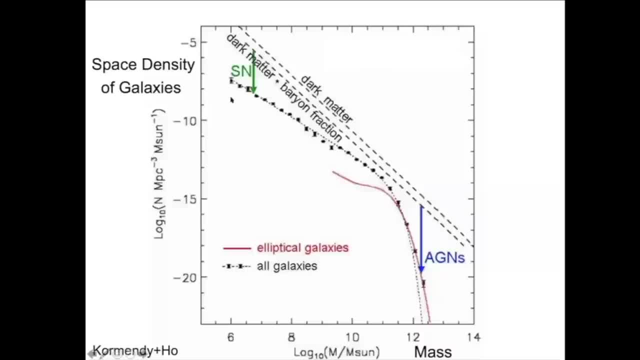 if that's all there was to galaxy formation, formation, formation, instead of which we see something, instead of which we see something, instead of which we see something looking like the points like this, looking like the points like this, looking like the points like this: there are very few very massive galaxies. 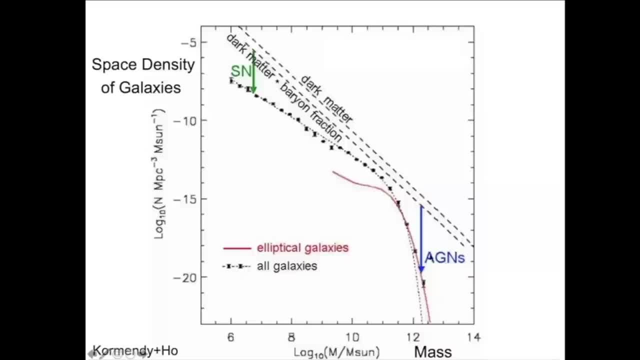 there are very few very massive galaxies. there are very few very massive galaxies. that's rather weird, but we now think that's rather weird. but we now think that's rather weird, but we now think that's due to active galactic nuclei. that's due to active galactic nuclei. 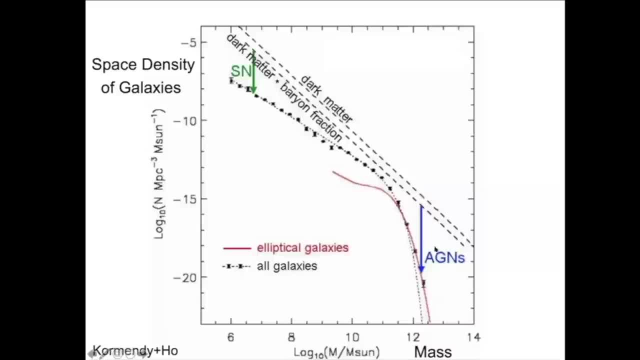 that's due to active galactic nuclei black holes. at the centers of these black holes, at the centers of these black holes, at the centers of these galaxies, galaxies, galaxies have blown most of the gas out back, have blown most of the gas out back, have blown most of the gas out back out of the galaxy and stopped them making. 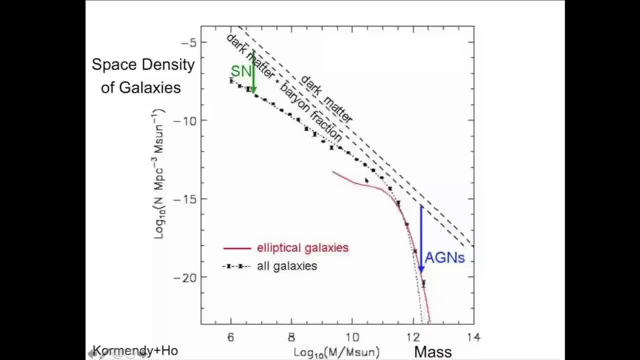 out of the galaxy and stopped them making out of the galaxy and stopped them making so many stars. because this is really a so many stars, because this is really a so many stars, because this is really a mass of stars in galaxies, mass of stars in galaxies, mass of stars in galaxies and similarly, at low. 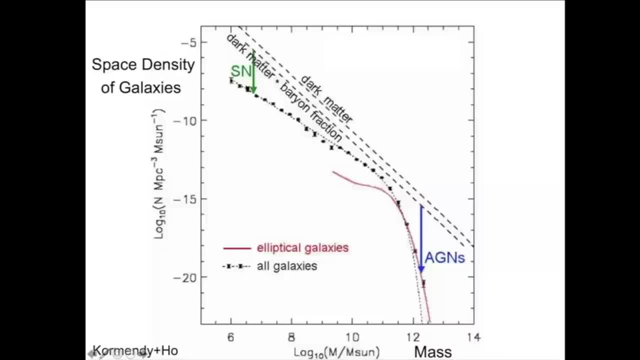 and similarly at low, and similarly at low masses. it's- we think it's supernovae masses. it's we think it's supernovae masses. it's we think it's supernovae- blew it out, blew it out, blew it out. so there's what is known as feedback. 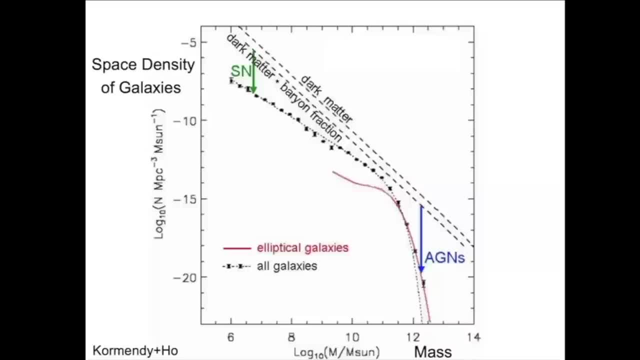 so there's what is known as feedback. so there's what is known as feedback taking place, taking place, taking place where black holes at the center are, where black holes at the center are, where black holes at the center are feeding energy and momentum back out, feeding energy and momentum back out. 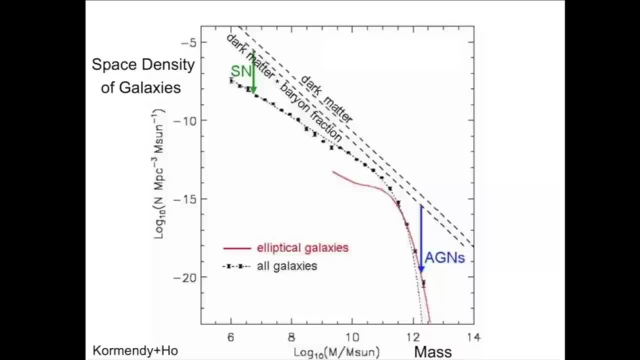 feeding energy and momentum back out into the galaxies, into the galaxies, into the galaxies, which is affecting, uh the masses of, which, is affecting, uh, the masses of which is affecting, uh, the masses of those galaxies, those galaxies, those galaxies, the elliptical galaxies in the universe, the elliptical galaxies in the universe. 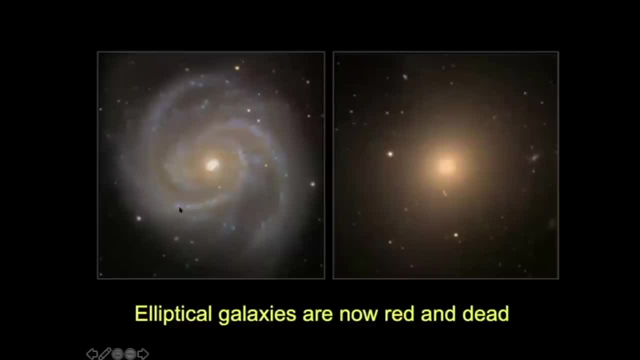 the elliptical galaxies in the universe are now red and dead, are now red and dead, are now red and dead. the spiral galaxies are full of blue. the spiral galaxies are full of blue. the spiral galaxies are full of blue arms and stars. like that, they're young. 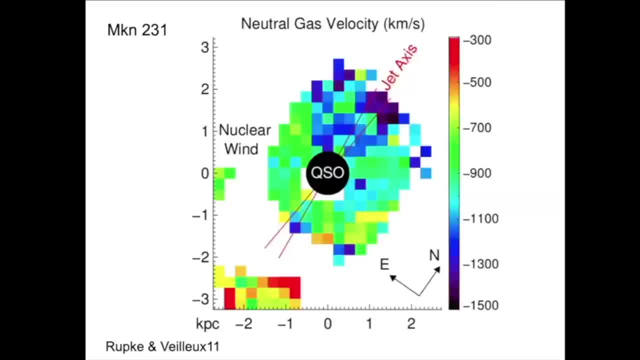 arms and stars like that. they're young arms and stars like that. they're young stars that are forming and evidence that things are blown away. and evidence that things are blown away and evidence that things are blown away from galaxies, from galaxies, from galaxies into the galaxies by um. 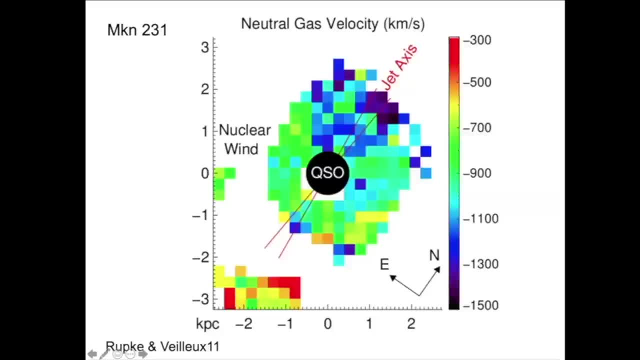 into the galaxies by um, into the galaxies by um, in particular, winds from the nucleus is, in particular, winds from the nucleus is, in particular, winds from the nucleus is. this is a quasar. this is a quasar. this is a quasar that's relatively near to us. 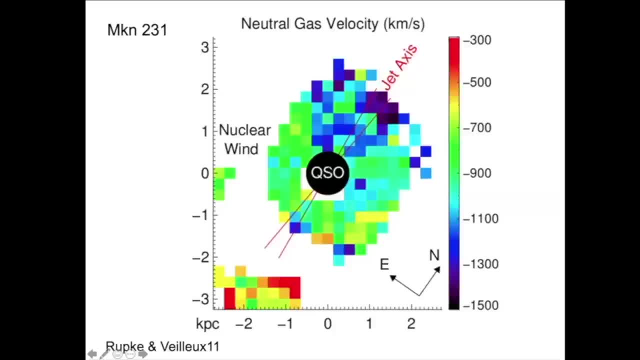 that's relatively near to us. that's relatively near to us and somebody's gone and looked in and somebody's gone and looked in and somebody's gone and looked in detail, detail, detail, with at the spectra of gas around the, with at the spectra of gas around the. 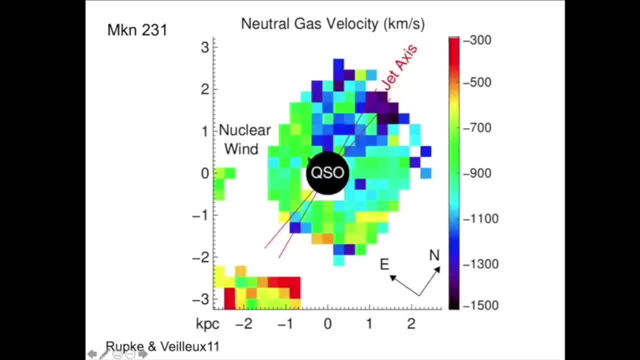 with at the spectra of gas around the center of that center, of that center of that nucleus, and compared to the velocity of nucleus, and compared to the velocity of nucleus, and compared to the velocity of the stars which are not the stars, which are not the stars which are not shown at all in um this image. 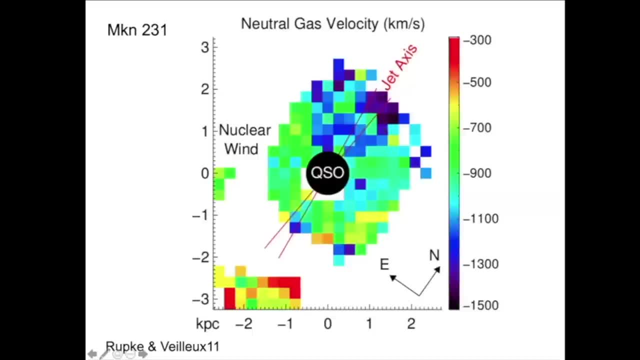 shown at all in um this image, shown at all in um this image, this representation. we see that the this representation, we see that the this representation. we see that the all of these points have got negative. all of these points have got negative. all of these points have got negative velocities, some of them very large. 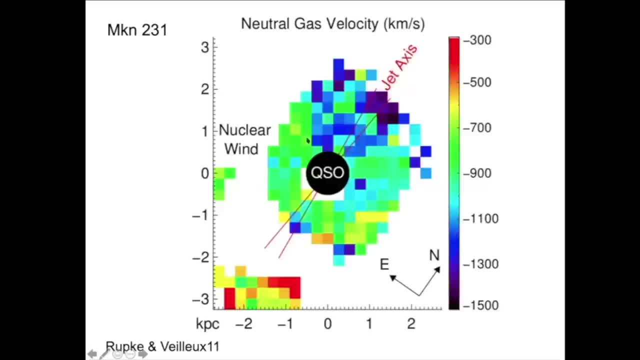 velocities, some of them very large velocities, some of them very large, thousands, well over a thousand kilometers, thousands, well over a thousand kilometers, thousands, well over a thousand kilometers per second for the gas. this is a per second for the gas. this is a per second for the gas. this is a measurement of the gas near the center of. 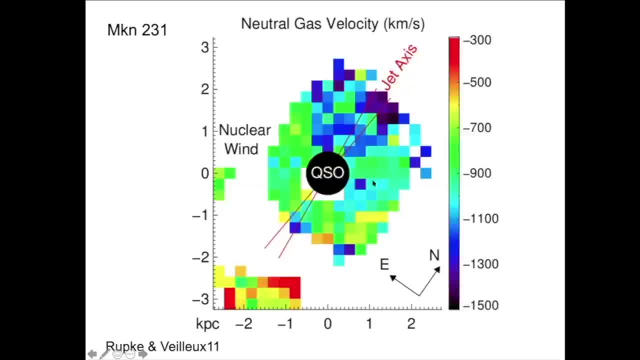 measurement of the gas near the center of measurement of the gas near the center of the galaxy, the galaxy, the galaxy, and basically it's coming out at a very and basically it's coming out at a very and basically it's coming out at a very high velocity, velocities of a thousand. 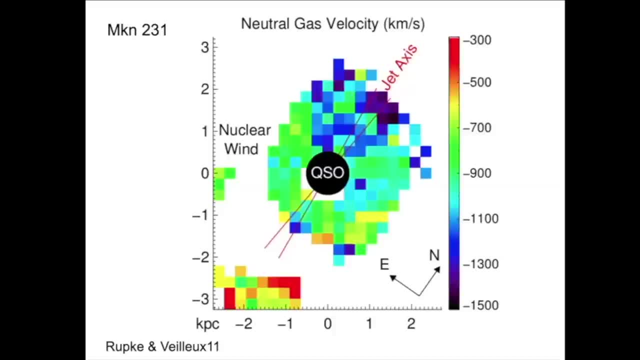 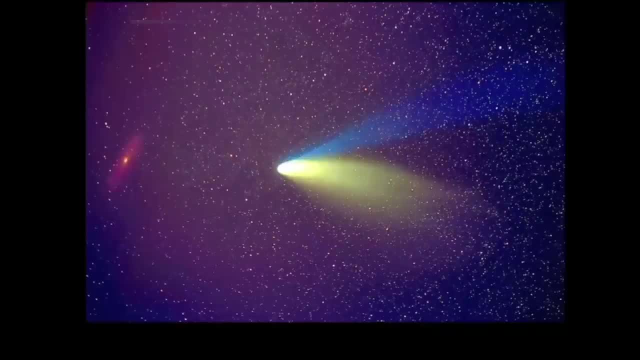 high velocity, velocities of a thousand. high velocity velocities of a thousand kilometers per second are very difficult. kilometers per second are very difficult. kilometers per second are very difficult to sustain, to sustain, to sustain due to stellar processes in a galaxy, due to stellar processes in a galaxy, due to stellar processes in a galaxy. another process which is important. 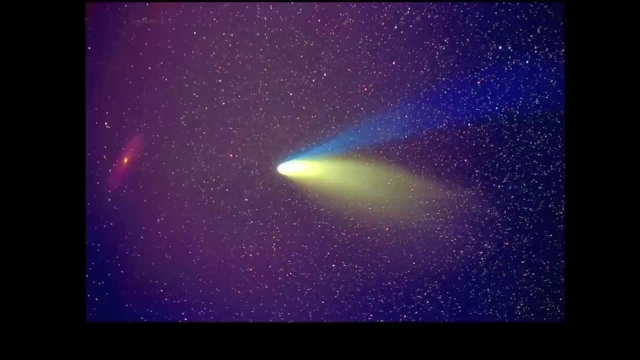 another process which is important, another process which is important, shown just in projection near the, shown just in projection near the, shown just in projection near the andromeda galaxy. but i like it because andromeda galaxy, but i like it because andromeda galaxy, but i like it because it's of this coincidence. 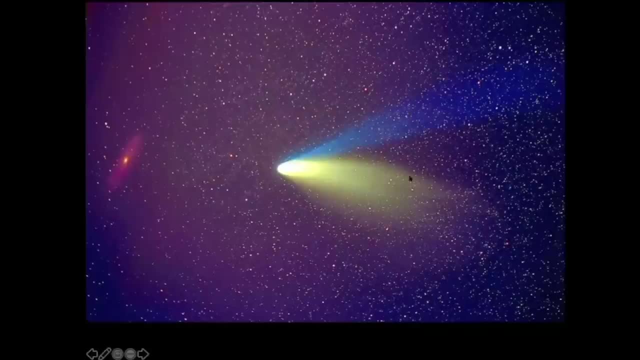 it's of this coincidence. it's of this coincidence that it's got two tails and the tail. i'm that it's got two tails and the tail. i'm that it's got two tails and the tail i'm interested in is this one, the dust tail. 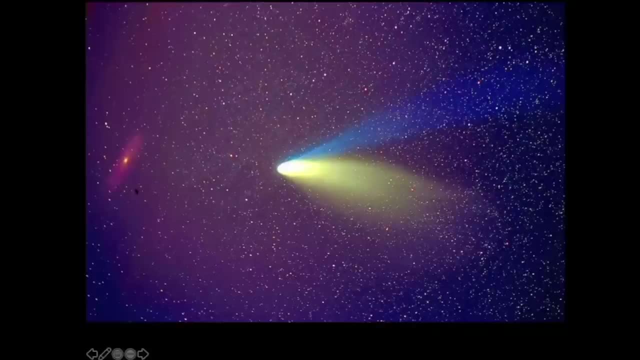 interested in? is this one the dust tail interested in? is this one the dust tail? and the sun happens to be over on the and the sun happens to be over on the and the sun happens to be over on the left. you can't see it in this image and. 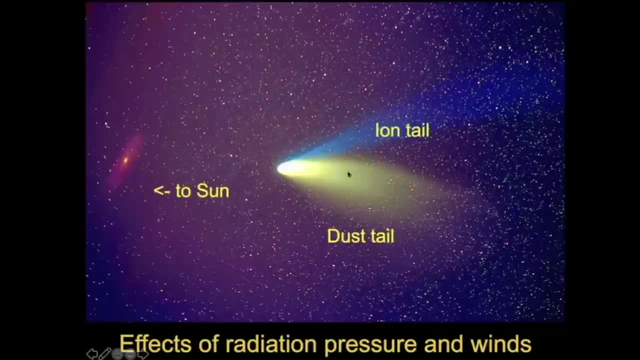 left, you can't see it in this image and left, you can't see it in this image. and basically, basically, basically, the dust tail is caused by radiation. the dust tail is caused by radiation. the dust tail is caused by radiation pressure from the sun, pressure from the sun. 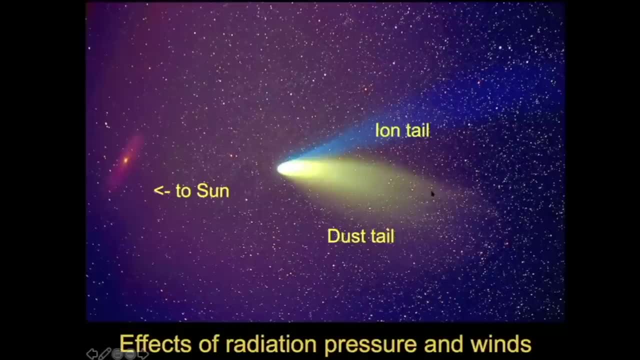 pressure from the sun which pushes the dust from the comet out, which pushes the dust from the comet out, which pushes the dust from the comet out, away from it, forming this wonderful tail. away from it. forming this wonderful tail. away from it. forming this wonderful tail, the iron tail is caused by the wind from. 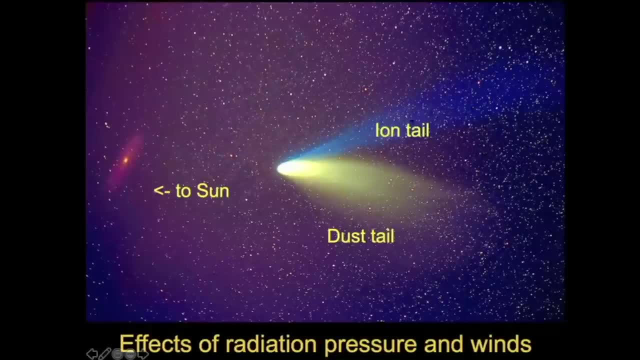 the iron tail is caused by the wind from. the iron tail is caused by the wind from the sun, the solar wind, the sun, the solar wind, the sun, the solar wind, and picking up ions in the comet and and picking up ions in the comet and and picking up ions in the comet and taking them out as well. 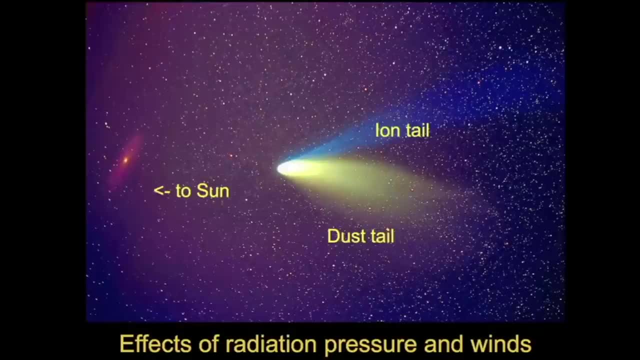 taking them out as well, taking them out as well. so a lot of this, the radiation pressure. so a lot of this, the radiation pressure, so a lot of this, the radiation pressure, and winds push gas out and winds push gas out, and winds push gas out, and that's probably what's happening in. 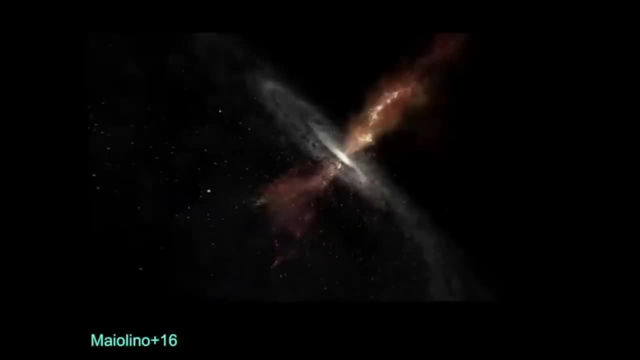 and that's probably what's happening in and that's probably what's happening in these active galaxies, these active galaxies, these active galaxies. and this is just showing a schematic in, and this is just showing a schematic in, and this is just showing a schematic in work i did with roboto. 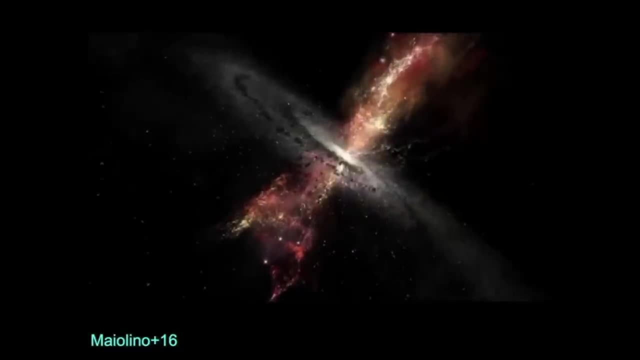 work i did with roboto work i did with roboto maolino, and we ended up with this press maolino. and we ended up with this press maolino and we ended up with this press release, release release. press release of a paper we had in. 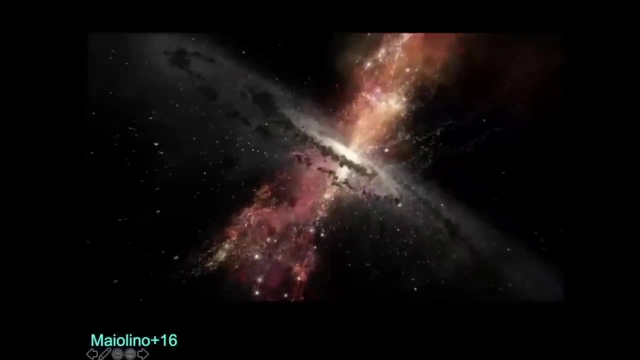 press release of a paper we had in press release of a paper we had in nature, nature, nature, where we had predicted there would be where we had predicted there would be where we had predicted there would be star formation in these outflows. star formation in these outflows. 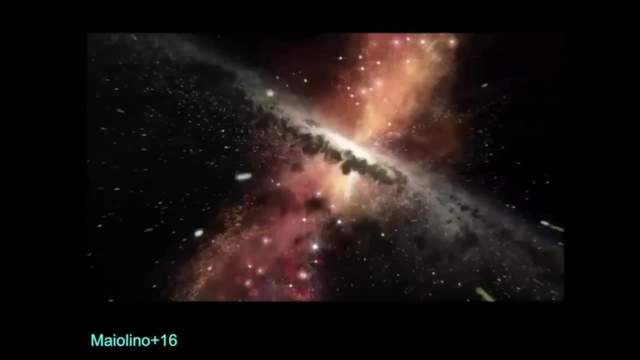 star formation in these outflows, and indeed that's what we saw. so this is, you've got to get the picture. so this is, you've got to get the picture. so this is- you've got to get the picture- that the enormous amounts of that, the enormous amounts of 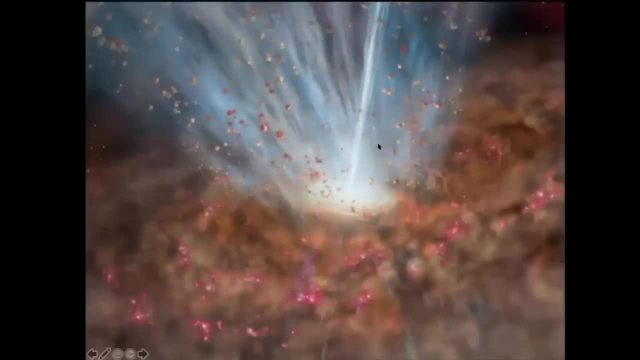 that the enormous amounts of energy from the jets, energy from the jets, energy from the jets, jets like this and winds and radiation jets like this and winds and radiation jets like this and winds and radiation, pressure pushes and forces, pressure pushes and forces, pressure pushes and forces much of the rest of the gas and the. 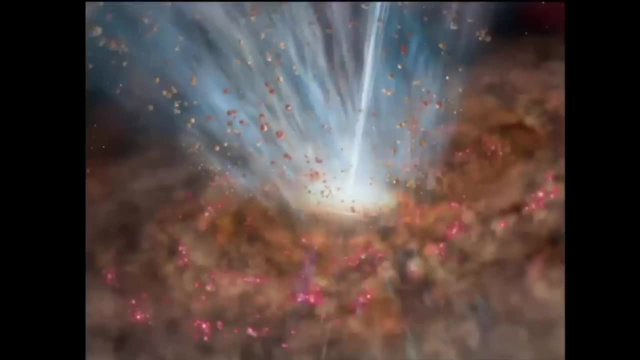 much of the rest of the gas and the much of the rest of the gas and the galaxy out and away. so we change the galaxy out and away. so we change the galaxy out and away. so we change the map: the potential for more stars to form. map- the potential for more stars to form. 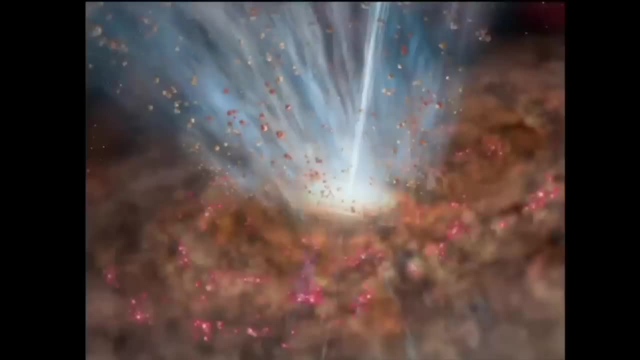 map the potential for more stars to form in the galaxy. it truncates the star in the galaxy. it truncates the star in the galaxy. it truncates the star, information and the galaxy when we get information and the galaxy when we get information and the galaxy when we get all this activity. 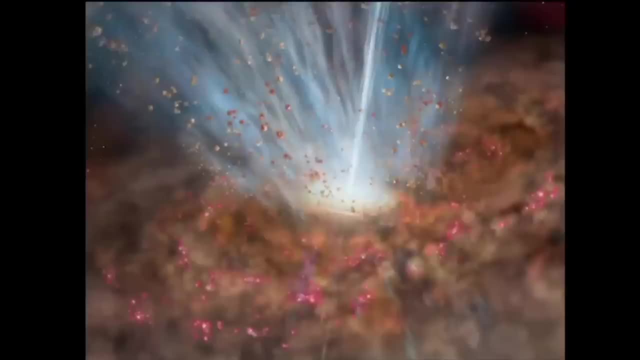 all this activity, all this activity, and also because we could maybe inform, and also because we could maybe inform, and also because we could maybe inform stars in the outflow at the same time, stars in the outflow at the same time, stars in the outflow at the same time, we can change the shape of the galaxy. so 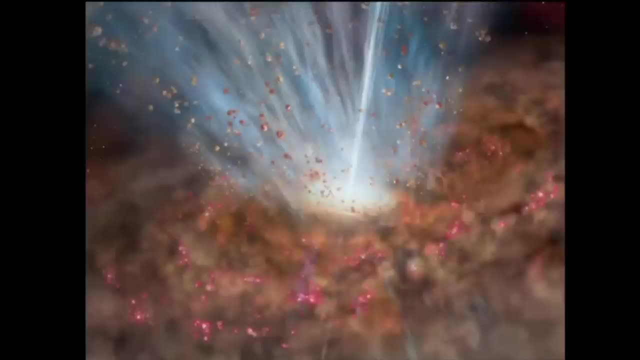 we can change the shape of the galaxy. so we can change the shape of the galaxy. so all of these things are quite profound. all of these things are quite profound. all of these things are quite profound in terms of how the whole thing will, in terms of how the whole thing will. 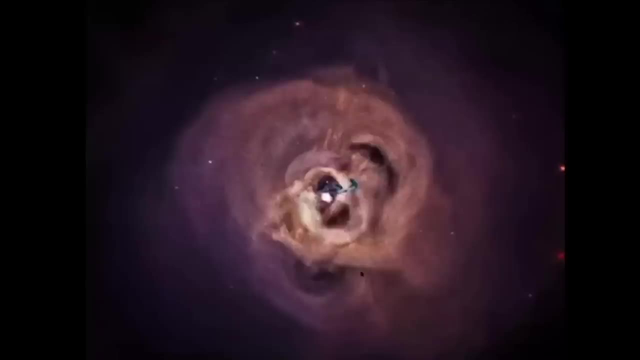 in terms of how the whole thing will, of the perseus cluster of galaxies. it's of the perseus cluster of galaxies. it's of the perseus cluster of galaxies. it's an image i had a lot to do with, and what an image i had a lot to do with and what 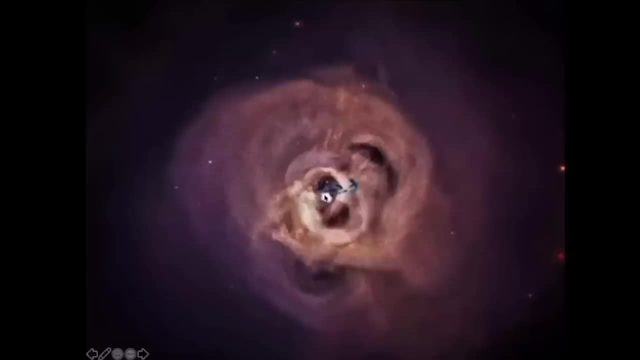 an image i had a lot to do with and what we see there is that nucleus, the active we see there is that nucleus, the active we see there is that nucleus, the active, nucleus of this object. is there nucleus of this object? is there nucleus of this object? is there? not going to talk about all the details? 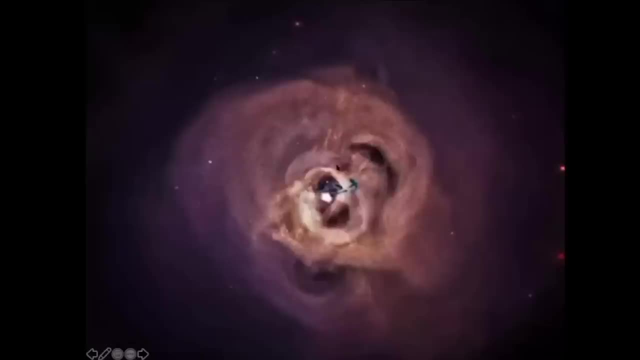 not going to talk about all the details, not going to talk about all the details, but much of this inner structure, but much of this inner structure, but much of this inner structure which is on a scale bigger than that of, which is on a scale bigger than that of 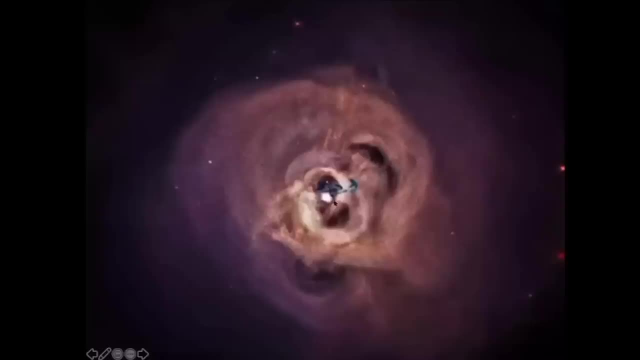 which is on a scale bigger than that of our galaxy, our galaxy. our galaxy has caused these holes in the emission, has caused these holes in the emission, has caused these holes in the emission and those holes and these are, and those holes, and these are and those holes and these are essentially bubbles. 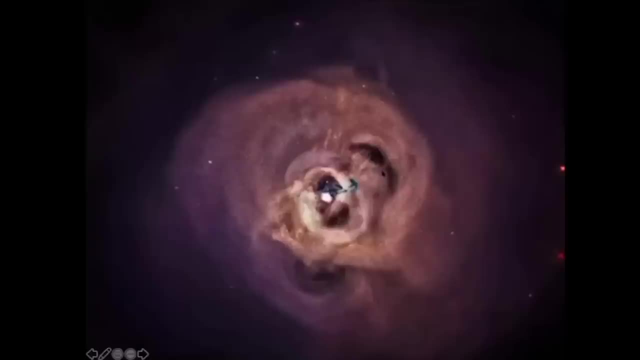 essentially bubbles, essentially bubbles: bubbles in the surrounding hot gas, bubbles in the surrounding hot gas, bubbles in the surrounding hot gas. and this bubble here is much bigger, and this bubble here is much bigger, and this bubble here is much bigger than the size of a whole of our galaxy. 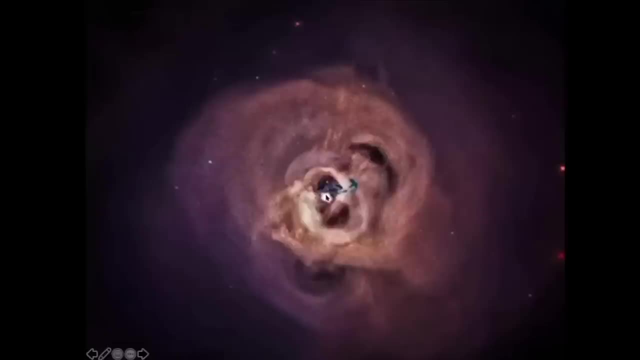 than the size of a whole of our galaxy, than the size of a whole of our galaxy. and that's all being produced by energy, and that's all being produced by energy, and that's all being produced by energy coming out of the active galaxy, the coming out of the active galaxy, the. 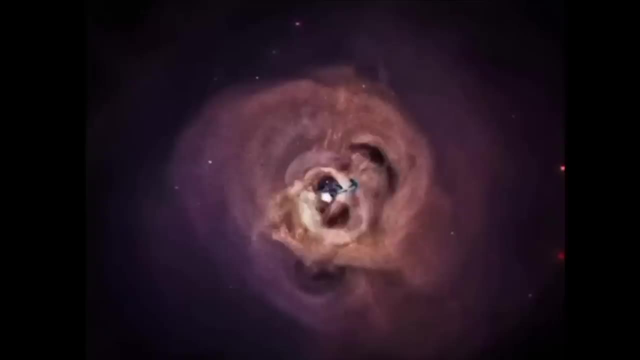 coming out of the active galaxy, the black hole of the center. black hole of the center, black hole of the center, if you compare the size of the event, if you compare the size of the event, if you compare the size of the event horizon of that black hole. 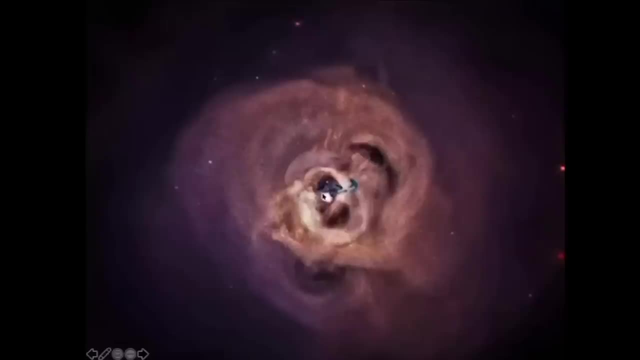 horizon of that black hole, horizon of that black hole, to the size of this region. we're looking to the size of this region. we're looking to the size of this region. we're looking, at, at, at. so i can't possibly draw the size of the. so i can't possibly draw the size of the. 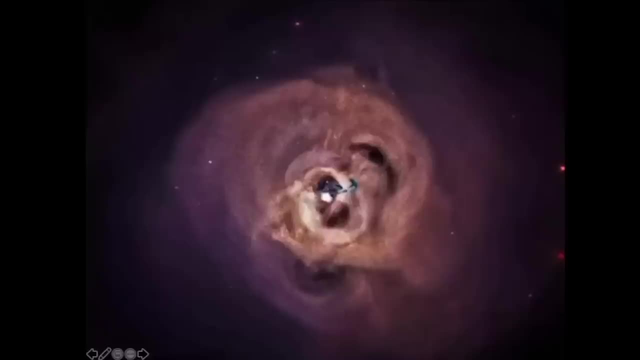 so i can't possibly draw the size of the black hole here. it's black hole. here it's black hole. here it's atom sized compared to this size, atom sized compared to this size. atom sized compared to this size. the ratio is about a billion. the ratio is about a billion. 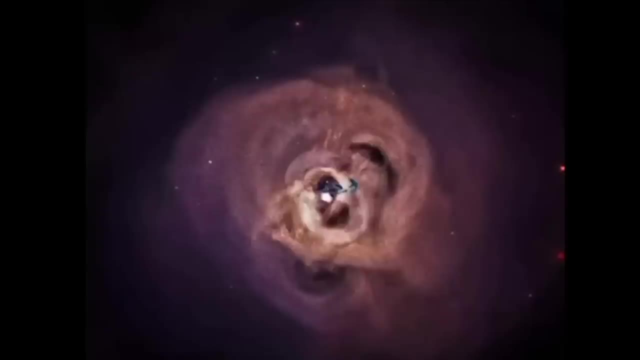 the ratio is about a billion. okay, and it's comparable the effect of okay and it's comparable. the effect of okay and it's comparable the effect of a black hole on its host galaxy, a black hole on its host galaxy, a black hole on its host galaxy, is rather like thinking of something, the 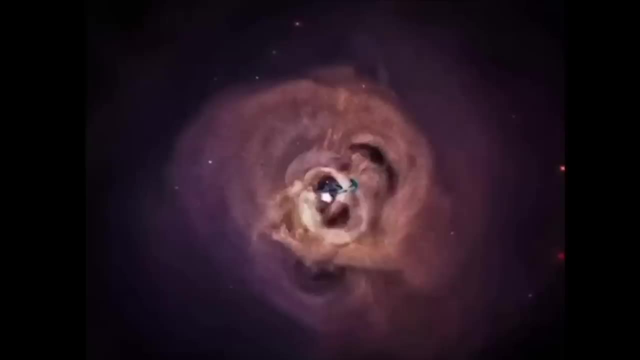 is rather like thinking of something. the is rather like thinking of something: the size of an orange, size of an orange, size of an orange, affecting the evolution of the earth, affecting the evolution of the earth, affecting the evolution of the earth. that's what these black holes are doing. 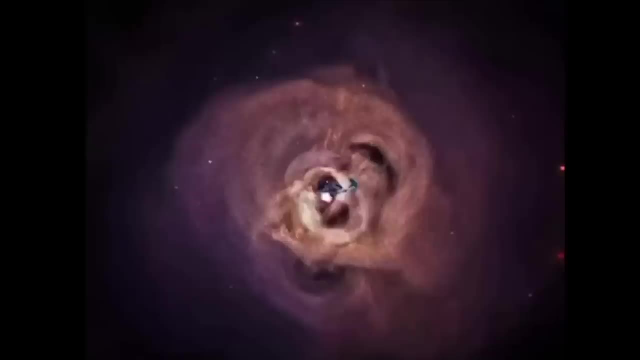 that's what these black holes are doing. that's what these black holes are doing. that super massive black holes, that super massive black holes, that super massive black holes are controlling the galaxy saint david, are controlling the galaxy saint david, are controlling the galaxy saint david. that's radio emission. i want to end just. 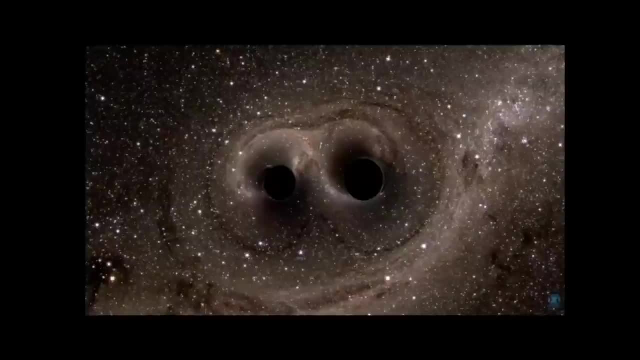 that's radio emission. i want to end. just that's radio emission. i want to end just by talking about merging black holes, by talking about merging black holes, by talking about merging black holes. and another nobel prize: this is just an. and another nobel prize: this is just an. 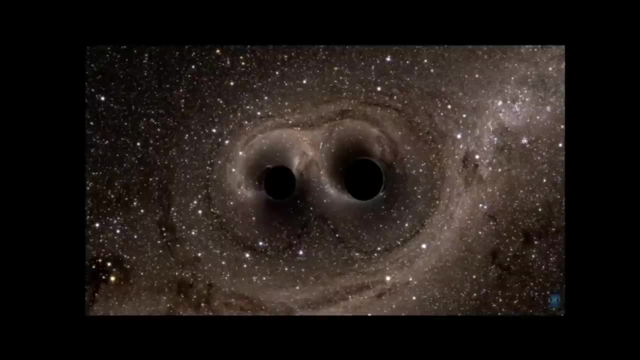 and another nobel prize. this is just an image of imagine that you've got two. image of imagine that you've got two. image of imagine that you've got two black holes in the sky, black holes in the sky, black holes in the sky and gravitational light bending has. 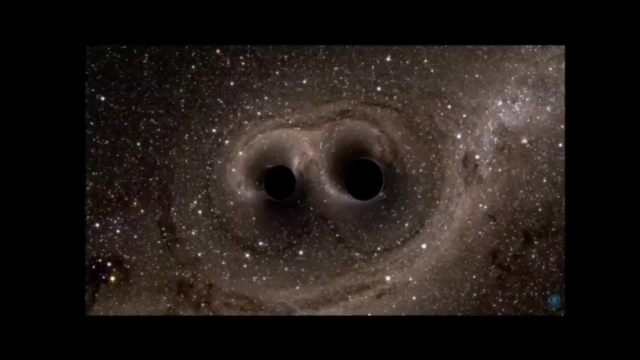 and gravitational light bending has, and gravitational light bending has- distorted the background star fields, distorted the background star fields, distorted the background star fields. that's how you can tell the black holes. that's how you can tell the black holes. that's how you can tell the black holes are there. 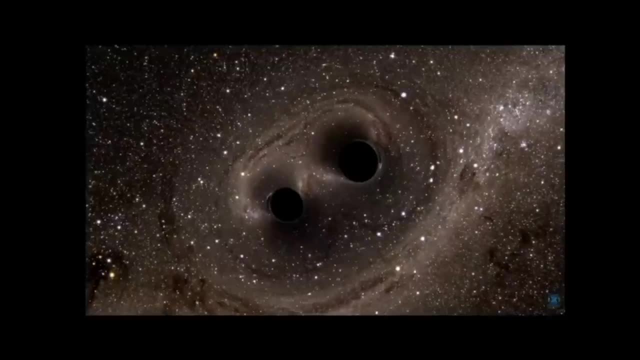 are there, are there, and these black holes are orbiting each, and these black holes are orbiting each, and these black holes are orbiting each other. other other and massive black holes are going to, and massive black holes are going to, and massive black holes are going to orbit each other, and in about five 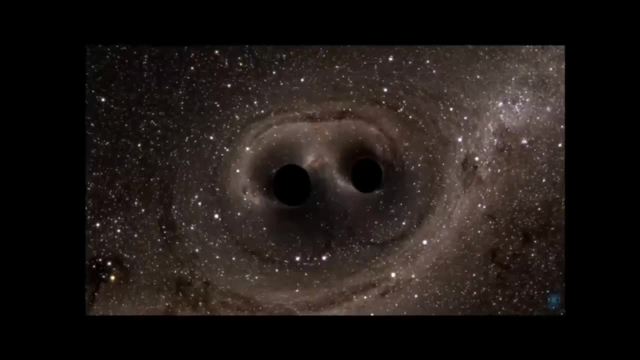 orbit each other, and in about five orbit each other, and in about five billion years, billion years, billion years. our, the black hole at the center of our, our, the black hole at the center of our, our, the black hole at the center of our galaxy, is going to merge with that of 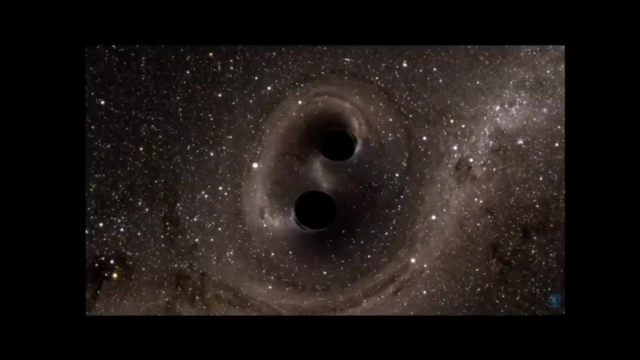 galaxy is going to merge with that of galaxy, is going to merge with that of the andromeda galaxy, because that the andromeda galaxy, because that the andromeda galaxy, because that has actually is coming towards us but has actually is coming towards us, but. 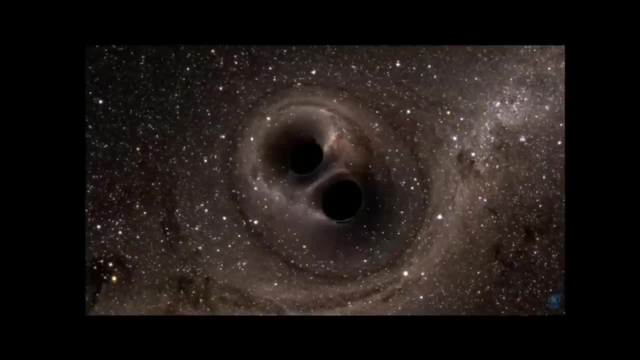 has actually is coming towards us, but this is really made. this is really made. this is really made for stellar mass black holes, where it's for stellar mass black holes, where it's for stellar mass black holes, where it's a black hole of, say, a 30 solar masses. 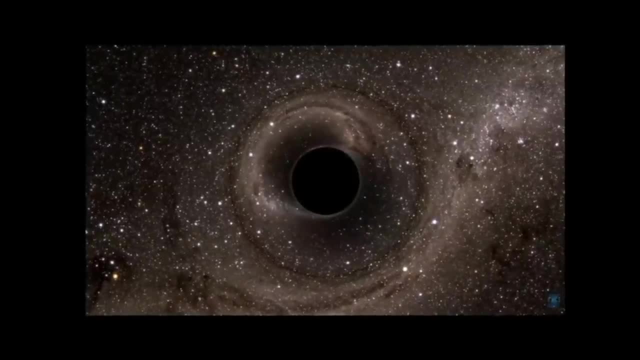 a black hole of, say, a 30 solar masses. a black hole of, say, a 30 solar masses and 50 solar masses merging together and 50 solar masses merging together and 50 solar masses merging together and something like that's a computer and something like that's a computer. 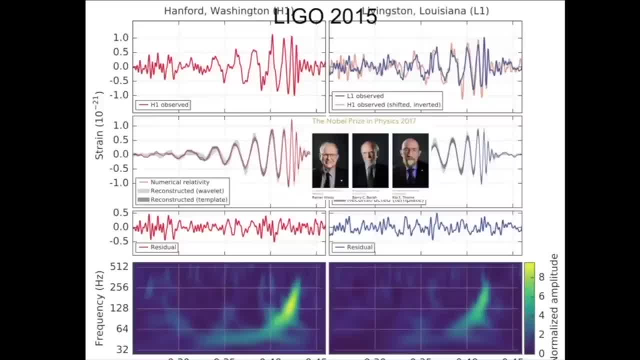 and something like. that's a computer simulation, simulation, simulation. but this was actually observed with the. but this was actually observed with the. but this was actually observed with the ligo instrument, ligo instrument, ligo instrument. well, there are two such instruments one. well, there are two such instruments one. 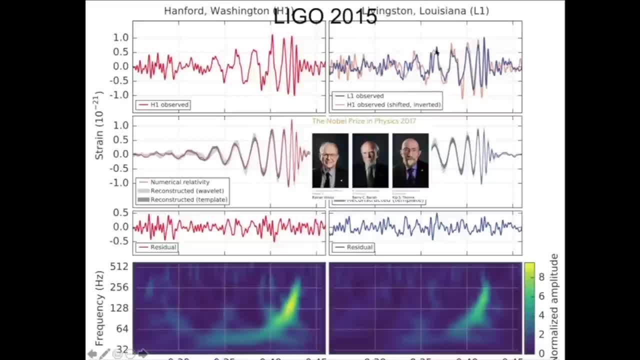 well, there are two such instruments, one in hanford washington and one in in hanford washington and one in in hanford washington and one in livingston louisiana, livingston, louisiana, livingston, louisiana. and they showed that in when they switch and they showed that in when they switch. 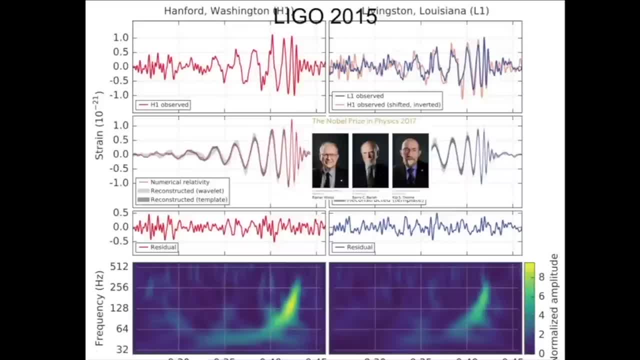 and they showed that in when they switch this instrument on in september 2015, this instrument on in september 2015, this instrument on in september 2015. they saw this chirp of, they saw this chirp of, they saw this chirp of x, the, the, the, it's the strain. now they 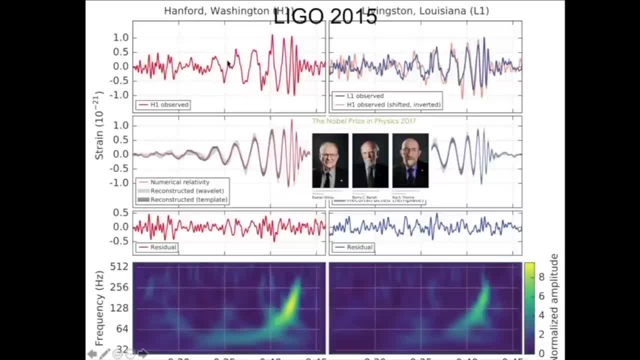 x the the it's the strain, now they. x the the it's the strain, now they, they. they were interferometers, only this, they. they were interferometers, only this, they. they were interferometers only this time. interferometers like the ones you time. interferometers like the ones you. 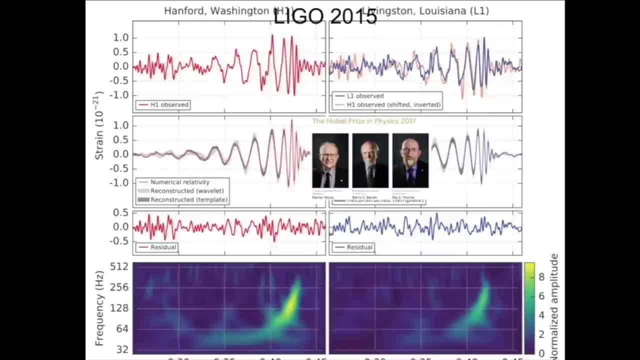 time interferometers like the ones you have in a physics lab, where you're have in a physics lab, where you're have in a physics lab, where you're measuring the length of something and measuring the length of something and measuring the length of something, and it's two arms. 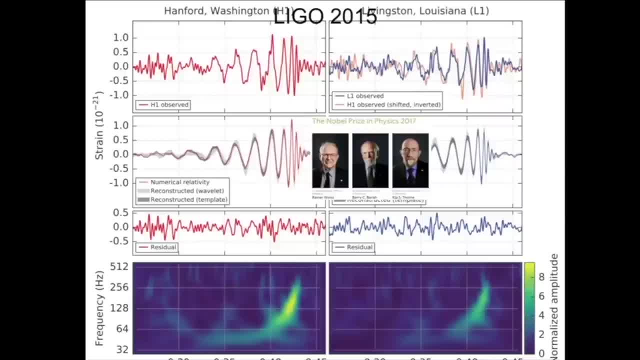 it's two arms. it's two arms perpendicular to each other. and what perpendicular to each other and what perpendicular to each other. and what they arms are being. they arms are being. they arms are being. their length is being oscillated. their length is being oscillated. their length is being oscillated by a gravitational wave passing. 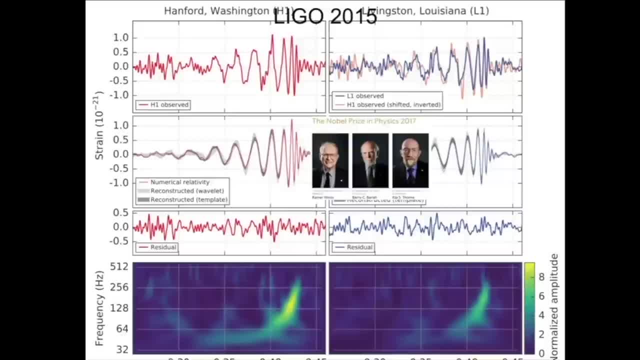 by a gravitational wave passing by a gravitational wave passing through these instruments, through these instruments, through these instruments, and the gravitational wave is coming and the gravitational wave is coming. and the gravitational wave is coming from a very distant galaxy, from a very distant galaxy, from a very distant galaxy. and you can see that the frequency 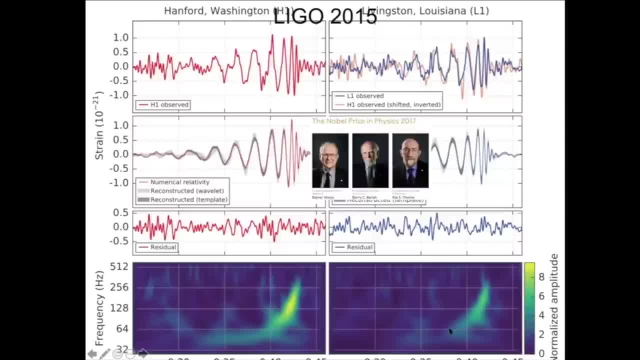 and you can see that the frequency, and you can see that the frequency, the strain is going up and the frequency, the strain is going up and the frequency, the strain is going up and the frequency is going up at the end, and all of this is going up at the end and all of this. 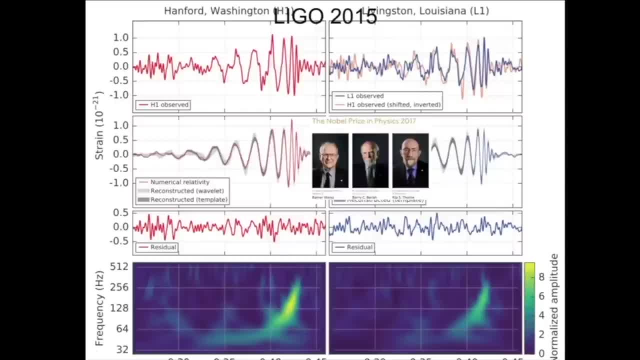 is going up at the end and all of this fits, fits, fits. what is expected for a gravitational wave, what is expected for a gravitational wave, what is expected for a gravitational wave passing through the instrument? passing through the instrument, passing through the instrument? gravitational waves were first predicted. 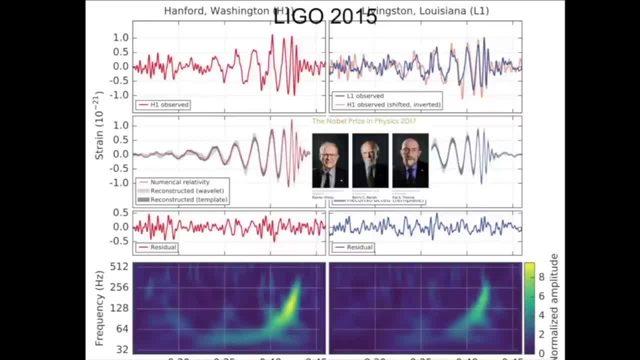 gravitational waves were first predicted. gravitational waves were first predicted by einstein in 2016, by einstein in 2016, by einstein in 2016, and they were discovered here in uh 2015 and they were discovered here in uh 2015. 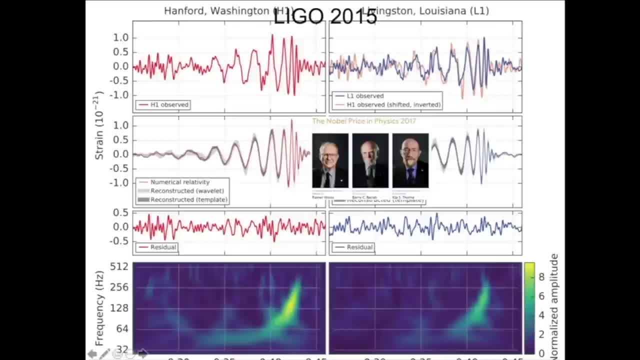 and they were discovered here in uh 2015 and uh weiss um and uh and uh weiss um and uh burr and um and uh burr and um. kip thorne got the nobel prize in 2017. kip thorne got the nobel prize in 2017. 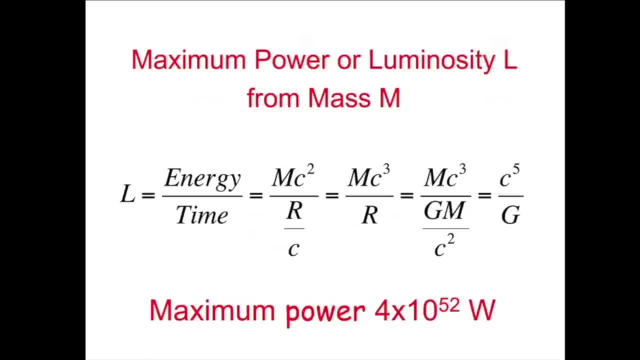 kip thorne got the nobel prize in 2017 for discovering it, for discovering it, for discovering it. i'm just gonna. i've got a couple of. i'm just gonna. i've got a couple of. i'm just gonna. i've got a couple of slides. i just want to finish with. 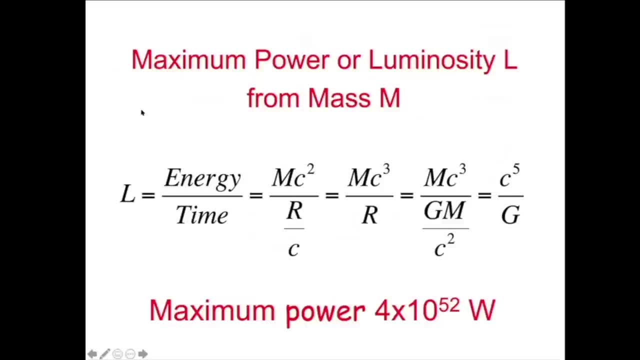 slides. i just want to finish with slides. i just want to finish with and this has got equations on. i know, and this has got equations on. i know, and this has got equations on. i know you're going to say oh, you're going to say oh, you're going to say oh, equations, yes. well, i hope some of you. 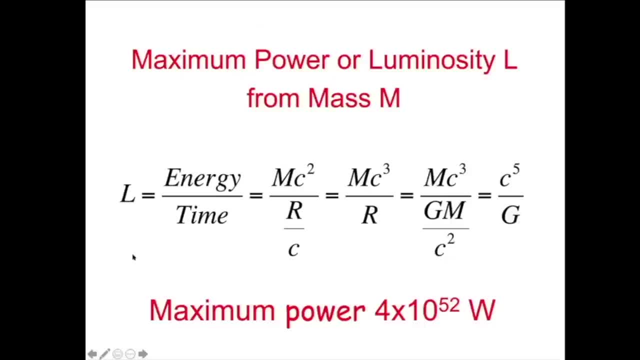 equations- yes, well, i hope some of you equations- yes, well, i hope some of you like equations. you can do this like equations. you can do this like equations. you can do this yourself on the back of an envelope, i yourself on the back of an envelope, i yourself on the back of an envelope. i want to just ask what is the maximum? 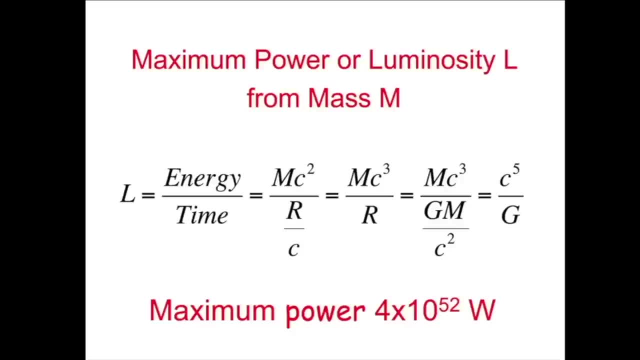 want to just ask what is the maximum, want to just ask what is the maximum power? power, power or luminosity you can get from mass m, or luminosity you can get from mass m, or luminosity you can get from mass m. now, power is energy and i recall it. 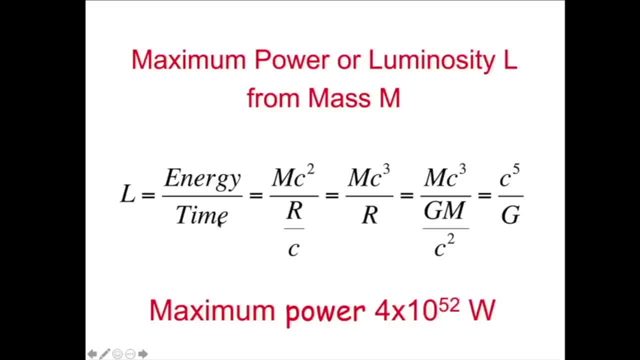 now, power is energy and i recall it. now. power is energy and i recall it: luminosity, luminosity, luminosity, and that is energy divided by time i, and that is energy divided by time i, and that is energy divided by time. i want to get maximum, want to get maximum. 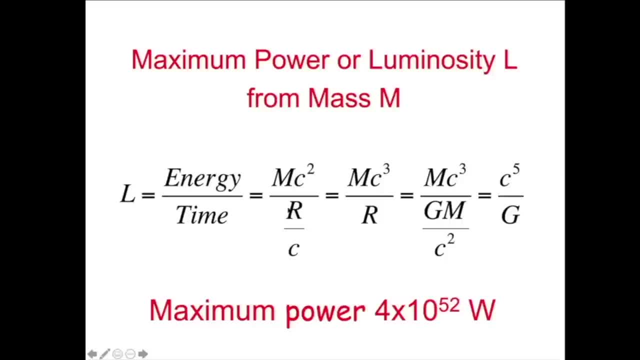 want to get maximum side of it to know about the other, the side of it to know about the other, the side of it to know about the other. the shortest time is going to be r over c. shortest time is going to be r over c. shortest time is going to be r over c. so i divide them and i get mc jupiter. 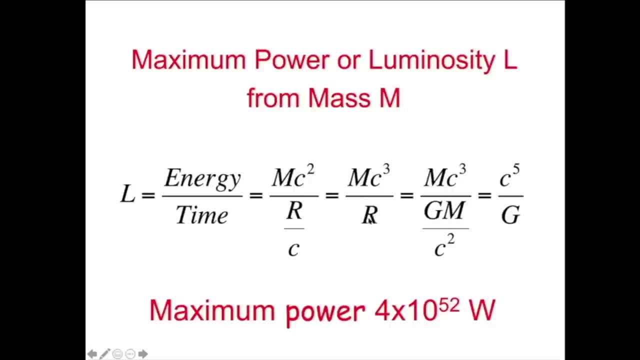 so i divide them and i get mc jupiter. so i divide them and i get mc jupiter over r, over r, over r. so i've got to make it as small as so. i've got to make it as small as so. i've got to make it as small as possible to make the time. 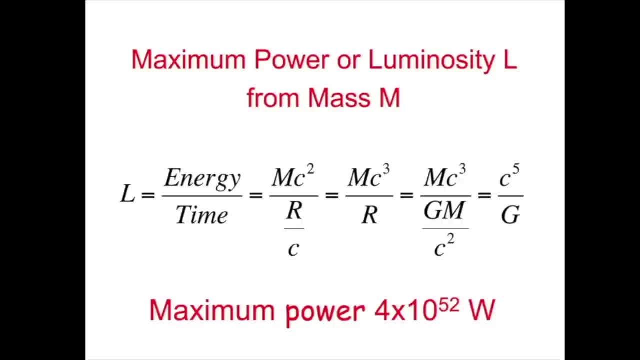 possible to make the time possible, to make the time as short as possible. i'm going to release as short as possible. i'm going to release as short as possible. i'm going to release the energy, the energy, the energy. how small can i make it? i can make it the. 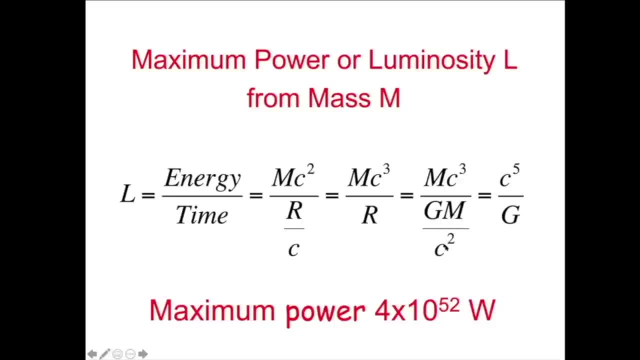 how small can i make it? i can make it the. how small can i make it? i can make it the size of a black hole. size of a black hole. size of a black hole: gm over c squared, that's for a spinning. gm over c squared, that's for a spinning. 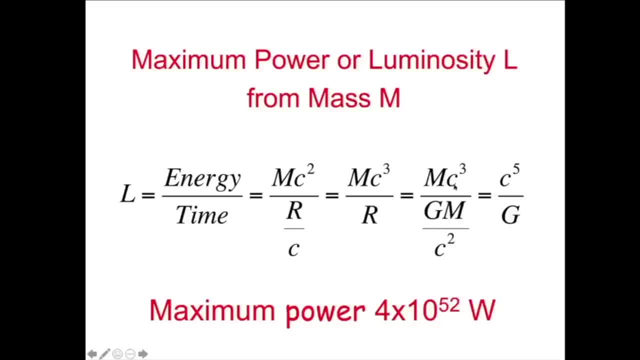 gm over c squared, that's for a spinning black hole. so they're going to make the black hole. so they're going to make the black hole. so they're going to make the very smallest black hole, very smallest black hole, very smallest black hole. when i do that, the m cancels and i'm. 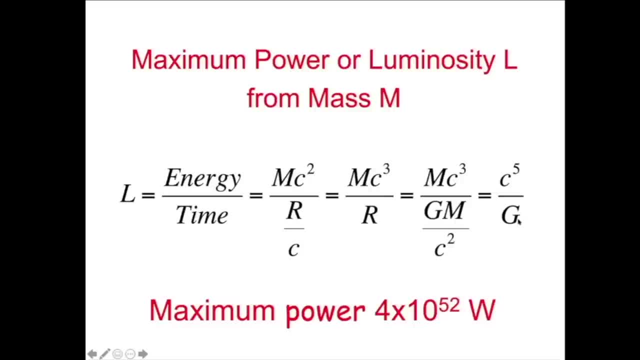 when i do that, the m cancels and i'm when i do that the m cancels and i'm left with c to the fifth over g, left with c to the fifth over g, left with c to the fifth over g. i'm sure all of you know that c is a. 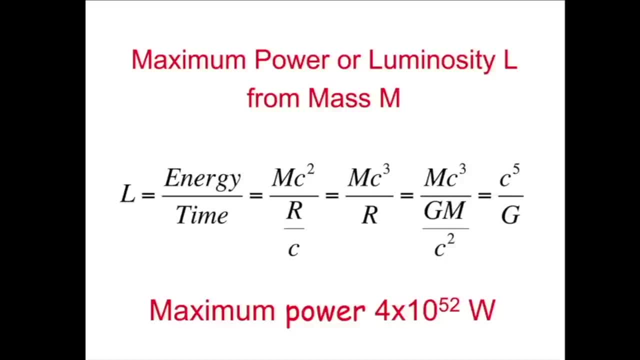 i'm sure all of you know that c is a. i'm sure all of you know that c is a very large number, very large number, very large number. that's the speed of light to the fifth. that's the speed of light to the fifth. that's the speed of light to the fifth. power is a very, very large number. 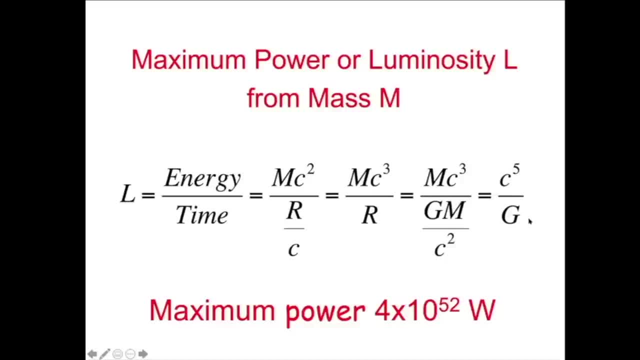 power is a very, very large number. power is a very, very large number and g is a very small number. so c to and g is a very small number. so c to and g is a very small number. so c to the fifth over g, the fifth over g. 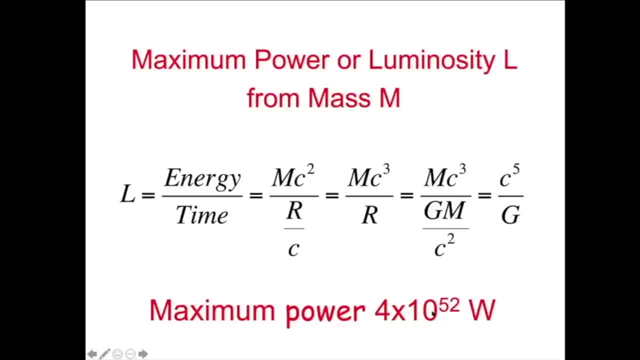 the fifth over g is actually a very large number. the is actually a very large number. the is actually a very large number. the maximum power is 4 times 10 to the 52. maximum power is 4 times 10 to the 52. maximum power is 4 times 10 to the 52 watts. 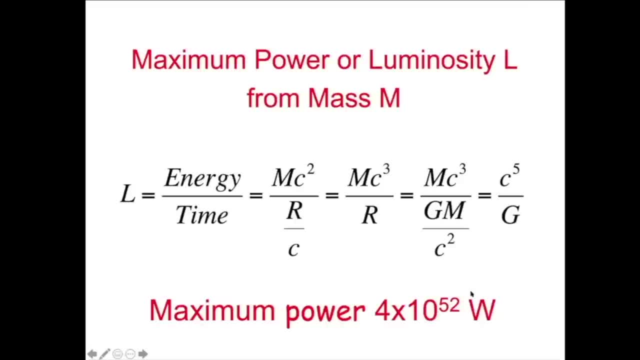 watts, watts. do you notice that mast cancelled out? do you notice that mast cancelled out? do you notice that mast cancelled out of this, of this, of this? that's because the power only lasts for that's because the power only lasts for that's because the power only lasts for a time which is r over c. 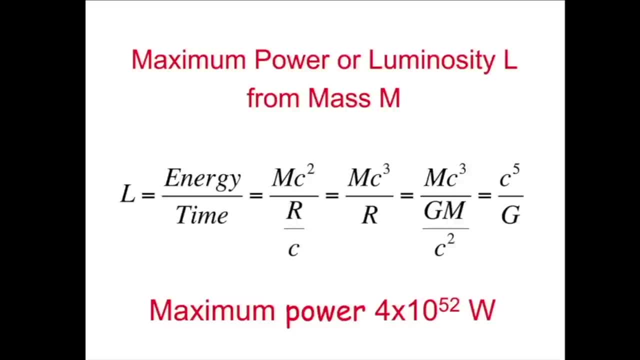 a time which is r over c, a time which is r over c? okay, so which for a low mass object? okay, so which for a low mass object? okay. so which for a low mass object can be very, very short, can be very, very short, can be very, very short. but the maximum power is 10 to the 26. 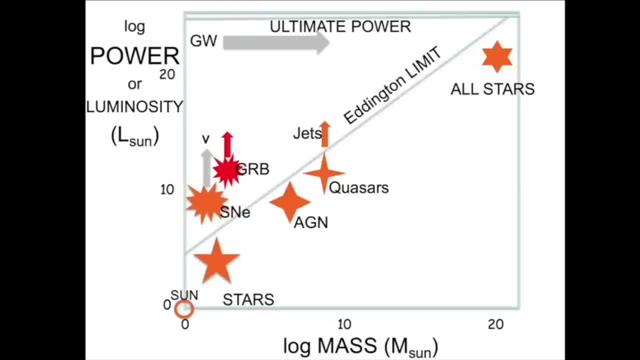 but the maximum power is 10 to the 26. but the maximum power is 10 to the 26 solar luminosities, 10 to the 26 solar solar luminosities, 10 to the 26 solar solar luminosities, 10 to the 26 solar luminosities. 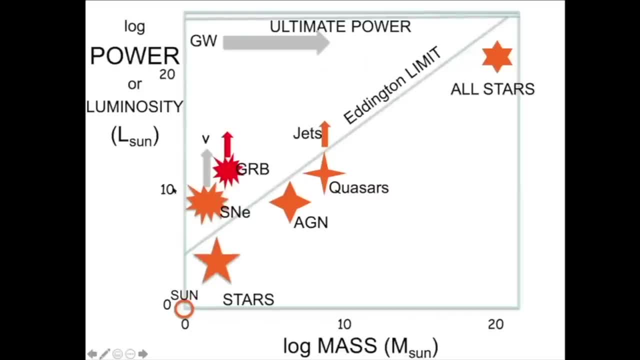 luminosities, luminosities, so we can put it on this diagram which, so we can put it on this diagram, which, so we can put it on this diagram which is power or luminosity versus mass, is power or luminosity versus mass, is power or luminosity versus mass, and is the mass of the universe, or at 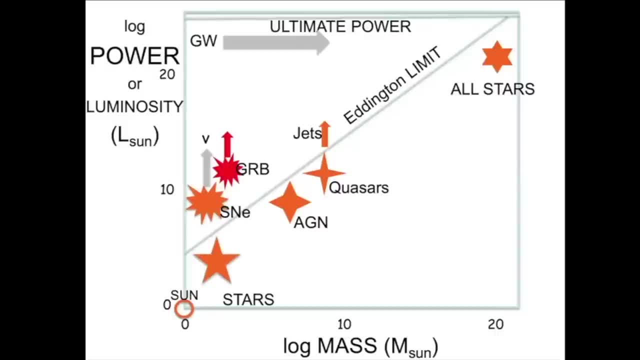 and is the mass of the universe, or at and is the mass of the universe, or at least the variable content of the least, the variable content of the least, the variable content of the universe, universe, universe, is, is here and that's, is is here and that's. 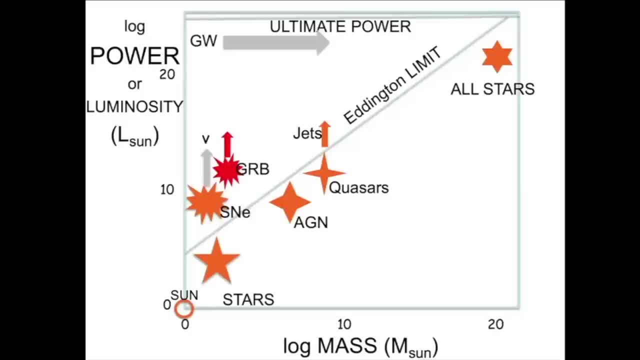 is is here and that's. there's a 100 million, 10 to 11 stars. there's a 100 million, 10 to 11 stars. there's a 100 million, 10 to 11 stars in the galaxies- 10 to 11 galaxies in the. 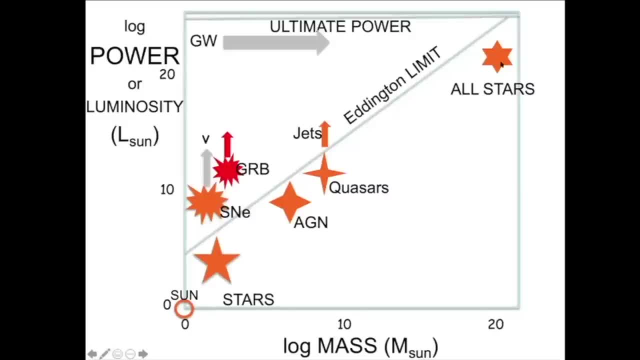 in the galaxies: 10 to 11 galaxies in the. in the galaxies: 10 to 11 galaxies in the universe. that's all universe. that's all universe, that's all. all the stars in the universe. 10 to the. the stars in the universe. 10 to the. 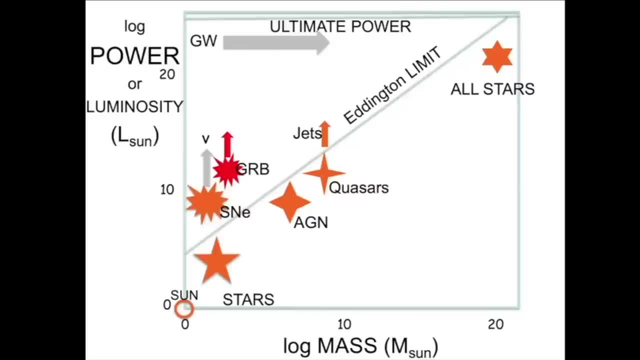 the stars in the universe, 10 to the 22, 22, 22 solar luminosity. and it turns out this solar luminosity, and it turns out this solar luminosity and it turns out this gravitational wave, gravitational wave. gravitational wave was more luminous than that, so just 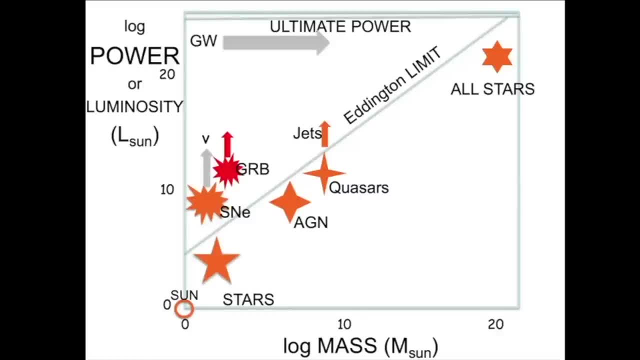 was more luminous than that. so just was more luminous than that. so just briefly, briefly, briefly, the production of that flash of gamma, of the production of that flash of gamma, of the production of that flash of gamma of gravitational radiation, gravitational radiation, gravitational radiation which is coming from the other side of 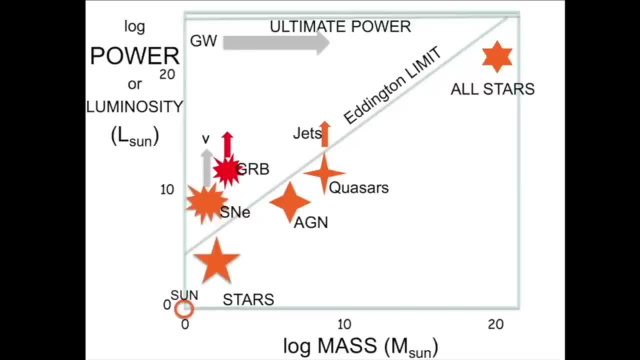 which is coming from the other side of, which is coming from the other side of the universe, the universe, the universe, equaled the radiation out of all the equaled the radiation out of all the equaled the radiation out of all the stars, stars, stars in the universe, and this the rest of. 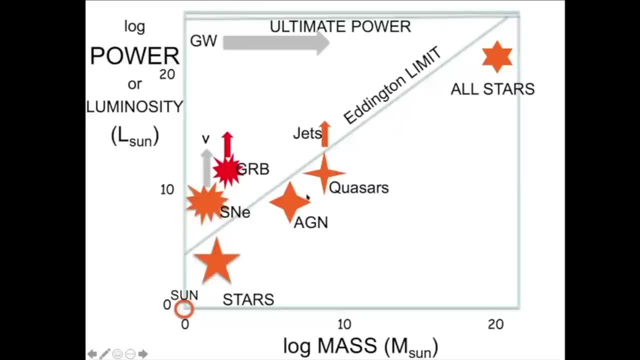 in the universe and this the rest of in the universe and this the rest of this plot, this plot. this plot you can look at some other time. it's you can look at some other time. it's you can look at some other time. it's got quasars, agn and so forth on. 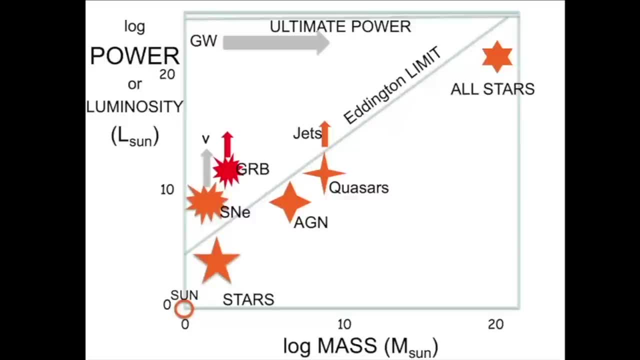 got quasars agn and so forth on. got quasars agn and so forth on. now one can think about power in the now. one can think about power in the now. one can think about power in the universe, but universe, but universe. but i think it interesting to realize that 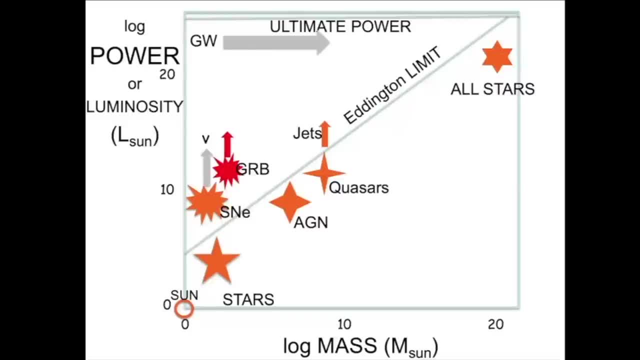 i think it interesting to realize that. i think it interesting to realize that black holes can produce black holes can produce black holes can produce the highest levels of power in the, the highest levels of power in the, the highest levels of power in the universe, universe, universe. so there's much more we could say about. 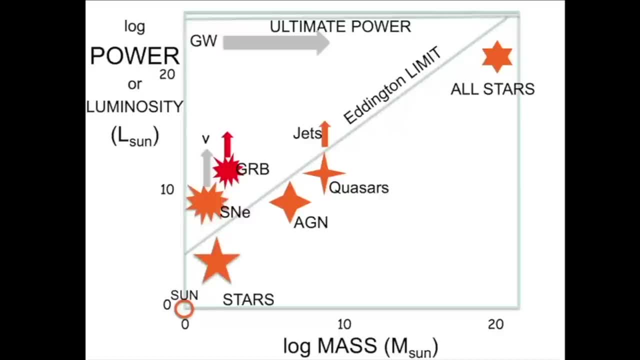 so there's much more we could say about. so there's much more we could say about black holes, but they're certainly here, black holes, but they're certainly here, black holes, but they're certainly here to stay, to stay, to stay, and astro visible black holes are. 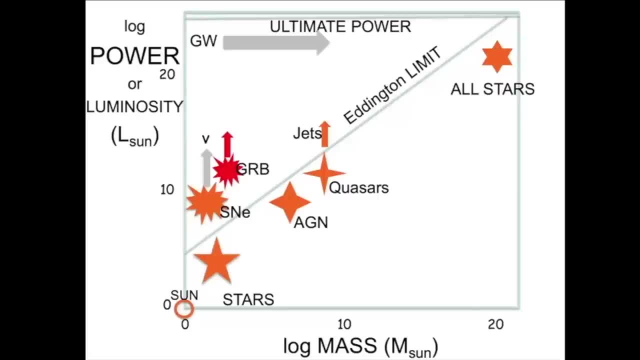 and astro visible black holes are, and astro visible black holes are playing a very large part, playing a very large part, playing a very large part in shaping galaxies and telling us, and in shaping galaxies and telling us, and in shaping galaxies and telling us, and affecting, affecting, affecting, how, uh, they act and evolve. 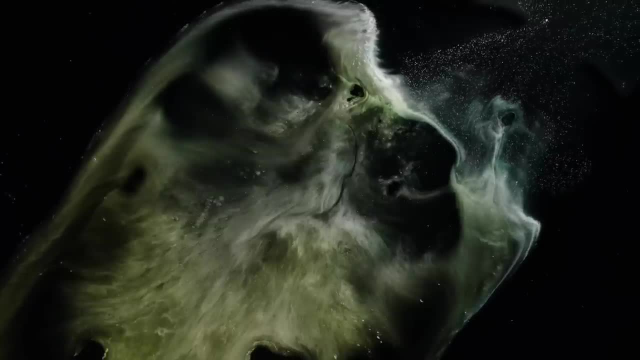 how uh they act and evolve. how uh they act and evolve. i'll stop there, thank you. i'll stop there. thank you, i'll stop there. thank you. uh, you mentioned the angle of image. uh, you mentioned the angle of image. uh, you mentioned the angle of image captured by eht. 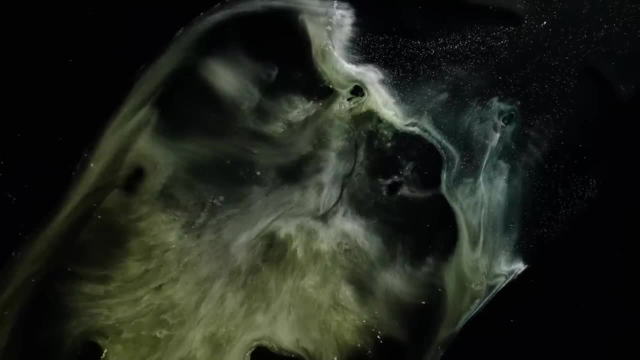 captured by eht. captured by eht of m87 black hole. so is it solid angle of m87 black hole? so is it solid angle of m87 black hole? so is it solid angle? no, it's, it's just well the the. no, it's, it's just well the the. 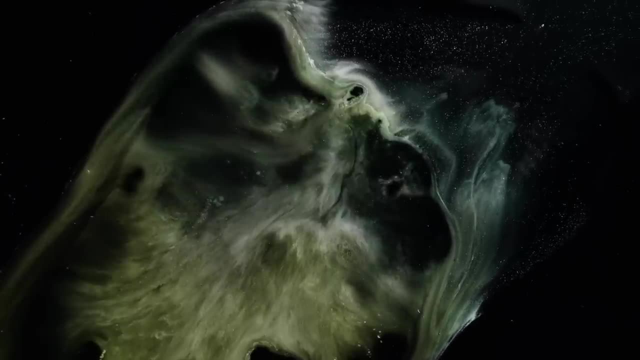 no, it's, it's just well. the the 50 micro up seconds is is purely you. 50 micro up seconds is is purely you. 50 micro up seconds is is purely you, know at a regular angle, know at a regular angle, know at a regular angle, and that is the radius of this ring. 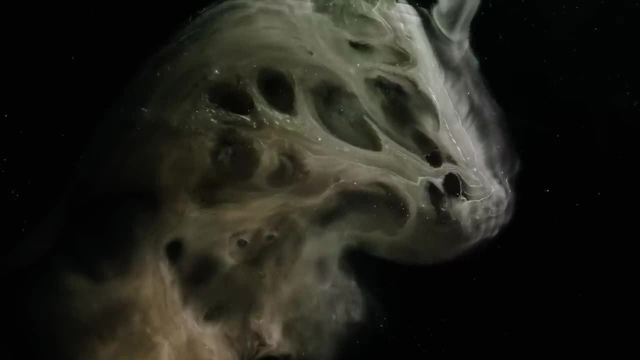 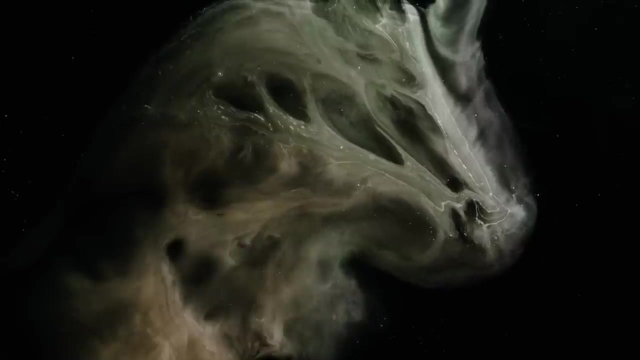 and that is the radius of this ring, and that is the radius of this ring that you can see. so the next one is uh. so the next one is uh. so the next one is uh. why time slows around massive objects. why time slows around massive objects. why time slows around massive objects at high velocities and stops at even. 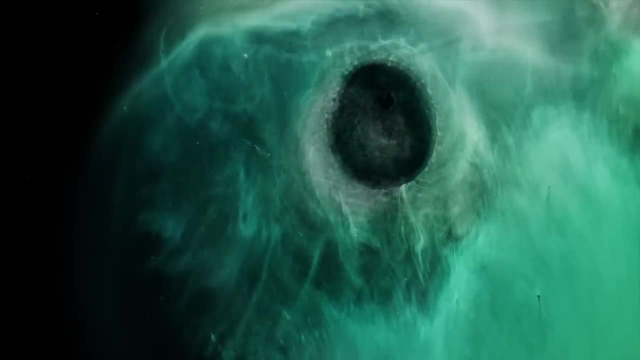 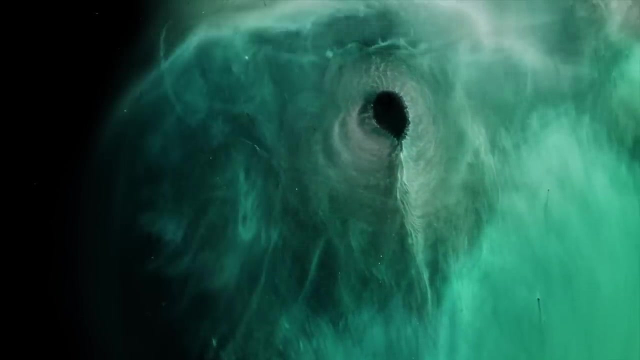 at high velocities and stops at even at high velocities and stops at even horizon of a black hole. well, it turns out that um time. well, it turns out that um time. well, it turns out that um time. as you know, if you know anything about, as you know, if you know anything about, 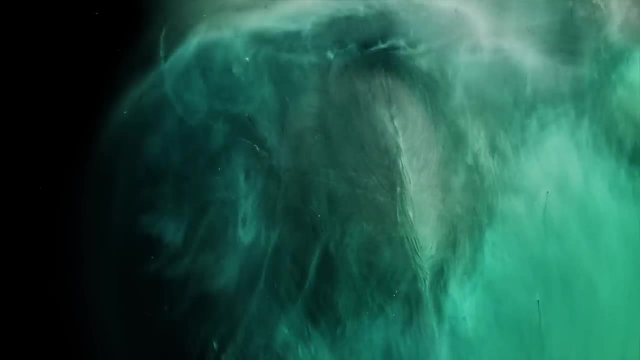 as you know, if you know anything about relativity, special relativity, if you relativity, special relativity, if you relativity special relativity, if you move, move, move, moving clocks run slower and things like moving clocks run slower and things like moving clocks run slower and things like this. 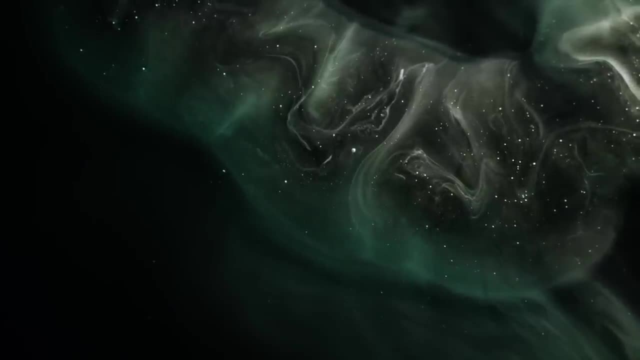 this, this and essentially, uh, what has happened, and essentially, uh, what has happened and essentially, uh, what has happened is the effect of the black hole is to, is the effect of the black hole is to is the effect of the black hole is to completely wrap, completely wrap. 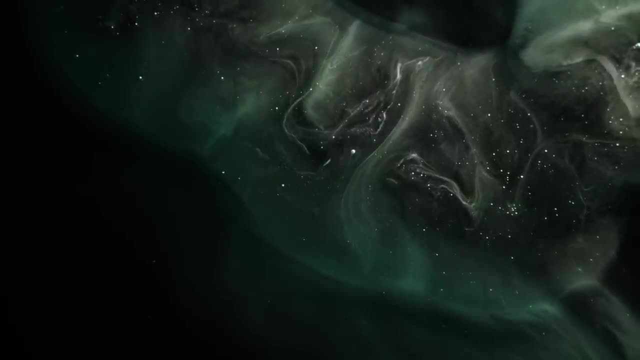 completely wrap space-time up, space-time up, space-time up. that's the best way i can put it to cloak. that's the best way i can put it to cloak, that's the best way i can put it to cloak: the black hole, the black hole, the black hole with space-time which is wrapped up into. 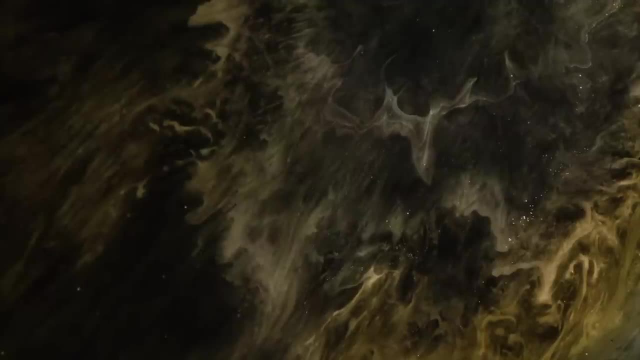 with space-time which is wrapped up into, with space-time which is wrapped up into this, this, this with this event horizon which, in the case with this event horizon, which, in the case with this event horizon, which, in the case of an object of one solar mass, is a 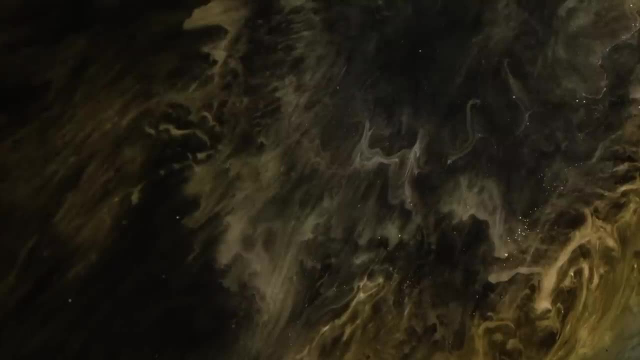 of an object of one solar mass is a of an object of one solar mass is a radius, radius, radius of uh three kilometers, so of uh three kilometers, so of uh three kilometers. so what this means is that, in order to do, what this means is that, in order to do, 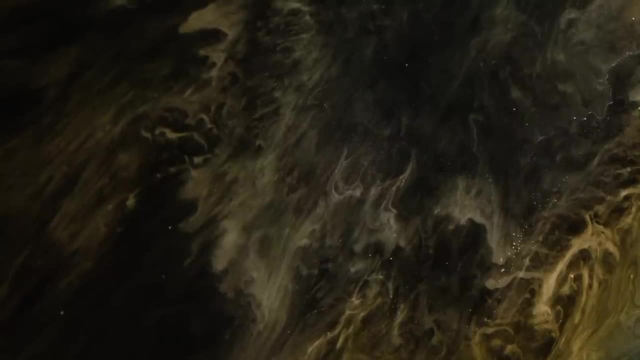 what this means is that, in order to do this, you need a lot of matter in a very this. you need a lot of matter in a very this. you need a lot of matter in a very small radius, small radius, small radius. and just to say, it is my hand and if i 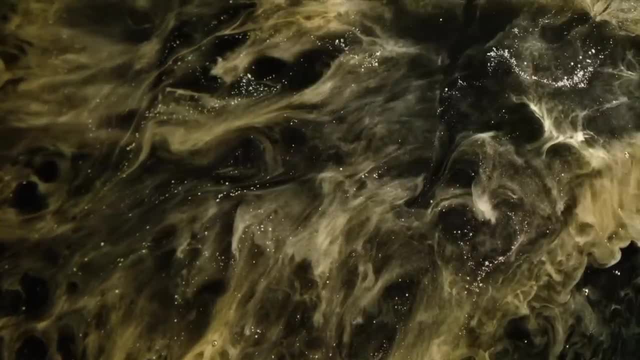 and just to say it is my hand. and if i, and just to say it is my hand, and if i was have a black hole, was have a black hole, was have a black hole that i could put in my, the cup of my, that i could put in my, the cup of my. 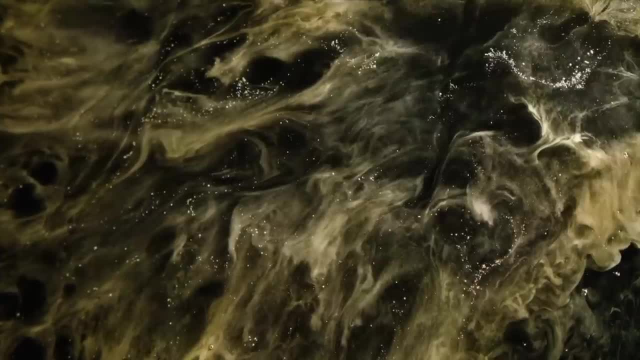 that i could put in my, the cup of my hand. it would have a mass hand. it would have a mass hand. it would have a mass that is about 10 times the mass of the. that is about 10 times the mass of the. that is about 10 times the mass of the earth. 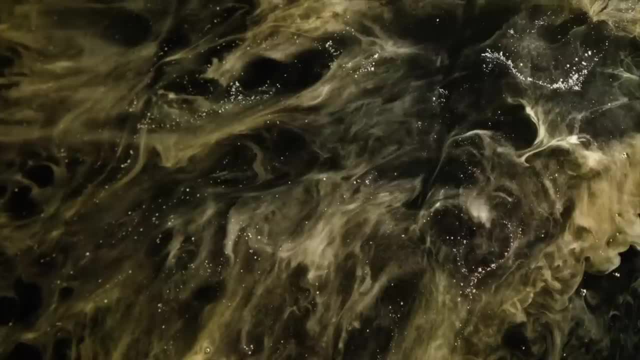 earth, earth. so we're talking about very compact. so we're talking about very compact, so we're talking about very compact things. but if we could do that, then things. but if we could do that, then things. but if we could do that, then basically, as you approach, 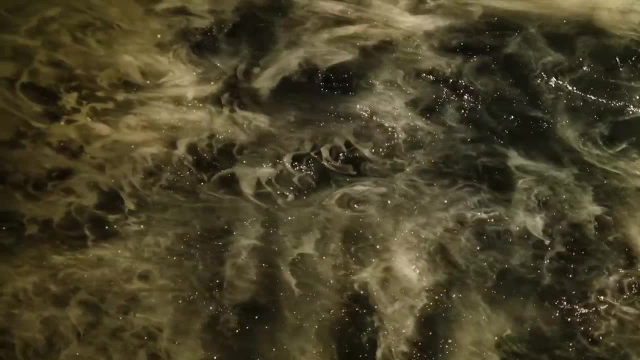 basically, as you approach, basically, as you approach the event horizon, um then as seen by an, the event horizon, um then as seen by an, the event horizon, um then as seen by an outside observer, outside observer, outside observer, then time appears to slow down, then time appears to slow down. 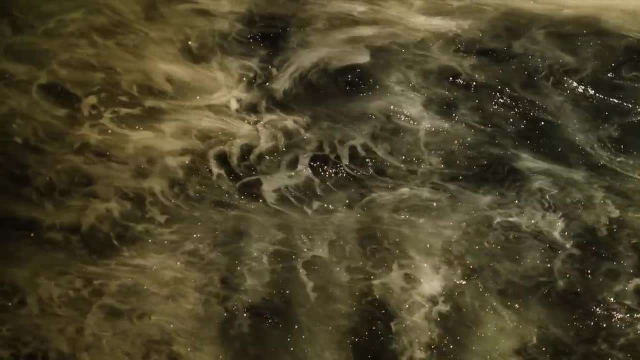 then time appears to slow down now, if i may just say now, if i may just say now, if i may just say that, if we go the other way in terms of that, if we go the other way in terms of that, if we go the other way in terms of mass, if we go up to these 10 billion, 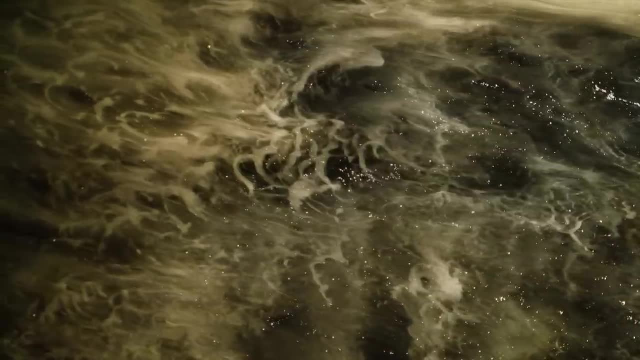 mass. if we go up to these 10 billion mass, if we go up to these 10 billion solar mass black holes, solar mass black holes, solar mass black holes, then the size of their event horizons, then the size of their event horizons, then the size of their event horizons is the size of our solar system. 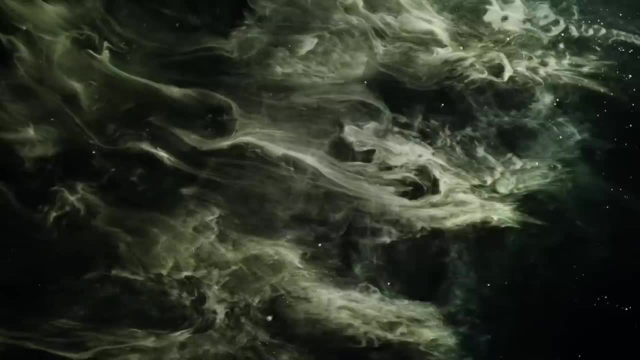 is the size of our solar system, is the size of our solar system and if you fell into one of those, and if you fell into one of those, and if you fell into one of those, it would take you a week to fall to. it would take you a week to fall to. 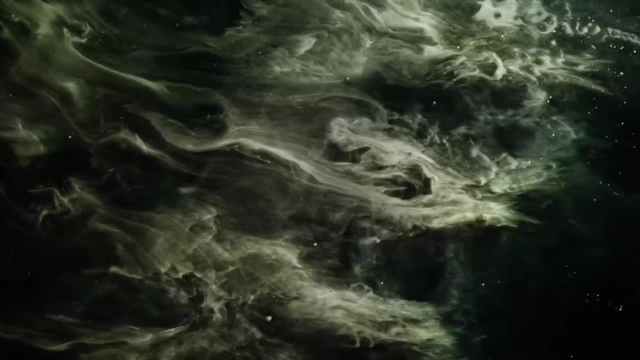 it would take you a week to fall to the center, the center, the center. and as you fall through the event, and as you fall through the event, and as you fall through the event- horizon, horizon, horizon- you would not notice anything. okay, you would not notice anything, okay. 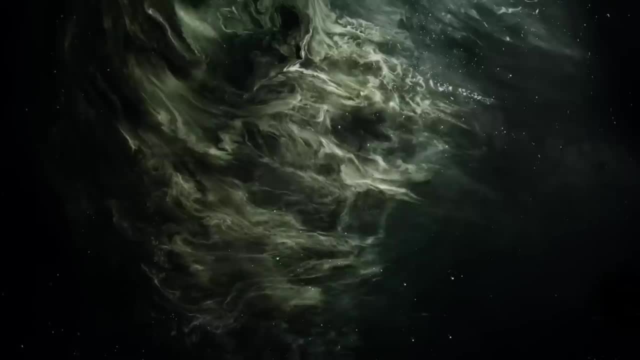 you would not notice anything. okay, and actually the mean density of such and actually the mean density of such, and actually the mean density of such black holes, black holes, black holes- is less than the density of air, however, is less than the density of air, however, is less than the density of air. however, as you fall closer and closer into the. 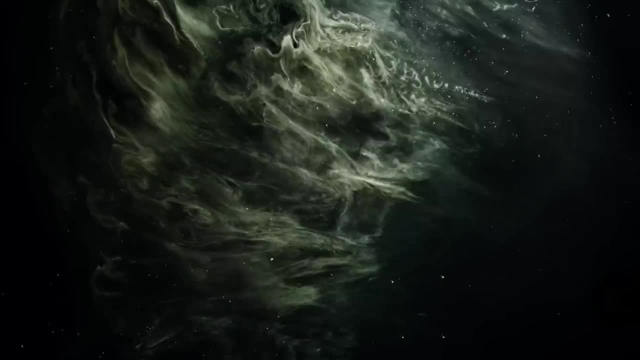 as you fall closer and closer into the, as you fall closer and closer into the center, center, center, then the rest of the universe would do, then the rest of the universe would do, then the rest of the universe would do its. it would appear to speed up to you. 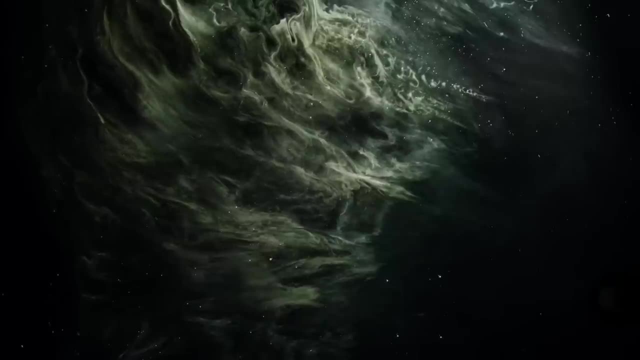 its it would appear to speed up to you, its it would appear to speed up to you, but you're also falling in, but you're also falling in, but you're also falling in, so that that stops you seeing the end, so that that stops you seeing the end. 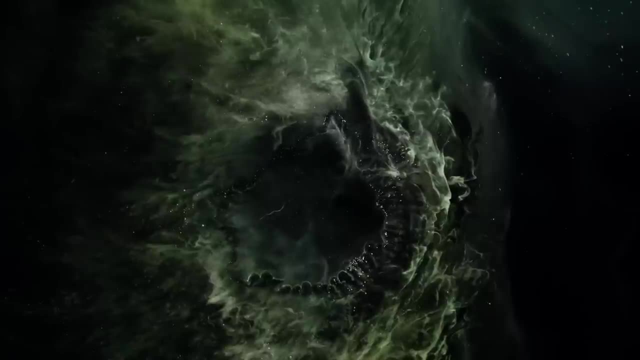 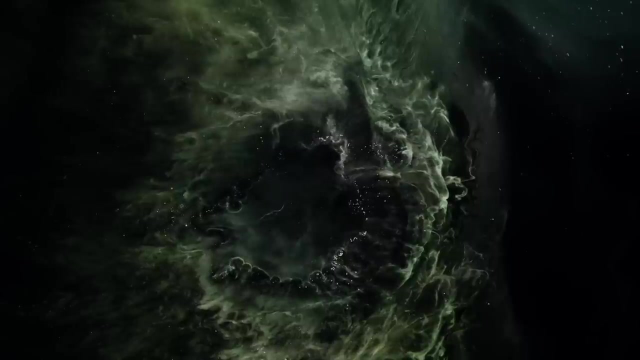 so that that stops you seeing the end of the universe, of the universe of the universe, but essentially you would fall in until, but essentially you would fall in until, but essentially you would fall in until you reach the spaghettification level. so the next one is: uh, if speed of light. 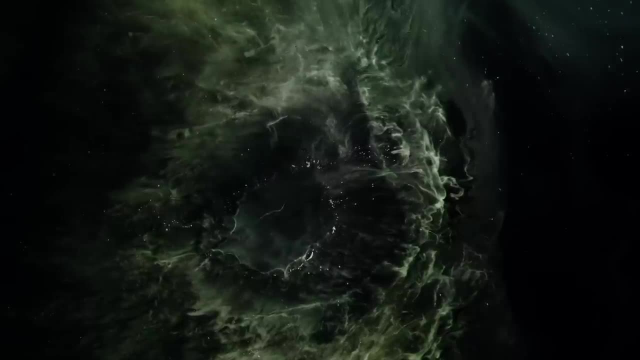 so the next one is: uh, if speed of light. so the next one is: uh, if speed of light slows down in different mediums, slows down in different mediums, slows down in different mediums, though gravitational waves slows down, though gravitational waves slows down, though gravitational waves slows down to in different mediums. 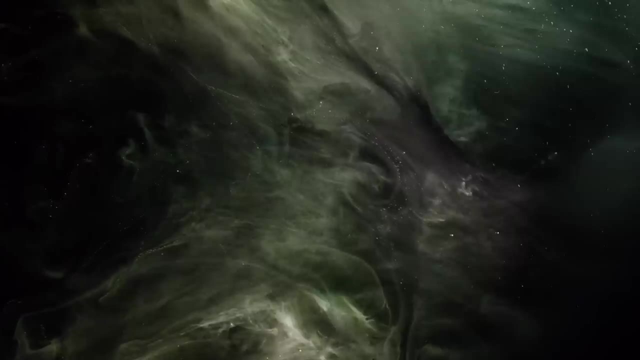 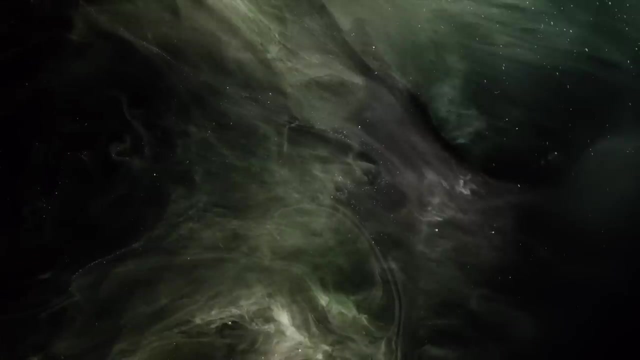 to in different mediums. to in different mediums. um a good question, i i guess so. um a good question, i i guess so. um a good question, i i guess so. but um, basically, um, but um, basically um, but, um, basically um. i mean gravitational waves that we see. 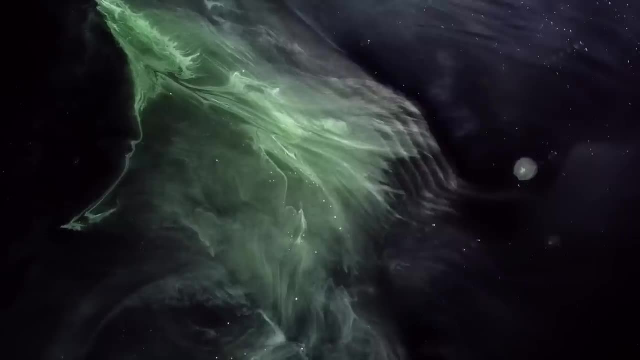 i mean gravitational waves that we see. i mean gravitational waves that we see um i i doubt you could to actually detect um i i doubt you could to actually detect um. i i doubt you could to actually detect anything like that, anything like that, anything like that. and then i'm more. 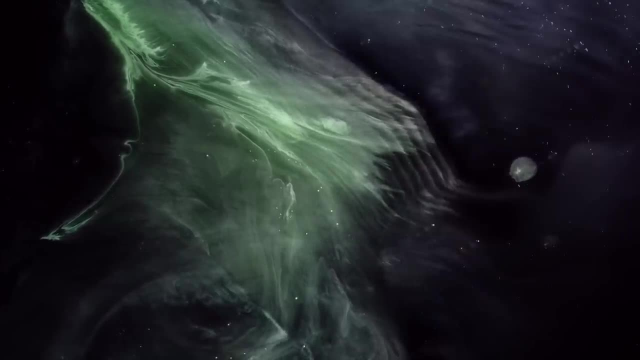 and then i'm more, and then i'm more of an observer than a theorist, of an observer than a theorist, of an observer than a theorist. i think we don't have enough matter, uh. i think we don't have enough matter, uh. i think we don't have enough matter, uh, to to be able to make any experiments. 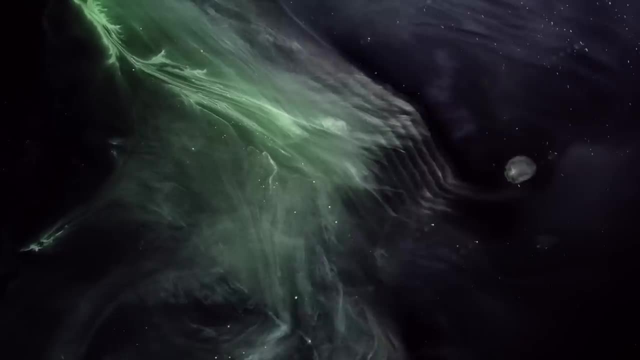 to, to be able to make any experiments, to, to be able to make any experiments that could test that, but that could test that, but that could test that. but as far as we know the um, as far as we know the um, as far as we know the um, gravitation, yeah. 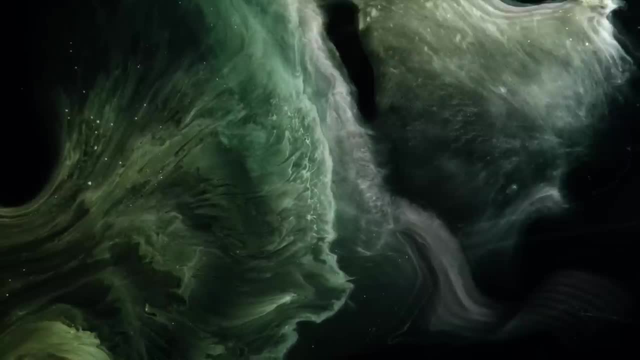 gravitation, yeah, gravitation, yeah it it it travels at the speed of light, it, it, it travels at the speed of light, it, it it travels at the speed of light. and would um, i i guess there would be. and would um i i guess there would be. 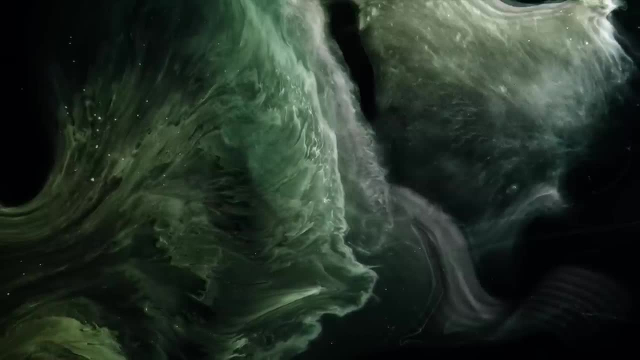 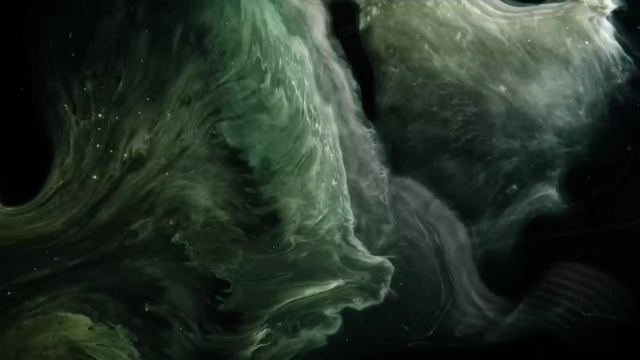 and would, um, i i guess there would be such effects. okay, uh, has there been any observed? okay, uh, has there been any observed? okay, uh, has there been any observed evidence supporting the theory of evidence, supporting the theory of evidence, supporting the theory of hawking radiation? 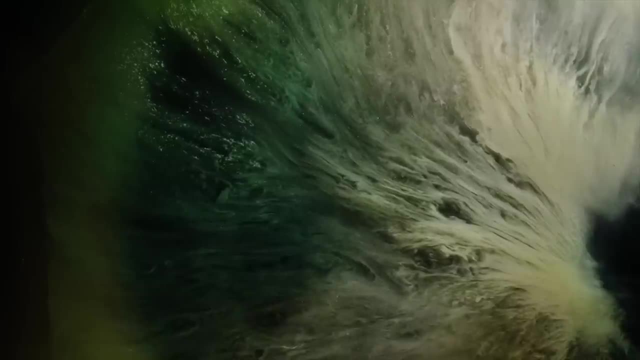 hawking radiation. hawking radiation: not yet, um, not yet, um, not yet, um that stephen hawking did an immense uh. that stephen hawking did an immense uh. that stephen hawking did an immense uh amount of very important work on the. 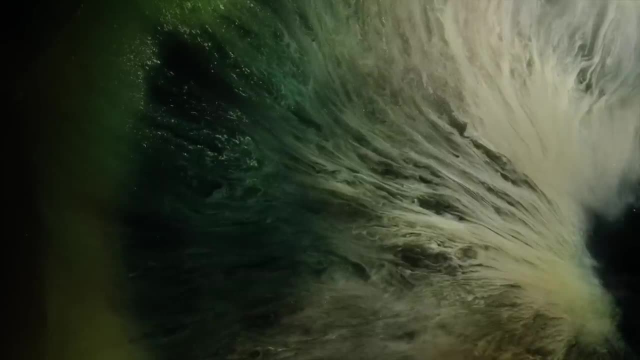 amount of very important work, on the amount of very important work on the theory of black holes, on theoretical theory of black holes, on theoretical theory of black holes, on theoretical black holes and black holes and black holes. and many of you will know if you've read his 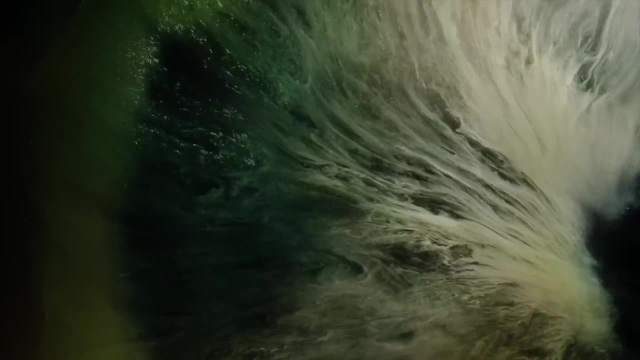 many of you will know if you've read his. many of you will know, if you've read his work, uh, that he predicted that, uh black work. uh that he predicted that, uh black work. uh that he predicted that, uh, black holes could evaporate due to the. 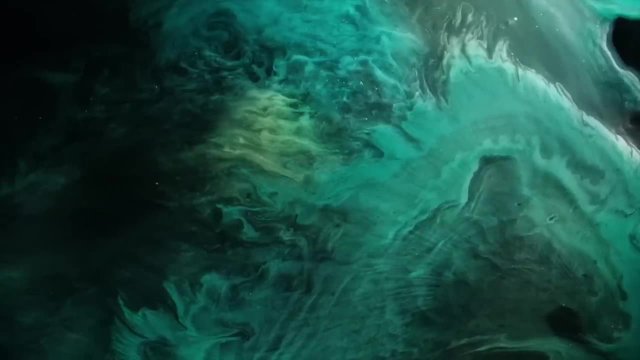 holes could evaporate due to the holes could evaporate due to the emission of hawking radiation. emission of hawking radiation. emission of hawking radiation um actually in terms of astrophysical um, actually in terms of astrophysical um, actually in terms of astrophysical black holes. 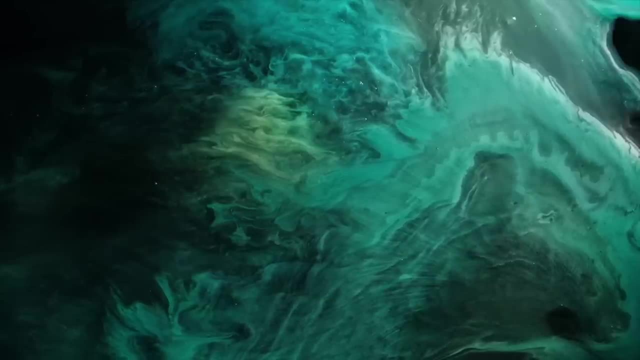 black holes, black holes, then the level of energy that comes out. then the level of energy that comes out, then the level of energy that comes out due to hawking radiation is tiny, due to hawking radiation is tiny, due to hawking radiation is tiny. okay, so if we were to look at one of 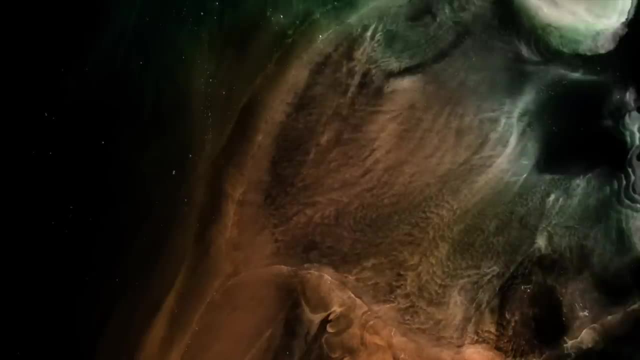 okay. so if we were to look at one of? okay. so if we were to look at one of these super massive black holes, these super massive black holes, these super massive black holes, then the energy that comes out in the, then the energy that comes out in the then the energy that comes out in the lifetime of the universe, lifetime of the universe, lifetime of the universe. in hawking radiation is less than the. in hawking radiation is less than the. in hawking radiation is less than the energy of one optical photon. 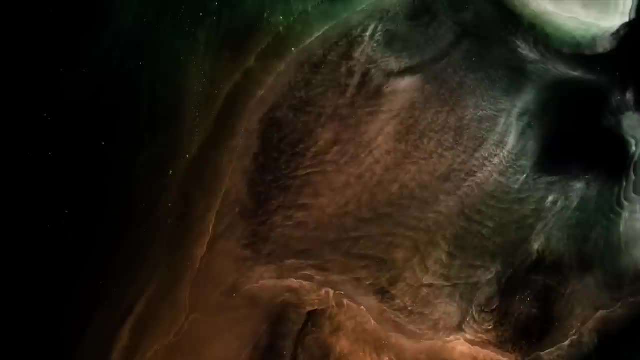 energy of one optical photon. energy of one optical photon. it's only from very small black holes, it's only from very small black holes. it's only from very small black holes that you expect to see that you expect to see, that you expect to see, uh, hawking radiation by small black. 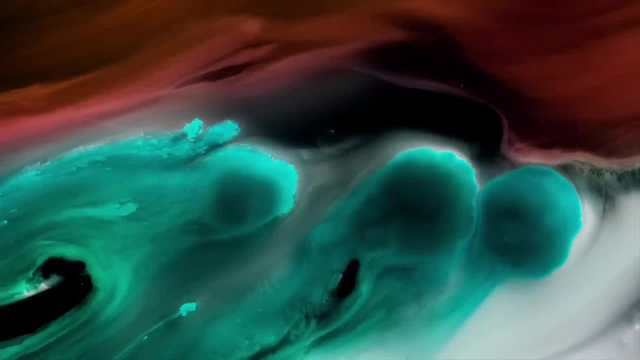 uh, hawking radiation by small black, uh, hawking radiation. by small black holes, i mean ones of masses, much less holes. i mean ones of masses, much less holes. i mean ones of masses, much less than the mass of the earth, than the mass of the earth. 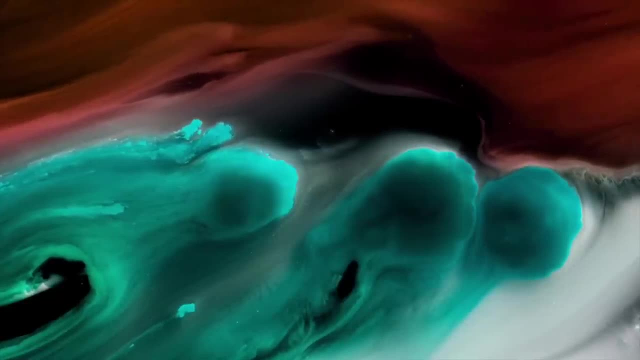 than the mass of the earth. and we don't know of any such black and we don't know of any such black and we don't know of any such black holes. it doesn't mean say they can't holes. it doesn't mean say they can't. 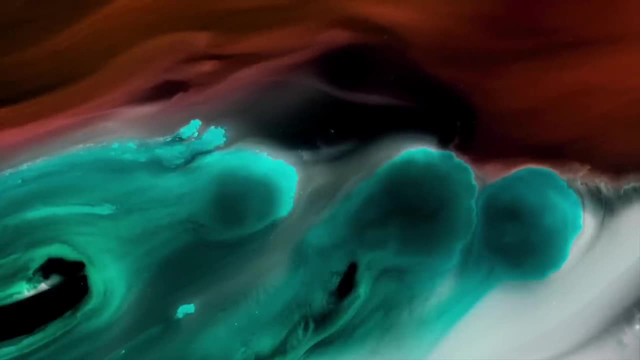 holes. it doesn't mean say they can't exist, but we exist, but we exist, but we, we can think of no way to form them. we can think of no way to form them. we can think of no way to form them other than in the primordial big bang. 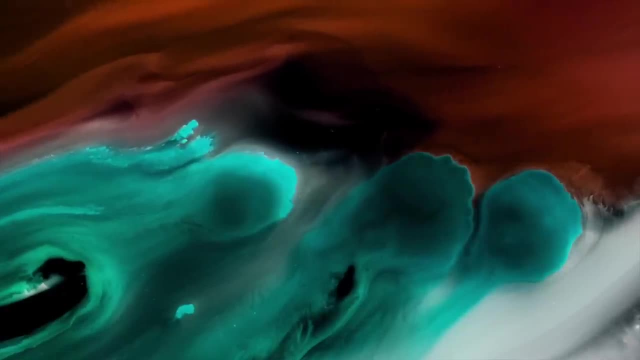 other than in the primordial big bang, other than in the primordial big bang, and uh there's currently no evidence and uh there's currently no evidence and uh there's currently no evidence that uh such black holes form during that uh, such black holes form during. 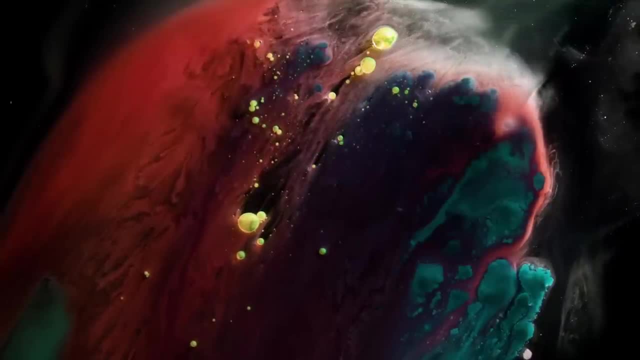 that, uh, such black holes form during the big bang, the big bang, the big bang. but who knows, uh, maybe somebody will. but who knows, uh, maybe somebody will. but who knows, uh, maybe somebody will discover such objects in the future, discover such objects in the future, discover such objects in the future? okay, so, uh, so, the next one is what? 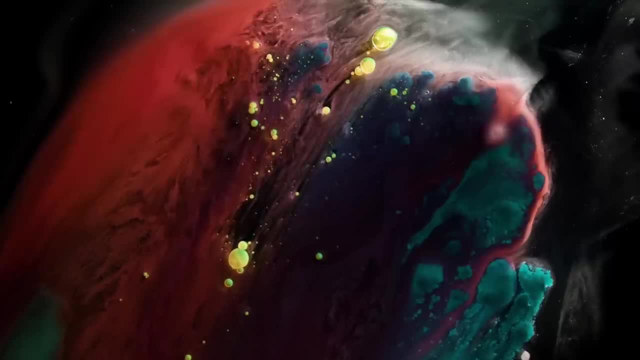 okay, so, uh. so the next one is: what? okay, so, uh. so the next one is what actually actually actually robbed space and time mean if possible. robbed space and time mean if possible. robbed space and time mean if possible. can you please explain it in an easy? can you please explain it in an easy? 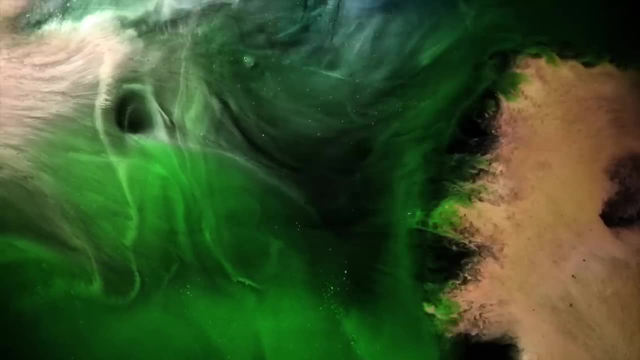 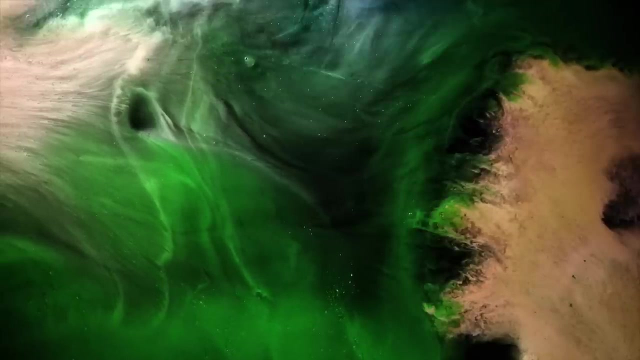 can you please explain it in an easy language? yeah, i mean it's, i mean you. yeah, i mean it's, i mean you. yeah, i mean it's, i mean you. if you go up in and look at. if you go up in and look at, if you go up in and look at look through a glass, look at, look through. 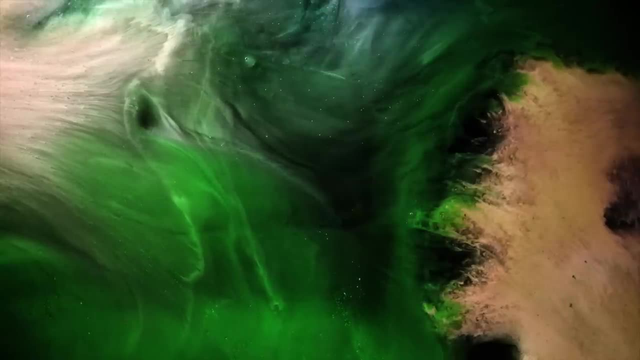 look through a glass, look at, look through, look through a glass, look at, look through legs and so forth. what you're doing, legs and so forth, what you're doing, legs and so forth- what you're doing is, uh, warping our appearance of space. is, uh, warping our appearance of space? 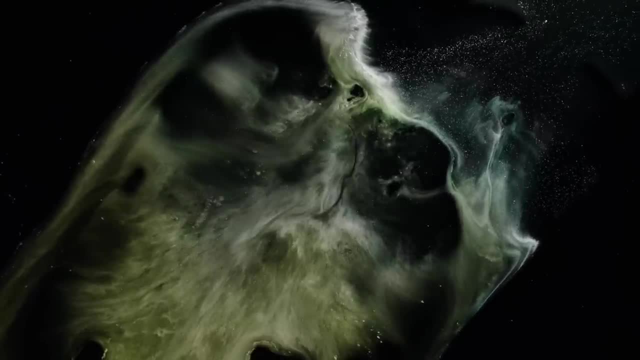 is, uh, warping our appearance of space. i don't know how to watch the appearance. i don't know how to watch the appearance. i don't know how to watch the appearance of time. i'm afraid of time, i'm afraid of time, i'm afraid, you know, maybe you can drink something, but 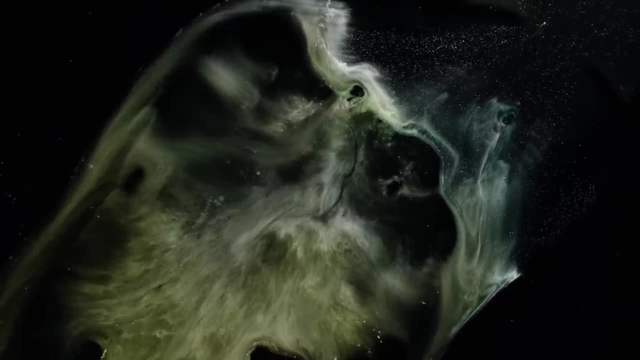 you know, maybe you can drink something. but you know, maybe you can drink something, but that's that will be personal to you. that's that will be personal to you. that's that will be personal to you. um, the, um, the, um, the but the effect on time gravity. 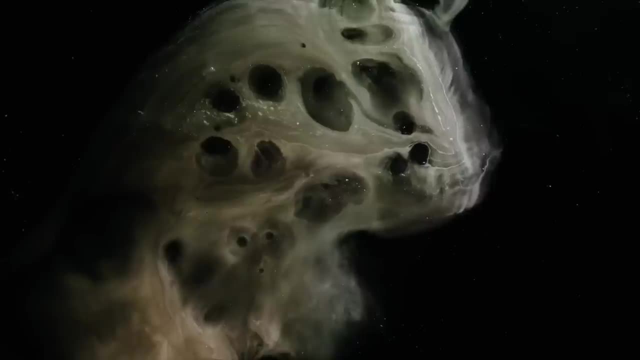 but the effect on time, gravity, but the effect on time, gravity, effect on time is, as i say, something, effect on time is, as i say, something, effect on time is, as i say, something we live with in terms of if you have a, we live with in terms of if you have a. 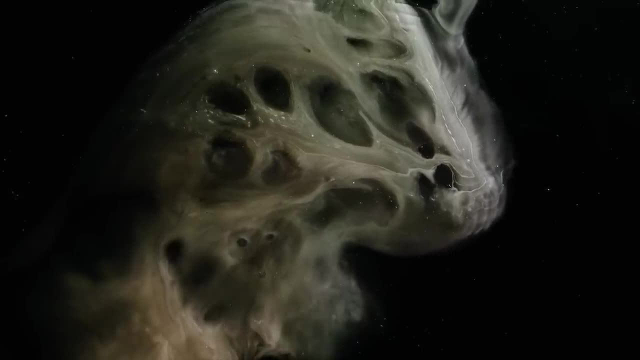 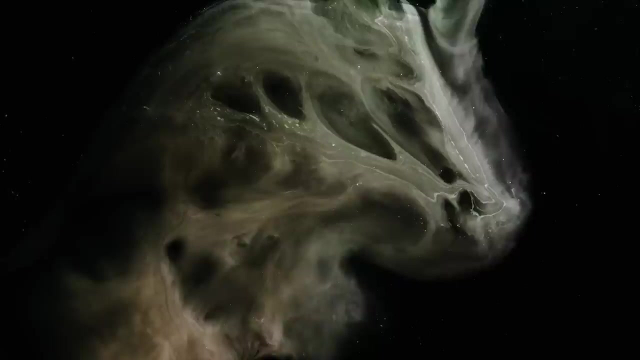 we live with in terms of if you have a sat nav, sat nav, but it just means that basically time, but it just means that basically time, but it just means that, basically, time is being completely distorted. it's not is being completely distorted. it's not is being completely distorted, it's not something. 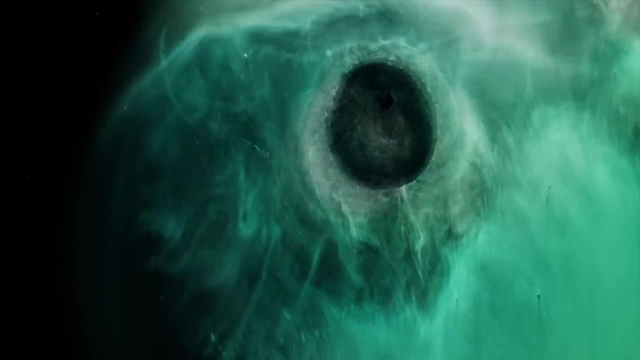 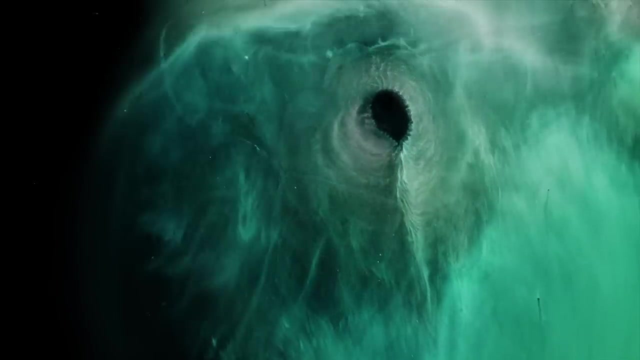 something, something absolute. there's not a rigid framework absolute. there's not a rigid framework absolute. there's not a rigid framework somewhere, somewhere, somewhere of space and time which is rigid, it's of space and time which is rigid, it's of space and time which is rigid, it's affected by the presence of matter. 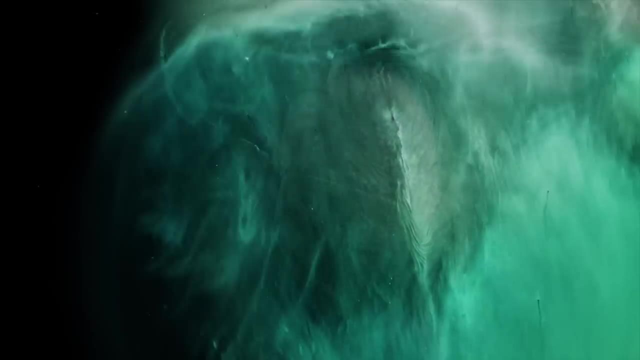 affected by the presence of matter. affected by the presence of matter. matter. you know changes and affects matter. you know changes and affects matter. you know changes and affects space-time, space-time, space-time and actually space-time affects the way and actually space-time affects the way and actually space-time affects the way that matter behaves. 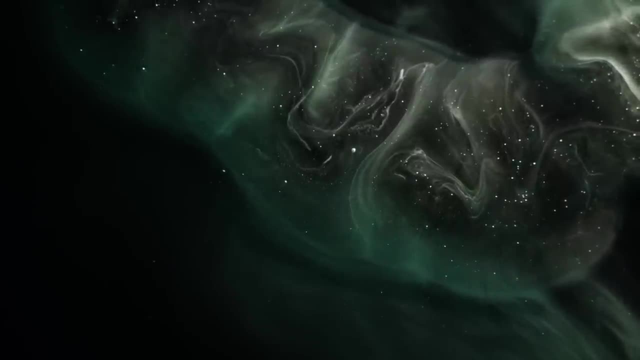 that matter behaves. that matter behaves. there's a sort of symbiosis there. there's a sort of symbiosis there. there's a sort of symbiosis there. okay, sir, uh. the next one is uh. can two? okay, sir, uh. the next one is uh. can two. okay, sir, uh. the next one is uh, can two neighboring black holes. 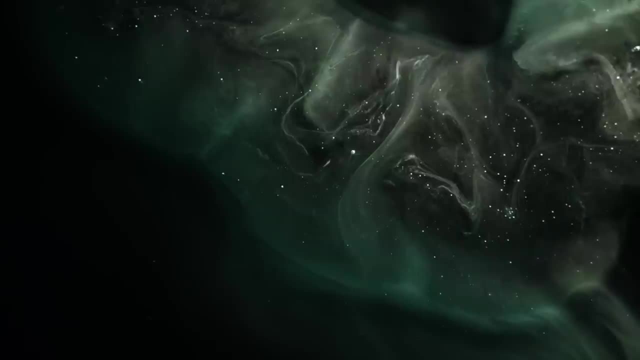 neighboring black holes. neighboring black holes spinning in opposite direction: repel each. spinning in opposite direction. repel each. spinning in opposite direction. repel each other. i don't think that they can repel each. i don't think that they can repel each. i don't think that they can repel each other. 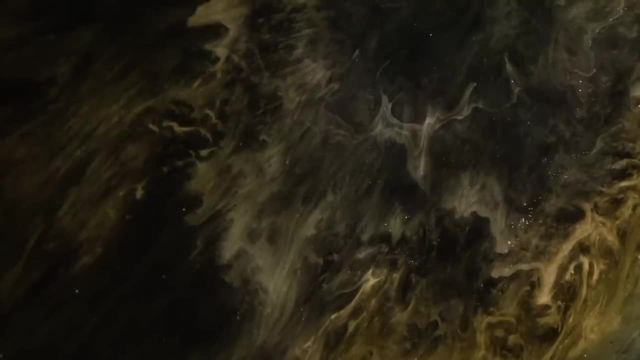 other other. i it's an interesting question, but i it's an interesting question, but i it's an interesting question, but certainly people have done lots of, certainly people have done lots of, certainly people have done lots of studies of merging of black holes. studies of merging of black holes. 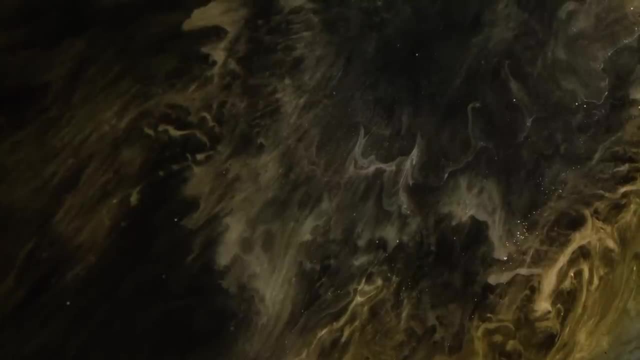 studies of merging of black holes, including spinning black holes, and ones including spinning black holes, and ones including spinning black holes, and ones that are spinning, that are spinning, that are spinning opposite to each other. so, rather than opposite to each other, so rather than opposite to each other. so, rather than going round together, 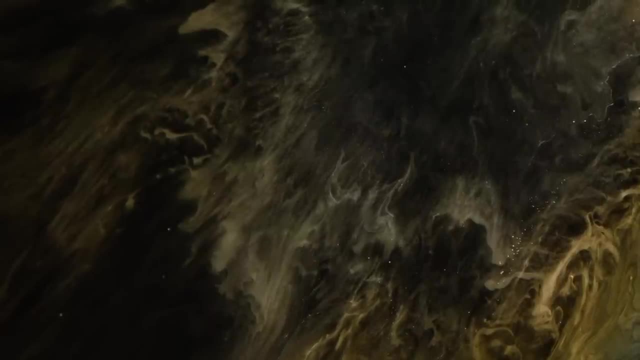 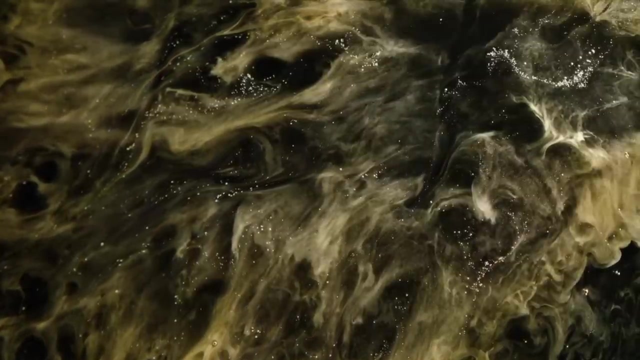 going round together. going round together, they're going against each other. uh, they're going against each other. uh, they're going against each other. uh, such simulations show interesting. such simulations show interesting. such simulations show interesting features, features, features, but they don't show them being repelled. 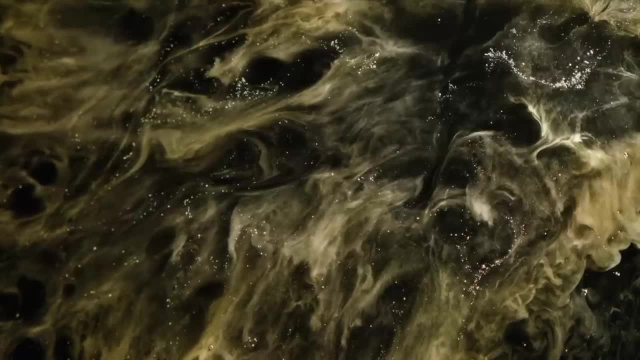 but they don't show them being repelled. but they don't show them being repelled. the one interesting thing just in terms. the one interesting thing just in terms. the one interesting thing just in terms of, of, of repulsion. okay, i just want to mention repulsion. okay, i just want to mention. 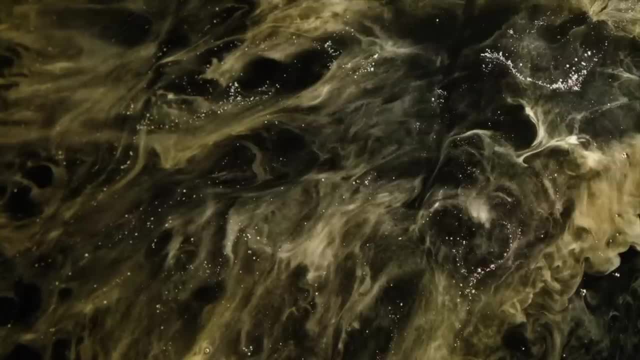 repulsion. okay, i just want to mention is if you have two black holes, which is if you have two black holes, which is if you have two black holes which come together and merge. when they come together and merge, when they come together and merge, when they finally merge, they merge at a particular. 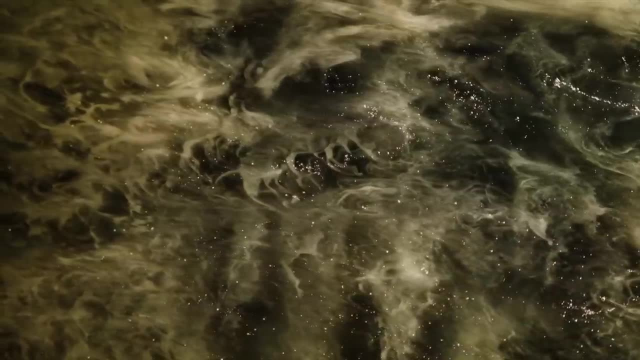 finally merge. they merge at a particular finally merge. they merge at a particular angle, angle, angle, okay, and if you think about it, you know okay, and if you think about it, you know okay. and if you think about it, you know that's something a little odd. they have 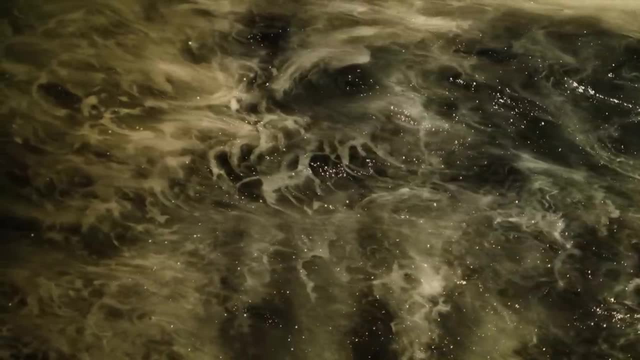 that's something a little odd. they have. that's something a little odd. they have to to to. it's something to do with the initial. it's something to do with the initial. it's something to do with the initial conditions, but they conditions, but they conditions, but they, they merge along a particular angle. okay. 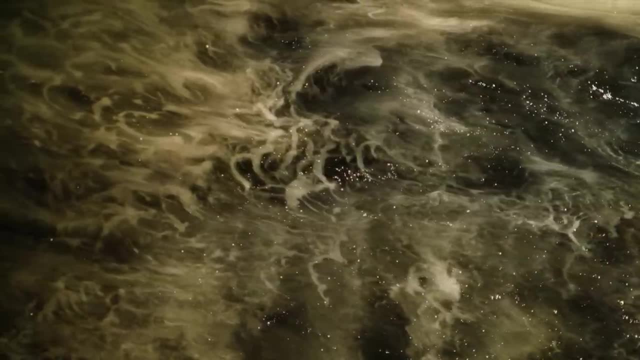 they merge along a particular angle. okay, they merge along a particular angle, okay, and that means because they're sending, and that means because they're sending, and that means because they're sending out gravitational waves, out gravitational waves, out gravitational waves, and gravitational waves carry momentum and gravitational waves carry momentum. 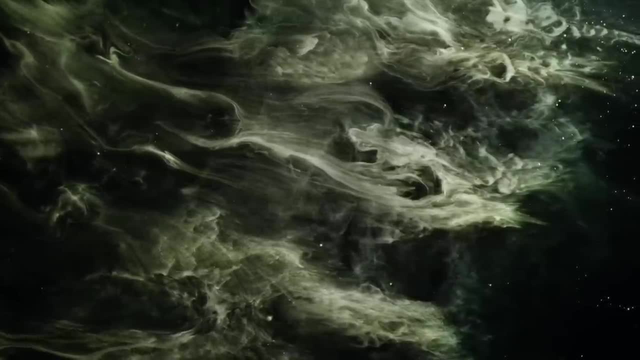 and gravitational waves carry momentum. so there's a problem about momentum. okay, so there's a problem about momentum, okay, so there's a problem about momentum, okay, and this can lead to a recoil, and this can lead to a recoil, and this can lead to a recoil of the collapsed object. 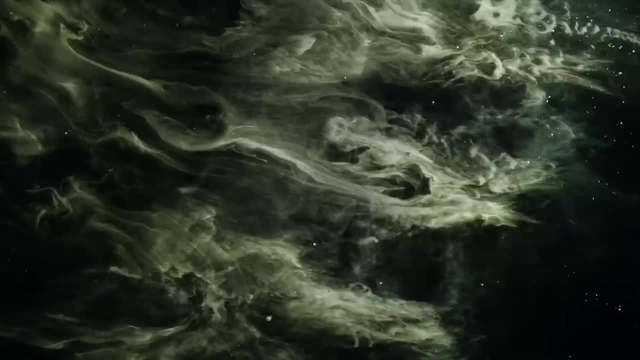 of the collapsed object, of the collapsed object, so the black holes come together, emerge. so the black holes come together, emerge. so the black holes come together, emerge to form an object, to form an object, to form an object, and depending upon and depending upon, and depending upon the spin of those objects, 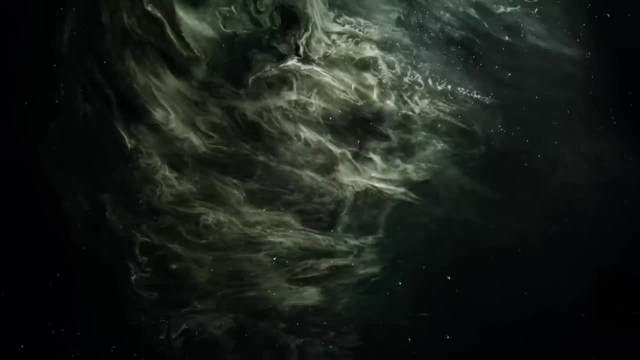 the spin of those objects, the spin of those objects, etc. etc. etc. so it could shoot off and you could get. so it could shoot off and you could get. so it could shoot off and you could get an example where the the resulting black. an example where the the resulting black. 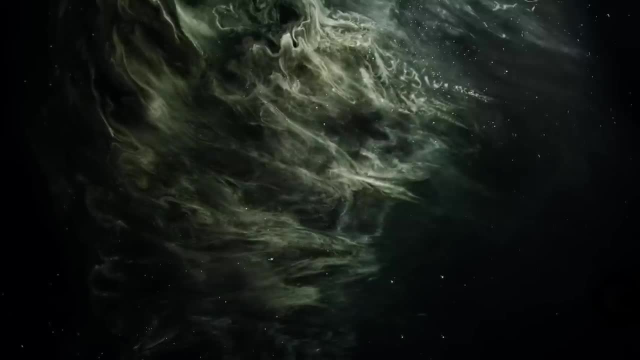 an example where the, the resulting black hole has a velocity of hundreds of hole, has a velocity of hundreds of hole, has a velocity of hundreds of kilometers per second, kilometers per second, kilometers per second- and is ejected from the galaxy, and is ejected from the galaxy. and is ejected from the galaxy. i mean, people have started to look for 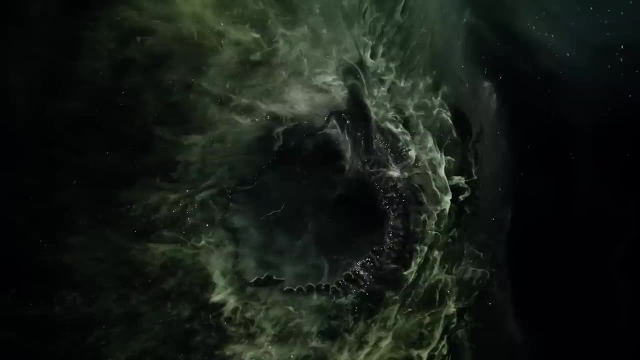 i mean people have started to look for. i mean people have started to look for such things, but that there are such things, but that there are such things, but that there are interesting things to do with how it goes. interesting things to do with how it goes. interesting things to do with how it goes, obviously. 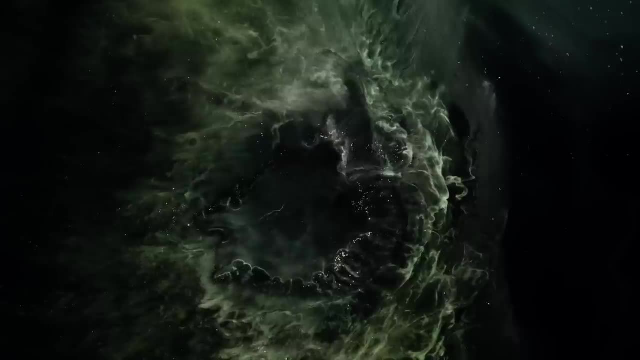 obviously, obviously. and if i could just say one thing about, and if i could just say one thing about, and if i could just say one thing about: the black hole merger, that is is amusing. the black hole merger, that is is amusing. the black hole merger, that is is amusing to do. 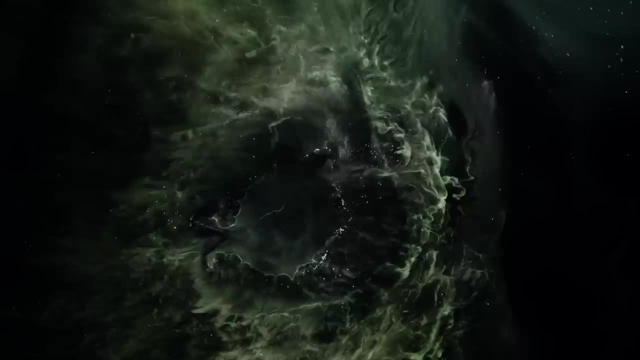 to do. to do is um get a dinner plate um don't get is um get a dinner plate um don't get is um get a dinner plate um don't get your um, your um your um partner or mother or grandmother's best partner or mother or grandmother's best. 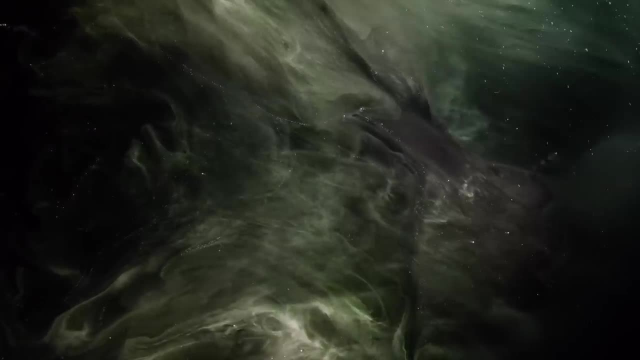 partner or mother or grandmother's best dinner plate, but it's an old plate dinner plate, but it's an old plate dinner plate, but it's an old plate, um, and you know, so you've got the plate. um, and you know, so you've got the plate. 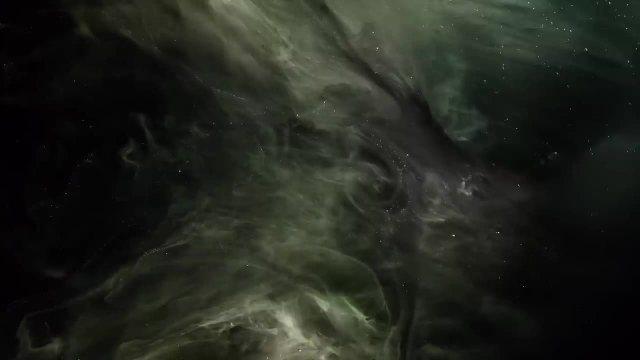 um, and you know, so you've got the plate and put it on a table and spin it so and put it on a table and spin it so and put it on a table and spin it, so it's sort of going round. you know like it's sort of going round, you know like. 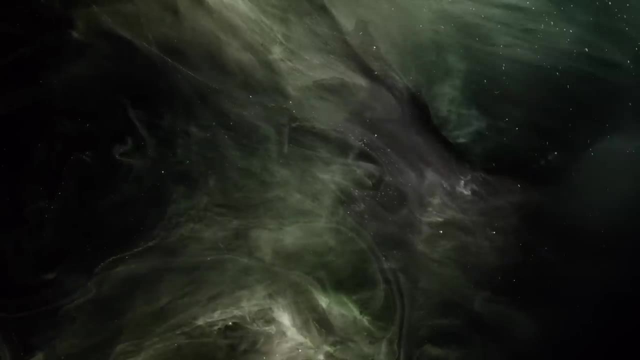 it's sort of going round, you know, like that: okay, so it spins around, and as that: okay, so it spins around. and as that: okay, so it spins around and as it. if you do it carefully, you can get it. it, if you do it carefully, you can get it. 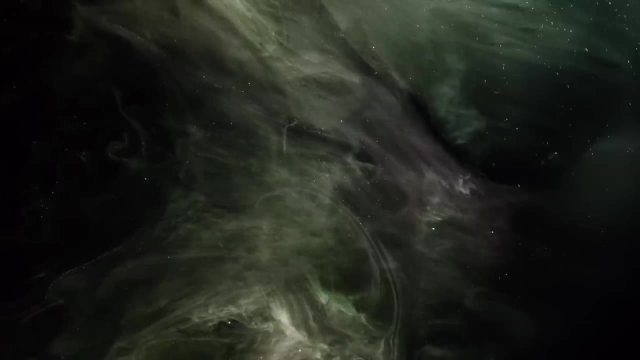 it. if you do it carefully, you can get it spinning for quite a long while, spinning for quite a long while, spinning for quite a long while, but eventually it'll start spinning, and but eventually it'll start spinning, and, but eventually it'll start spinning and it will. 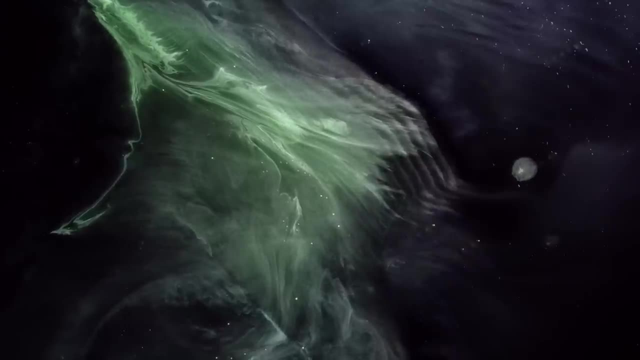 it will, it will, you know, go flat and in the final part, you know go flat, and in the final part, you know go flat. and in the final part of it, of it, of it, it actually the way in which the it actually the way in which the. 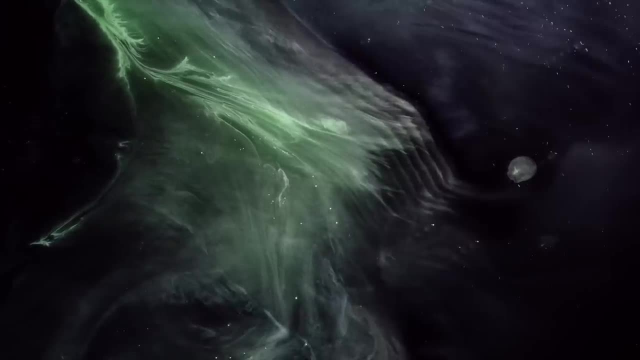 it actually the way in which the frequency with which it spins together, frequency with which it spins together, frequency with which it spins together, makes something which is uh, and it makes something which is uh, and it makes something which is uh, and it follows the chirp that i showed you in. 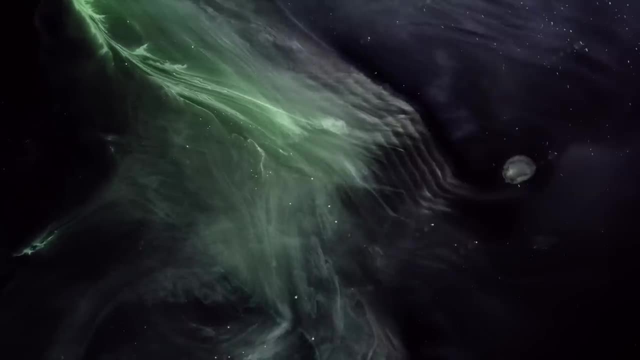 follows the chirp that i showed you in, follows the chirp that i showed you in that merger of the black holes. it's. it's that merger of the black holes. it's. it's that merger of the black holes. it's. it's a very similar development where it goes. 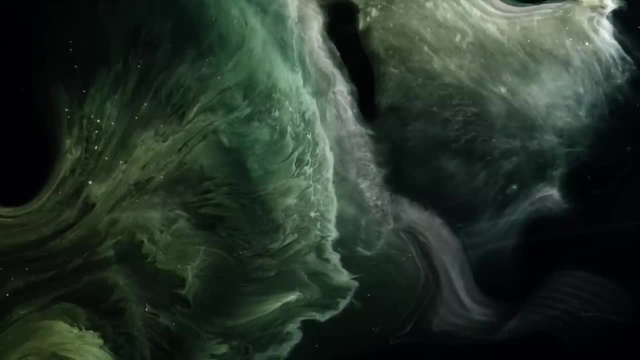 a very similar development where it goes. a very similar development where it goes faster and faster, faster and faster, faster and faster, and the frequency is going higher, and and the frequency is going higher, and, and the frequency is going higher and higher and the volume goes up, higher and the volume goes up. 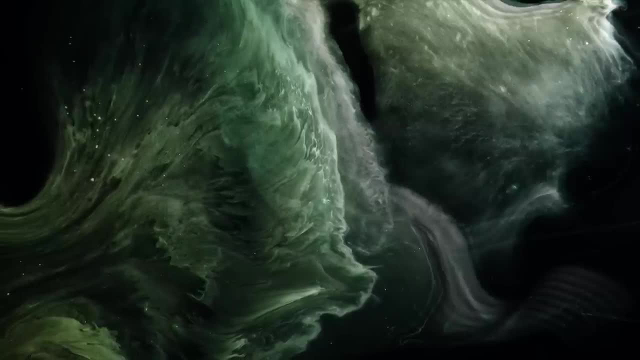 higher and the volume goes up. so that's a do-it-yourself experiment. so that's a do-it-yourself experiment. so that's a do-it-yourself experiment which is um telling you something, a which is um telling you something, a which is um telling you something a little bit about physics and how things. 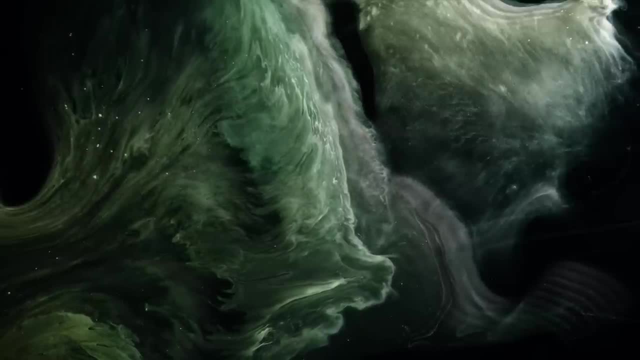 little bit about physics and how things. little bit about physics and how things can collapse, can collapse, can collapse, uh. so the next one is uh, uh. so the next one is uh, uh. so the next one is uh. last gravitational field, bend light. last gravitational field, bend light. 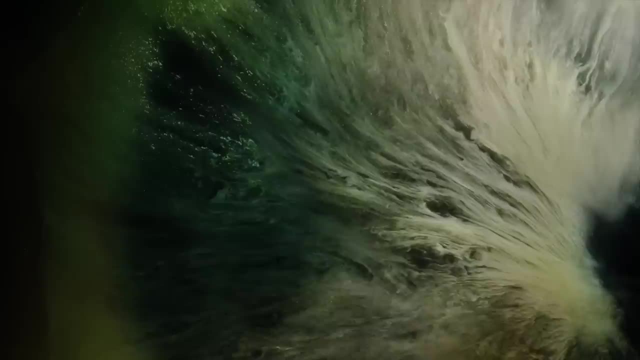 last gravitational field bend light. so there must exist a specific path. so there must exist a specific path, so there must exist a specific path through which the light moves and return through which the light moves and return through which the light moves and return back to its starting position. 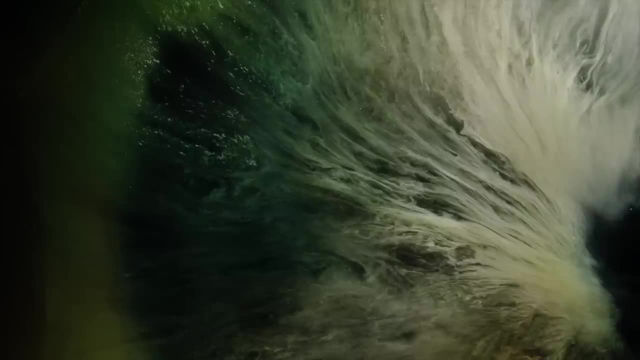 back to its starting position. back to its starting position, just like einstein thought experiment. just like einstein thought experiment. just like einstein thought experiment. it can allow time travel, can you please? it can allow time travel, can you please? it can allow time travel. can you please comment on this? 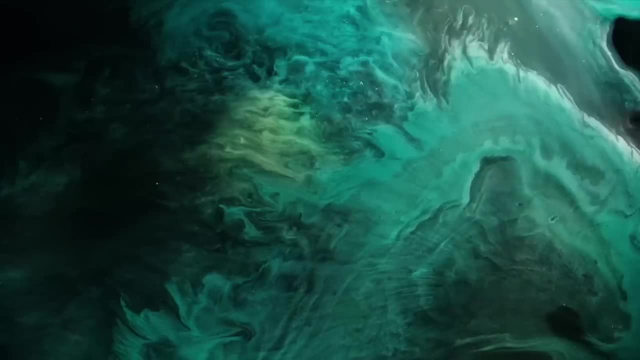 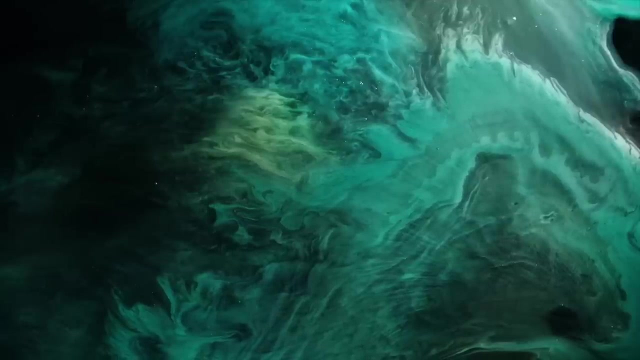 comment on this. comment on this: um, um, um, we, um, we, um, we, um. i don't know that. i don't know that, i don't know that we can actually. i mean, you can get light, we can actually. i mean, you can get light, we can actually. i mean you can get light to sort of turn back on itself. yes, 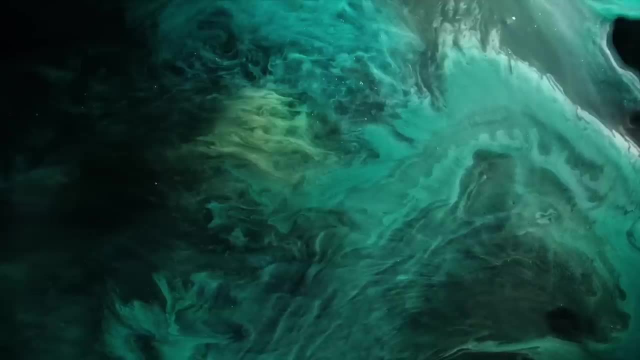 to sort of turn back on itself. yes, to sort of turn back on itself. yes, but uh, i don't see how you can actually but uh, i don't see how you can actually, but uh, i don't see how you can actually get, get, get um, couple that into. 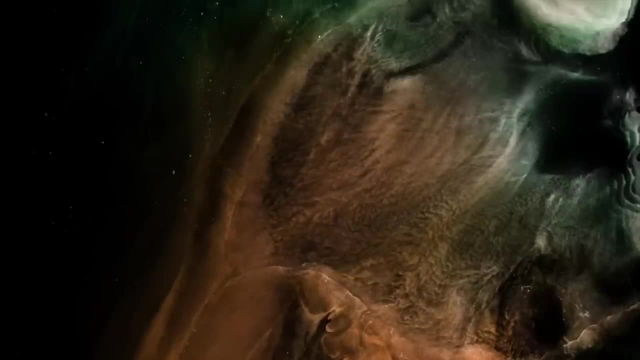 um couple that into um couple that into time travel, time travel, time travel. and i i'm just getting putting my and i i'm just getting putting my and i i'm just getting putting my neck out. now. i don't think time travel is neck out now. i don't think time travel is. 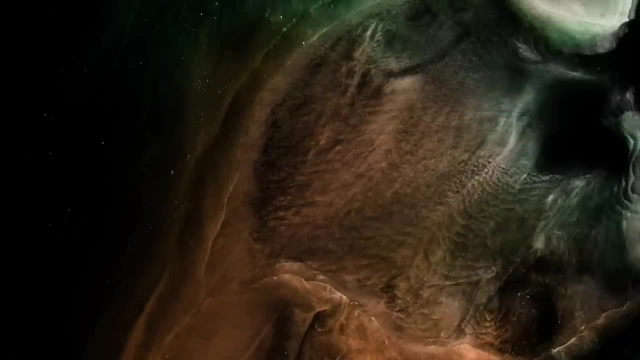 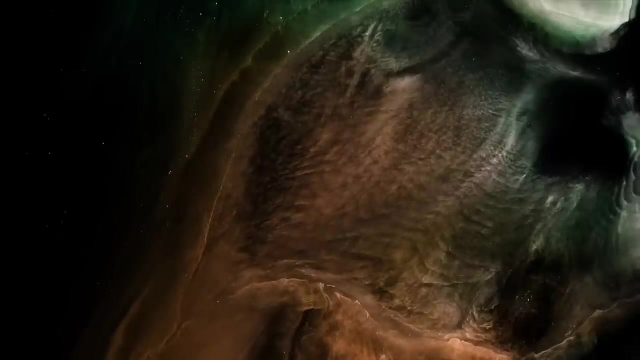 neck out now. i don't think time travel is possible, possible, possible, okay, but the only way to propose to do so is: but the only way to propose to do so is. but the only way to propose to do so is if you, if you, if you get something called a wormhole and you. get something called a wormhole. and you get something called a wormhole and you fall into that and it has to be in a fall into that, and it has to be in a fall into that and it has to be in a spinning black hole, spinning black hole. 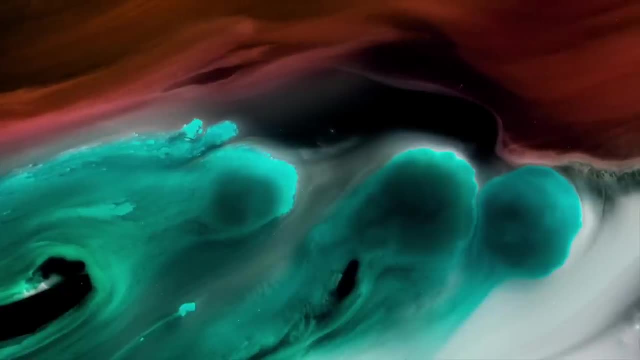 spinning black hole where the singularity is actually not a where the singularity is actually not a where the singularity is actually not a point. it's a ring and you have to fall. point. it's a ring and you have to fall. point. it's a ring and you have to fall through the ring. 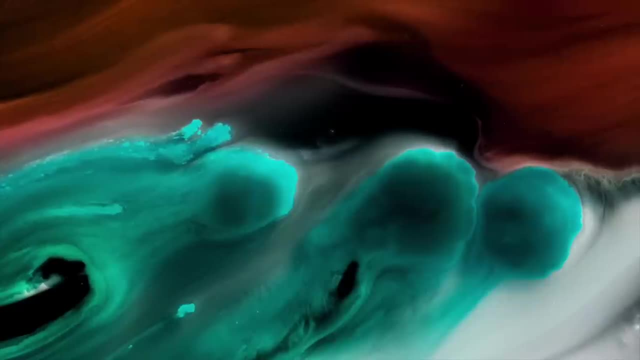 through the ring, through the ring. um. i think you'll be killed in doing um. i think you'll be killed in doing um. i think you'll be killed in doing that, but um that, but um that, but um. what you do is you end up in another. 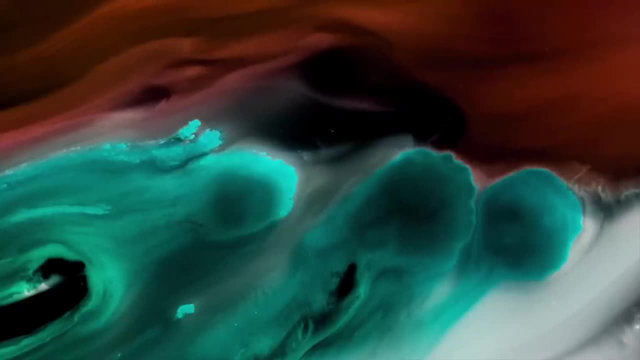 what you do is you end up in another. what you do is you end up in another universe, universe, universe, so if that is if there are other, so if that is if there are other, so if that is if there are other universes, i don't even know about that. 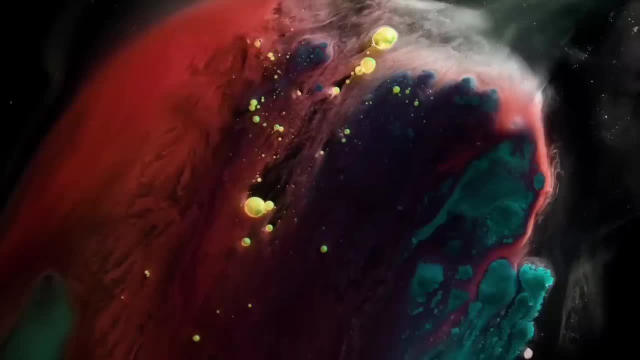 universes. i don't even know about that. universes, i don't even know about that. but um, but, um, but um. i personally, um, yeah, i personally, um, yeah, i personally, um, yeah, actually, most of us love to love to. actually, most of us love to love to. 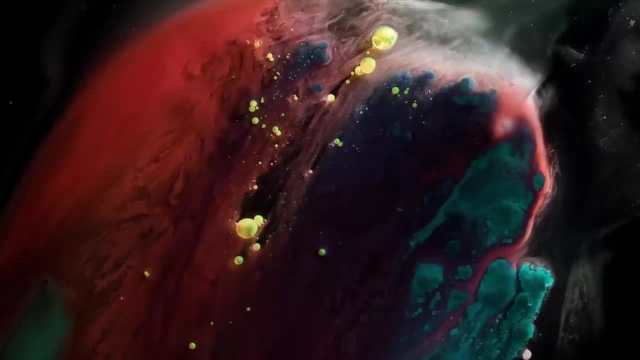 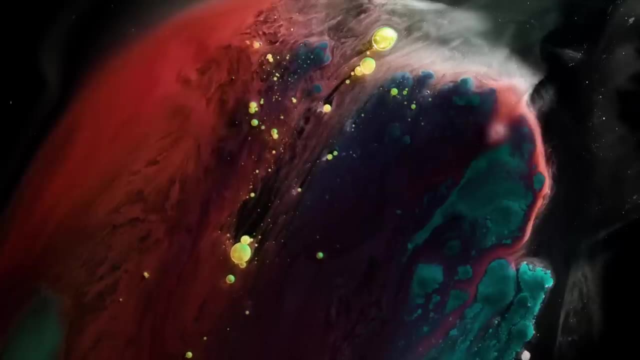 actually most of us love to love to watch star treks and star wars, watch star treks and star wars, watch star treks and star wars and so and so and so, oh yeah, oh yeah, oh yeah. okay, sir, so the next one is uh. okay, sir, so the next one is uh. 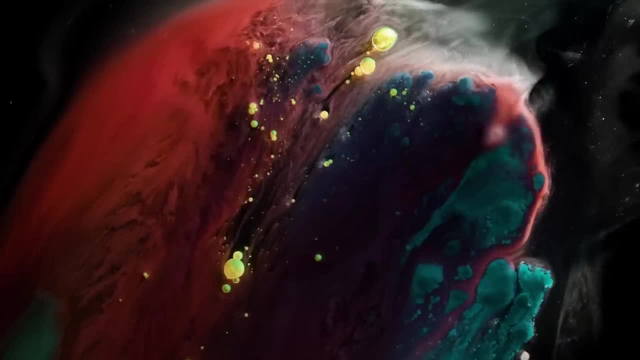 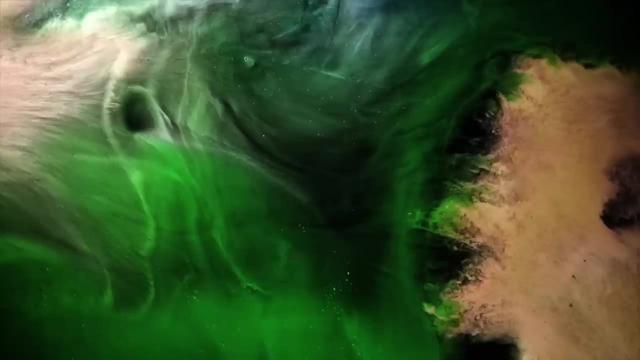 okay, sir. so the next one is: uh, uh. does spiral shape of milky way is a? uh. does spiral shape of milky way is a? uh. does spiral shape of milky way is a consequence of presence of black pool? consequence of presence of black pool. consequence of presence of black pool. no, i don't shape, yeah. 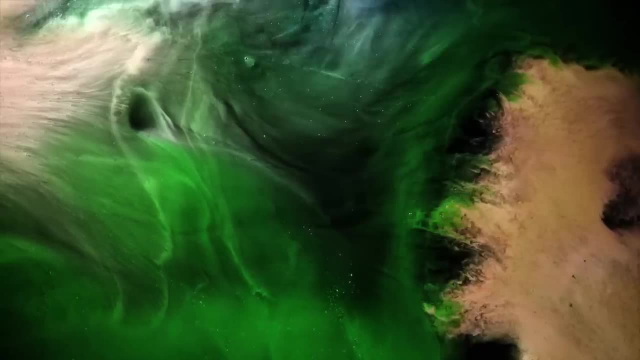 no, i don't shape. yeah, no, i don't shape. yeah, cause the spiral shape, the spiral shape, cause the spiral shape, the spiral shape, cause the spiral shape, the spiral shape. i think is because we've got the galaxy. i think is because we've got the galaxy. 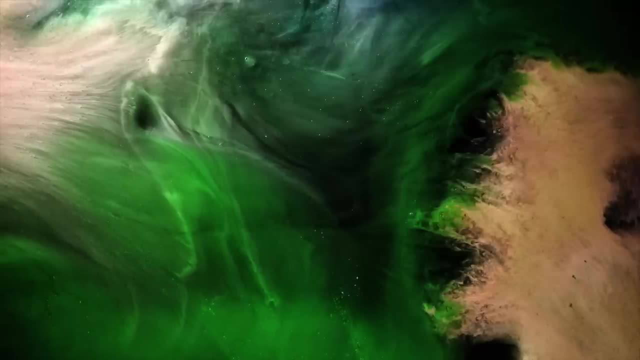 i think is because we've got the galaxy is a disc shape, is a disc shape and it's it's the spiral is caused by, and it's it's the spiral is caused by, and it's it's the spiral is caused by interactions within stars, and it's a 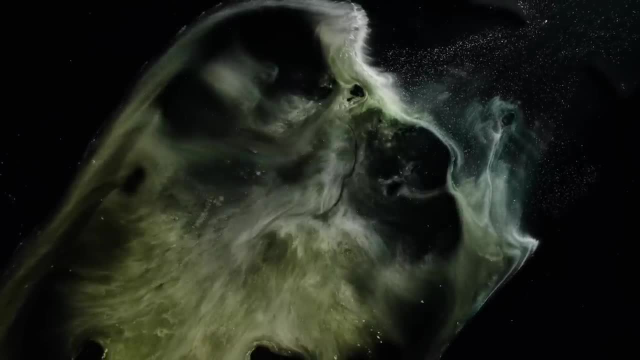 interactions within stars, and it's a interactions within stars and it's a self-gravity of the material in the disc. self-gravity of the material in the disc. self-gravity of the material in the disc, in other words, parts of the disc being, in other words, parts of the disc being. 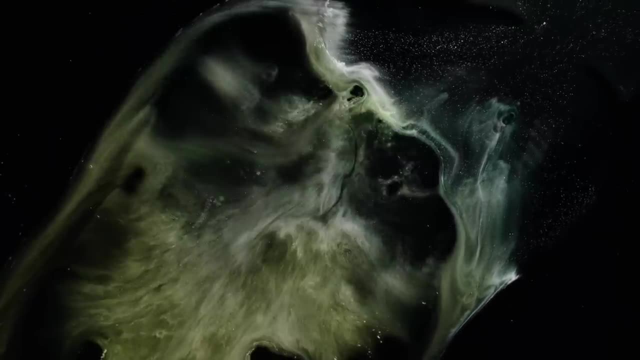 in other words, parts of the disc being gravitationally attracted to others. it gravitationally attracted to others. it gravitationally attracted to others. it creates an instability that leads to creates an instability that leads to creates an instability that leads to spiral arms. spiral arms. 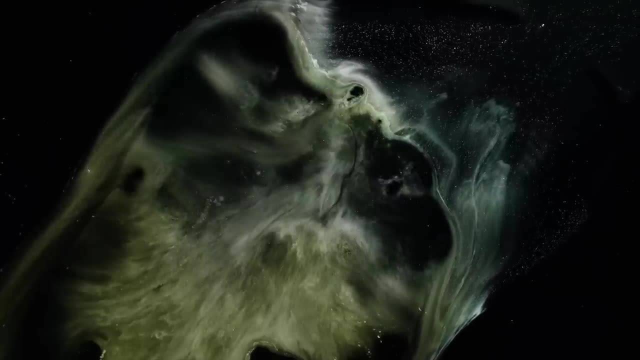 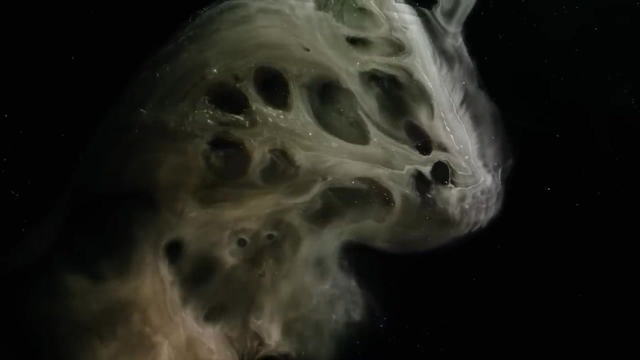 spiral arms. where the angular momentum from our, where the angular momentum from our, where the angular momentum from our galaxy came from in the first place. galaxy came from in the first place. galaxy came from in the first place, uh. so the next one is: why are super? uh, so the next one is: why are super? 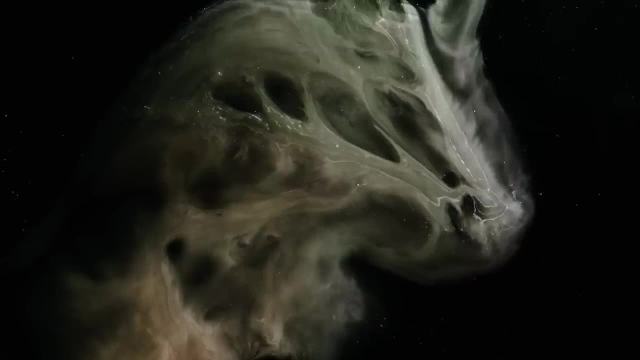 uh. so the next one is: why are super massive black holes always located at massive black holes, always located at massive black holes, always located at the center of galaxies, the center of galaxies, the center of galaxies? it's in the same way that, if you, if you, it's in the same way that if you, if you. 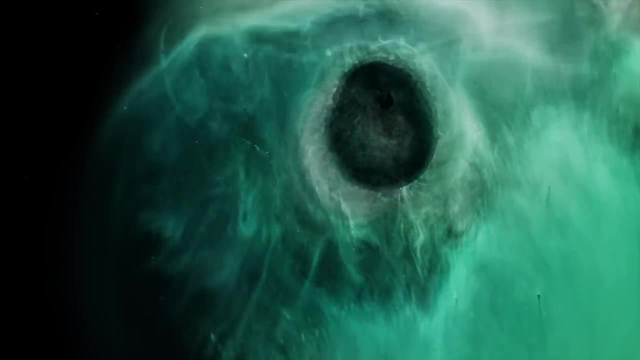 it's in the same way that if you, if you have a sort of, have a sort of, have a sort of a bowl with water in and you put mud and a bowl with water in, and you put mud and a bowl with water in and you put mud and stones in. 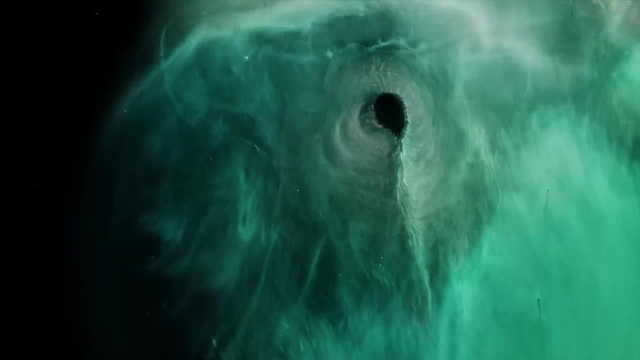 stones in stones in very quickly, the the um very quickly, the the um very quickly, the the um. stones go to the go to the bottom and stones go to the go to the bottom, and stones go to the go to the bottom and will go to the middle of the ball. 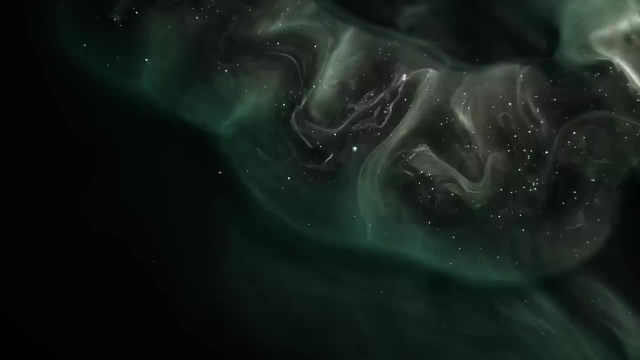 will go to the middle of the ball, will go to the middle of the ball and and the mud particles will float and and the mud particles will float and and the mud particles will float around and take a. you know if you leave around and take a, you know if you leave. 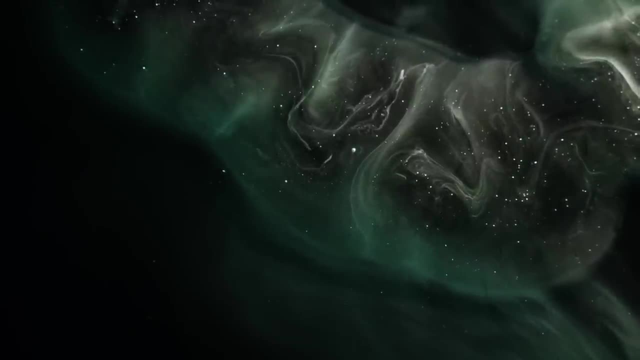 around and take a. you know, if you leave it long enough, the mud will settle out it long enough, the mud will settle out it long enough. the mud will settle out as well. but if you swirl it around, give as well. but if you swirl it around, give. 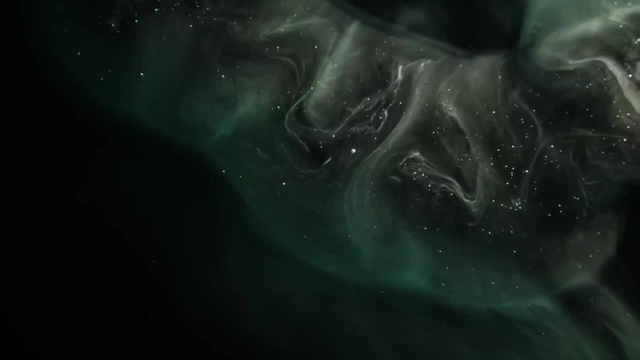 as well. but if you swirl it around, give it a bit of rotation, it a bit of rotation, it a bit of rotation, then they probably won't um, so it's, then they probably won't um, so it's, then they probably won't um, so it's because they're much the black holes. 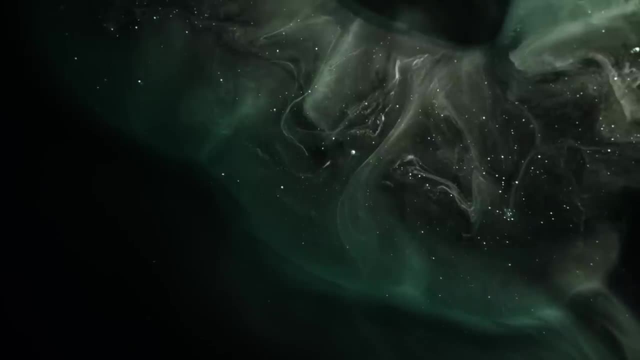 because they're much. the black holes? because they're much the black holes are much more massive than the stars, are much more massive than the stars, are much more massive than the stars, and so they move relatively and so they move relatively and so they move relatively to the stars that the black holes will. 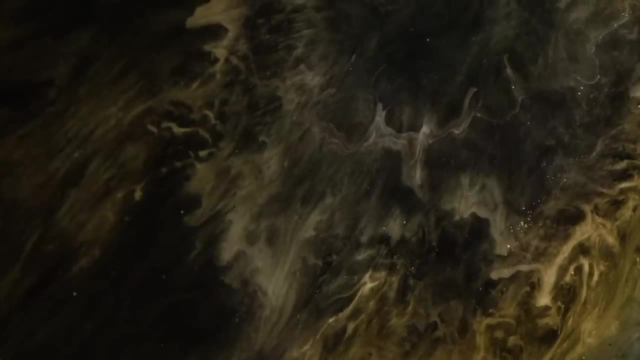 to the stars that the black holes will to the stars, that the black holes will move through a star field, move through a star field, move through a star field, and they will perturb it, and they and they will perturb it, and they and they will perturb it, and they actually 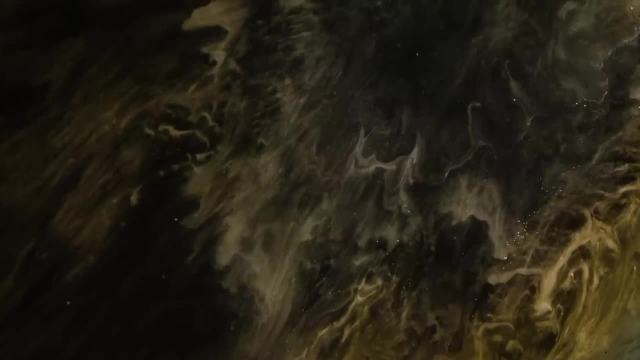 actually actually will through gravitational perturbations, will, through gravitational perturbations, will, through gravitational perturbations, they will transfer some of their energy. they will transfer some of their energy, they will transfer some of their energy to the stars and that will cause it them to the stars and that will cause it them. 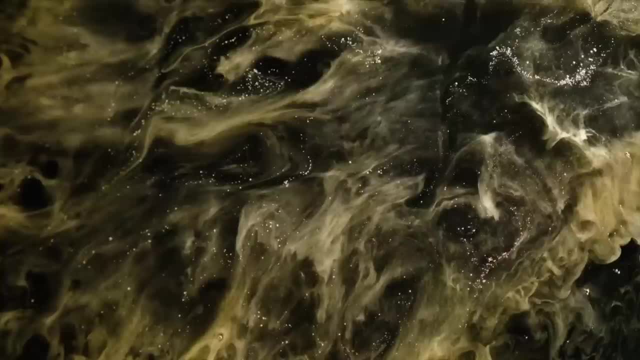 to the stars and that will cause it them to fall into the center. but that's how to the stars and that will cause it them to fall into the center. but that's how to the stars and that will cause it them to fall into the center. but that's how it works. 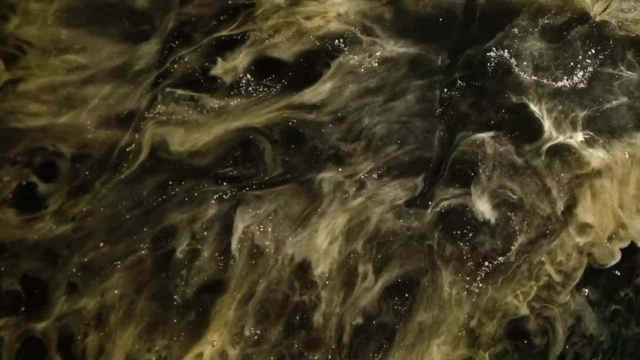 it works. it works. he said i'll pick up last three to four. he said i'll pick up last three to four. he said i'll pick up last three to four. questions now. questions now. questions now. the first one is matter that get lost in. the first one is matter that get lost in. 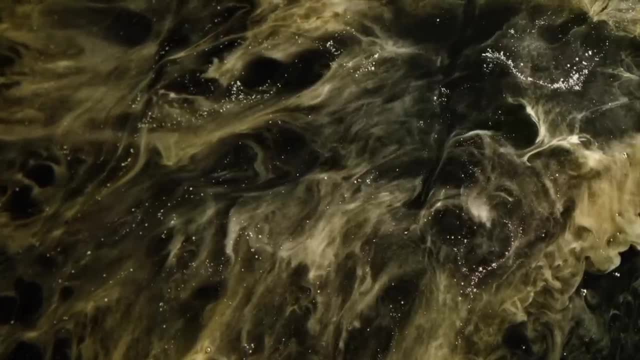 the first one is matter that get lost in black holes, black holes, black holes. so is it possible that a reverse higgs so is it possible that a reverse higgs so is it possible that a reverse higgs field, field, field is generated inside a back hole? that 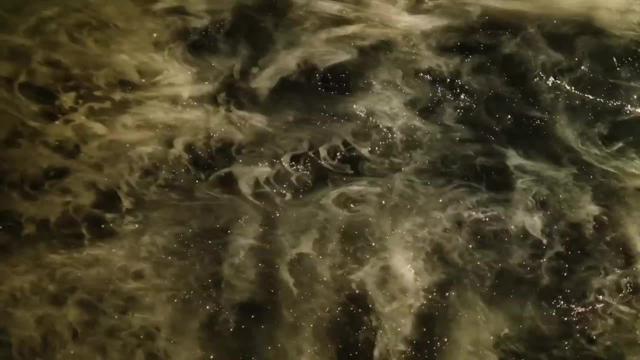 is generated inside a back hole. that is generated inside a back hole. that takes away the mass from the particles, takes away the mass from the particles. takes away the mass from the particles. just as higgs field provides mass to all. just as higgs field provides mass to all. 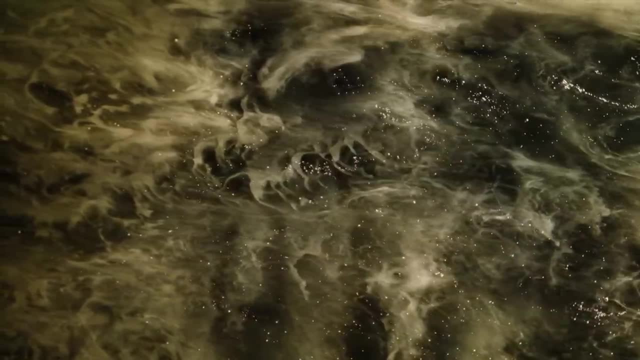 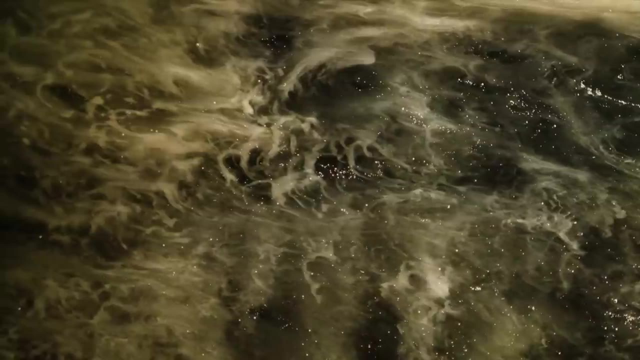 just as higgs field provides mass to all particles, particles, particles. sorry, i have no idea, sorry, i have no idea, sorry, i have no idea. so so like, so, so like, so, so like resist um and uh, so yeah, sorry, i can't. resist um and uh, so yeah, sorry, i can't. 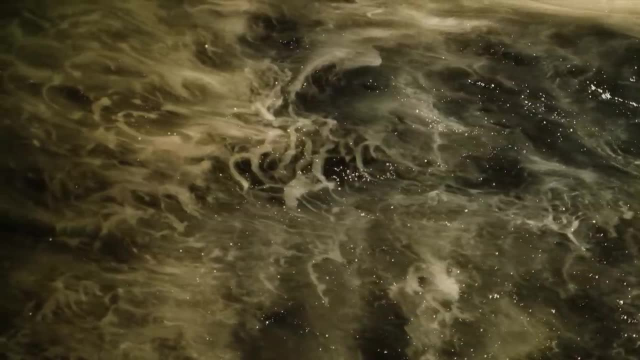 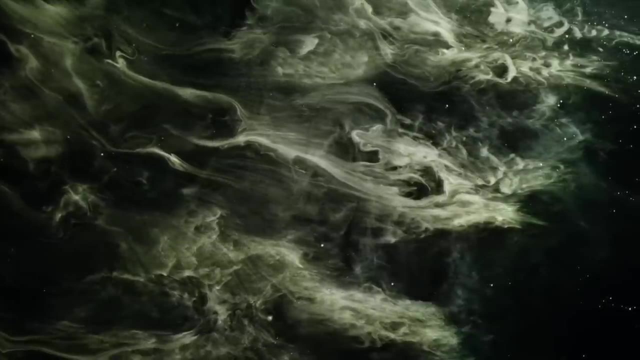 resist, um and uh. so, yeah, sorry, i can't answer that one. answer that one, answer that one. okay, sir, uh, let me ask you the next. okay, sir, uh, let me ask you the next. okay, sir, uh, let me ask you the next question. question, question. what will, what will happen if the sun 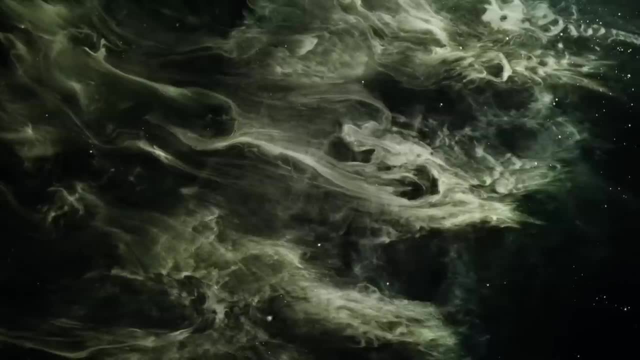 what will? what will happen if the sun? what will? what will happen if the sun turns into a black hole? the sun will not. the sun will not. the sun will not. turn into a black hole- okay, it will end. turn into a black hole: okay, it will end. 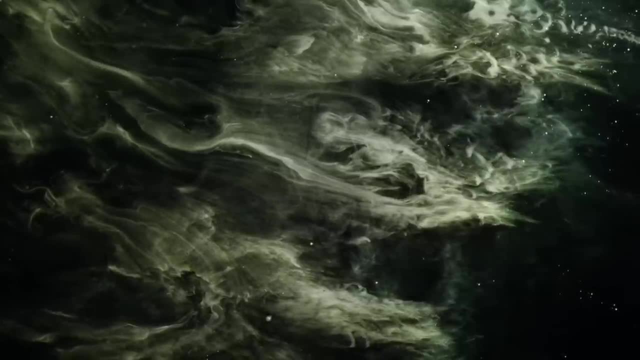 turn into a black hole. okay, it will end its life as a white dwarf. it will its life as a white dwarf. it will its life as a white dwarf. it will collapse to an object. the size of the collapse to an object. the size of the collapse to an object: the size of the earth. 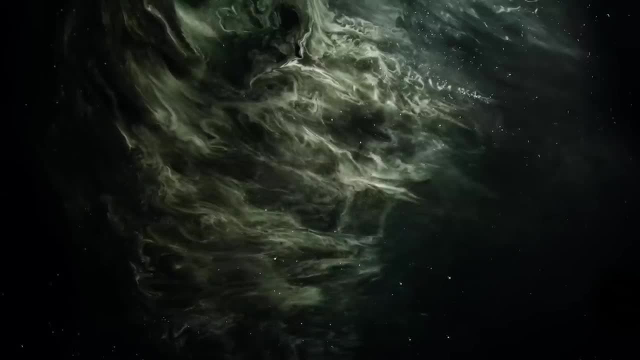 earth, earth. if, however, due to some unknown process. if, however, due to some unknown process. if, however, due to some unknown process, the sun was suddenly to convert to a, the sun was suddenly to convert to a. the sun was suddenly to convert to a black hole, black hole. 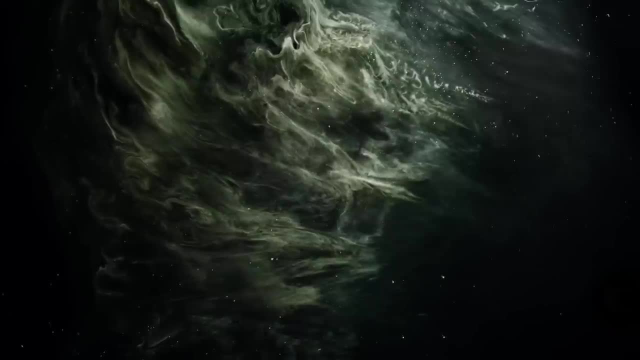 black hole. we could continue to orbit it. we could continue to orbit it. we could continue to orbit it and uh. roughly at the same radius. if and uh roughly at the same radius, if and uh. roughly at the same radius. if there was no math slots. there was no math slots. 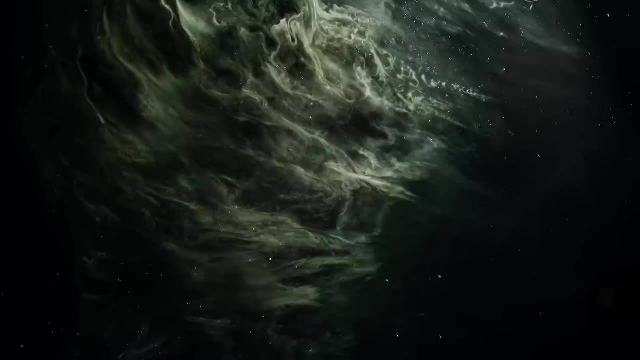 there was no math slots. i i you know, i don't know how this i i you know, i don't know how this i i you know, i don't know how this process would work, process would work, process would work. but um, basically, we would continue to. 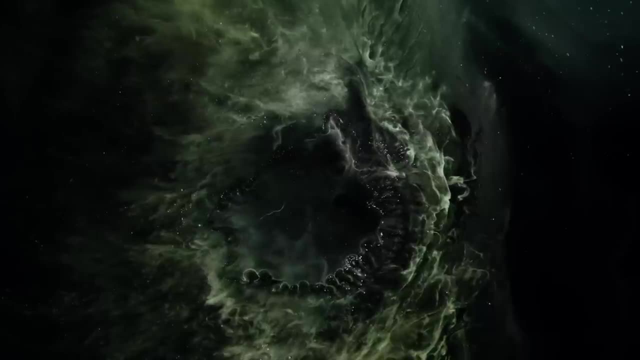 but um, basically, we would continue to, but, um, basically, we would continue to orbit it, so, orbit it. so, orbit it, so black. the idea that black holes suck black, the idea that black holes suck black, the idea that black holes suck everything in, everything in, everything in, is actually a false idea, and you need 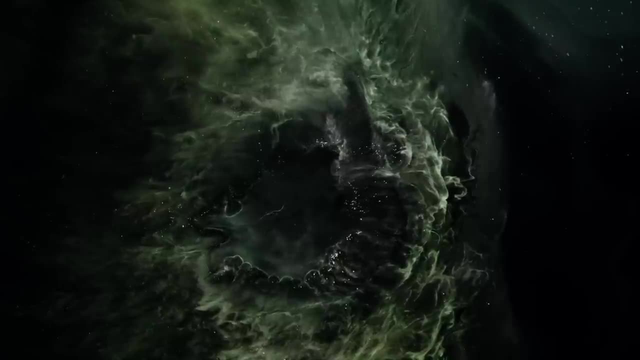 is actually a false idea. and you need is actually a false idea and you need friction to cause some of the friction, to cause some of the friction, to cause some of the to cause some matter to sink inwards and to cause some matter to sink inwards, and 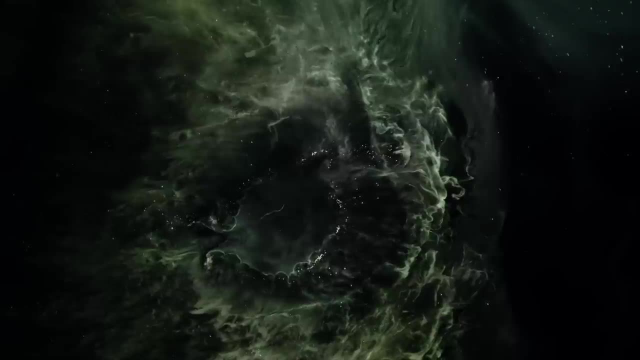 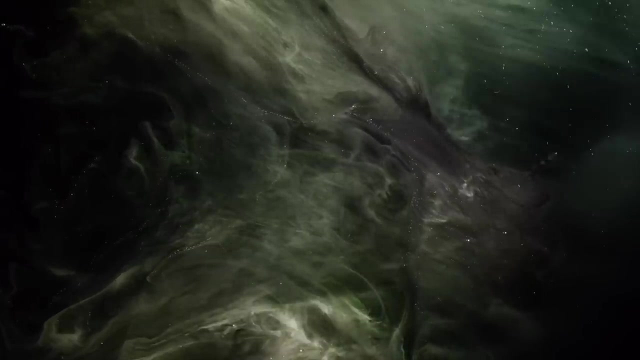 to cause some matter to sink inwards, and that requires that, requires that requires collisions and or magnetic fields. so what is your view on mass and spin? so what is your view on mass and spin? so what is your view on mass and spin of standard mass black holes? by fitting 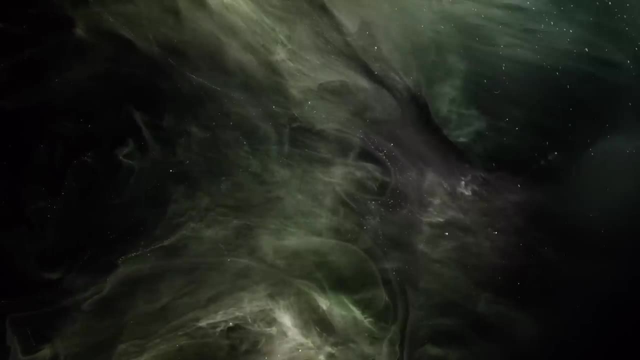 of standard mass black holes by fitting of standard mass black holes, by fitting the continuum x-ray spectrum. we um the what the work that i do we use. we um the what the work that i do we use. we um the what the work that i do. we use the. 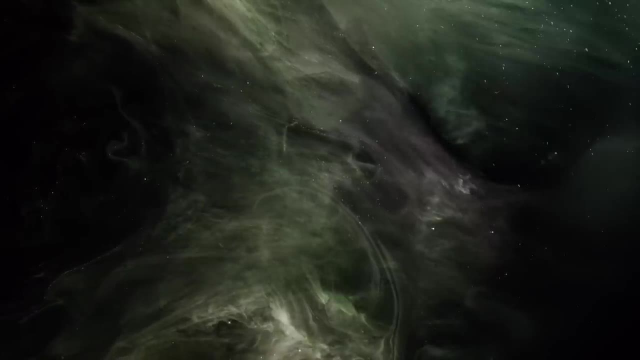 the, the imk line. there's another approach. which imk line? there's another approach: which imk line. there's another approach which is using, is using, is using the continuum measurements when they're the continuum measurements, when they're the continuum measurements when they're in the so-called soft state, when you're. 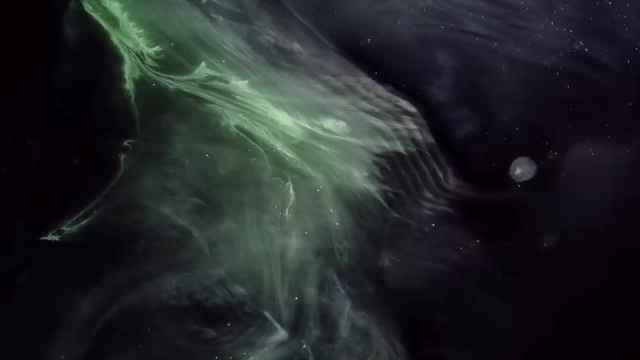 in the so-called soft state. when you're in the so-called soft state, when you're measuring, measuring, measuring the emission: the emission from the hot accretion disc, when from the hot accretion disc, when from the hot accretion disc when they're in a particular state. 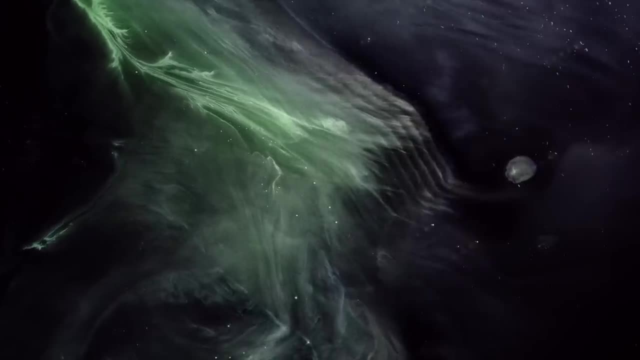 they're in a particular state. they're in a particular state that there's very fine work being done, that there's very fine work being done, that there's very fine work being done on that, on that, on that, by the late jeff mcclintock and others. 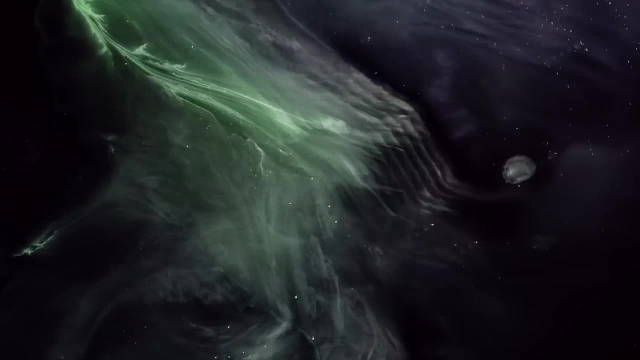 by the late jeff mcclintock and others, by the late jeff mcclintock and others. and uh, they often come up with answers. and uh, they often come up with answers. and uh, they often come up with answers which are very similar to ours. 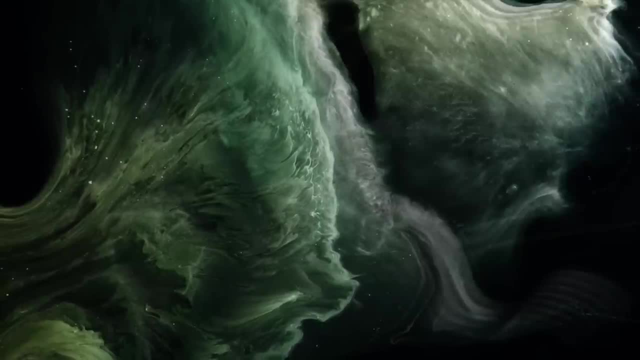 which are very similar to ours, which are very similar to ours, um on the same objects, if we actually um on the same objects, if we actually um on the same objects, if we actually happen to have them. so these are just happen to have them. so these are just. 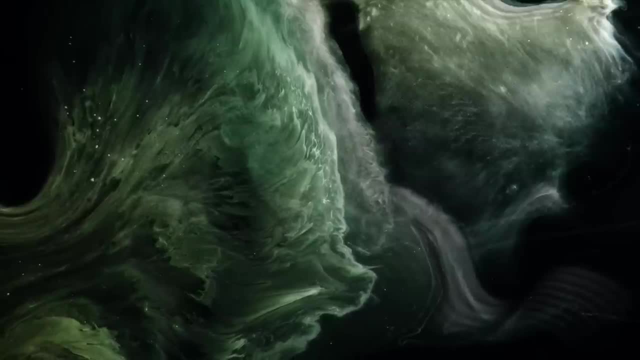 happen to have them. so these are just two uh ways of uh measuring um the two uh ways of uh measuring um the two uh ways of uh measuring um the properties and measuring the spin of the properties. and measuring the spin of the properties and measuring the spin of the black hole. 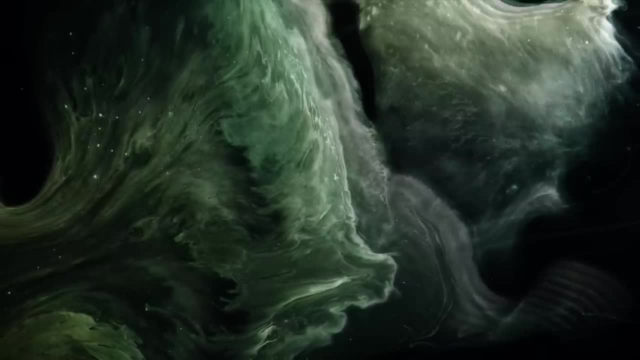 sir, i'll take up the last one. uh, is it, sir? i'll take up the last one. uh, is it, sir? i'll take up the last one. uh, is it possible to have more than one black? possible to have more than one black? possible to have more than one black pool in a galaxy? 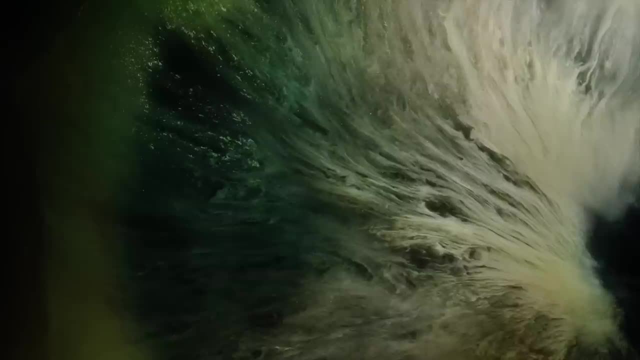 pool in a galaxy pool in a galaxy? um? yes, you can, if there's been a merger, um yes, you can. if there's been a merger, um yes, you can. if there's been a merger, you can end up with two black holes at. you can end up with two black holes at. 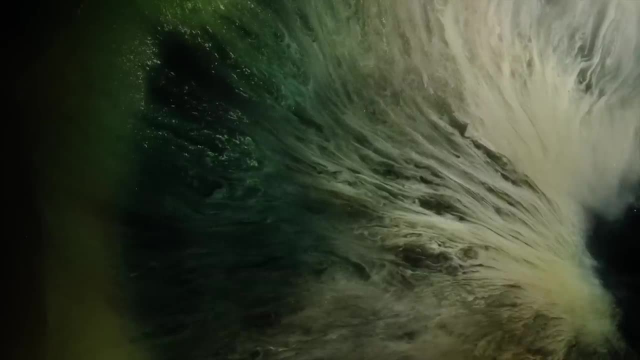 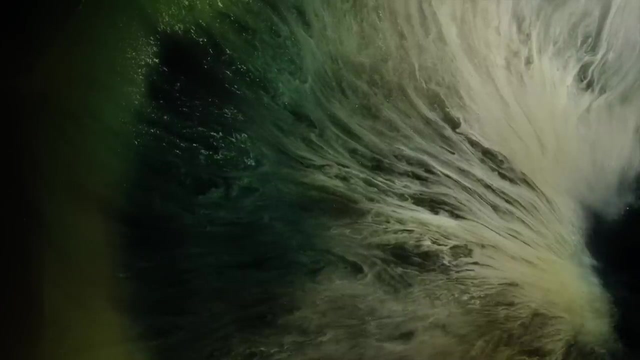 you can end up with two black holes at the center, the center, the center. see, the black holes would merge very. see, the black holes would merge very. see, the black holes would merge very quickly. but that doesn't happen very quickly, but that doesn't happen very quickly, but that doesn't happen very quickly. so you can have two. 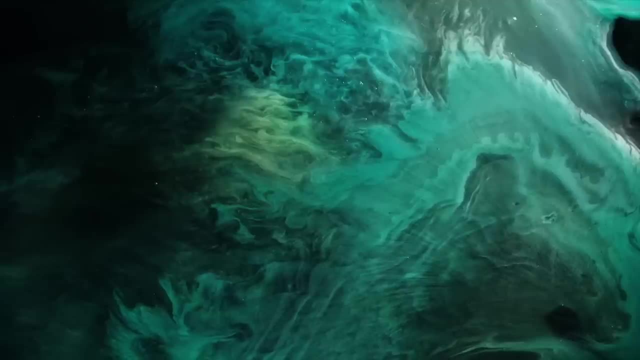 quickly, so you can have two quickly, so you can have two. and people are looking for search and people are looking for search and people are looking for search objects and objects and objects. and when those mergers occur, then when those mergers occur, then when those mergers occur, then we can actually measure the 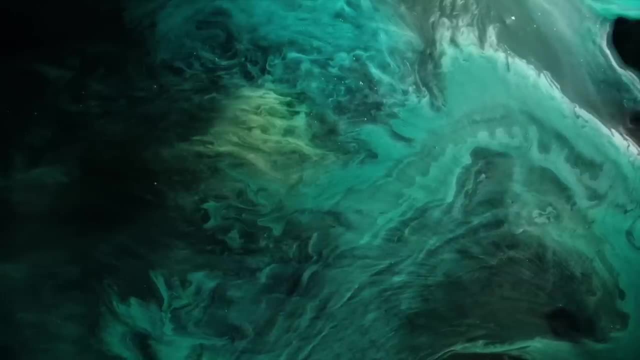 we can actually measure the, we can actually measure the gravitational waves from them, if we gravitational waves from them, if we gravitational waves from them, if we have instruments capable of doing so, have instruments capable of doing so, have instruments capable of doing so, the ligo instrument and, by the way, 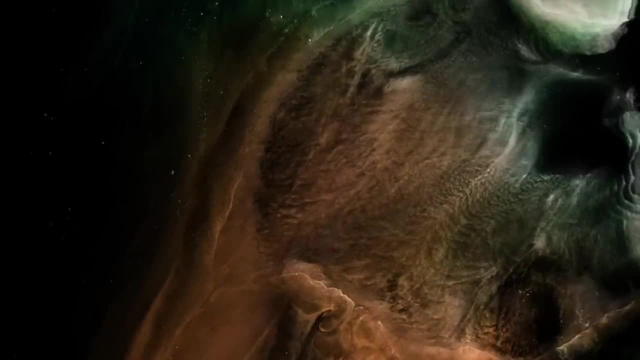 the ligo instrument and, by the way, the ligo instrument. and, by the way, there is uh like ligo india. uh, there is uh like ligo india. uh, there is uh like ligo india. uh, india is going to have a ligo project. um, india is going to have a ligo project. um, 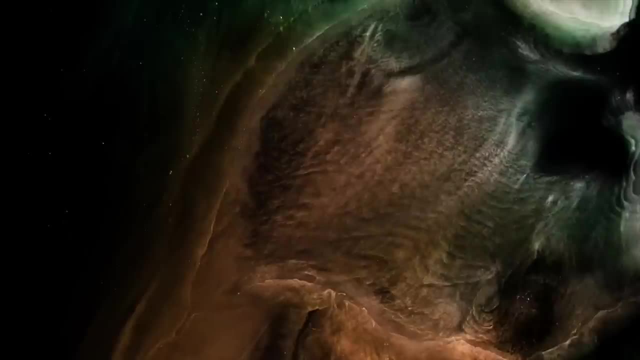 india is going to have a ligo project um, pres i i hope up and running by 2025. pres i i hope up and running by 2025. pres i i hope up and running by 2025. but um to measure mergers of black. 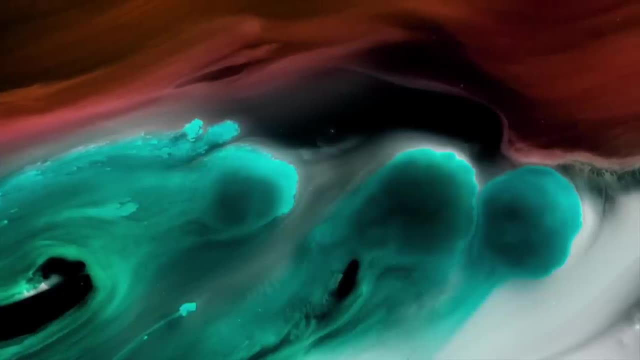 but um to measure mergers of black, but um to measure mergers of black. supermassive black holes. you need to supermassive black holes. you need to supermassive black holes. you need to have uh to be able to operate at much. have uh to be able to operate at much. 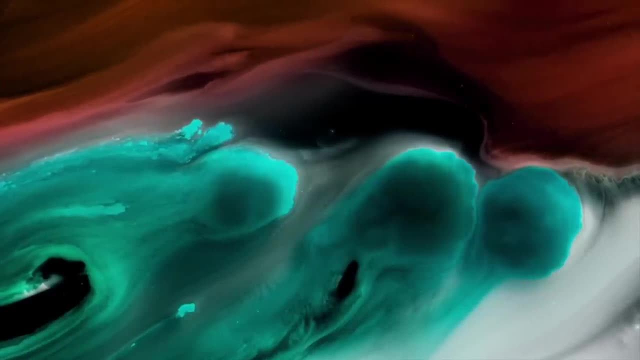 have, uh, to be able to operate at much lower frequencies which you can't on the lower frequencies which you can't on the lower frequencies which you can't on the surface of the earth. so you need to surface of the earth, so you need to surface of the earth, so you need to go into space. 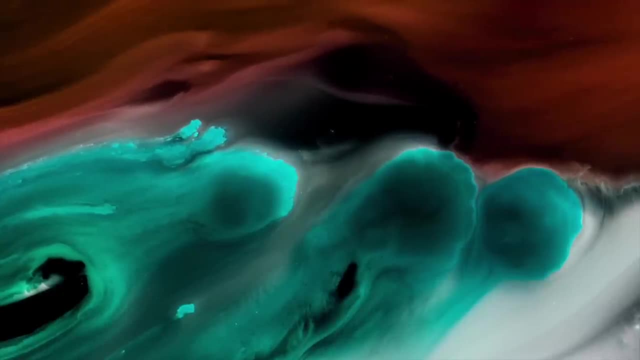 go into space. go into space and lisa: uh sorry, uh, isa european and lisa. uh sorry, uh, isa european and lisa. uh sorry, uh, isa. european space agency has a planned space agency, has a planned space agency, has a planned mission in the 2030s called lisa, which. 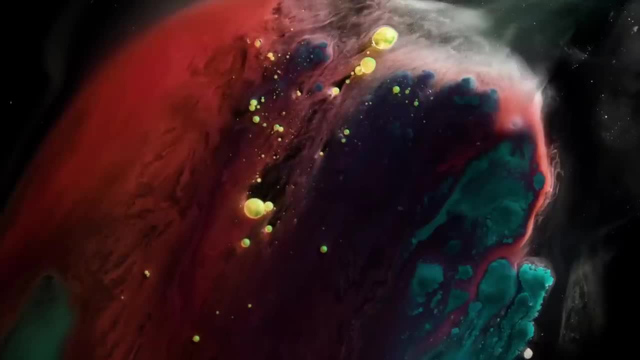 mission in the 2030s called lisa, which mission in the 2030s called lisa, which will measure such such things and will measure such such things and will measure such such things, and mergers of binary black holes is one of. mergers of binary black holes is one of. 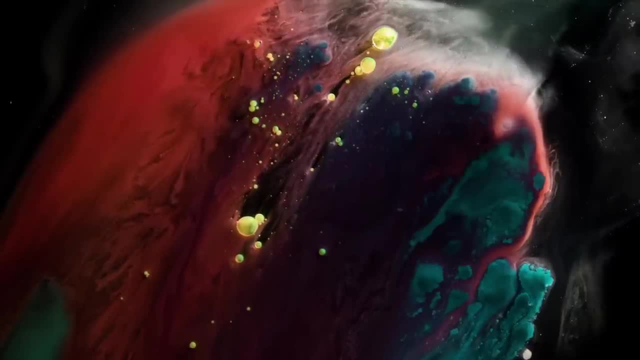 mergers of binary black holes is one of the top things to do. thank you, professor fabian, for such. thank you, professor fabian, for such. thank you, professor fabian, for such comprehensive explanations. thank you so comprehensive explanations. thank you so comprehensive explanations. thank you so much. 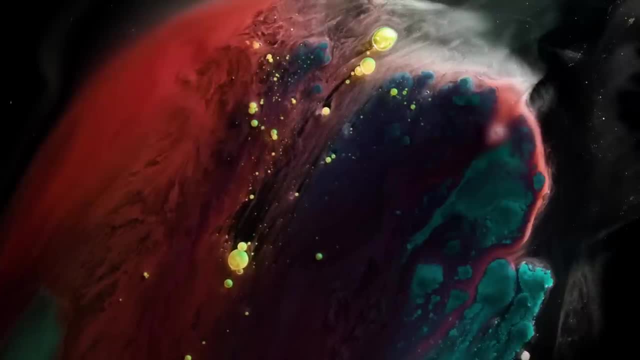 much, much over to manage. thank you, thank you very over to manage. thank you, thank you very over to manage. thank you, thank you very much, professor fabian. much professor fabian, much professor fabian. uh, any concluding remarks from your side? uh, any concluding remarks from your side. 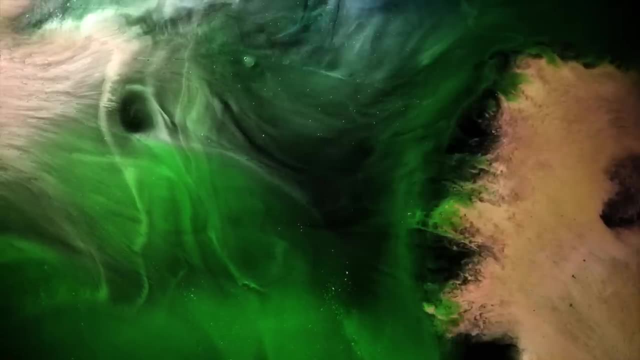 uh, any concluding remarks from your side, and then i'll close the session. and then i'll close the session. and then i'll close the session. thanking for the opportunity to talk to. thanking for the opportunity to talk to, thanking for the opportunity to talk to a large number.